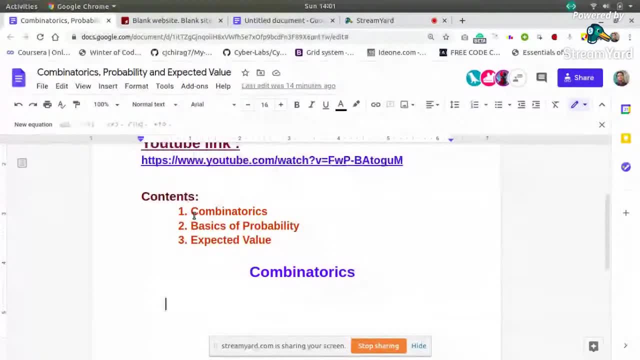 some normal, some easy, some problems, some of the easy problems also. So, okay, let us begin. So, first of all, let us start with one of the basic things of combinatorics, which you all might be knowing, but still I should tell you so that, okay, so one thing. 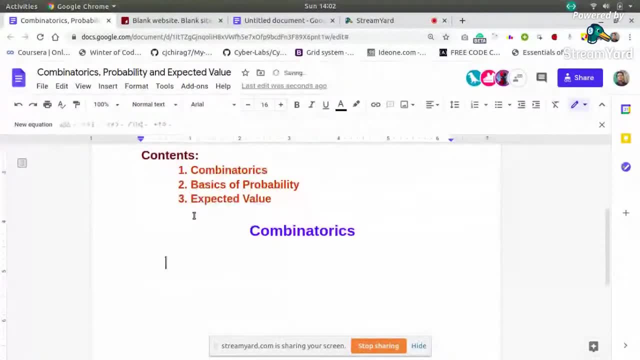 is like one is SUM rule and one is product rule, Product rule and one is SUM rule. So product rule is saying that suppose you have to do, you have to do two jobs, one one is job A and one is job B, such that Job A can be done in some m ways and job B can be done in some n ways. 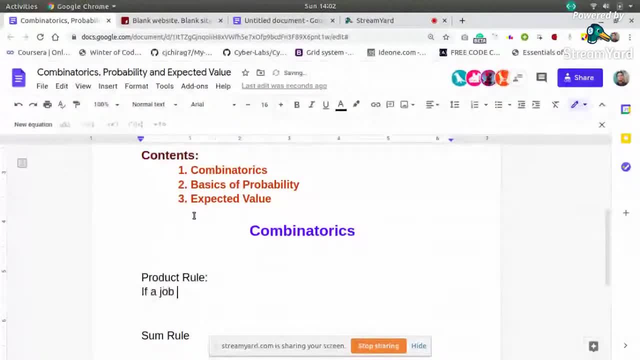 So it is something like if any job or anything A can be done in m ways and after that, after performing once, you have done the job A, now, after that, after it is done, you have to do some job B which can be done in another job B can be done in some m ways and n ways. let us say: 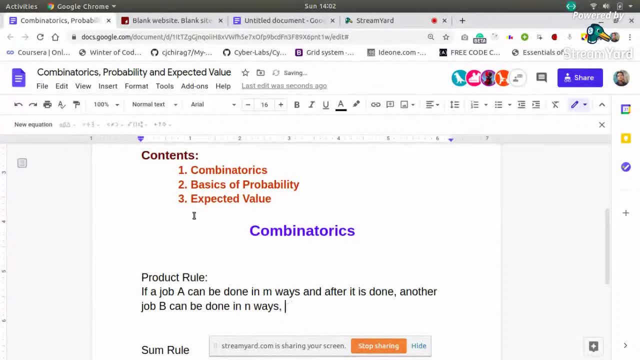 So what is the total number of ways? total number of ways, if this is the condition, then total number of ways to perform or to do both, means to do both, to do both A and B- is m multiplied by n in, m multiplied by n ways. 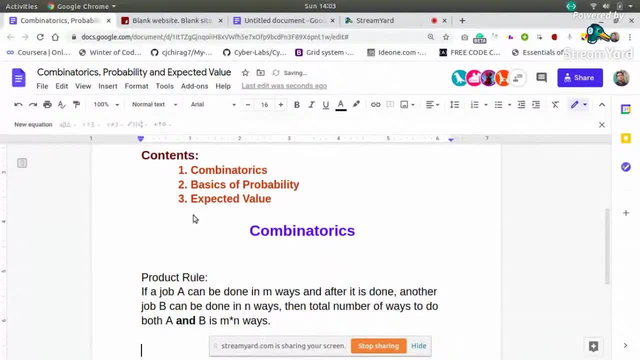 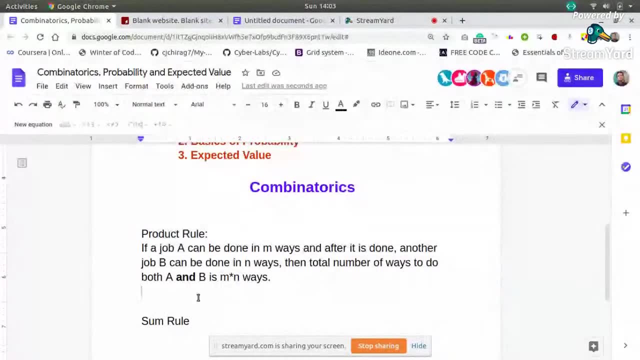 So, because sometimes it happens when you are solving problems related to dynamic programming or some of the topics in which combinatorics is involved, So sometimes People confuse when it will be multiplied and when it will be added. So this is very uh means, foundation, uh, foundational thing, basic thing which you should know whenever something some of the you need to perform two tasks and such that you need to perform both of the tasks. 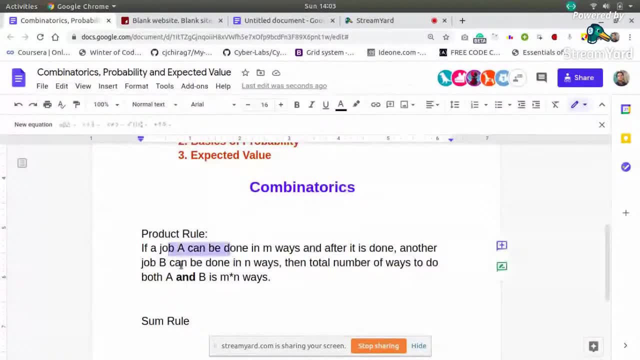 And you can say that after one task is performed, then you perform the second task. It is like that. So whenever such a thing is there, that time you multiply things to get the number of ways. So I will give you an example. it becomes more clear. 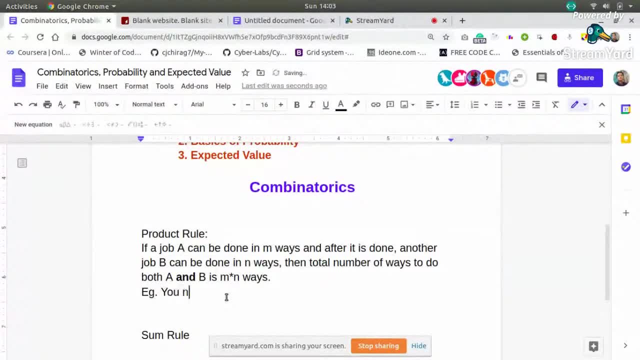 So let us say, let us say you have to uh, uh, you need to form a team of uh. let us say of one, uh, you need to form a team for ICPC. ICPC, all might be knowing is a competitive programming like, like Olympics of competitive programming. 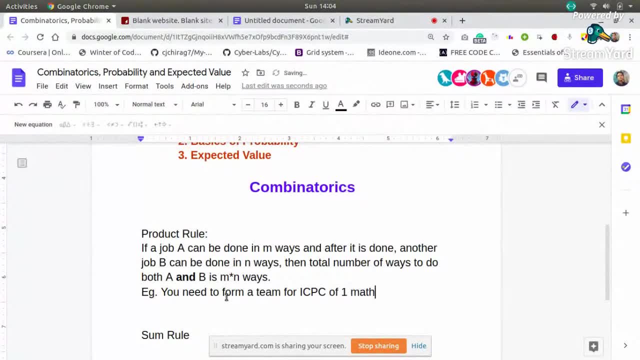 So you have to form a team for that, and it should contain one mathematician and one programmer. And let us say it should contain one uh. what to say when? uh, let us say one uh gamer. Okay, So, and, and there are total, uh, there are total, let us say, 10 mathematicians and 15 programmers and, uh, five gamers in your college. 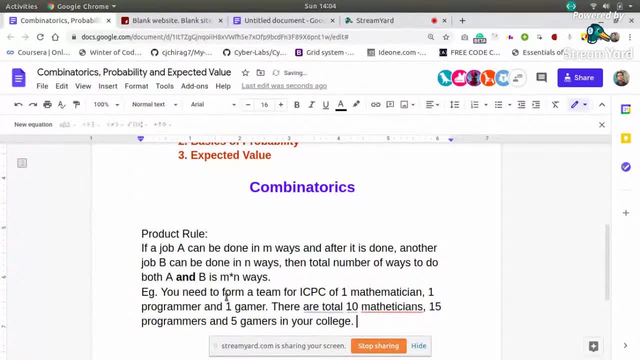 Let us say: now need uh, now uh. you need to answer in how many ways? how many ways uh can you form your team? Can you form a team? So the number of ways in which you can form your team. 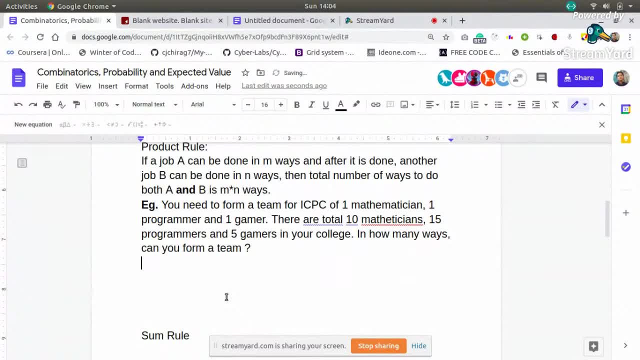 Try to answer. So try to break it in parts Like: uh, if you want to form a team, you need one mathematician. So how many ways you can get one mathematician? So, uh, try to answer in live chat. if you know, if you know how to calculate it, it's easy. 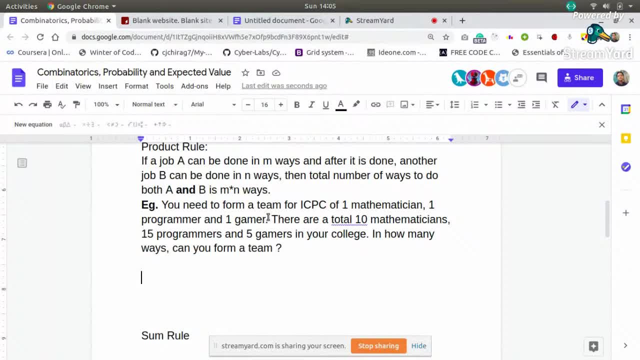 Like: uh, you need to select first one mathematician. So how, in how many ways can you select? You have total 10 mathematicians. So obviously in 10 ways you can select. Okay, Mathematician. in 10 ways, select a mathematician. 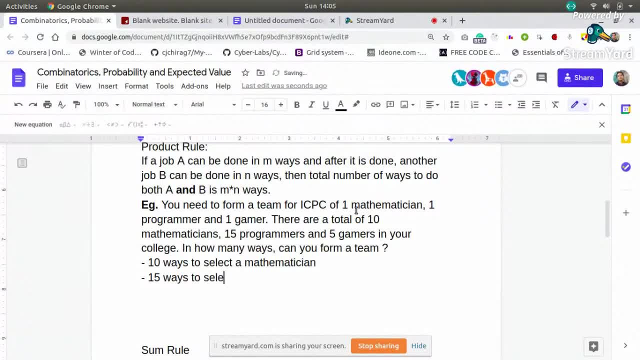 And uh, if you have- and you have five ways to select a programmer, and you have again five ways to select a gamer- Now here we need to select all of them here. And is important means every task we need to do. 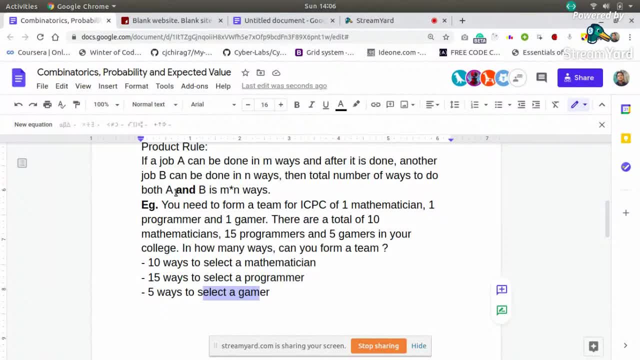 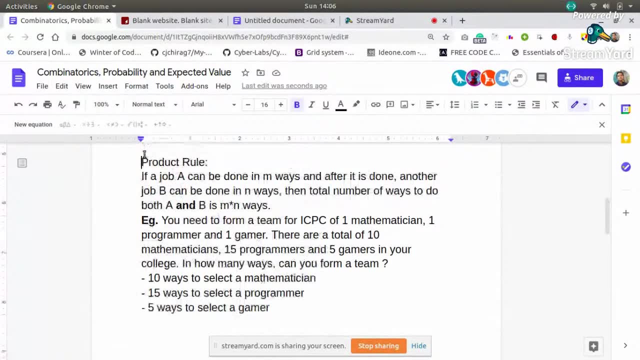 We need to first select a mathematician, then a programmer, then a gamer. So Everything we need to do, and is there, So we multiply these. We are not adding them by because and is there, So product rules say: multiply them to get the total number of ways to do all of them. 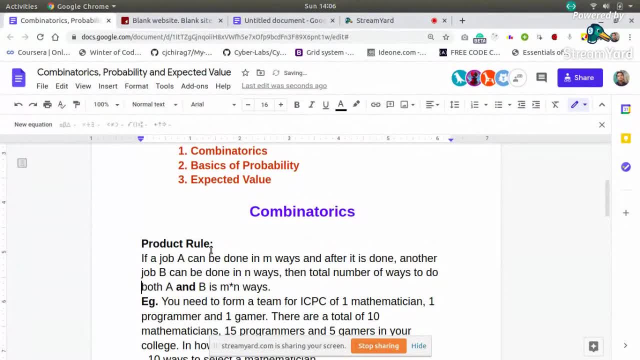 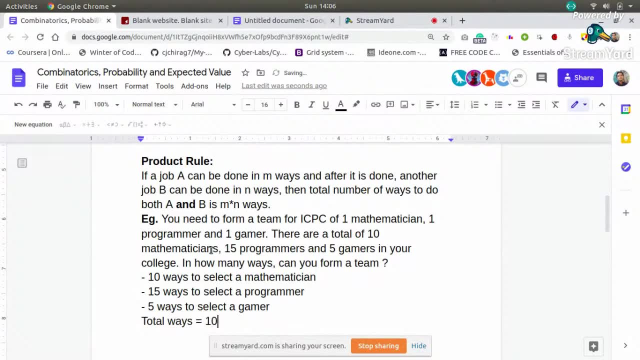 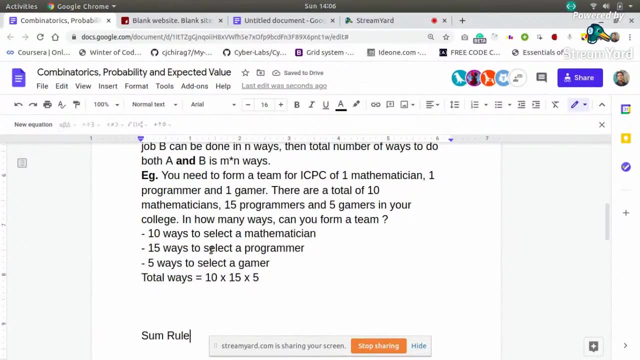 So we will multiply them to get the total number of ways. So the total number of ways will be 15 into 10, into five. total ways, uh, equals to 10 into 15, into five. Fine, Now let us consider the same sum rule. 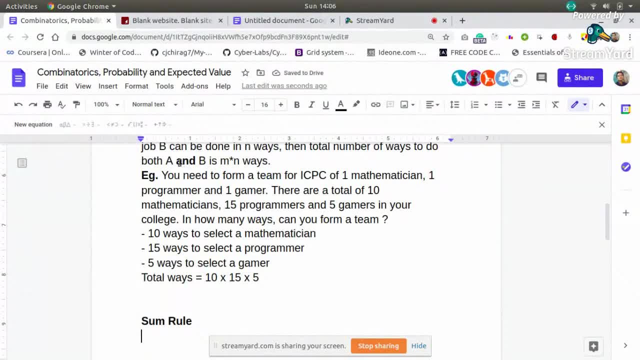 So some rule, some rule is just similar to that, but instead of and or is there. so it is like you need to perform two tasks, but you need to do any one of them. Uh break or a voice, Yeah. 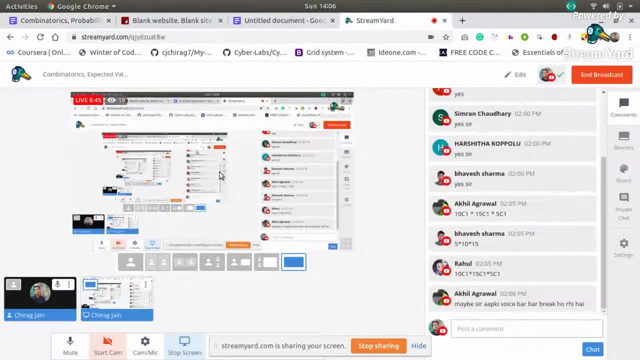 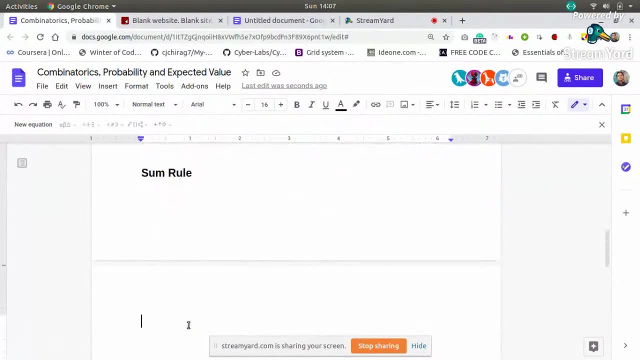 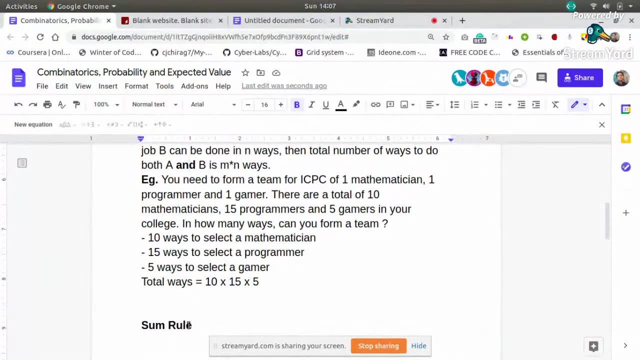 Okay, Uh, I think, Hmm, Take it, Uh, I got a break with the batana. Okay, So if a job can be done, Uh, in N ways and another job can be done in N ways and you need to do only one of them, 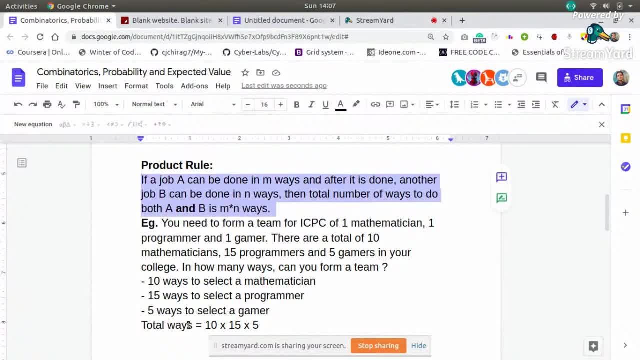 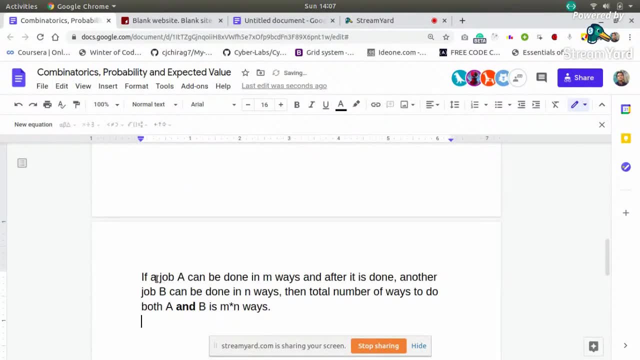 So, like similar to the above, but anyone you need to do, so that the answer for that will be M plus N, like you need to do, uh, if a job- I am a, can be done in M ways And uh after it and another job, B, can be done in M ways and ways, and then the total number of ways to do either A or B. 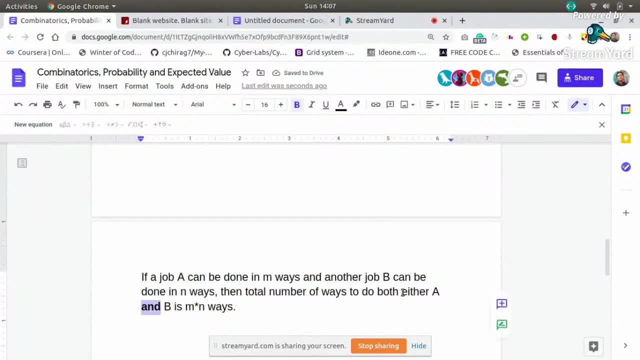 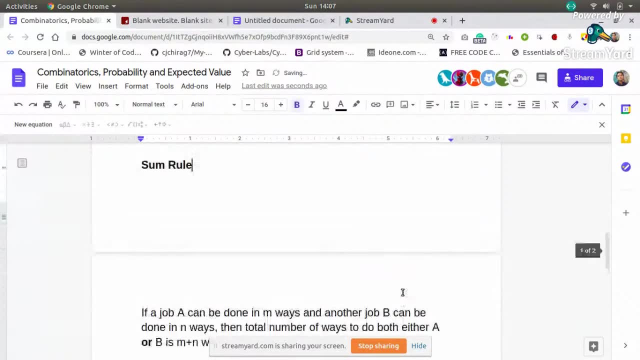 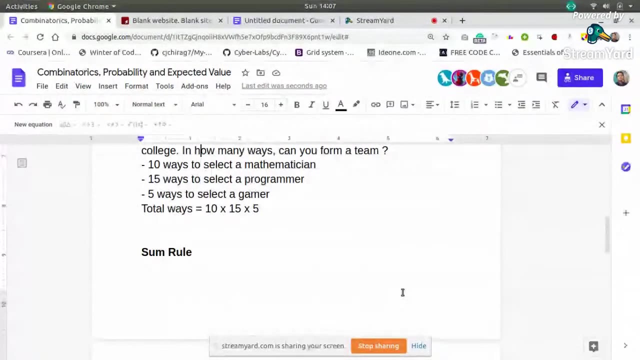 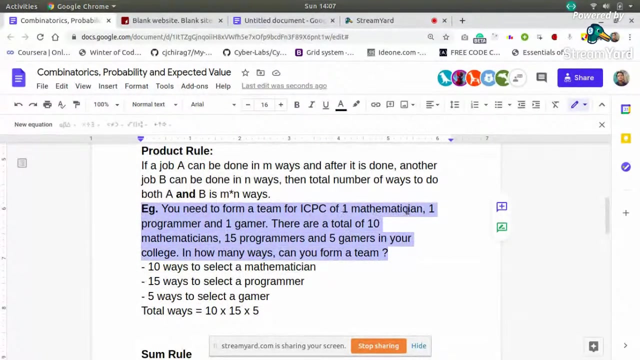 And so you select any one. you need to do any one of them to either a or B his M plus N, M plus N ways. So this is the summary. Okay, So if we have the same things, if we have the heart-ierto, if we have the same question, but now the question is lettable, but change that you need any one of them, either a mathematician or a programmer or a gamer. So what will be your answer? to perform the number of ways to, To form a number of ways, So um, let's start with one with keyword. So um, where do I start with a keyword? What I would say is that, Inside of this, 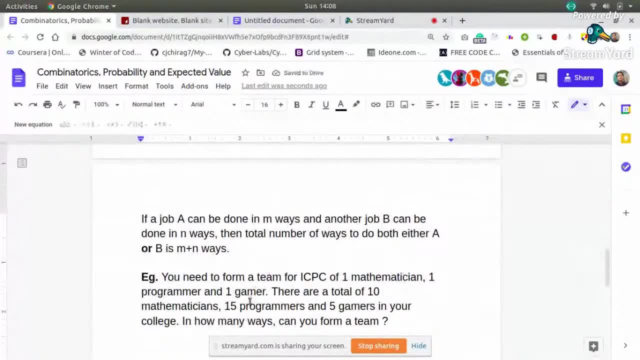 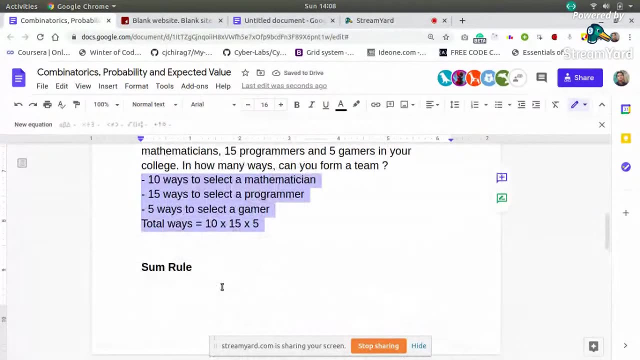 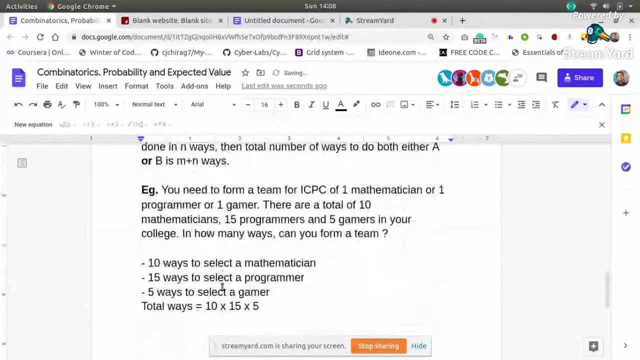 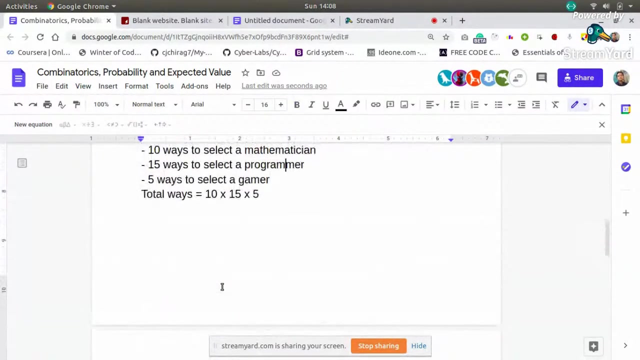 a team. so you need, okay, so you need to form a team for icpc of one method imitation, or one programmer or one gamer, anyone you need. so what should be your answer? 10 plus 15 plus 5, right, so your answer would be 30. okay, 30 ways are there. so, uh, this is one of the basic thing and uh, similarly, you can also. 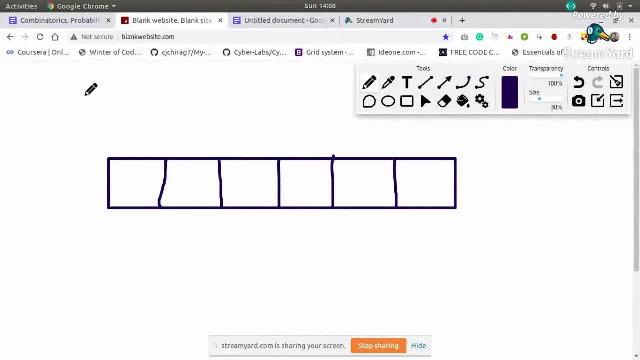 consider one more example, if you want, suppose, suppose the you are at a and to go to b there are m ways, and from b to c. if you want to go from b to c, then there are n ways to how many ways to go from a to c. so the answer would be: first, you need to go to b in m ways. anyways, you can go in. 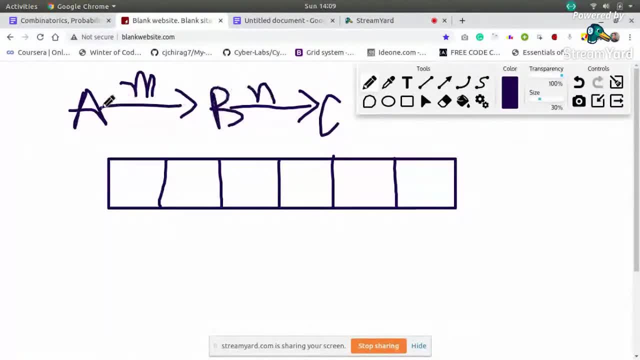 and then you. after that, you need to go to n, so you need to go both. uh, you need to first go to this and eight, from a to b, then b to c, so you need to perform both of the tasks. to multiply, multiplication would be there. so, uh, the answer of this would be m into n, m into n. ways are there to. 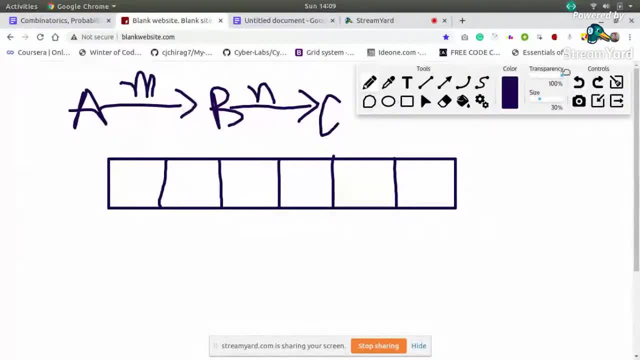 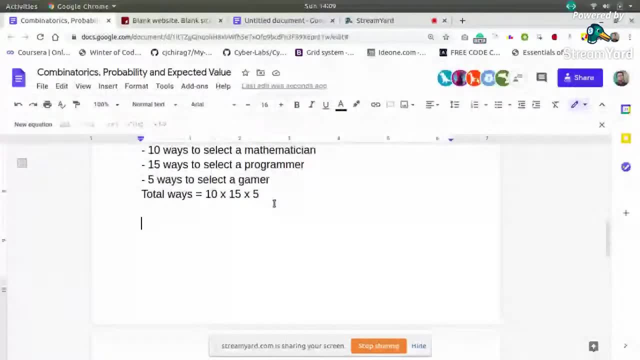 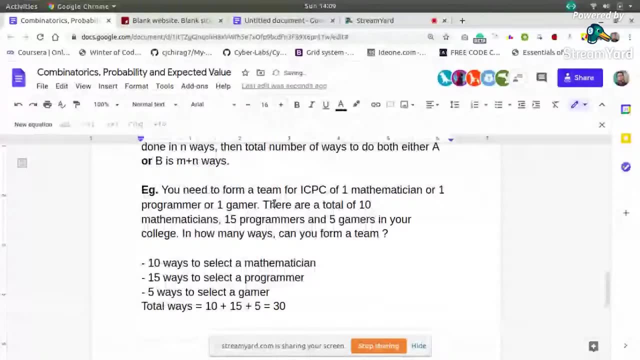 reach c from a take care. so one more example. this was so. i hope it should be clear now. so when to multiply and when to add, take care now. uh, let us take one more example for take one more. let us see one more thing, like: if you want to arrange n. 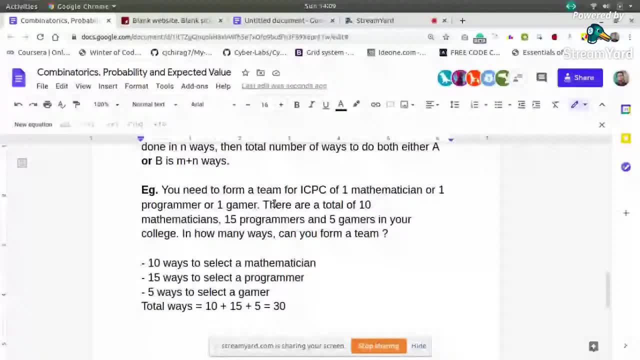 things, uh. so number of ways, number of ways to arrange, arrange n people. let us say, arrange in any people, so here we need to, uh, and people are standing somewhere so you need to arrange them. what are the number of ways to do that and distinct people you can say. 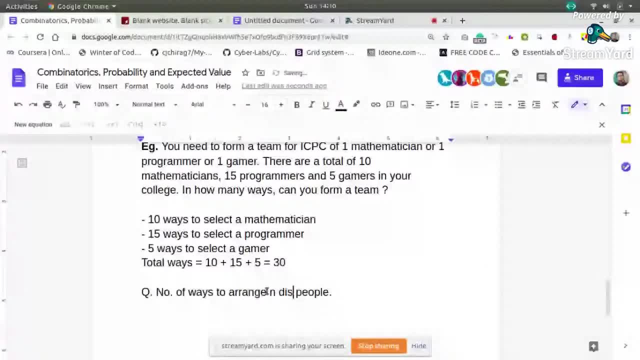 people, all the people are different people and distinct objects. also, you can say anything you can take, so how many ways are there to arrange them? so, uh, try to answer. if you know there are n distinct objects or people and you need to arrange them, what is the number of ways to do so? 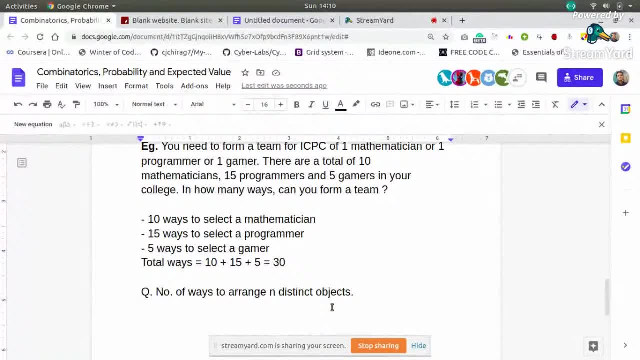 it okay, so this is also simple. you can also see this by using product rules, like if you see the product rule uh, so we can break the things into smaller uh tasks. so like we need to arrange and objects and factorials. you know how n factorial comes. so its simple way is to: 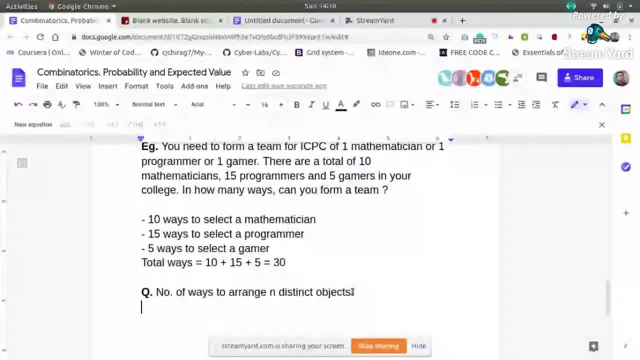 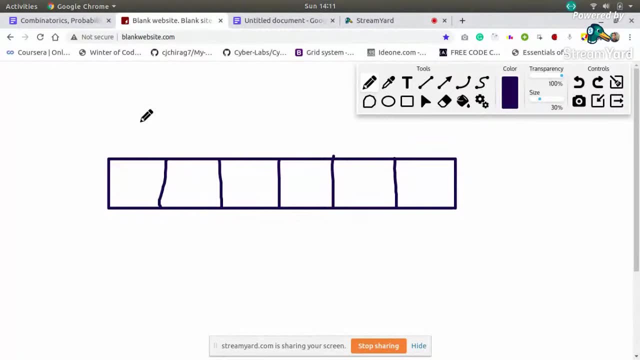 just consider the first person. so suppose there are n places, there will be n places total. so first person can, uh, can, be occupying any one place. so what are the number of ways to arrange the first person? so there are n ways for the first person. okay, so there are n ways for the first person. 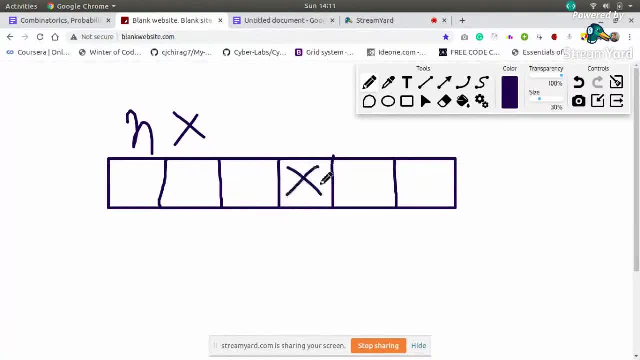 okay, guys, you can go into the field, ok. so now let's say i have here over here, right here, this: i have one split of 1. okay, now first person is fixed somewhere, so let us say i affect the first person here, so this place is occupied by someone. now there are n. 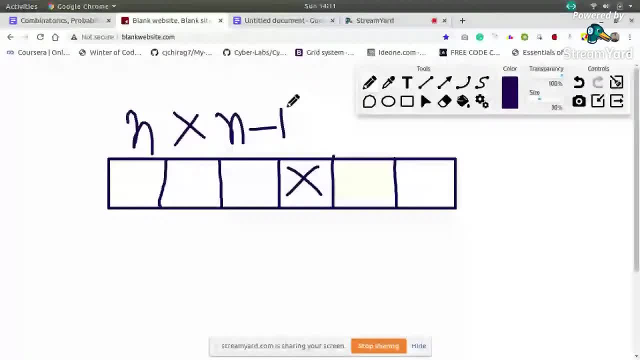 minus one places left. so for the second person there are n minus one ways to get n1 seed. similarly, suppose now second person is also occupied, any other seed and it may be anything. now let the seeds left would be n minus two. so for the third person n minus two seeds are available in. 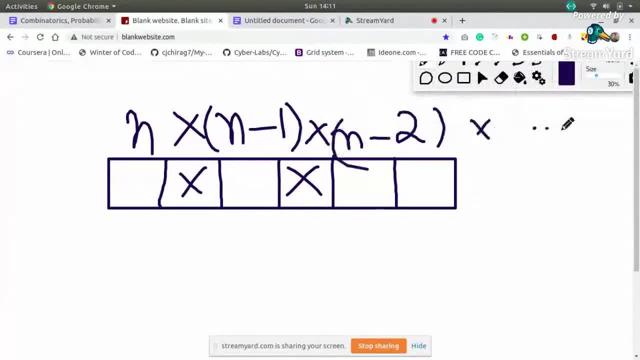 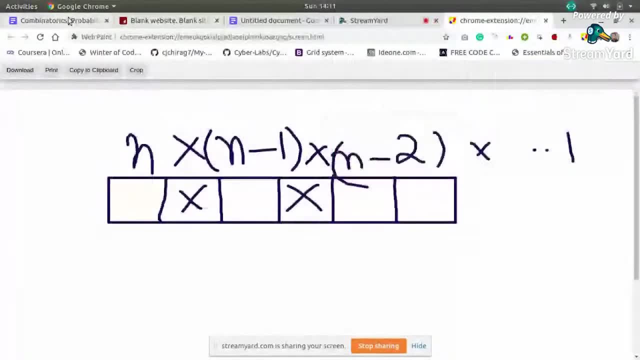 this way, if you continue this series, if you continue with this multiplication, you will get n minus one, so for will get that. uh, until you need to do up to one. so this is called factorial, n factorial. okay, so the answer would be n factorial, so this is also called n factorial. 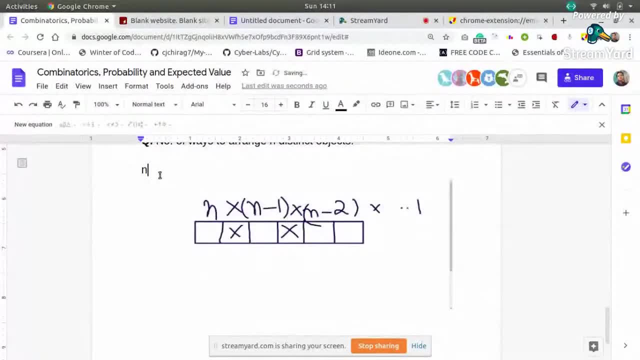 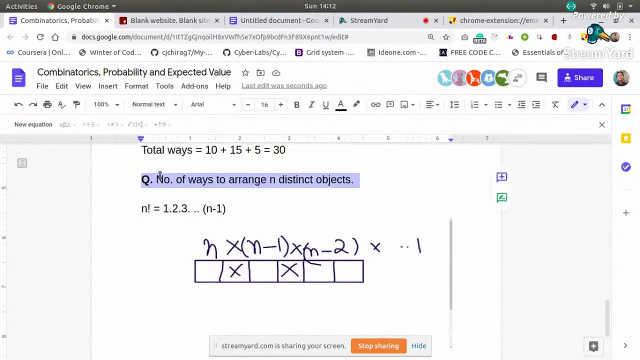 so it is n. you can see n factorial or n factorial can also be written as 1 into 2, into 3, into up to n minus 1. in the reverse you also can write anything. so now, uh, this is number of ways to arrange distinct people. now suppose you have something like this. so, uh, you have, i want to. 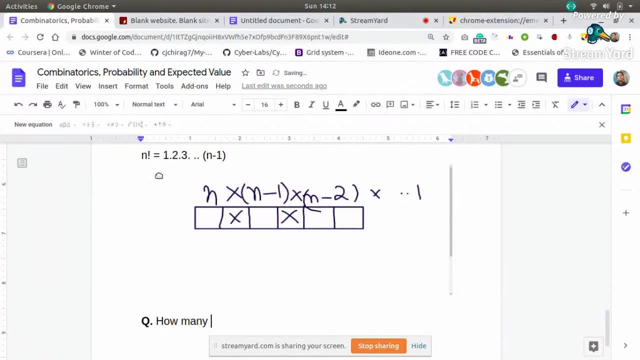 ask you how many, uh, uh, how many ways, how many different arrangements of of this set of letters is possible. so you have a set of later letters and you can arrange them in any ways you want. so these are the set of letters: a, a, b, b, b, c, c, c, c, something like this. so there, how many arrangements are possible? 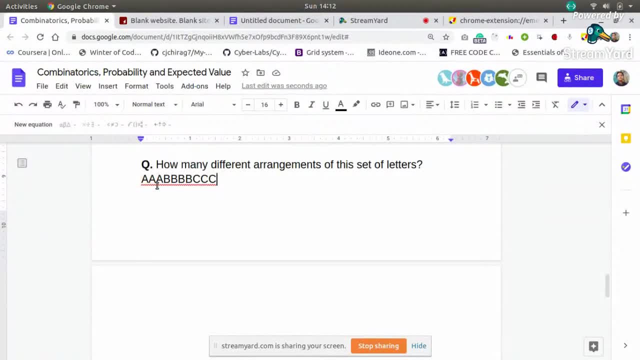 so there are three a's, four b and three c, so you can arrange them in any way like one. one arrangement can be uh, a, one like this. one a can be at the last something. this is one arrangement. one arrangement is something like c. this c can be here. 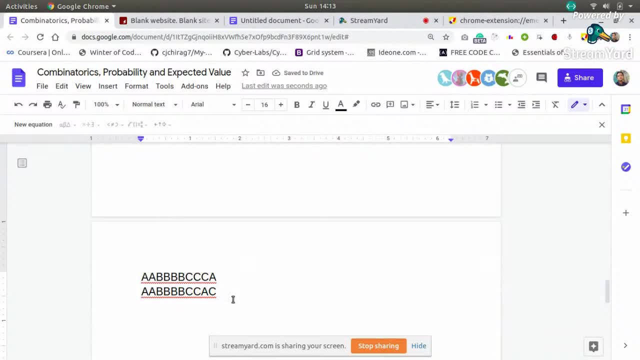 so the total number of a's and b's and c should be same, but in how many ways you can arrange them? so there are here three a's, four b's and three c's. you know that if different, if, if this, these all characters were different, let us say then: 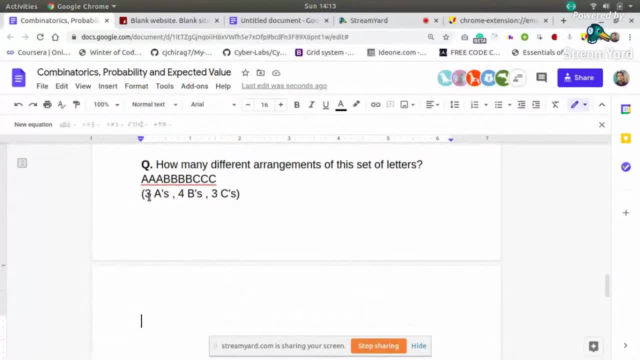 what are. what would be the total number of ways? that would be three plus four plus three means there are total 10 characters. so 10 factorial will be the total number of ways if they were different. but since these three are same, so these three can be arranged in themselves. 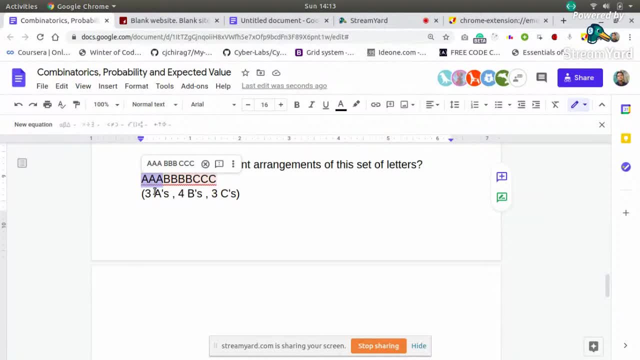 in three factorial ways. so we will divide by that, because we need to. we need not count that. so the answer would be: 10 factorial divided by three factorial multiplied by, multiplied by four factorial multiplied by three factorial. okay, why? because these three are equal, these three are same thing. so they are there. uh, you can say their uh arrangement, do not matter. 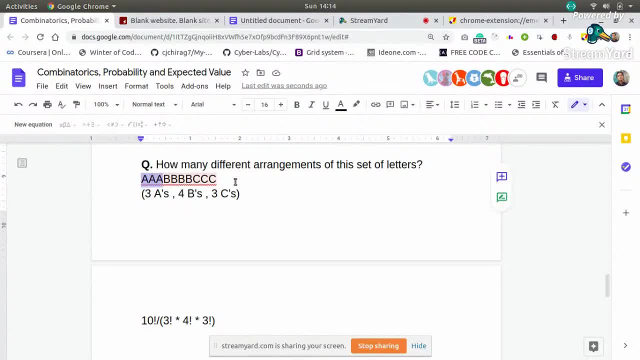 so they can be arranged in three factorial ways, so we need to divide it by that. so, similarly, because these are same, this will let these four are same. so i divide by four factorial. similarly, these three are same, i divide by three factorial like this: okay, total number of ways if they were. 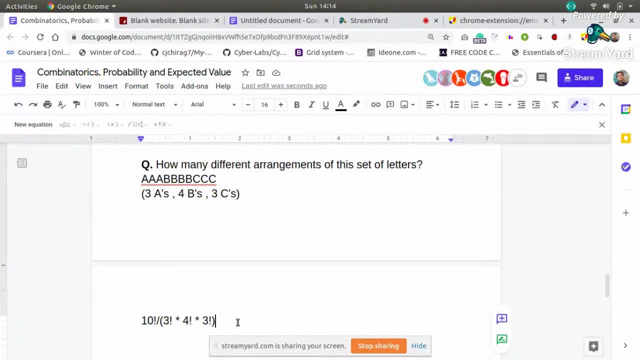 different, then the total number of ways was only 10: factorial, but since some of them are same, so i divide it by this. so this is one more type of problem now. uh, let us see like, uh, okay, so, okay, so, let us come to permutation and combination. so like, permutation and combination, and uh, you all. 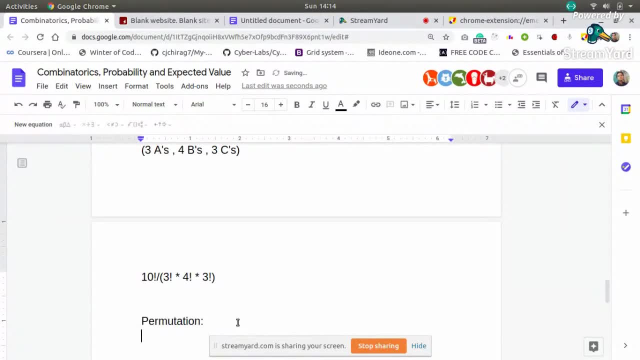 might be knowing. so what is permutation? so permutation means like, if you are given an uh, if you are given n objects, like uh, if n objects are there, we need to select any ordering of our object, but you need only our objects and their order matters, so you can say: order matters. 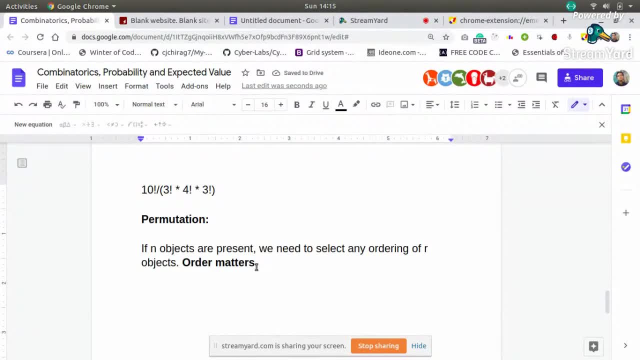 so what would be the number of ways to do this? like it can be anything. you have n objects and you need to select our objects, but their order matters in. in what order you are selecting them, that thing matters. so try to calculate in the similar way. like the first object, you have to have an object, and then 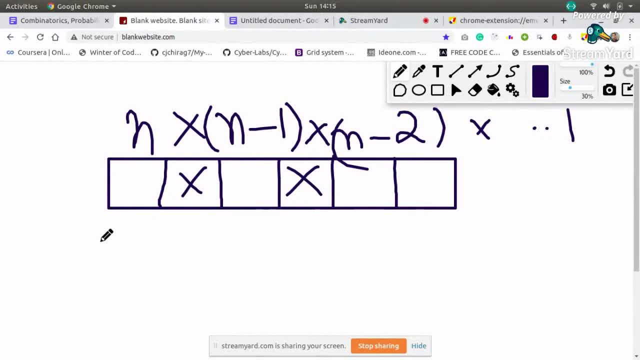 it can be anything. so first, the first object can be selected in n ways. if you need to select our object, then the first can be selected in anyways. second: now one object is selected, how many are remaining? n minus one. the second object can be in any of the n minus one thing. so there are n. 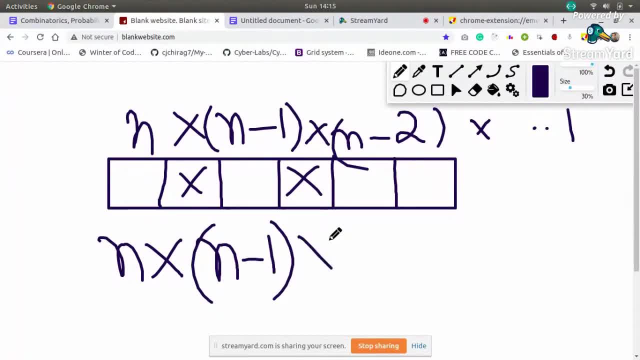 n minus one ways to select the second object. now for the third object, you have. how many objects are remaining? two have already been selected. so how many are remaining? two? n minus two are remaining. so for the third object, there are n minus two ways. similarly so on. you keep on doing this up to how? 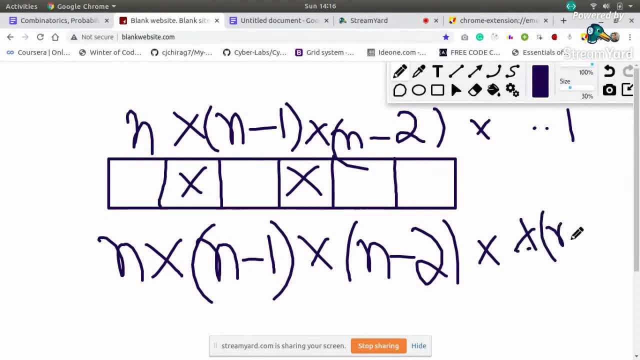 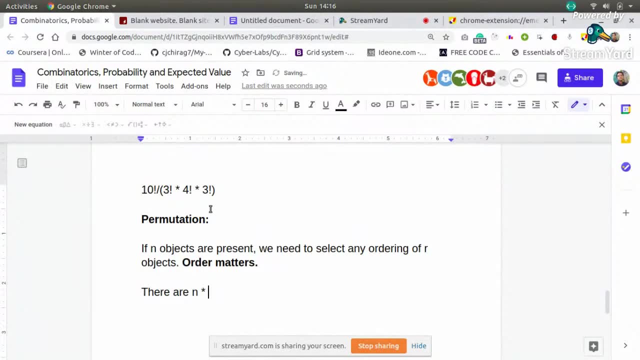 many times uh until you get n minus r plus one. okay, so this is called uh npr or n permutation r. so this is uh n multiplied by n minus one. so on, you do uh for n minus two and up to n my n minus r plus one. 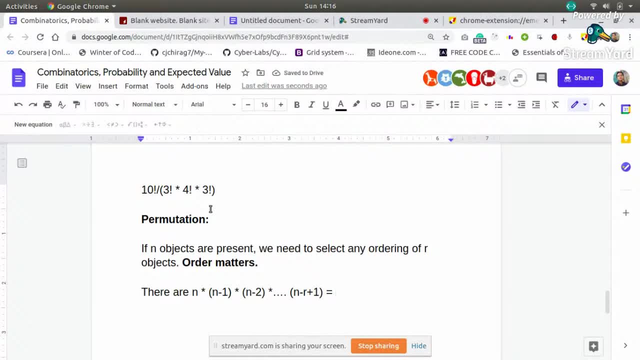 okay, so this is also called like uh. you can call it n. factorial means if you go by the formula, it is nothing but n factorial divided by n minus r factorial, because if you try to solve this so you will get that. you will get this this term only. so this is also called uh npr. 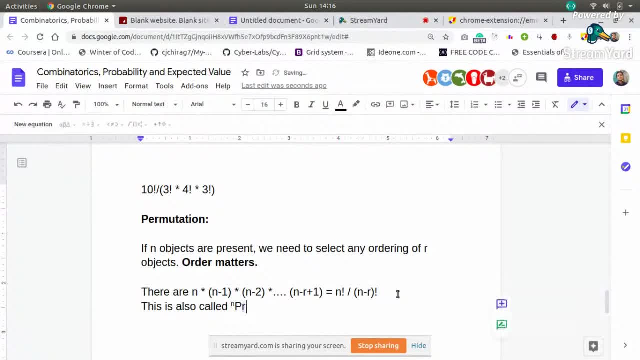 okay, this n can be in the subscript and this uh, if you want, then this r can be in the superscript. so this is npr, so this is permutation, now, uh, now, here it was, the order was mattering. but suppose the order doesn't matter then, then that will be called combination. so suppose the order doesn't matter. 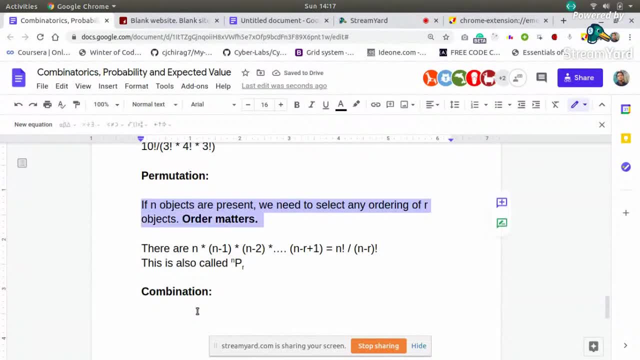 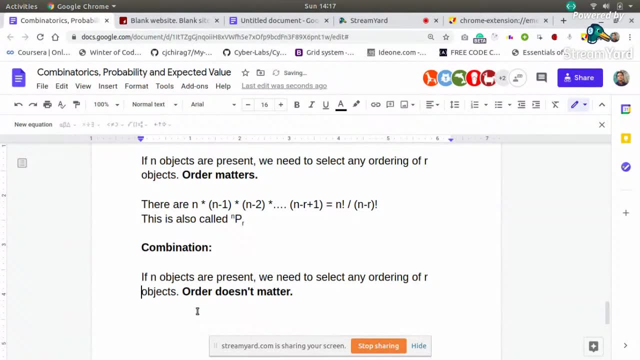 the question is saying there are n objects, you need to select any r of them, but the order doesn't matter any. in any order you can select them. so order doesn't matter this time. select any of the r objects, select, uh, uh, any r objects. so just the team matters, just the group. 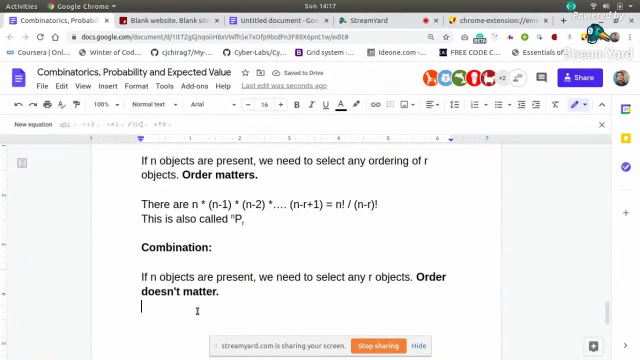 of objects matter. you can say that, uh, earlier we needed to select any particular sequence or order, but now in, uh, you need to just provide the r objects. who are the r objects? just you need to give them. so what would be the number of ways to do this? try to answer, let's see. let's see. 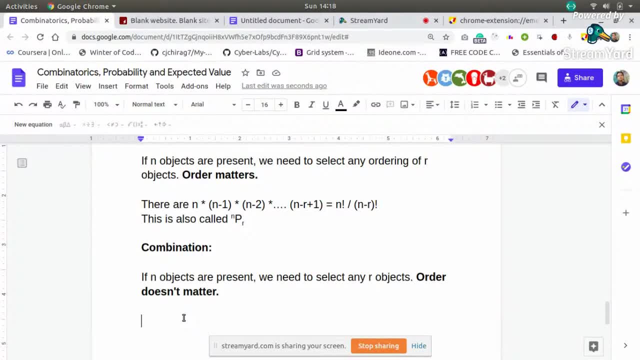 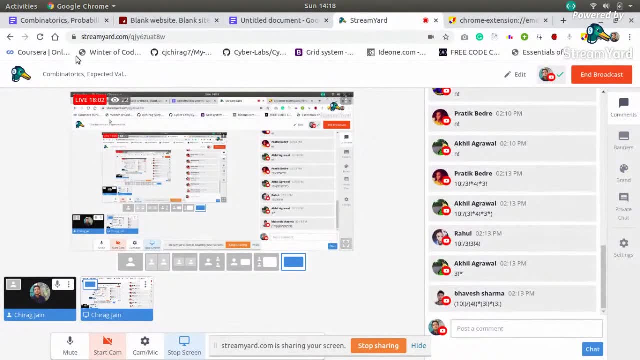 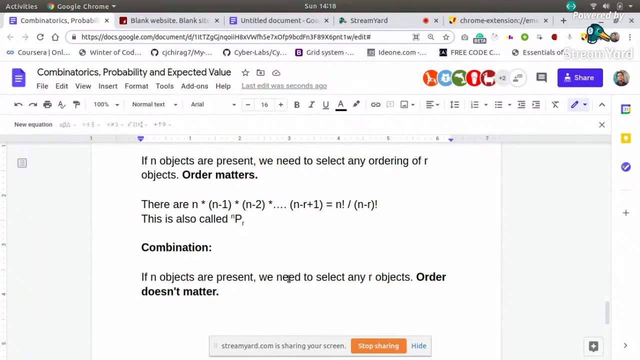 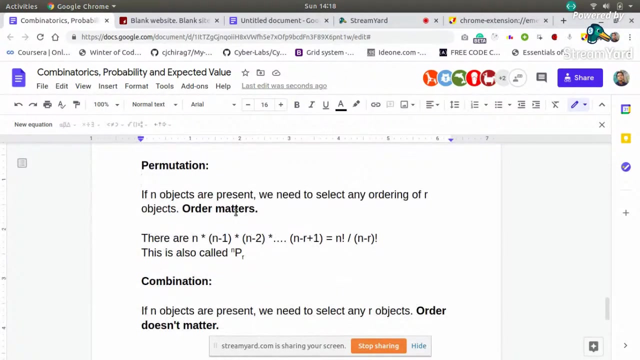 try to answer. hello, onds select. uh, any ordering, when order matters. the answer was n, factorial, divided by and minus our activity, this thing. but here the order doesn't matter. so it means that suppose we have, suppose we have selected the r objects in multiple orders, but we want to consider the 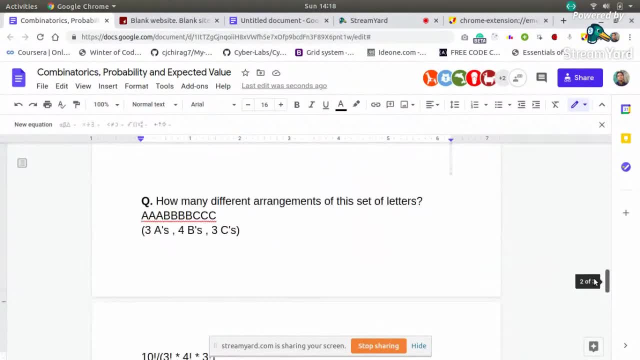 consider them as the same. so what we did earlier, whenever we had uh means whenever we need to arrange like and are. and what are the changes? um, if we do supply on late? the Ayyub means whenever we need to arrange like and r and r are in multiple orders, but we want to consider dem as the same. so what we did earlier, when ever we had, means whenever we need to arrange like and r and are in to many people subگraft. 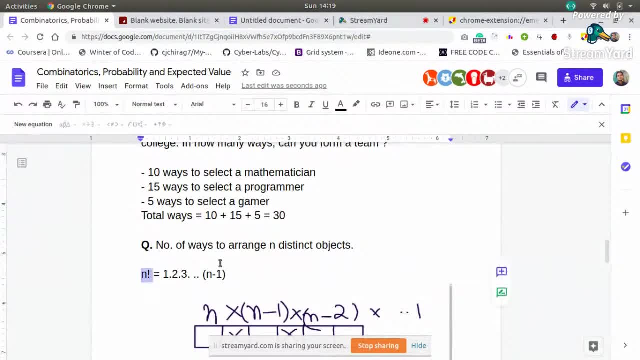 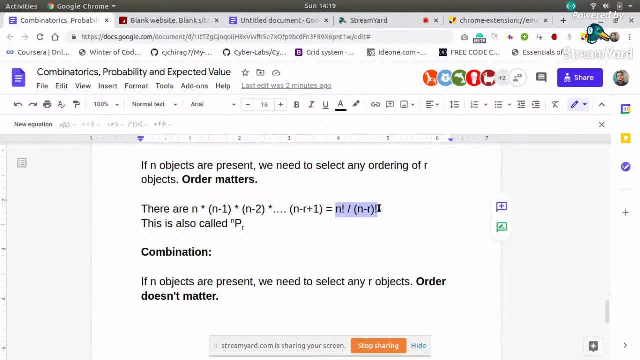 distinct people or n distinct object. the number of ways to arrange them was n factorial. Suppose I have selected any ordering of the r people, So it can be any of the ways in this. In these ways I can select r people, But there means ordering can be different. 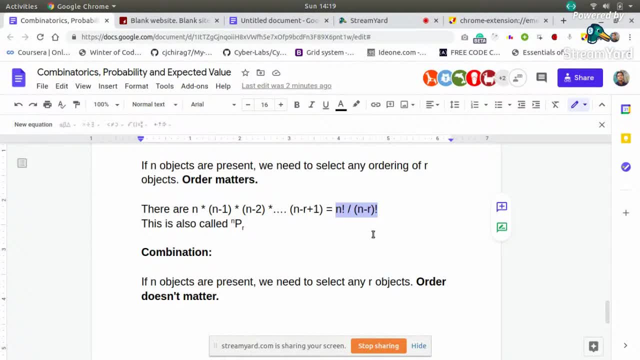 Here order matters, So I need to consider all of them same. So those r people which I have selected can be arranged in r factorial ways. So I will divide my answer by r factorial. So you can say this thing would always also be divided by r factorial multiplied by r. 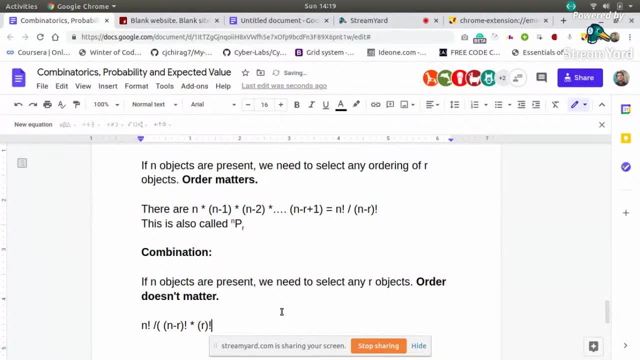 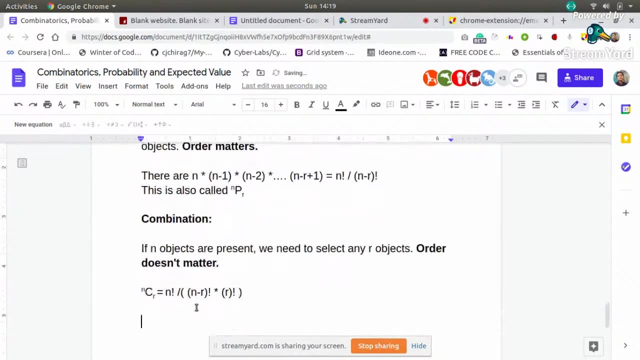 factorial. So this is ncr, This was npr and this is ncr How this came, Just npr. divided by r factorial, Because those r people can be arranged in r factorial ways. So this is npr and this is ncr How this came, Just npr. divided by r factorial, because those r people can be. 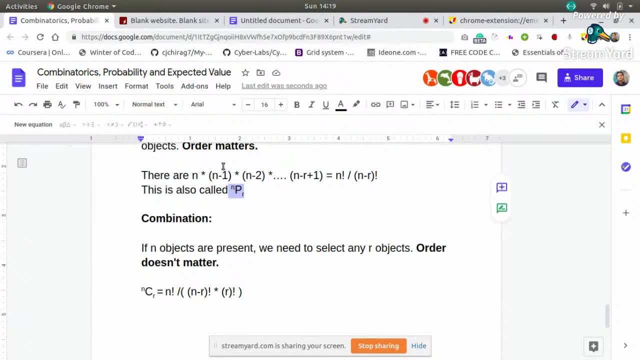 sorted by r factorial And the time is third column. These r people which I have selected can be arranged in r factorial ways, And I need to divide by that, because here the order doesn't matter. So any ordering will work. Any ordering will be considered as one thing. 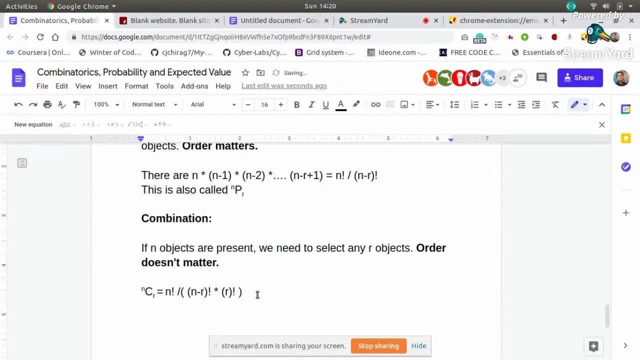 only So I divide it by r- factorial. Okay, So this is combination And now let us look at some of the properties that are useful. So let us say some of the properties are like: first is simple ncr. suppose you have ncr, so ncr will be always. equal to people which I have selected can be arranged in r factorial ways. And let us say some of the properties are like. first is simple ncr. suppose you have ncr, so ncr will be always equal to. 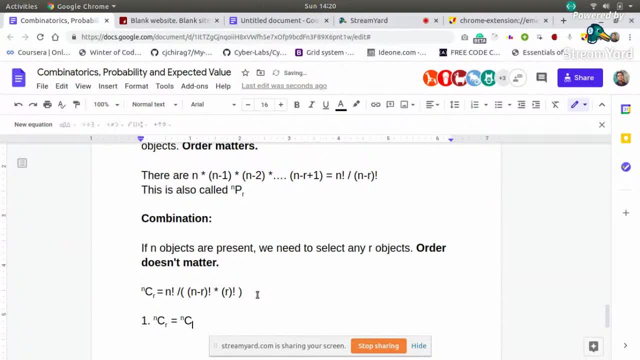 n, c, n minus r. how this come so simple? suppose there are n objects given to you and suppose you selected r, so automatically the remaining objects are also selected. suppose you want to select r people out of n in ncr ways, you can select them, but when you have removed those r person, 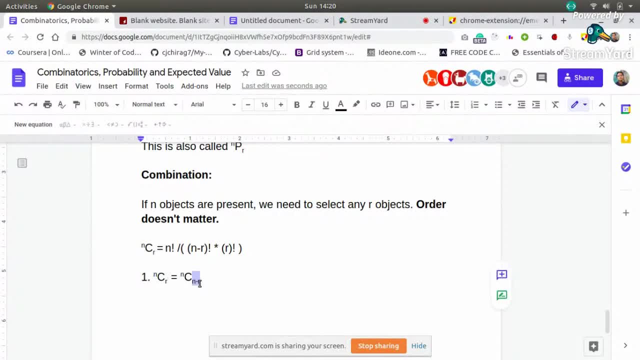 how many you are left with. you are left with n minus r people, so automatically you have selected n minus r people also. so in this way we can say that ncr is always equal to nc, n minus r, or one property is like ncr, which is useful to. 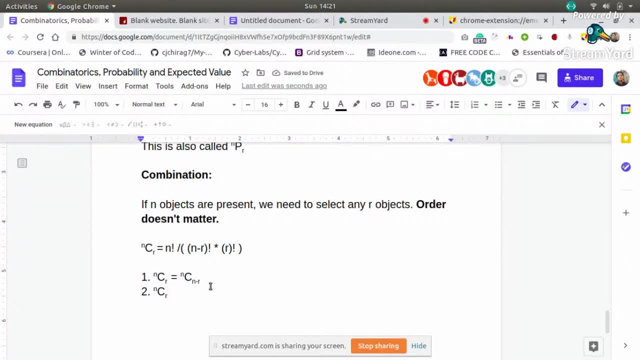 calculate ncr in competitive programming. so which is ncr equals n minus 1 cr, minus 1 plus n minus 1 cr. this is also called Pascal's triangle property, Pascal's triangle property. so how does this come? let us look how this has come, so you do not need to remember this. 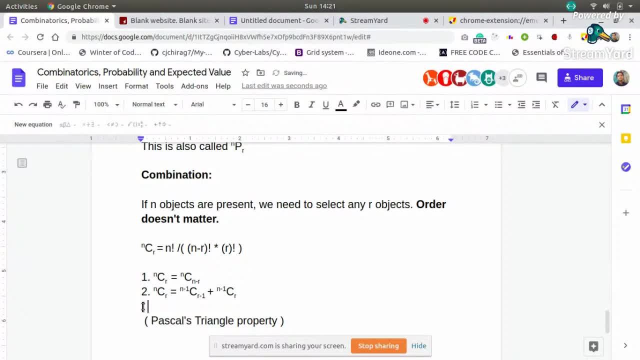 the simple way to like understand this is like: suppose there are n people and you need to select r out of them. let us say there is one person called jack, so any name you can give. let us say there is one person called jack in those n people. 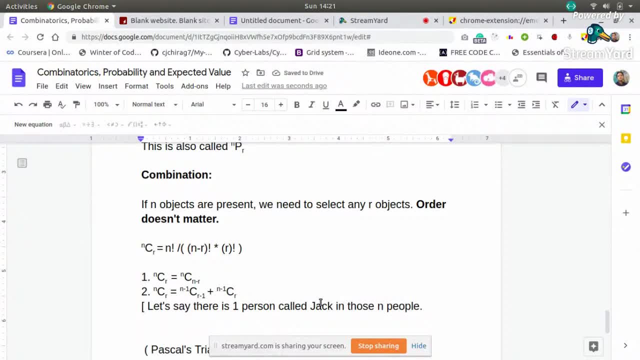 ok, now ok, so there are two cases: either i will select that jack or not. so let us say, in the first case, i select jack. so if i am means i am guaranteed that it is guaranteed that jack will always be selected in my team of r people. 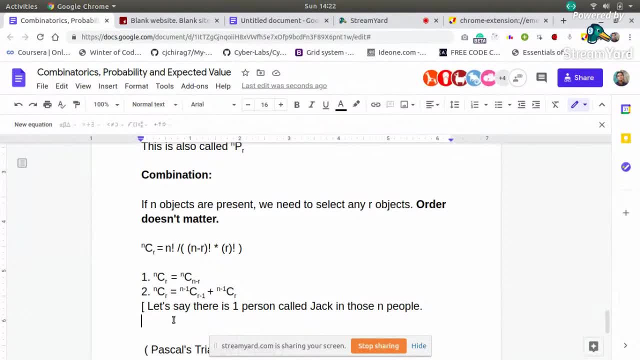 so now jack is already selected. how many people are remaining? there are n minus n minus 1 people, and since jack is already selected, you need to now select only r minus 1 people, because jack is already selected, so you need to just select r minus 1 people. 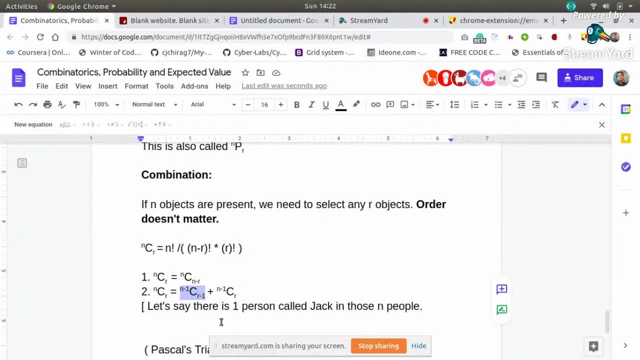 so this is the number of ways to select when jack is already included. so either jack will be there in team of r people or not, ok, so so first case was that jack is present in my r people team, so jack is already present. so i need to select only r minus 1 people. 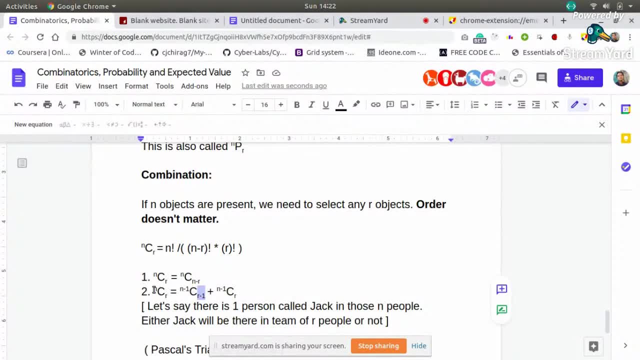 out of how many people. since jack is already selected, so i remove jack. so now there are only n minus 1 people in my class, so i need to select only n minus out of n minus 1 people. i need to select only r minus 1 people. 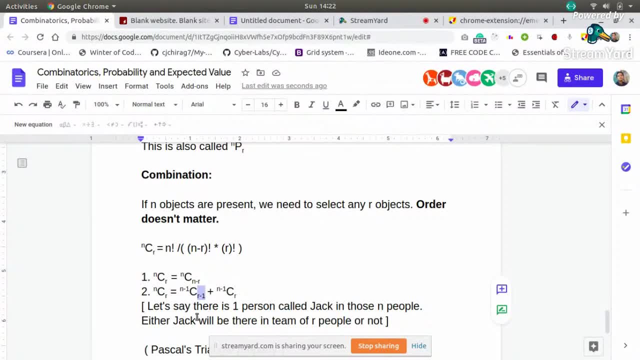 fine, now second case is that Second case is: if Jack is not present, Guarantee hai ki Jack to aayega hi nahi Toh. fir, how many people are there in the class now? N minus 1.. Since I have removed Jack, 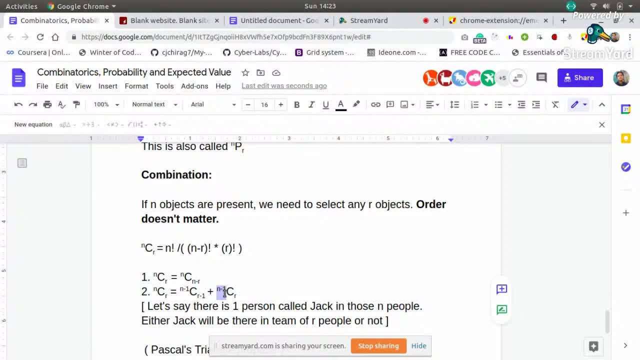 But now, since I need to select our people, So what are the number of ways to select our people? So it is N minus 1 CR. So from there this property is. you can say it is a simple proof, Theek hai. So either one person. 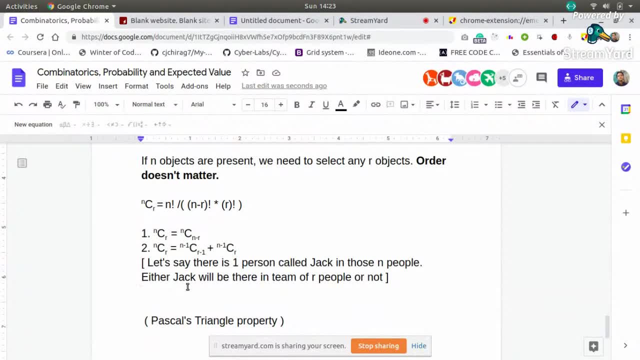 You fix one person. Let us say this person will be there or it will be not there. There are two ways. So here I have written or Means: either this will be there or it will not be there. So I have written a plus between them. 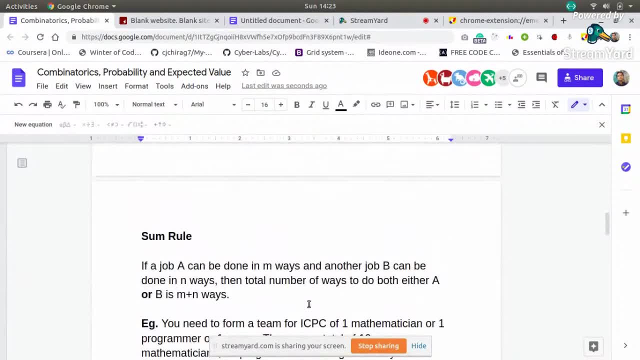 Why? Because some rule says that whenever you need to perform any one of the tasks, Either A or B, Then you do M plus N. In the total number of ways to do any one of them is M plus N. Fine, So if you have any doubt, 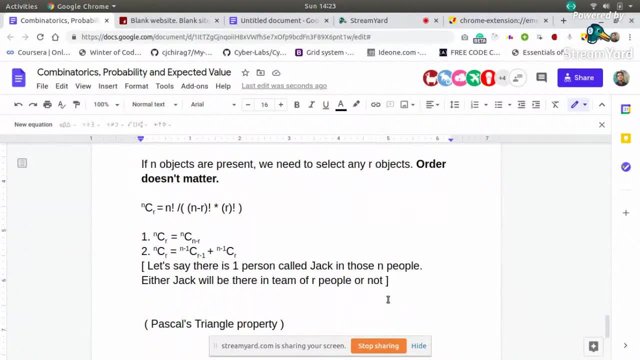 I will tell you now. You can just ask it, So that it will be better for me to clear Theek hai Now. one more important property is Like when you do NCR, So you can also write it as N. 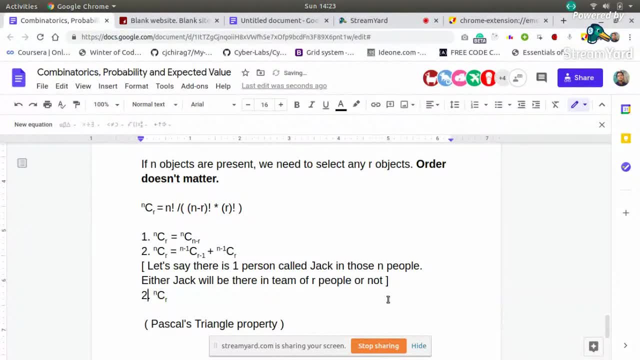 C, R Can also be written as, Or better say, One. Suppose this thing is there, One plus X to the power, One plus X to the power, One plus X to the power N. So this, If you expand this by binomial theorem: 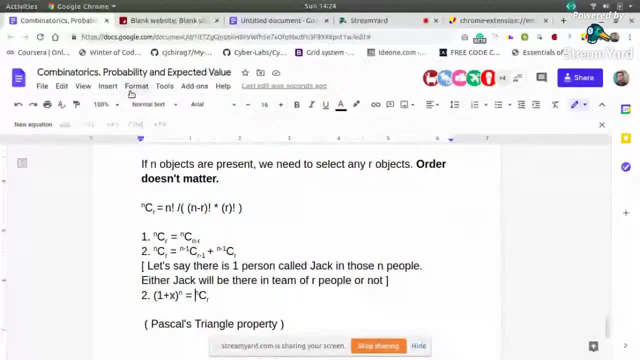 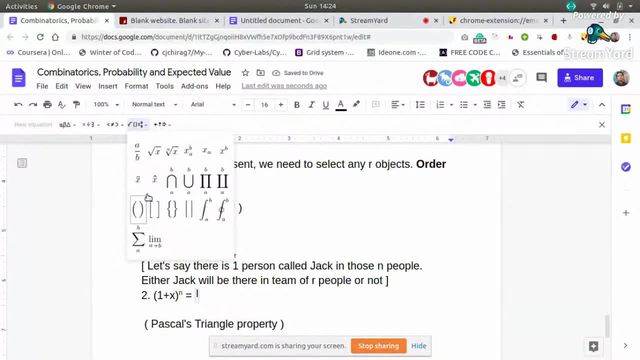 Then you will get summation here. It will be summation, Summation, Summation from R equal to zero to R equal to N, and NCR NCR will be there, or NCR NCR multiplied by X to the power R. 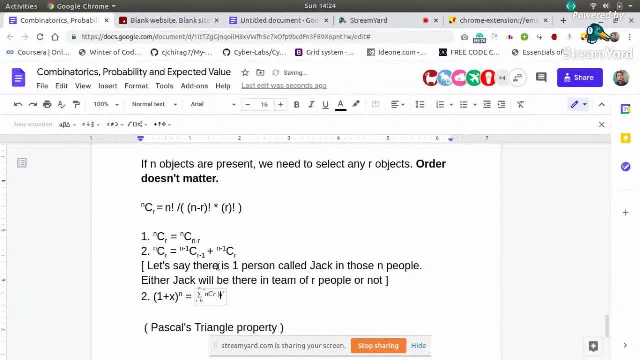 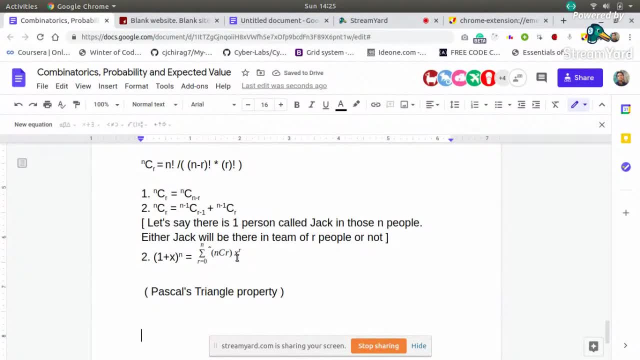 So it is something like this: to NCR X, to the power R, This summation you do. So this is the binomial expansion. So if you Past, the triangle property was the above one. So if you put Put X equal to one in the above equation, 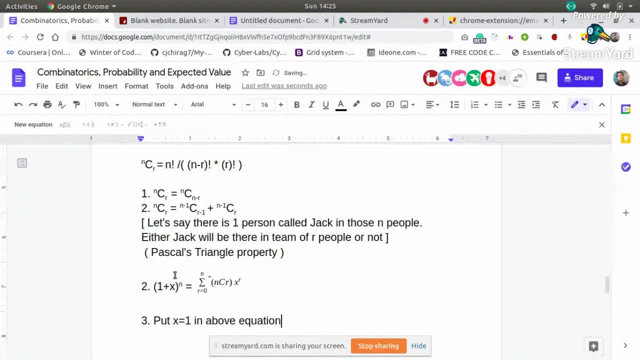 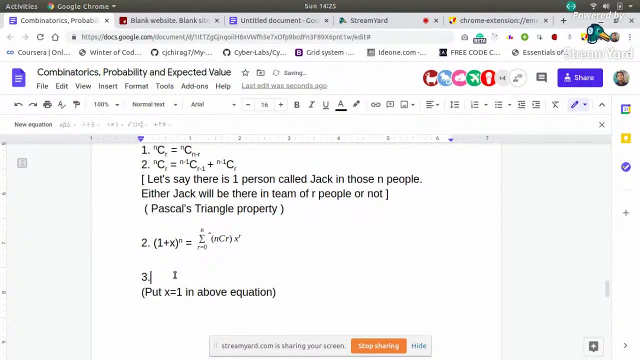 So you what you will get if you put X equal to one in the above equation, you will get two to the power N. So let me write in this way that some in the summation and CR summation, from the R equal to zero to N and CR will be two to the power N. So this is one more. 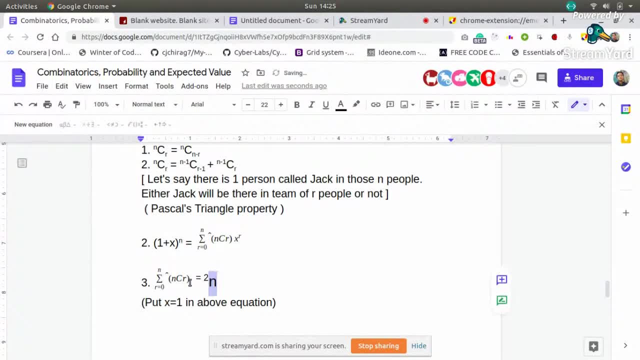 important property. Okay, Okay. Okay, This is not correct. Looks good Because I don't know how to divide this into two parts, but if it is relatively legitimate, be considered as a proof of that. This is 2 to the power n. 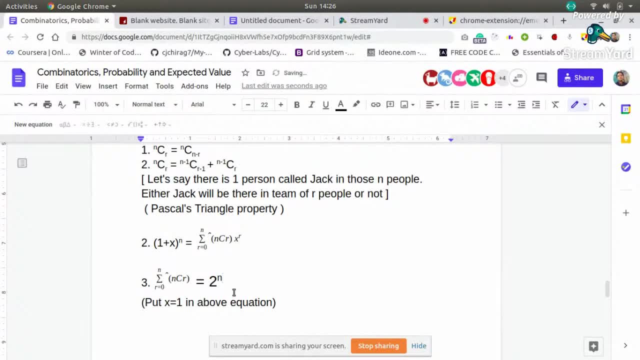 2 to the power n. OK, So after this we have one more thing: nc, if you do 2ncn, so what it should be Means if you write it in the form of summation, you can also write it in this way: 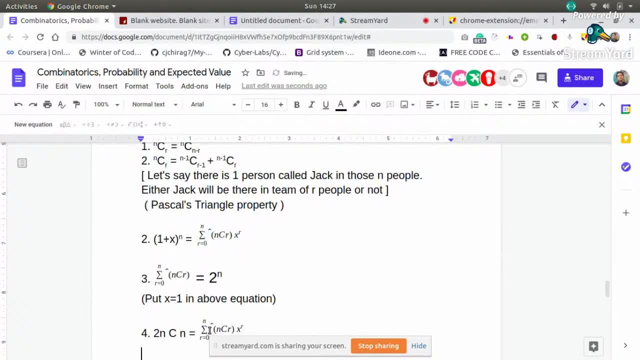 Summation 2ncn can be written as summation: nck whole square. OK, OK, OK, nck whole square, where this nck means this k equal to 0 to n. So can you say how this can be proved? 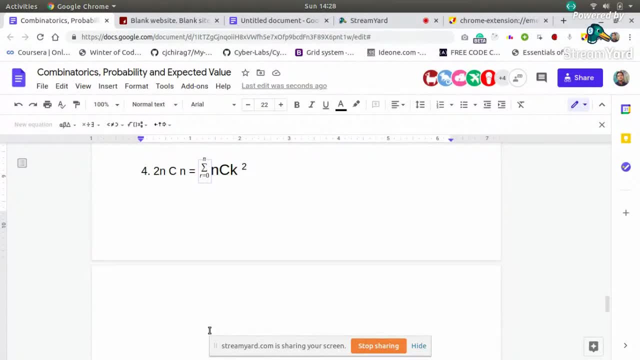 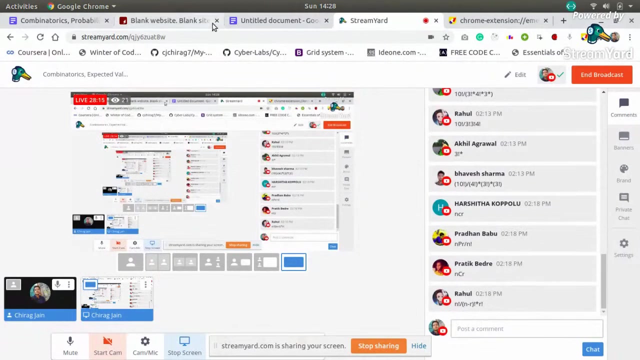 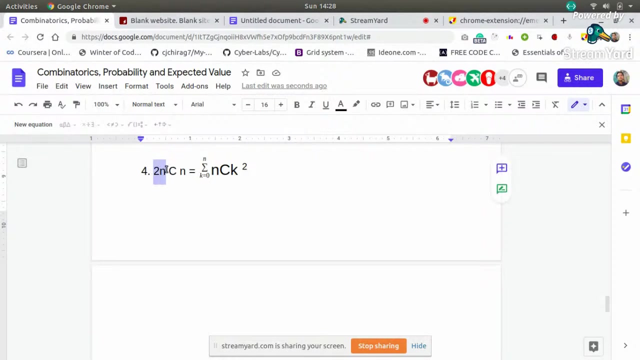 or any intuition for this. Anyone. 2ncn means what: There are 2n people, You need to select n out of them. So, if you think of this in this way, there are 2n people, So you can divide them into 2 groups of n people each. 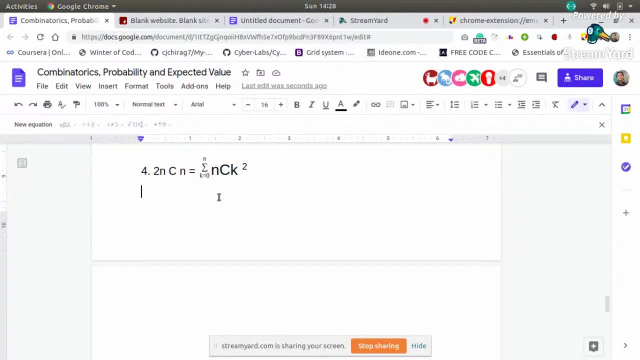 So in each group there are n people. So divide 2n people into 2 groups of n people each. So each group is having now n people Now. So from those n people you need to select, like from one group. 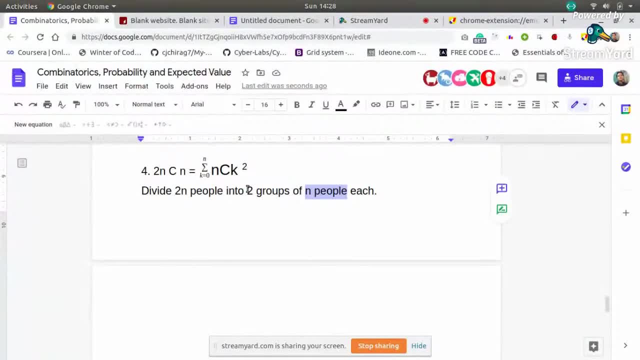 I selected, let us say, k people. So from the second group I need to select n minus k people, Because in total I need to select n people out of both of these groups. So I can write the thing as, and it just can also be written as: 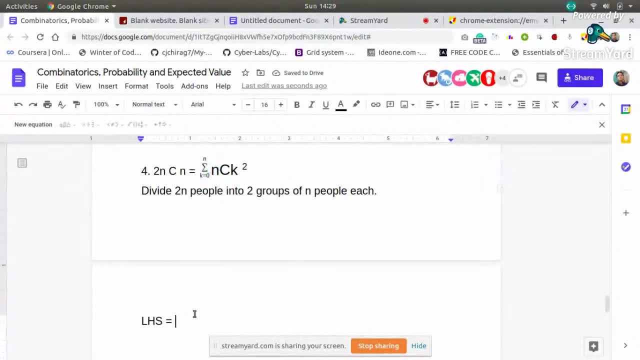 if you do summation from k equal to 0 to n, Summation k equal to 0 to n and nc n minus nc equal to n, So this is nck multiplied by nc n minus k. How does this come? 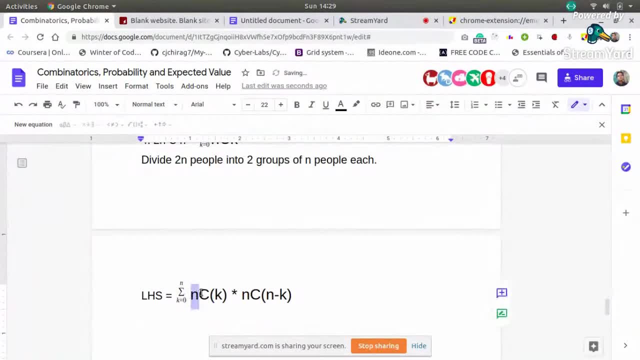 Because I divided these 2n people into 2 groups each of n people. From the first group of n people I select, let us say, any k people. k can vary from 0 to n, So I am bound to select from the second group. 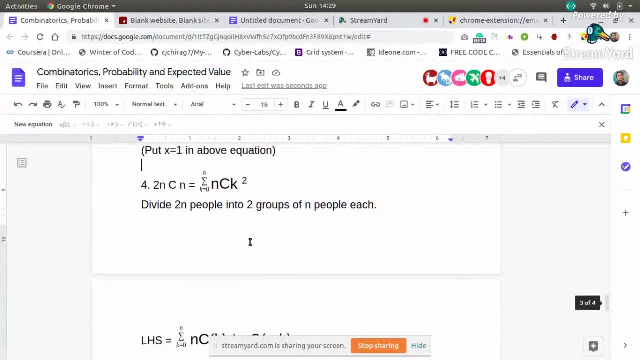 I need to select n minus k people, Because in total I need n people. So this is just like you can from this. if you do this, you know that nc are equal to nc and minus r, So these two things are equal. 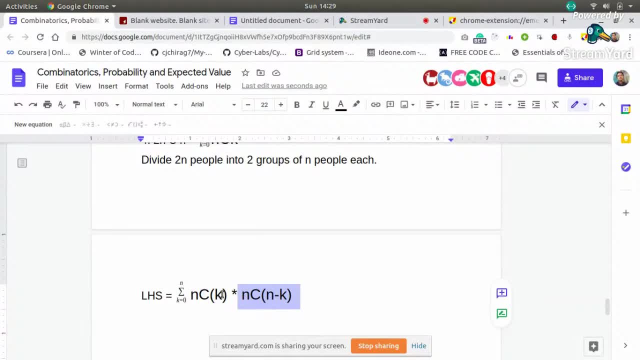 So you can write this also. This also has nck, So it becomes nck whole square. So this is summation k equal to 0 to n- nck whole square. So sometimes these can be used, sometimes indirectly, If you know how to just get an idea. 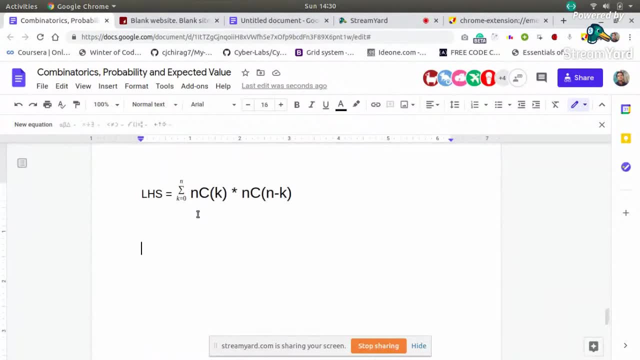 it means, if you know how to prove this thing or something, that it might be useful in solving some of the problems. So I think these are sufficient properties which you might need So like. So the second thing is how to compute ncr mod m- ncr mod m. 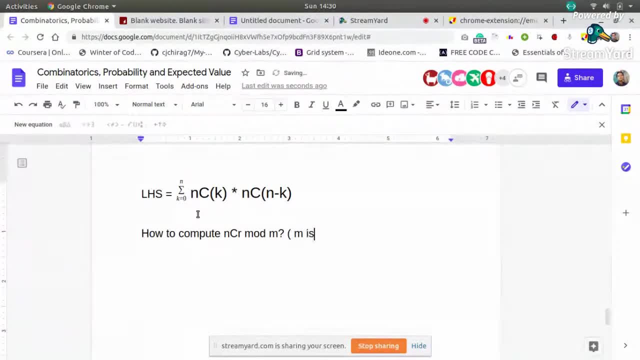 m can be anything Like. m is not necessarily prime. m is not necessarily prime. Then how would you do it? You need to find ncr mod m, But m is not prime here. It may be anything, So how would you compute it? 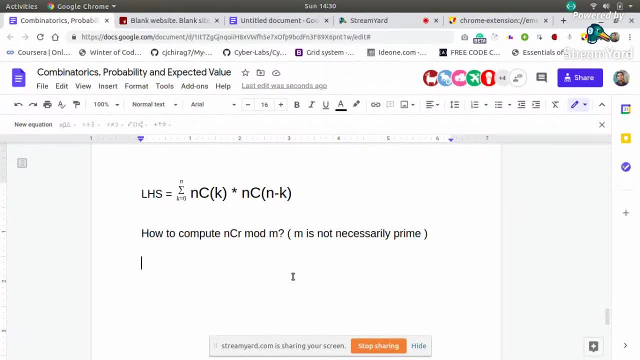 See, you can apply this Pascal's triangle property So like you can use dynamic programming like, say, create a dp array of, let us say 1,000 by 1,000. Or let us say we take a variable max here equal to 1,000 and let us say 1,005, something. 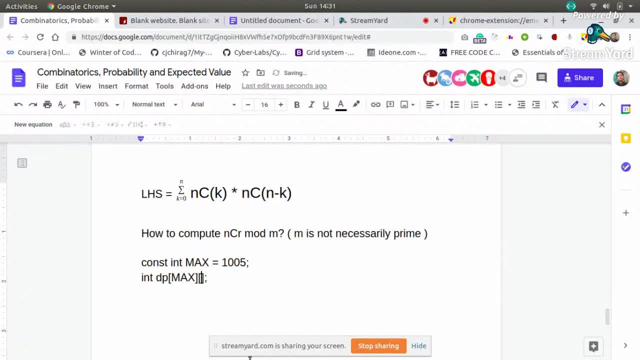 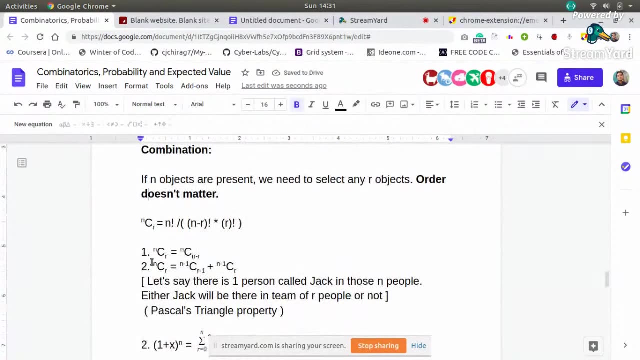 like this: And we create an array of max to max here, Yeah, And you create a recursive function for that, for like ncr, let us say So, int and intr. It is dynamic programming. It means like, basically, we will be using this property of ncr, which 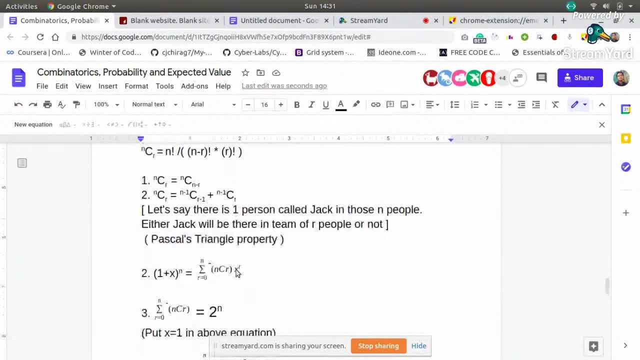 says ncr equals to n minus 1 cr minus 1 plus n minus 1 cr. So you can say that the answer would be simply return: ncr of n minus 1 r plus ncr of n minus 1 r minus 1.. 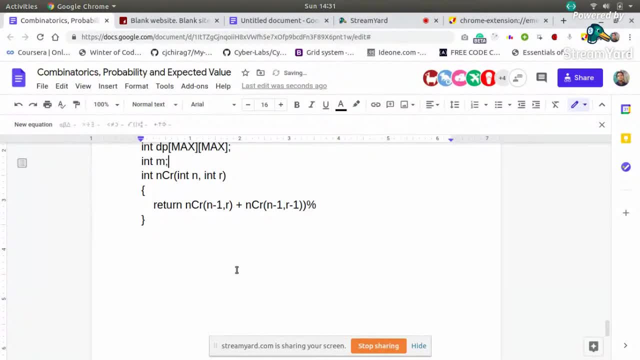 But since you need to find some, let us say int m, some variable is there, m which you need to find mod? So mod m, you should return Fine, Or one thing is like: if you've already computed, you will store this in the dp array, dp of. 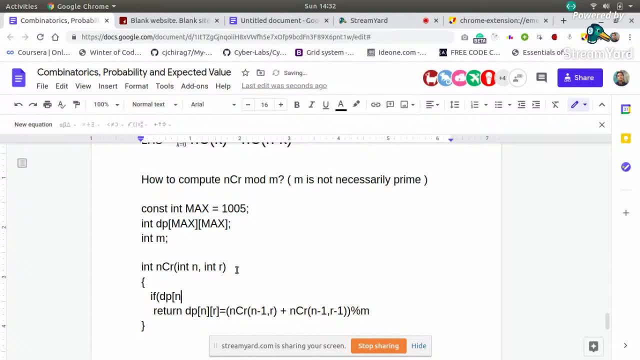 n r equal to this, And if this is already computed. so you are using. dynamic programming means you will compute one value at one time only. So there are total 10 to the power of 3.. This is 10 to the power 3 approximately. 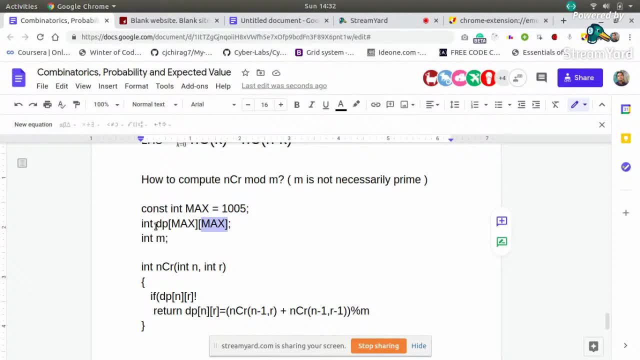 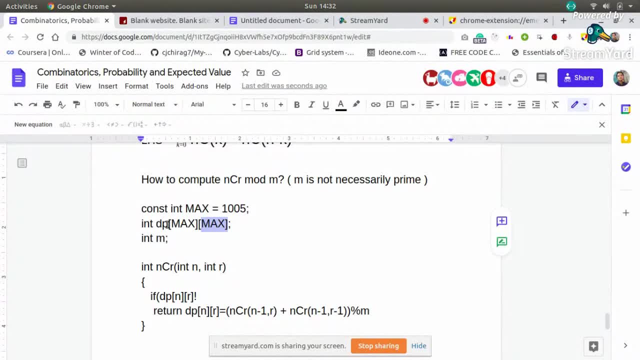 So you can say that each value will be computed once you have time complex. The number of operations which you will perform will be 10 to the power 6, because there are 10 to the power 6 values in the array approximately. So, if it is- and yes, all will be initialized to 1.. 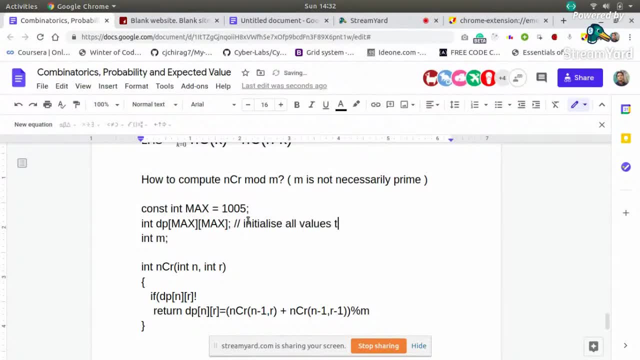 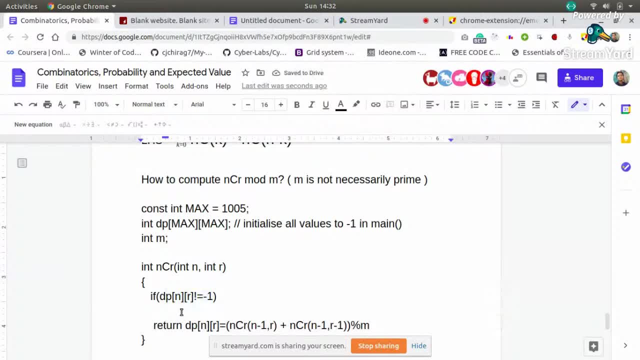 Not equal to minus 1 means that I have already computed it, So I will return directly. Return: dp of nr And base case would be when your r equals. one case would be when r is greater than n, Although this would not be required, but still suppose someone calls your function for ncr. 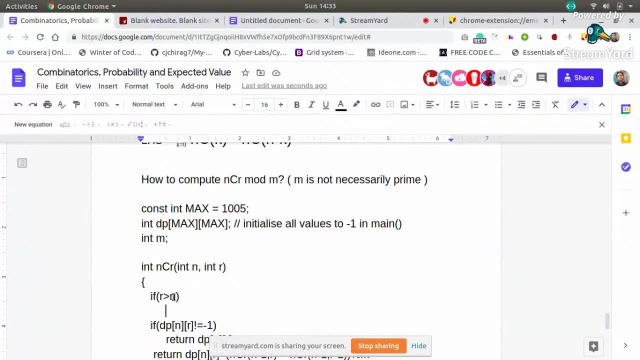 for r greater than n, So you would return 0.. There are no ways to select r people. if there are very less people, The number of people, total people are less and you select. you want to select more people, So it is not possible. 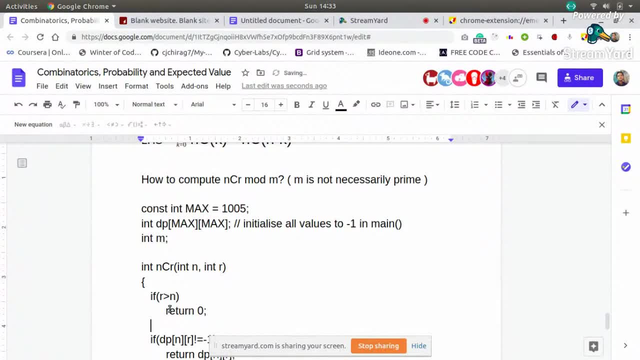 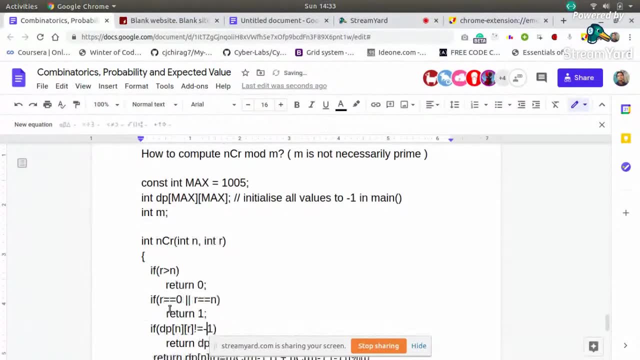 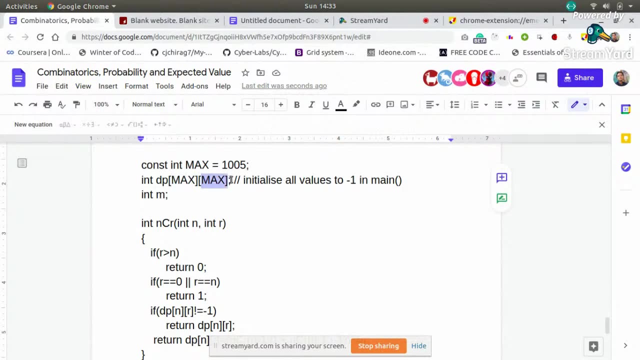 So you return 0. And otherwise what you do is, if r equal to 0 or r equal to n, then return 1.. So this is the base case. So using this you can compute directly. But the thing is, this will work only when- like when n and r both are of the order 10. 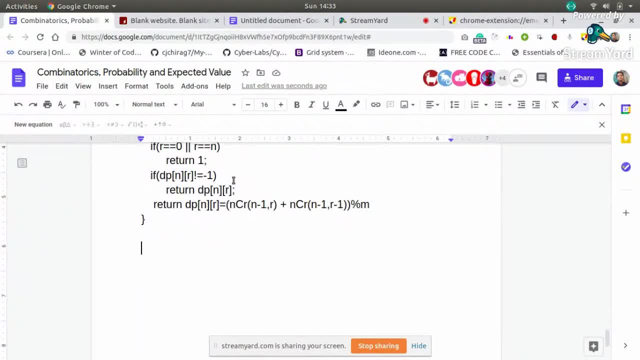 to the power 3.. But if suppose you have n greater than equal to 10, to the power 5,. so this: this would work only when n? r both are less than n. So this would work only when n? r both are less than n. 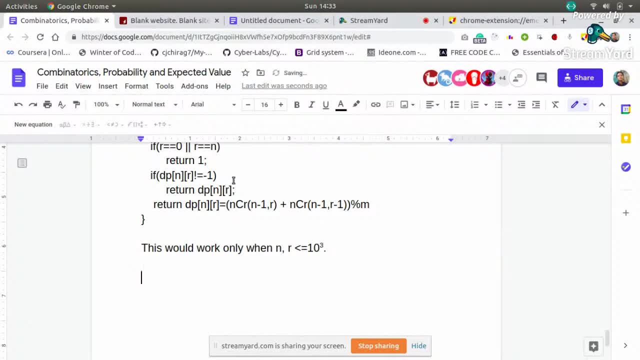 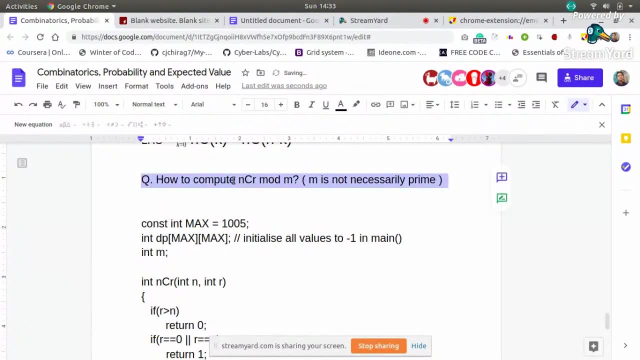 So this would work only when n, r, both are less than n. 0 is n equal to 10 to the power 3.. So this, this method like, will work. This is dynamic programming method, Or we use the Pascal's triangle property. 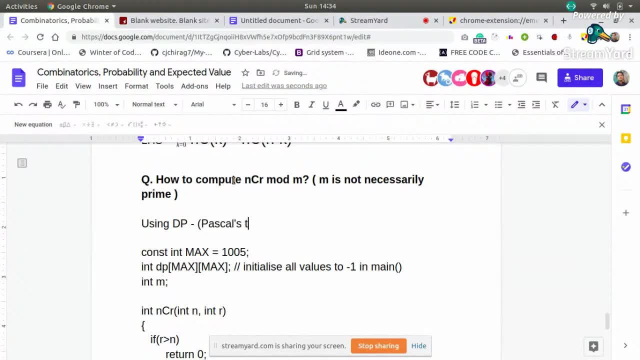 So can anyone tell if, what, what to do if an and r are both very large, like, let us say, both are of the order 10 to the power 5? so how will you compute this ncr mod m? and let us say, for simplicity, now m is prime. okay, now let us say m is prime. 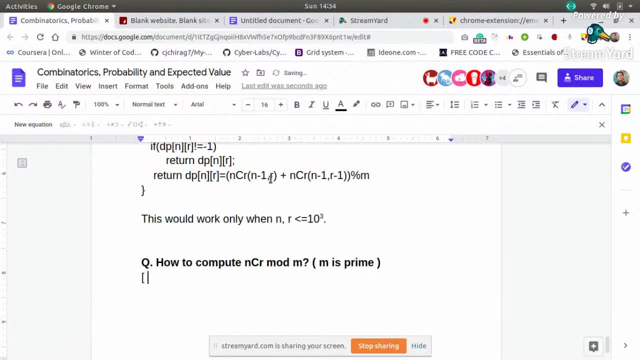 let us say n and r are both. now. let us say 10 to the power 5 or 6, you can say for simplicity, let us say for now, 10 to the power 5. so any idea how to compute now? you cannot use this method because you need to create an array. 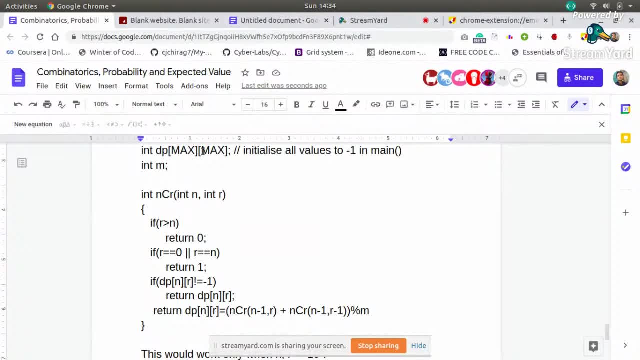 of 10 to the power 5, multiplied by 10 to the power 5. so 10 to the power 10. so such a big array you cannot create global array. also, you can create often if you want to create an integer array, so you can create of maximum size of 10 to the power 6 or 10 to the power 7 values. but if, if n and r, 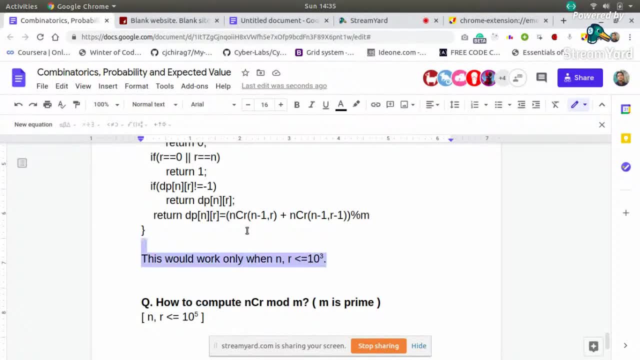 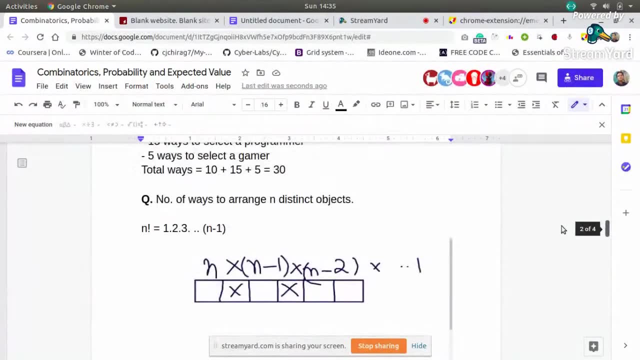 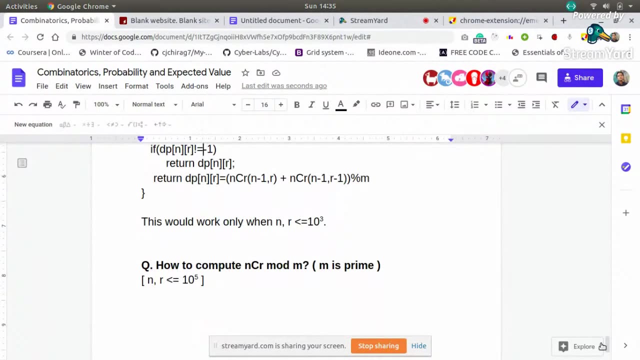 are both very large. so here you required a very large array for above method. so this will not work. okay, so any other idea how to compute? try to answer. if you know it, you need to find ncr, mod m, where m is prime number, permits you can use permits theorem. so directly means you use this above formula for that ncr. 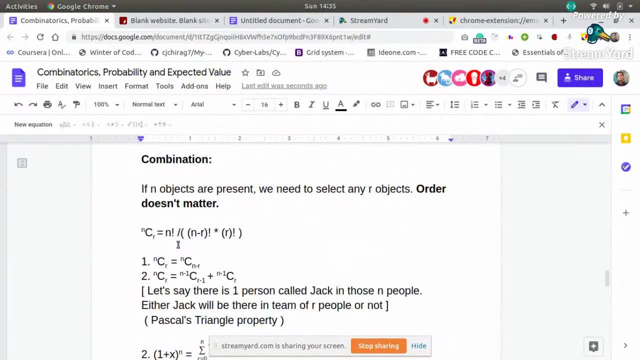 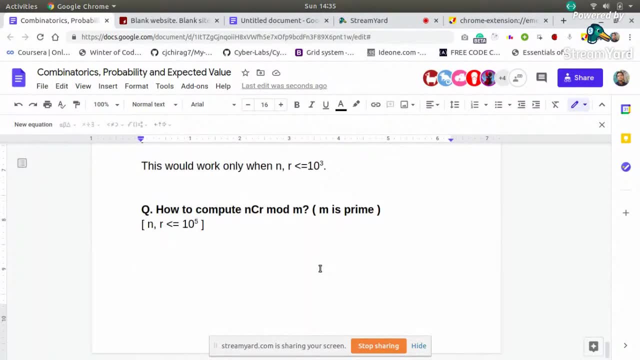 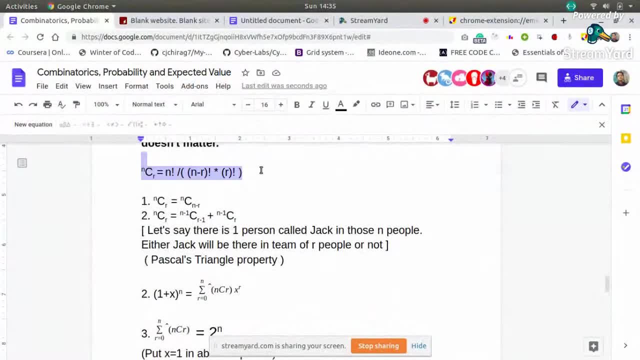 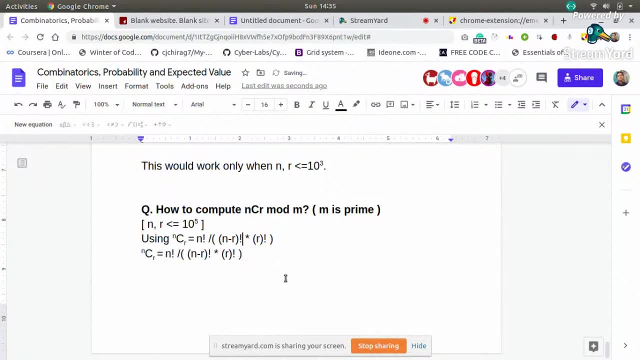 using this definition or, directly, this formula, we can compute it. so using this. so what will be ncr mod m? so ncr mod m will be n factorial mod m. fine, but these, the remaining two things, are in division. so what you need to do is you need to find the inverses of both. so, like you say, if you have the inverse of both of them, 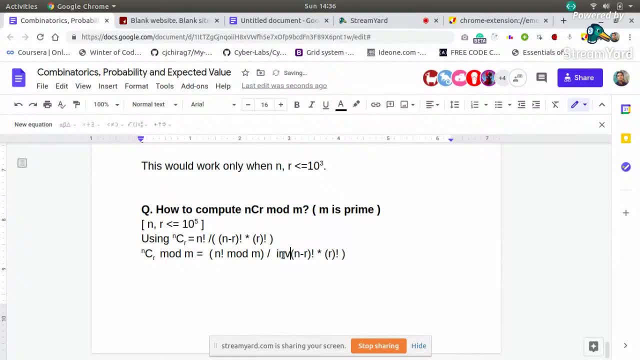 so if you do something like inverse of, let us say, inverse of n minus one, n minus r factorial multiplied by the multiplied by the inverse of n minus r factorial multiplied by inverse of r factorial, so something like this, so you need to find the inverse of this thing and inverse modular inverse. 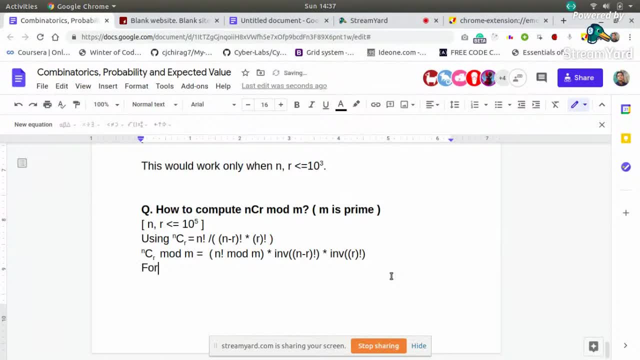 of this thing. since m is prime for finding inverse, you use theğini for finding inverse. we can use permits theorem, so пример theorem says calling customer premium getting cash permits theorem. so permits theorem, khaiti permits theorem says that, uh, if you have quantity of n plus part n, prime sampled masculine 그거 say envelope or greater than n, is n into upper. 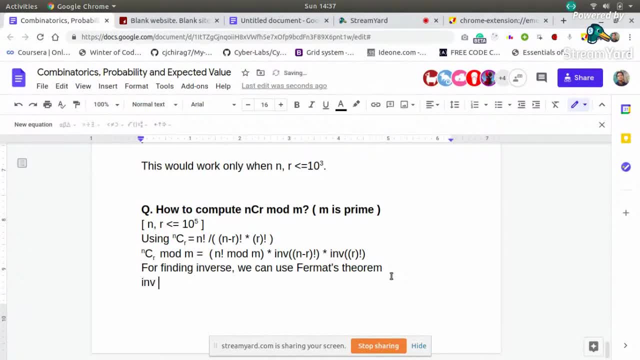 if you need to find an inverse, so inverse. this will be the value of champion in inverse. so parabolas are life: norma of n mod m is nothing but n to the power m by 2 m minus 2 mod m. so this thing is in power. so using this, just, uh, for inverse of this, just we need to find this thing. 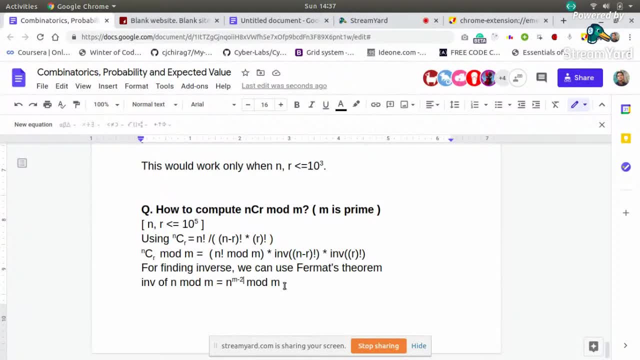 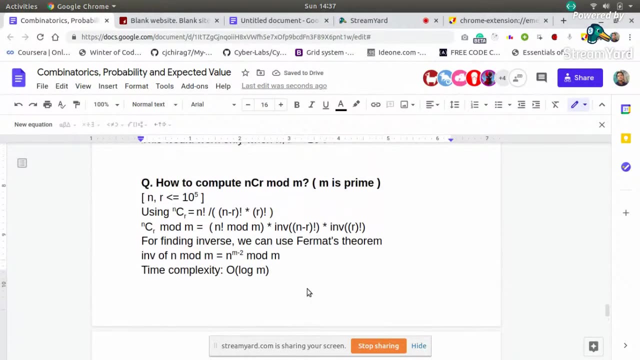 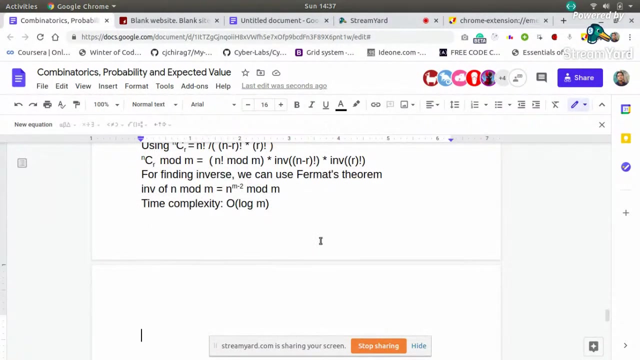 n to the power m minus 2, where m is prime. so this thing can be done in log of n, log of m. so time complexity would be log of m. so this is one more method. but suppose now this thing will also work when, like when your uh, let us say, n and r values are up to 10 to the power 6, or something like that. 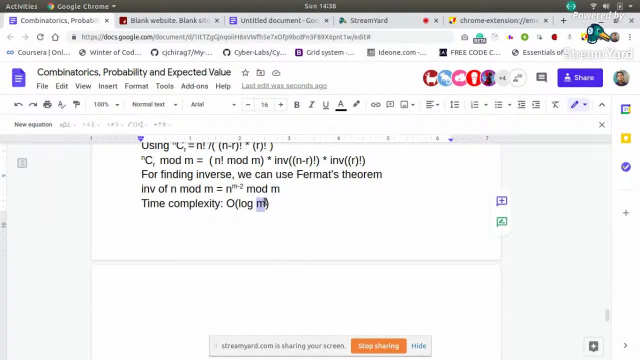 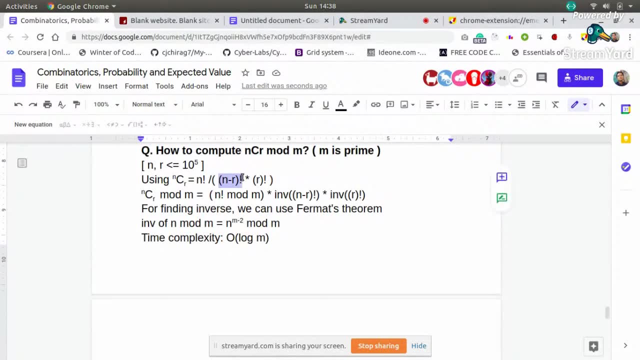 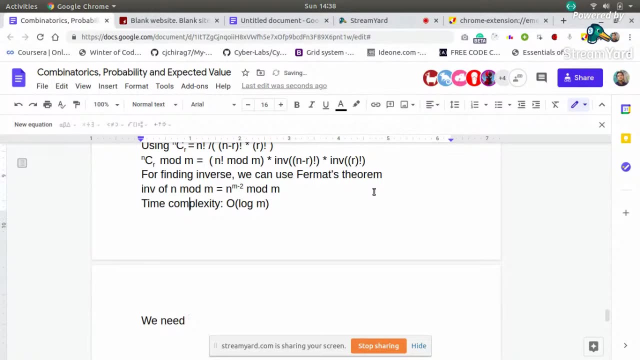 sorry. and when your m is uh, you can say: since it uh worked for this, we need to compute the factorial for this, we need to compute the factorial uh modulus also. so you can say: uh, we need, we need to pre-compute, if i am assuming that you have already pre-computed. 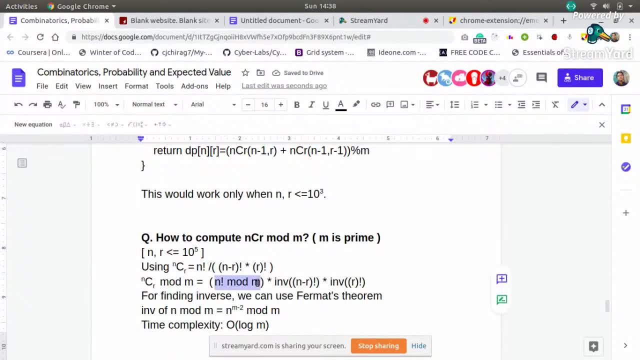 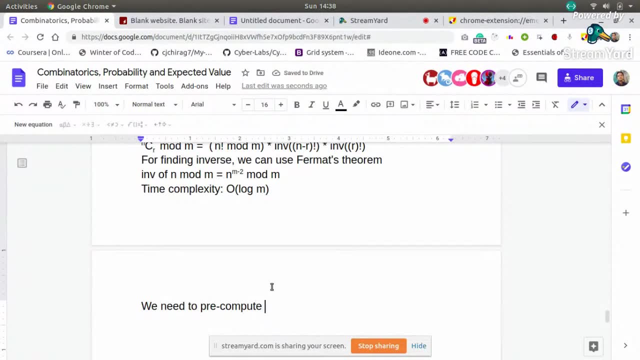 all the fact, uh modulus of the factorial, so n factorial mod m is already compute, pre-computed in one array, so we need to for this method we need to pre-compute uh module, uh modulo of like modulus of factorials, of all uh numbers, how much? let us say up to 10 to the power m. 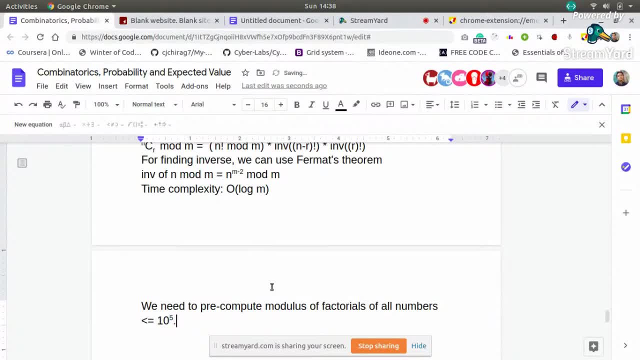 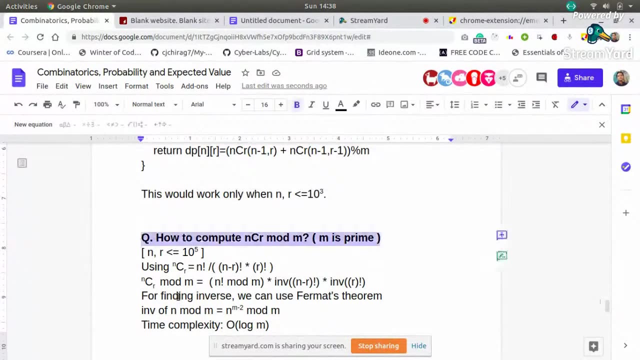 so. so this thing will work only in this case. but suppose you, uh, suppose n and m are very large. let us say n is uh, n and m are 10 to the power of the order, 10 to the power 12, 10 to the power 16, something like this. so again, my question is how to compute ncr mod m. 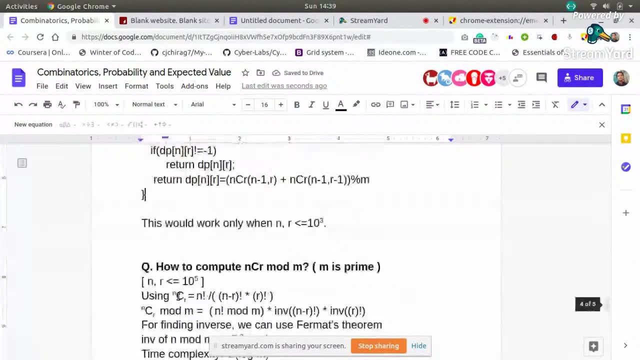 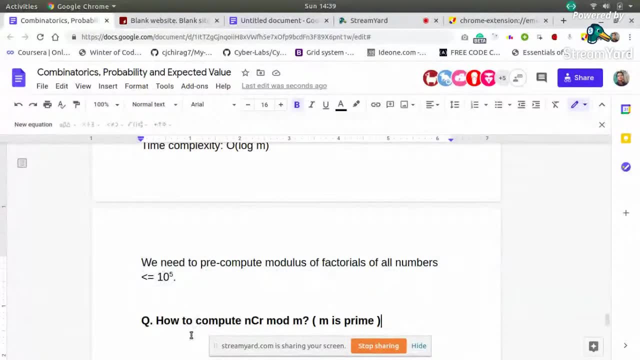 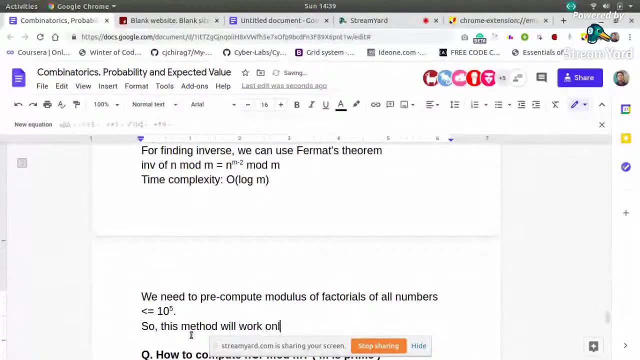 m is prime. but uh, but you, since for pre-computing you need to, you need to create an array of of the size n, at least so. but now let us say you can say that, uh, so this method will work only when your n and m are approximately of the order 10 to the power 6, or something like this. 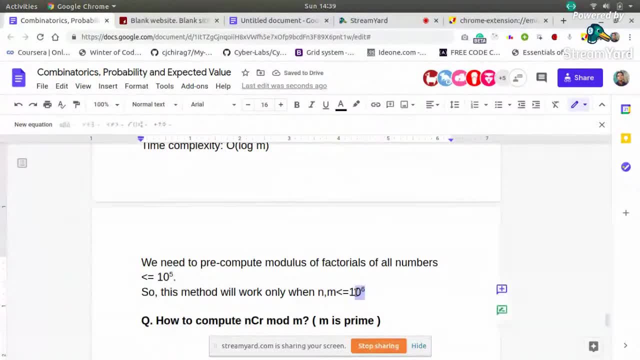 okay, this is approximately. it may work for 10 to the power 7. also, i'm not sure, but uh, of the order this, but suppose now uh, and then m and m are very large, let us say of the order 10 to the power 12 or something like this. then then any idea, anyone knows how to compute. 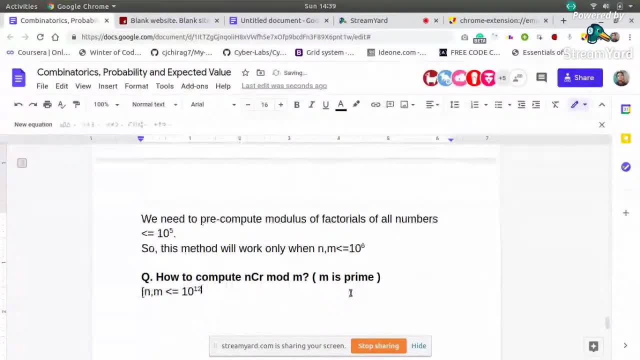 this anyone. you need to find ncr modulo m, but now n and m are very large. uh, okay, m can be very small. m, uh, like m can be small. you can say, of the order 10 to the power five, let us say sorry, uh, ncr here, n and r- i am talking about n and r- of the order 10 to the power 12, but m is very less. 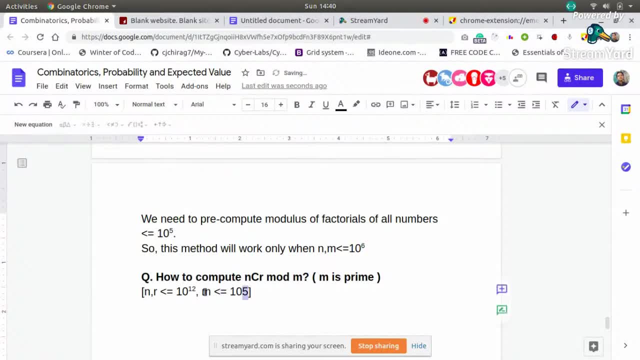 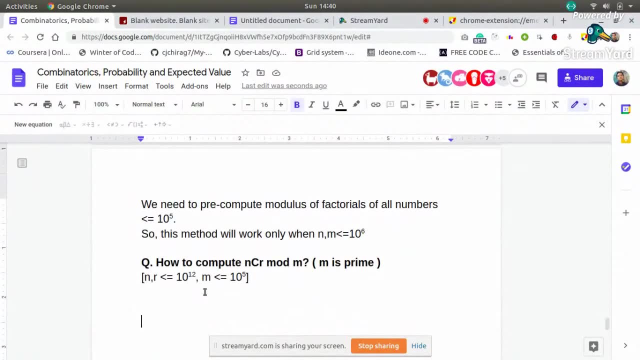 m is not very less, but of the order 10 to the power 5, let us say Any idea for this. So for such cases there is one theorem which we will use that is also called Lucas theorem. So by Lucas theorem you can say that whenever you need to find 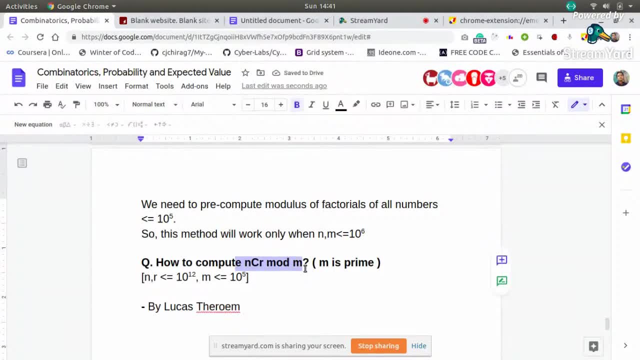 this ncr mod m, and let us say m is prime. So in that case, what you need to do is you need to find the ncr mod m. So in that case, what you need to do is you need to find the ncr mod m. 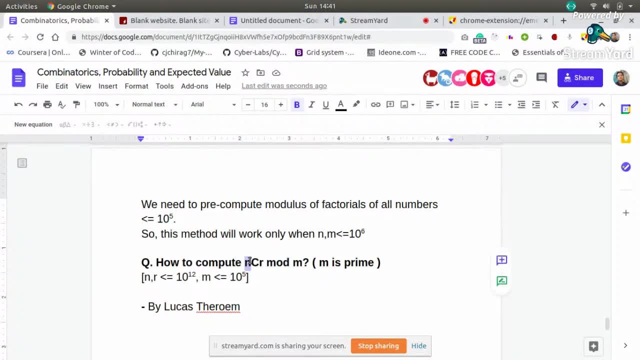 So in that case what you need to do is you need to find the ncr mod m, something like some number of digits will be there. So let us say n k minus. let me write in equation form, So it will be something like this: So n k minus 1, then there will 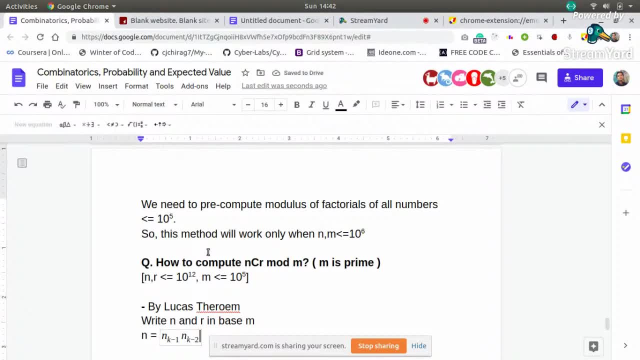 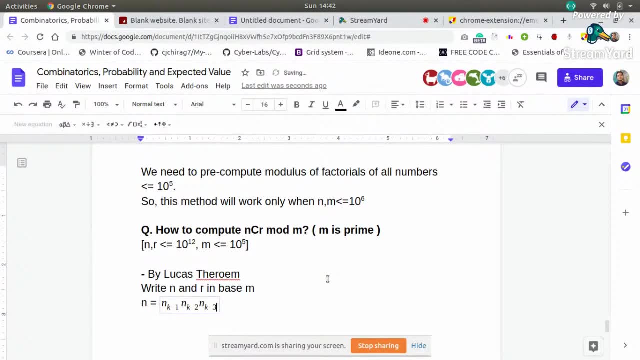 be n k minus 2, then there will be n? k minus 3 and so on. So there will be many digits like this And up to you can say there will be up to n? 0. So it will be something like: 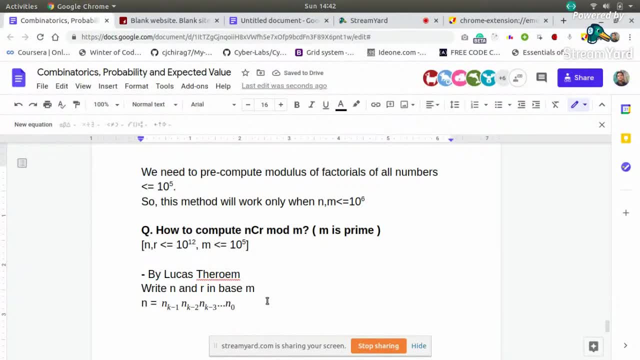 this. There will be many digits in that modulo base m And if I found, if I found this in this, is in base m. So how to convert in any base? Just find the first find, like what we do, So converting, for getting the binary of any number, what you do, divide by 2, store the remainder. 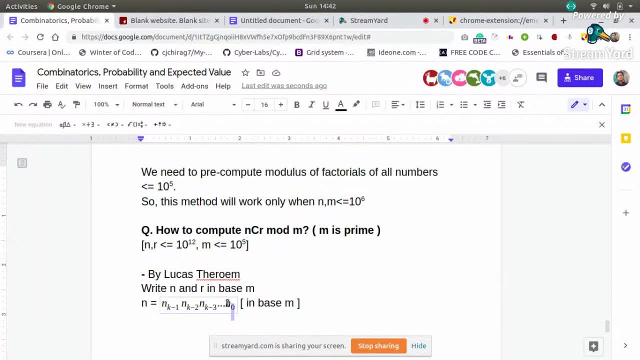 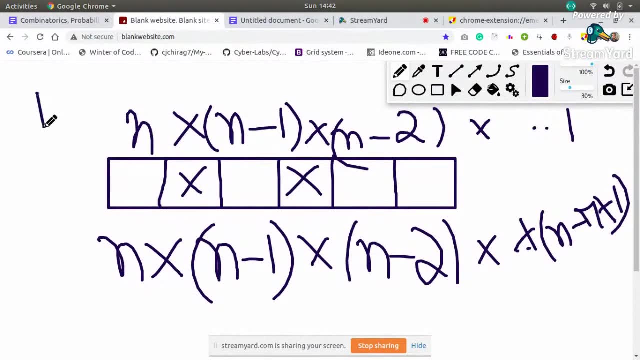 means just write the remainder And again n divided by 2, whatever the question you got for you recursively call that function means you recursively keep on doing this, Like if you know for binary, if you want to find the binary of, let us say, 9, what you do, 9, let me. 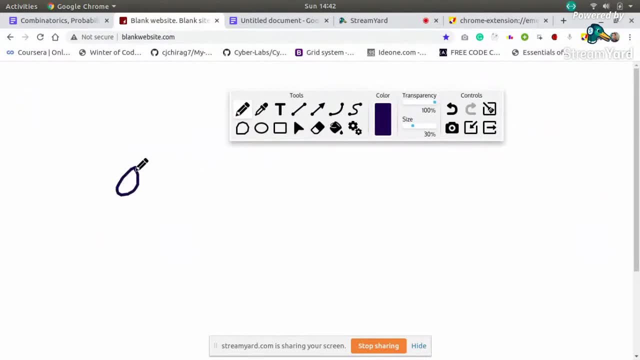 erase this all. So, for finding the binary of 9, what you do: 9 divide, because binary means base 2.. So you divide 9 by 2: what remainder you got, you got remainder 1.. So I write the remainder. 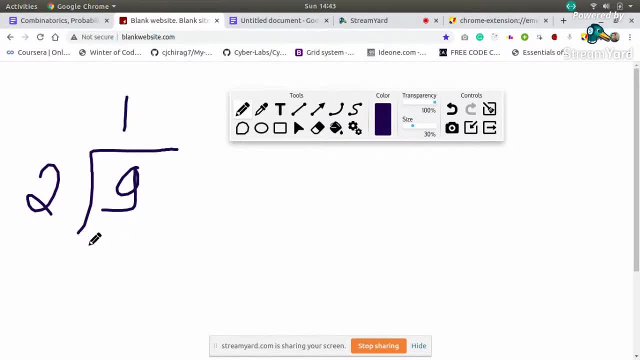 So I will do the remainder. I will add the remainder somewhere. Now, 2 divided by 9 will give me what question it will give. So it will give me remainder. will be 1 here and it will give me question 4.. So I will divide. I will now divide 4.. So 4 divided by 2 gives: 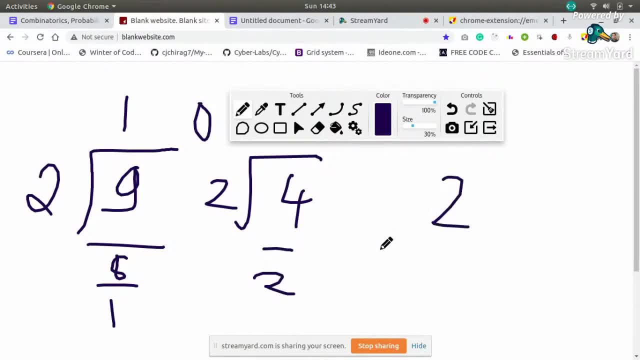 me remainder 0. So I will write remainder, let us say here, and 2 divided by 4.. The question is 2.. So I will repeat the process for 2.. For 2, you do the same thing: you get the remainder. 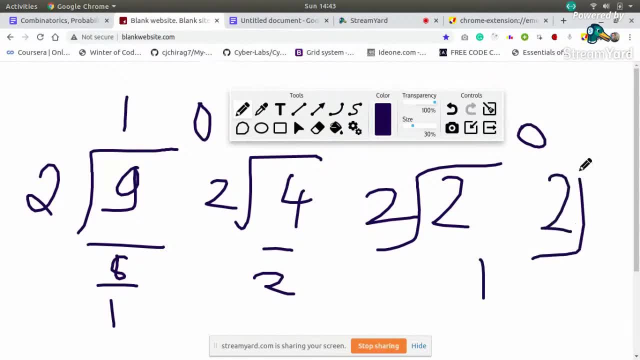 is 0.. Okay, And what you questioned, you get, you get question test 1.. So now you do the same thing for 1.. you will, finally, you will get: remainder is uh, remainder is one, and you will stop the process here because this question tells: is less than this number, okay, which? which is the base of the 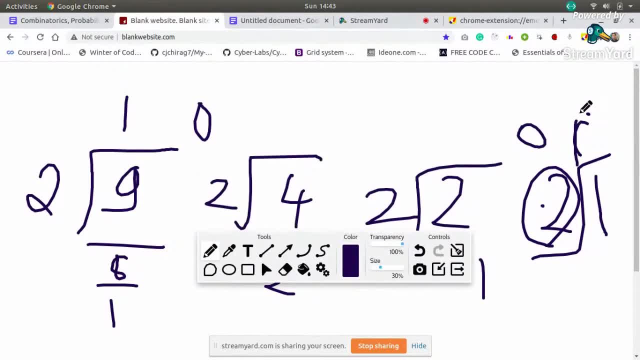 number. so, finally, you reverse the order of whatever, whatever remainders you got, so it will be one zero, zero one. i am reading from right to left: you reverse the order of remainders, so you get this thing, so you get one zero, zero. so, similarly, for any base you can do, first find the remainder. 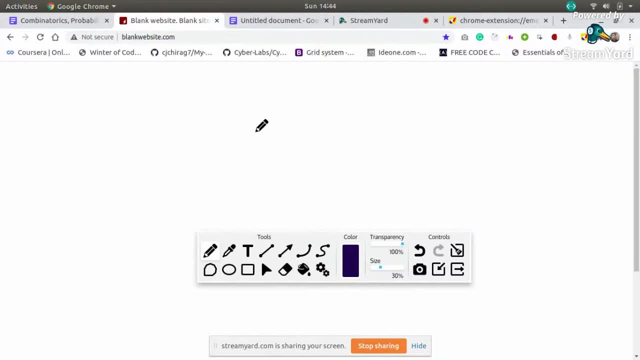 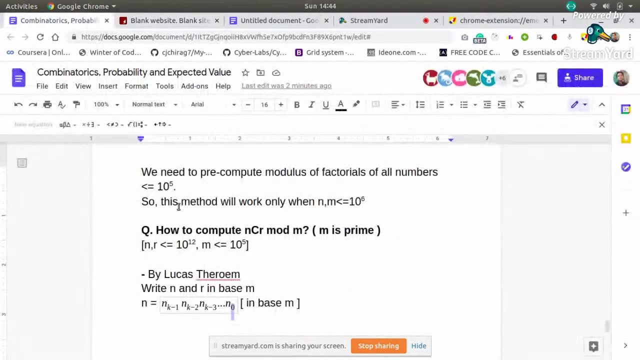 then whatever remainder you got you- uh means uh, whatever the number was. you divide that by that number- the question you got- do you repeat the same process for the question and store the remainders like. this means these remainders will be the digits in the base m when you write the. 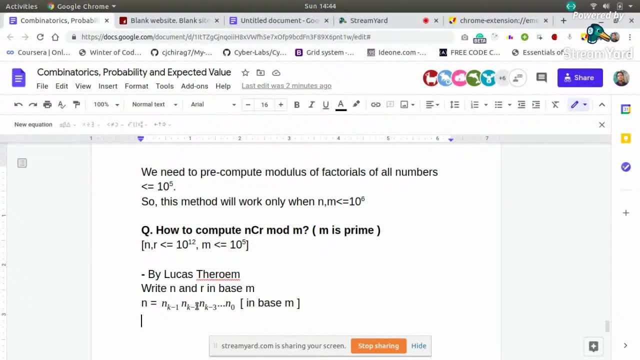 number in base m. fine. so if you do this thing for n, similarly you do this for r also. you write r also in base m. so it will be something like r will be rk minus 1 rk minus 2 rk minus 2 rk minus 1. 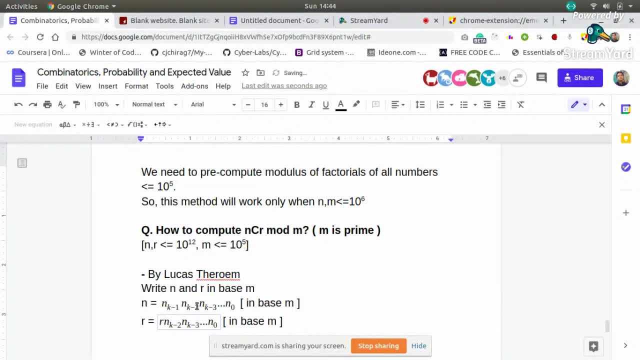 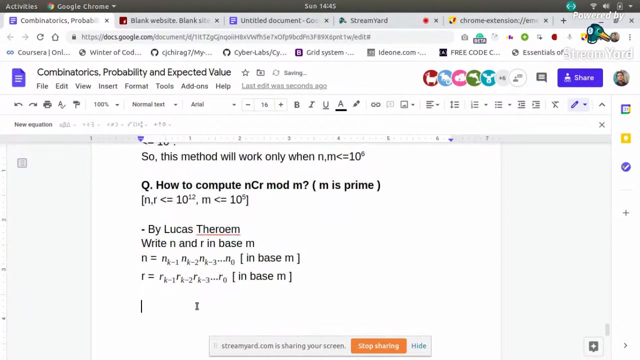 rk minus 2, rk minus 3 and so on. okay, up to r zero. so, uh, now. now the thing is by lucas theorem. it says that now, ncr modulo p, you want to calculate, so it will be nothing, but, uh, you just do ncr. uh, you need to find ncr mod p. so ncr mod p, uh mod m. 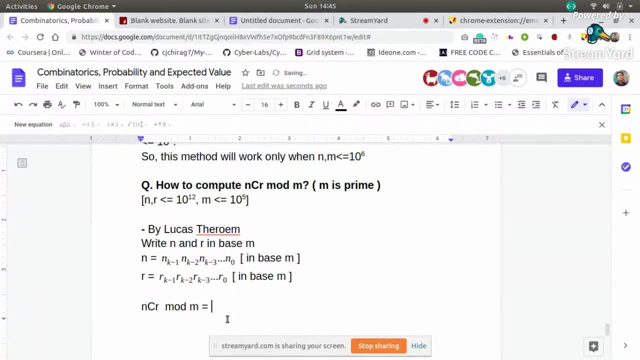 let us say m is our prime number, so mod m will be: just you go, you go, digit by digit. first there's digit, this digit multiplied by means uh, ncr, you do ncr of these two digits and you multiply it by the ncr of these two digits, and so on. like it will be: uh, i should say n k minus one. 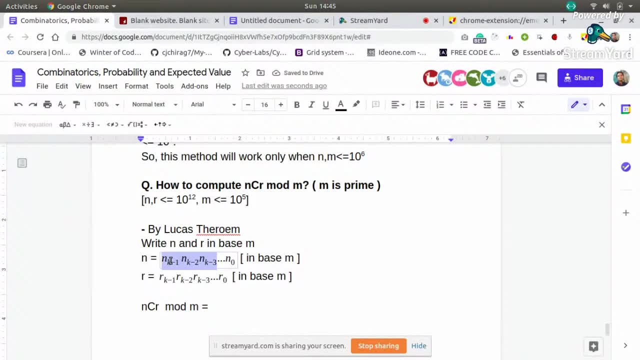 let me copy this: nk minus one, nk minus one, c, rk minus one. so i just took the ncr of these two digits. now for the second digit, i'm doing the same thing. you take the ncr of these two digits, soacula 1, so you multiply them and do, and cnc, k-2, crk-2. 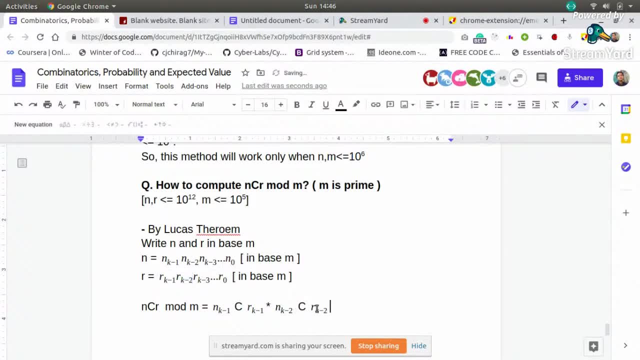 and so on. so this will give you uh, the modulo means. at every step, whenever you multiply, you take the modulo m, modulo m and similarly, you do keep on doing this. so, similarly for nk-3, you guys do this exactly 120 ort of r2 is Goo and this modulo history that was here is equal to is equal. 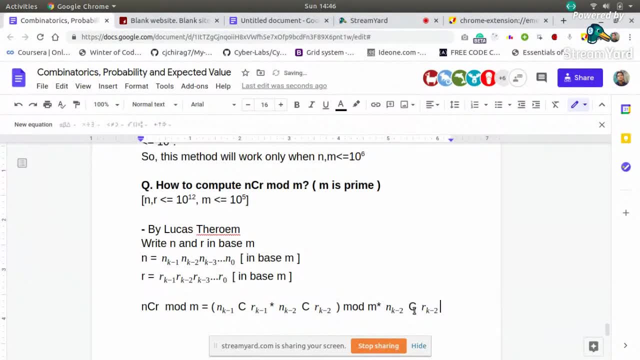 to the resolution of the modulo hypothesis. so essentially, if y and y is equal to y and k minus three, and so on, take it for n? k minus three, c, r, k minus three. these are nothing but digits in whenever you write the number in base p. okay, now i will write the code for this. so this: 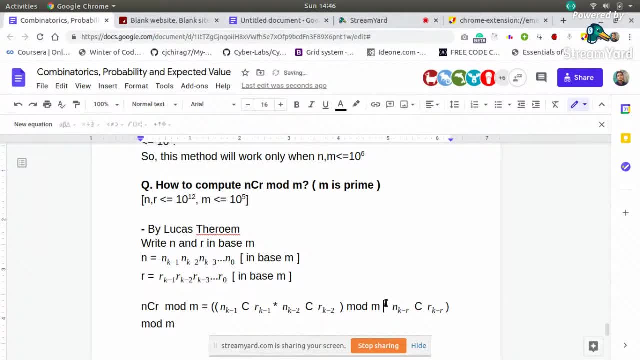 was the lucas theorem: modem, modem. you need to do it every step. so, and dot, dot, dot, i'm keeping. so you similarly do this up to n, zero, c, zero, up to the last digit. so this will work. when you are, let us say, m is uh, even when m is less than equal to 10, to the power 6, and when n and r are of the 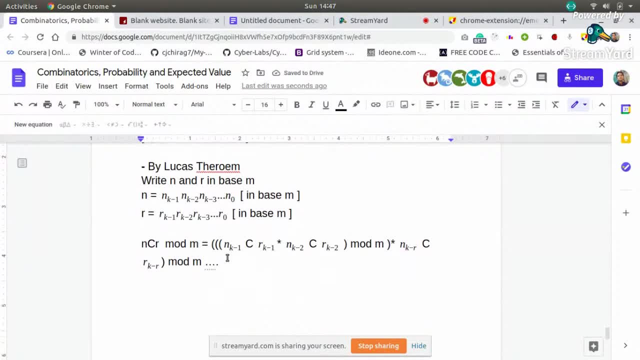 order, even 10 to the power 18 also, it would work. so the code is very easy to write like. if you know how to compute the uh, any number in base p, what you do remainder with p will be one digit and divide by p for the recursive function. so like it will be, i'm writing int ncr. you take n and r as. 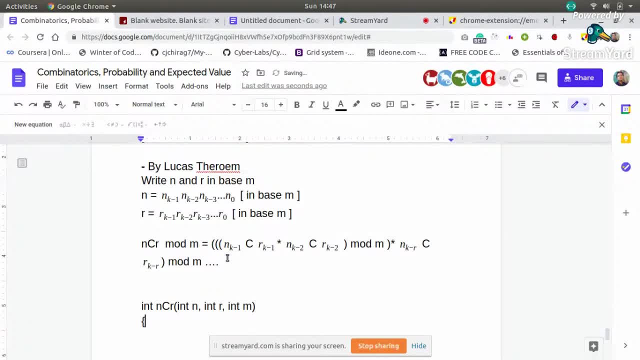 argument and you take m as your prime number, which you want to uh means, which you want to calculate mod with just one base case would be like: if r equal to zero, then directly return. if r equal to zero, you return directly. one now, uh, one thing is like when you calculate digits, when you calculate ncr. 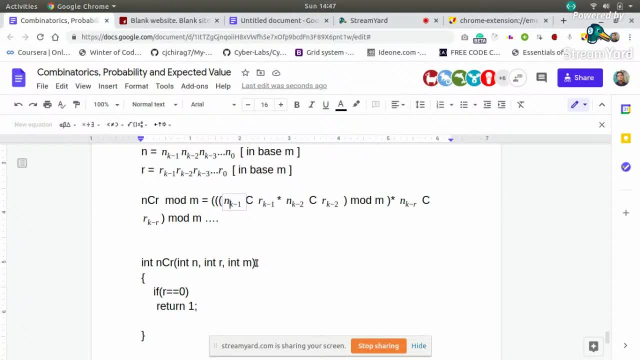 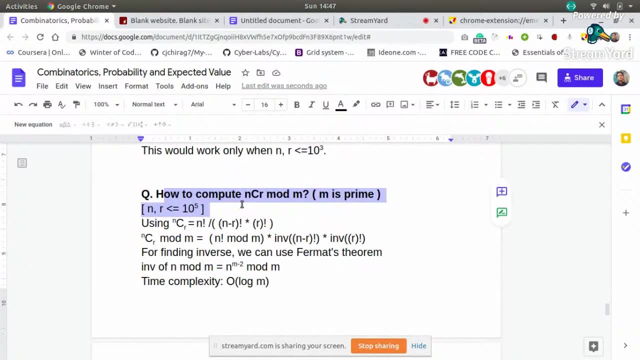 of digits, since m is very small, of the order 10 to the power 5. so for this, for ncr of these digits, you can choose any, any method previously discussed, so you can use this method for computing the ncr of these digits. so don't worry about the digits thing, but you will be able to calculate the ncr. 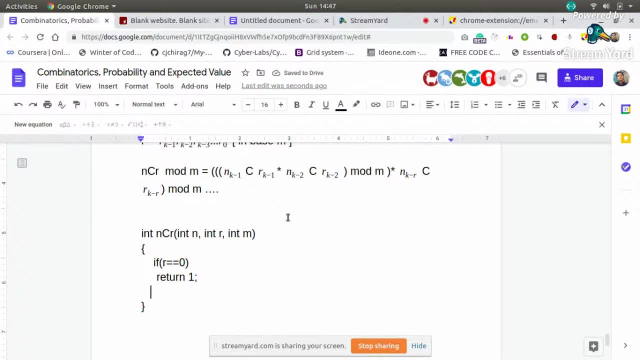 of the other digits and you will be able to calculate the ncr of the other digits. so you of the whole number using this technique. So let us say that one digit would be, I'd say digit of n would be n mod r, n mod m. 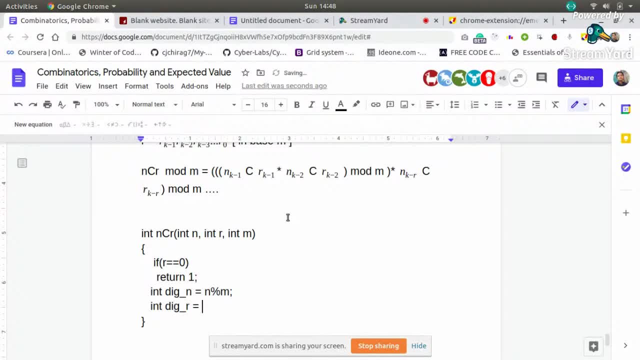 and one digit of this r would be r mod m. fine, Now what I need to do is I need to just return the answer for means ncr of these two digits. So I suppose I have one more ncr function, ncr of digits, or you can take ncr of digits. 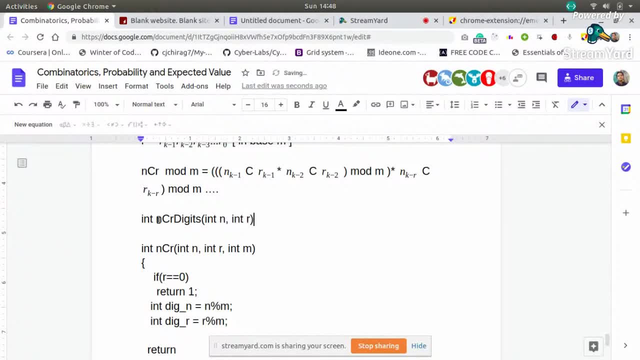 So it. let me call it int n, something it can be. I will not write the whole function. I will write key. use any above method, like any method for ncr of digits, as discussed above, It means Pascal's triangle, or you can use the inverse method. 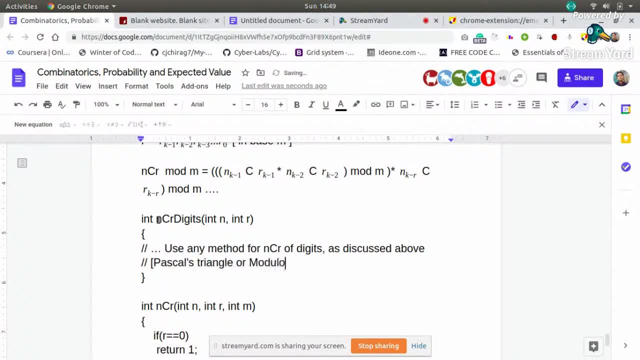 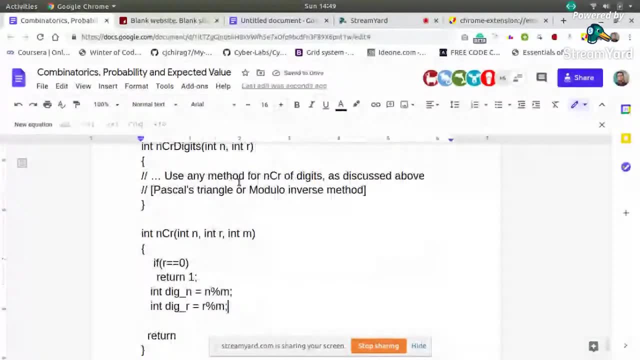 Pascal's triangle or Modulo inverse method. So we have discussed both of these methods above, So you can use any one of them To compute for because the digits are very small, When you write any number in base p, the digits will always be less than equal to p. 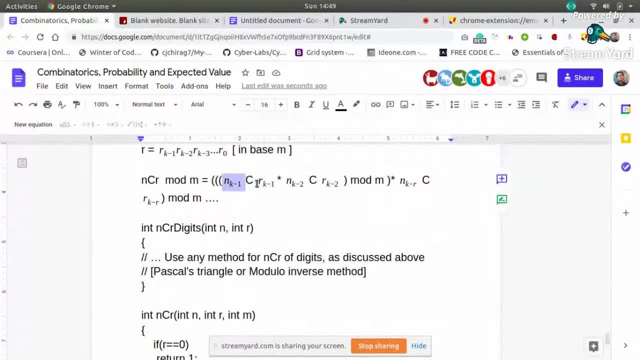 So we had the b in base m through all the digits n, m and k minus one, r, k minus these all will be always less than this, less than this m, since you, when you write in binary, always all the digits are less than 2, 0 or 1. similarly it is: 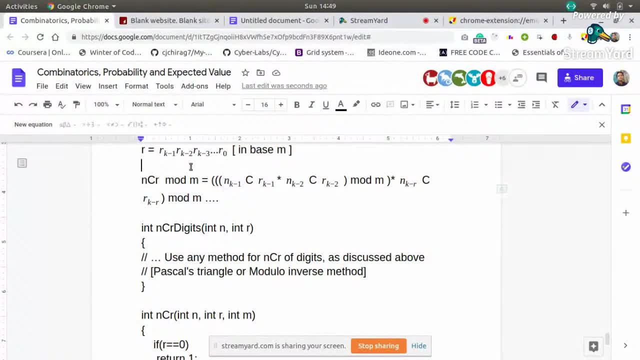 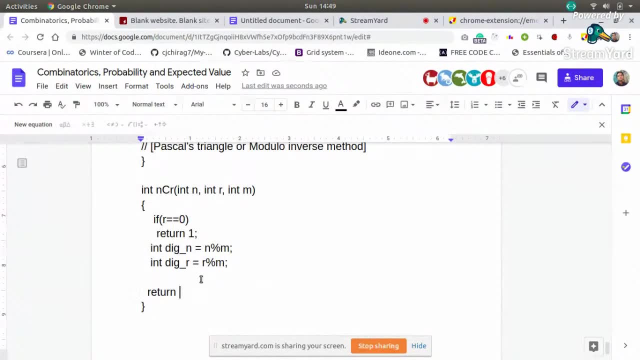 valid for every base. so the digits will be small. so you can use any primitive method, any earlier discussed method for that, for ncr of that. now i am not writing this function. you use any other method. now we will call this. this about function ncr digits for that, ncr digits for this digit of. 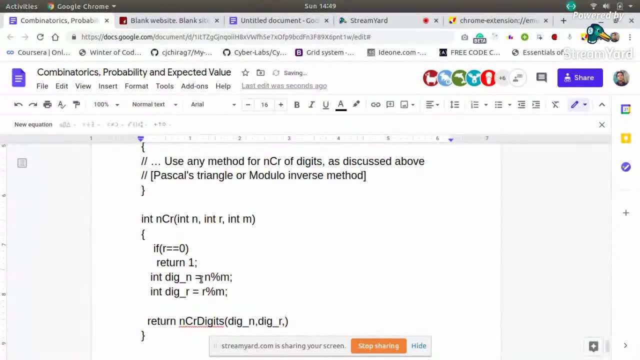 n digit of r, i will pass and i will pass this m here. so we will do this and after what we get, we need to multiply it with the remaining part. so the remaining part would be what the remaining part would be. we will call this function recursively, with the values as n by m, r by m and what is the? 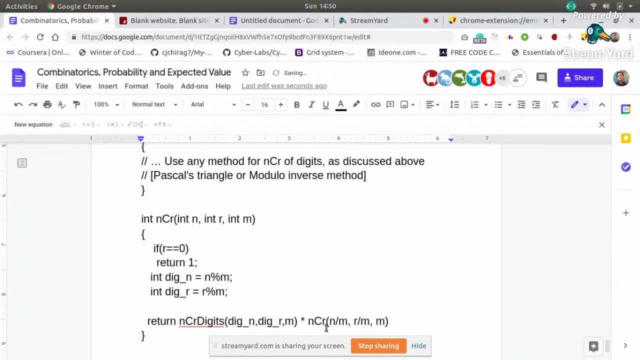 another thing. it is m. what. why i have done this? because this is the question when you divide n by m. so this will be called for our recursive function, because we are writing n and r in the base, m okay, and modulo. at every step you need to take modulo m so this will do your work. so i will give you one homework problem. 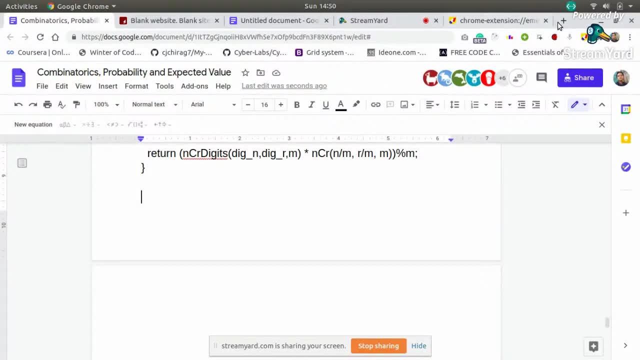 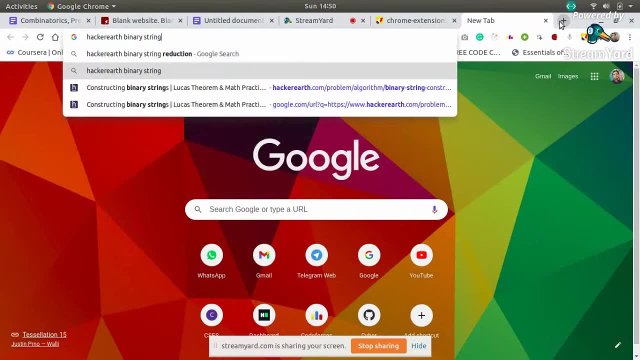 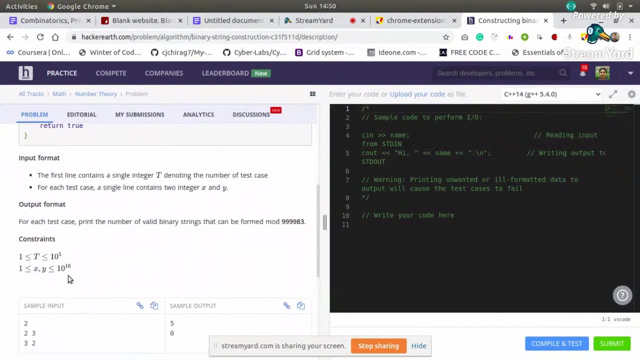 to try by yourself, so you you can try that problem. so binary string. so since you can see, as in in the in the problem, that here x and y very large of the order 10 to the power 16, but the modulo which you need to take is very of the order 10 to the power 6, so here you can apply locus theorem, because here, if 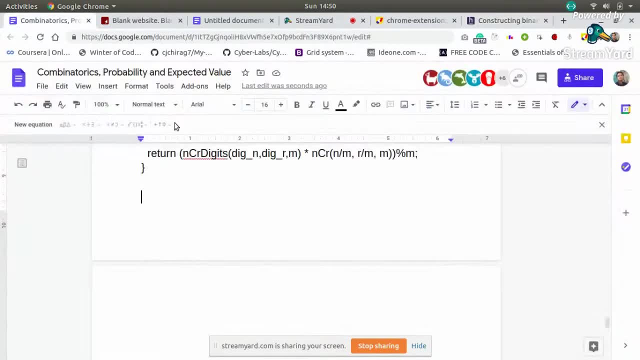 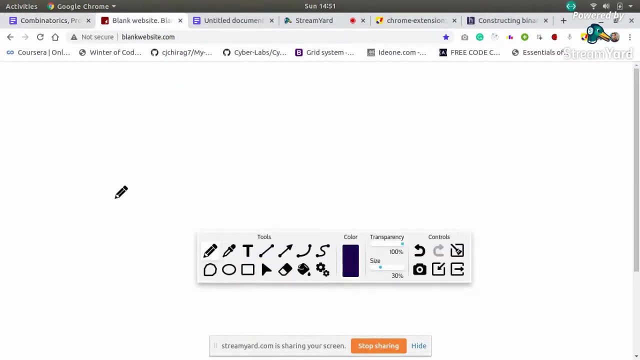 you apply the dp method to find ncr or any other method, you will fail. so just for practicing uh, practice this problem means try this problem, okay. so uh, whenever you get time, try this problem. so we will discuss some more prob, some other problems now. so, uh, let us come to one problem, for like, uh, suppose there are, uh, let us say there is a grid. 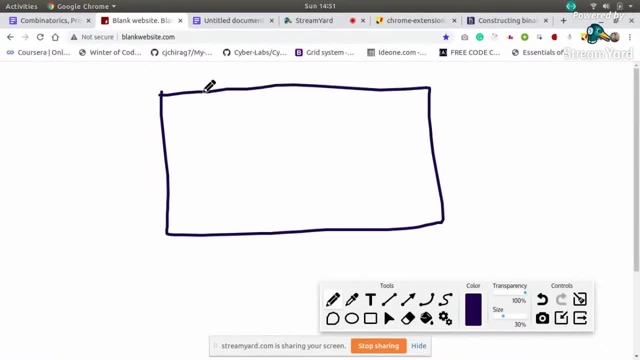 so there is a large grid and you can assume it. uh, in this way, it has some, some number of columns, some number of rows like this, and you need, uh, you are at the, uh, you can say bottom, most point, and uh, at here, you are at zero, comma zero, and you need to reach. 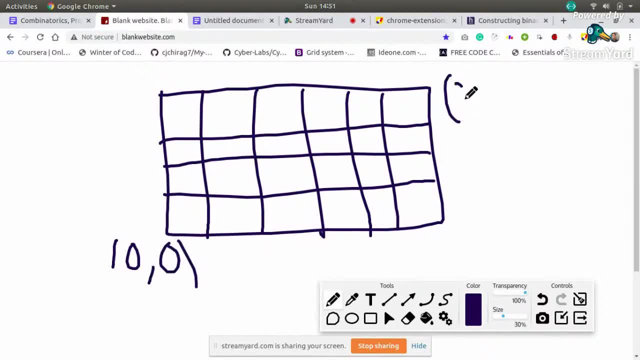 this point at the, let us say this is n, comma, m. so what would be the number of ways to reach if you can go only either to the right direction or above direction? in these two directions only, you need to move and you need to reach this place. 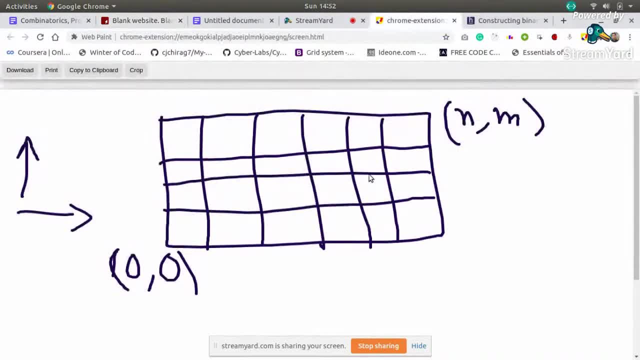 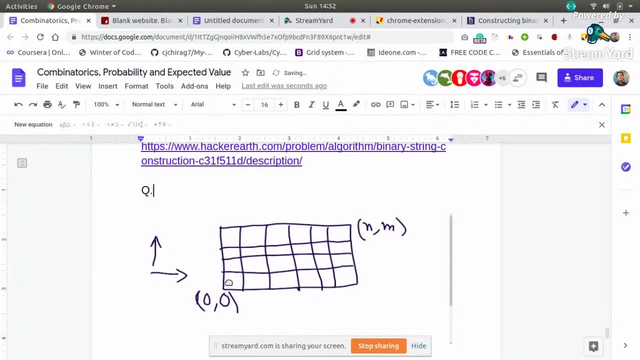 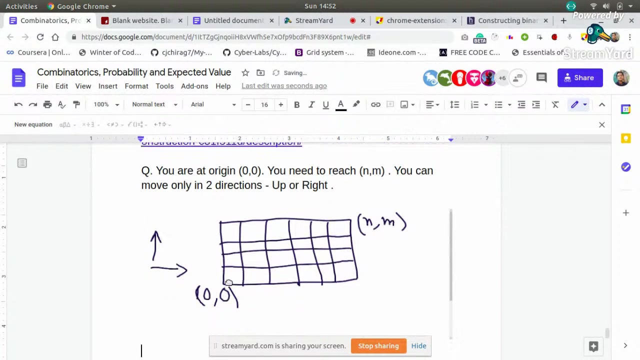 and the problem is so. the problem is this one. the problem is this one: you are at origin and you need to reach n comma m, but, uh, you can move only in two directions either. uh, either in two directions or in three directions. above You can say up or right. If you know, try to answer, Try to think in how many ways 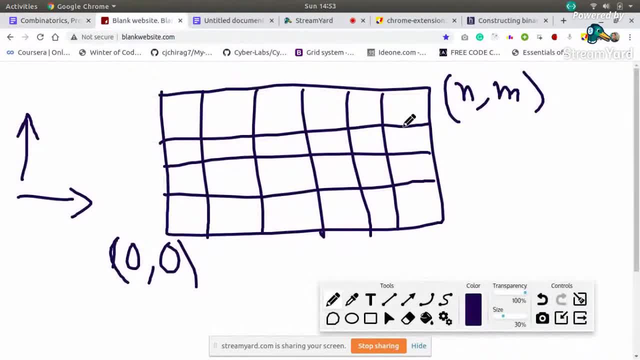 you can go from here to here, You are at this place and you need to go here. So one way could be like right, right, right, right right. then, up up up this way. this is one way. One way could be: right, right up, right up right, something like this There: 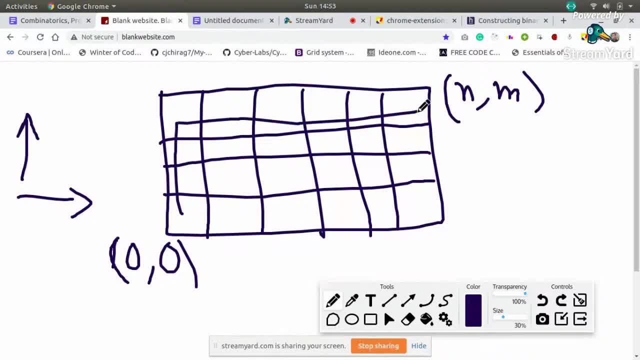 are many ways. So one way could be: up, up, up, up, up right, right, right right. So this is one way. So how many? the total number of ways would be? what Anyone any idea? Try. 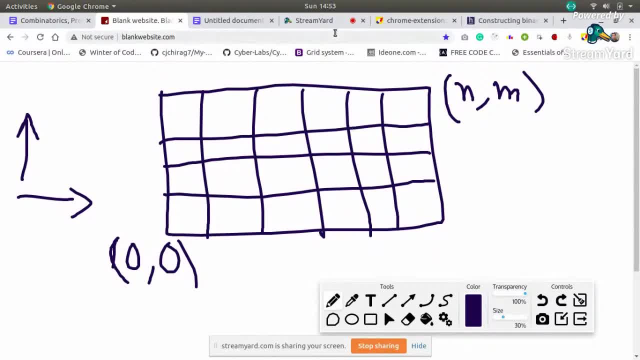 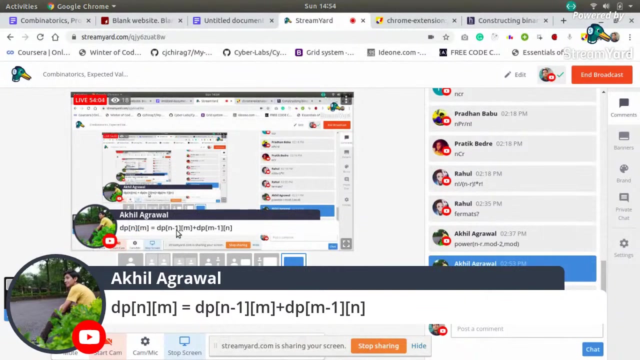 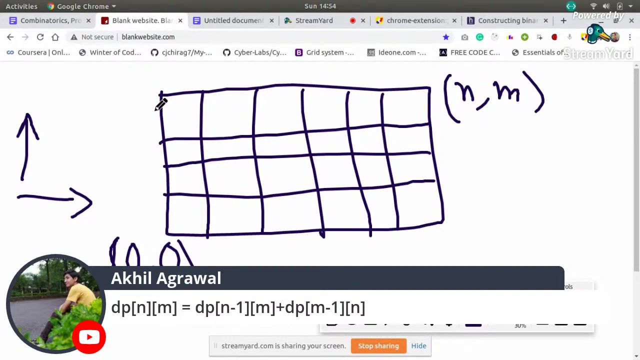 to answer if you know it or means if you know how to calculate it. So one way is to use DP. If you would use dynamic programming, it means you can use this recognition, So which Akhil has written: Okay, DP of M equals to DP of M minus 1 C, N and C plus DP of M minus 1 N Means basically: 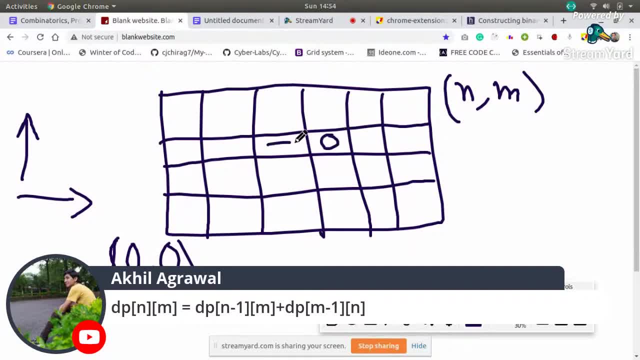 the idea is, if you are at this position, let us say X comma Y, so you can reach only from this place or this place. Okay, So this is this: the coordinate of this position is X minus 1 comma Y, and coordinate of this is Y minus 1 comma X, X. you can say X, this. 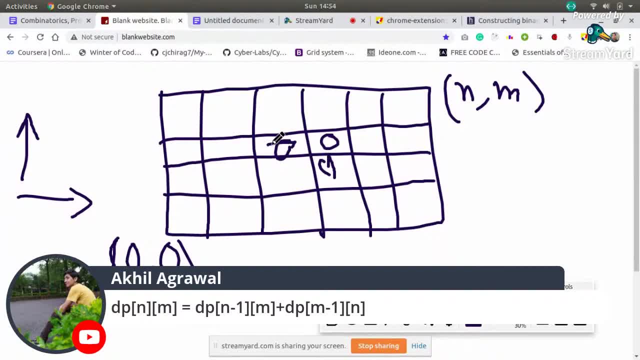 is X minus 1 comma Y, this is X comma Y minus 1.. So the number of ways to reach this place plus the number of ways to reach this place. So it would be something like this. So this is one way, but suppose the N and M are very. 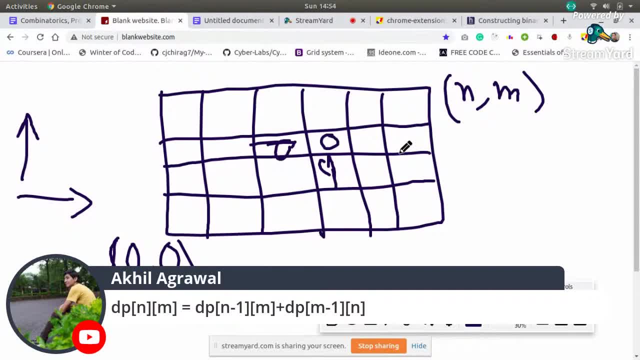 large. The dynamic programming method can be used when N and M are of the order. let us say it can be used only when N and M, multiplication of N and M is less than equal to 10 to the power six or seven. So the dynamic programming method can be used only in this case. But 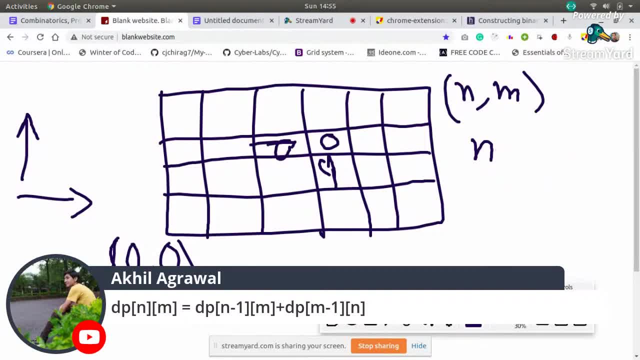 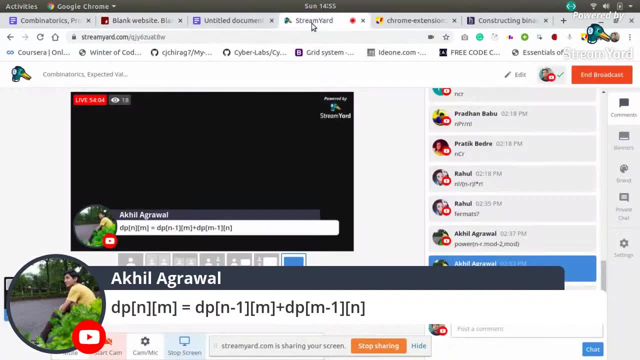 suppose N and M are very large. let us say N and M are of the order 10 to the power nine. Okay, N and M, N. both are 10 to the power nine. So this will give MLE dynamic programming. you cannot use that time, So any other idea? 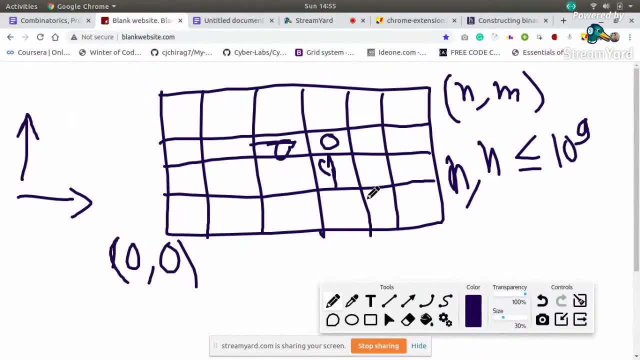 So, basically, if you think by the way of combinatorics, combinatorics, so if you see every path can be written in this way, like you want to reach this N comma M place, So in any case you choose any path, So you always need to go. since this is N comma M means you need to go N times. 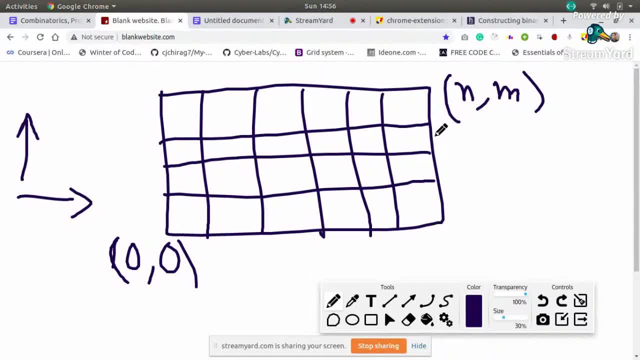 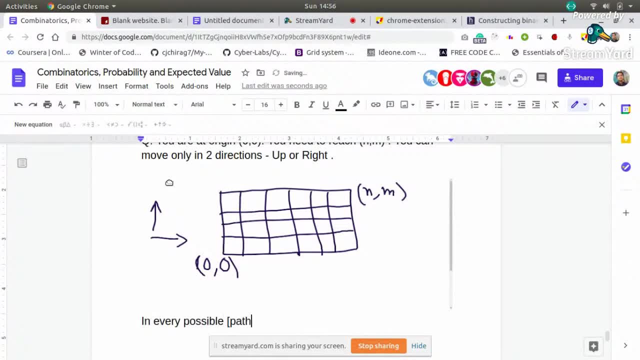 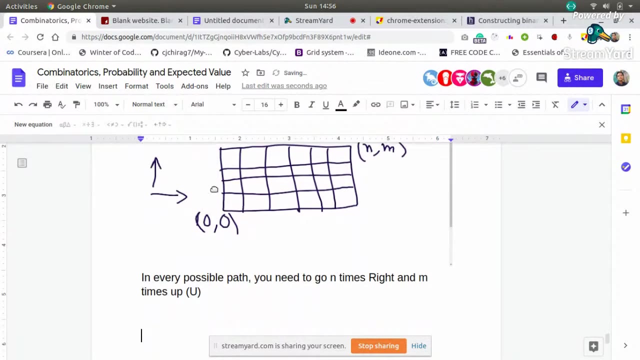 to the right, N times to the left, N times to the right And M times above, M times up. So in every possible path, if you take any path, in every possible path you need to go N times right and M times up. I am denoting up by U and right by R, So like 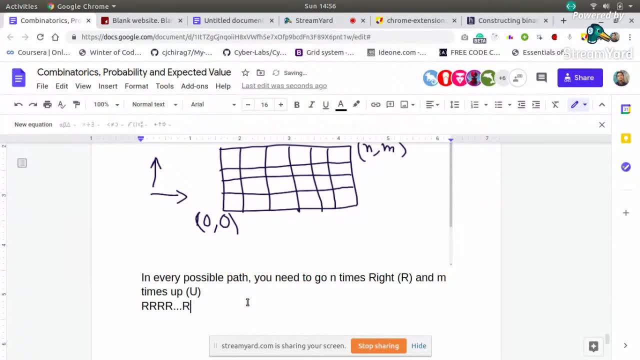 one path can be R R R R R up to N times, And then you go U U U up to M times. Okay, So, and every path will be just a permutation of this. Okay, You draw any other path, like. 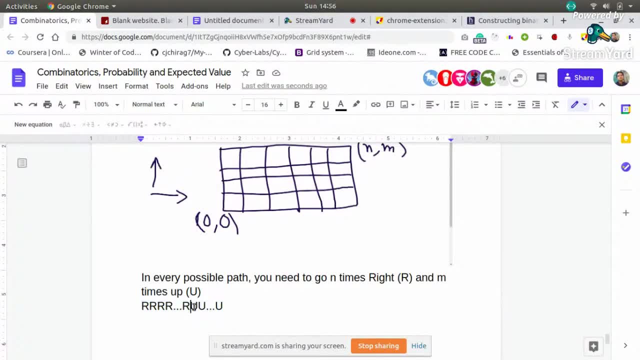 it can be first U, all the U, then all the R, But at every path, since you cannot go down, since you cannot go to the left, so you are bound to take this path. Any permutation of this will work. So all the paths are just the permutations of this string: R, R, N times. 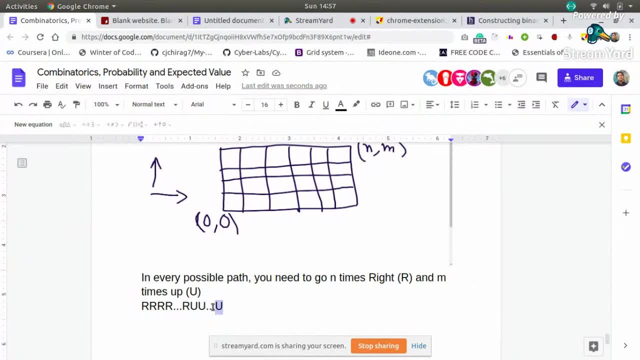 and U U M times. Okay, So just what will be the number of permutations of this string? So, number of permutations of the above string, So number of ways This is clear or not? Number of ways to reach the cell N, comma, M equals to just the permutation of this string, Because 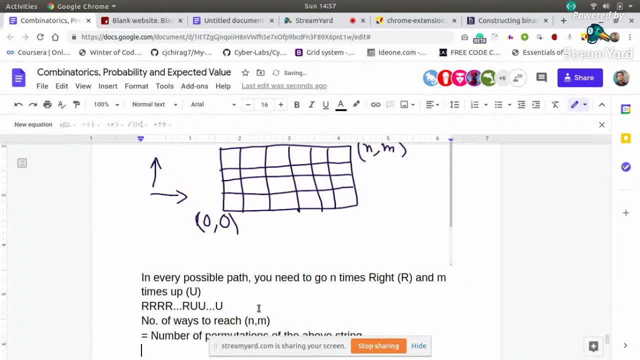 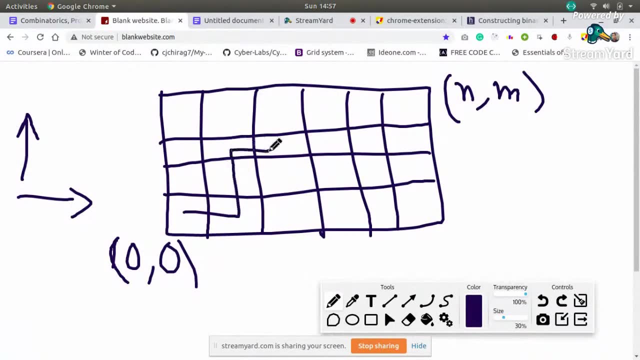 every path can be written this way, Since you cannot go to the left or down. Okay, You cannot go to the left or down, Only you need to go up or right. So every path, like this path, is there: Right up, up, right up, right, right, right, right. So you find that. 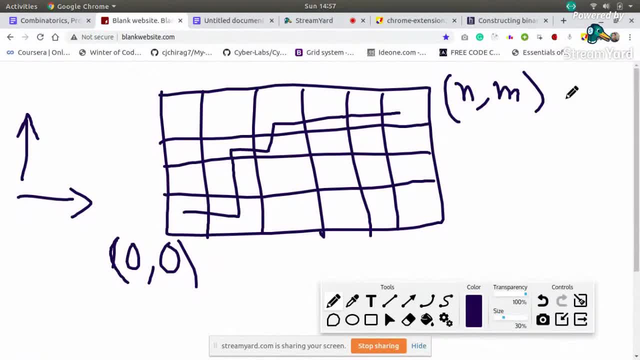 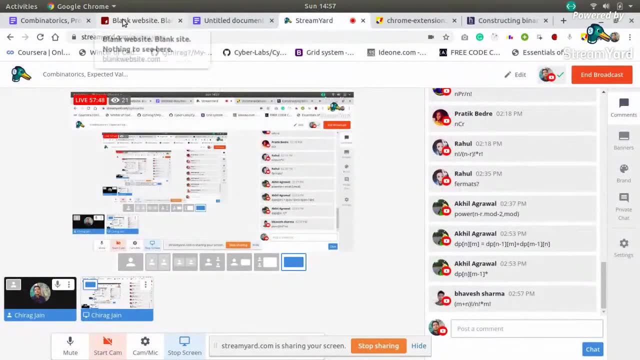 summation of R will be always equal to means. you need to take M. you need to take N right steps in any case, And you always need to take exactly M up steps in any case if you want to reach this cell N comma M. So our answer would be Yes. The answer would be: 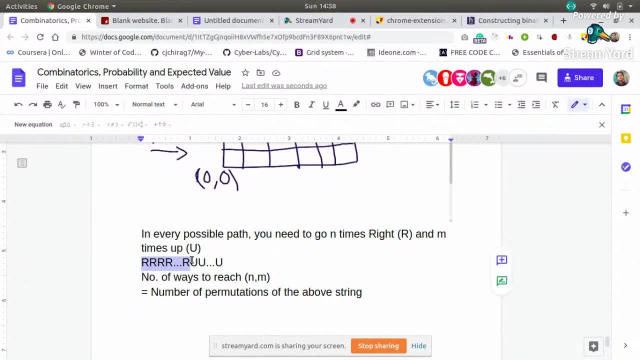 yes. Well, since there are how many, how many R's are there? There are N R's and there are M U's. So the number of ways to arrange this string is just N plus M factorial, divided by, divided by, since, since this R is same, So R, you will have N factorial and M factorial. 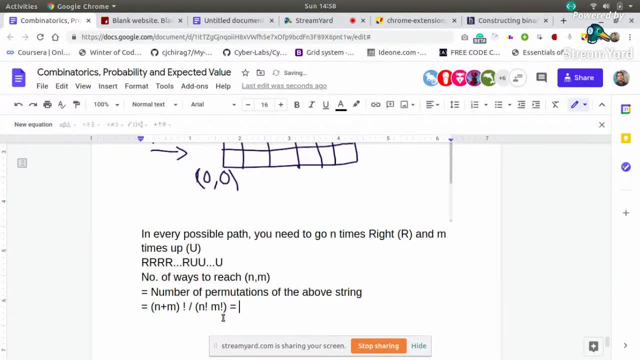 Right, Okay, So if you, if you want to write in the form of this, this, this in the form of combination, so it will become N plus M C N, So it can also be written as N plus M C N. Fine, Because 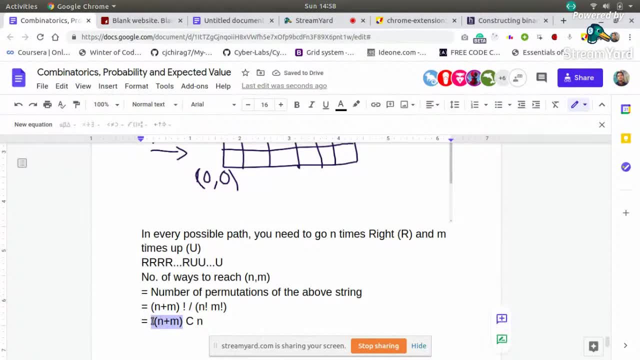 if you apply the formula of combination, it becomes, if you consider this as capital N, and then what will be capital N minus a small n? it will be M. So we have N C, R equals to N factorial by R factorial into N minus R factorial. So this thing is same as this. 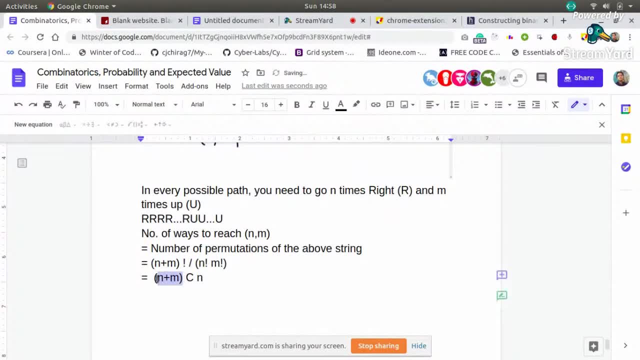 If you write in the form of combination, so both are same. So you know how to compute N plus M, C, N. Suppose the answer in the in the question that is asked to compute this thing: modulo M, modulo some P, where P is some prime number, So you can compute it. 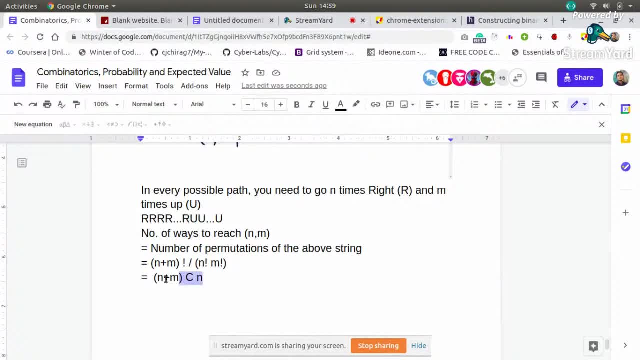 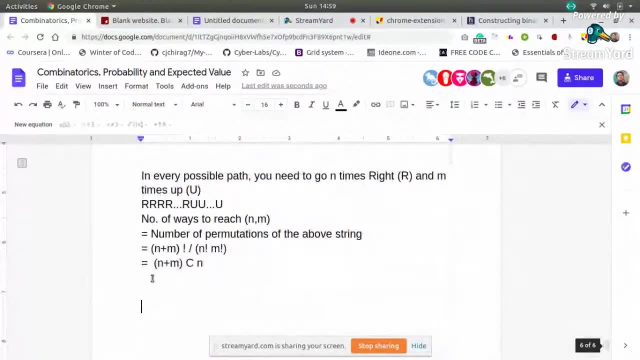 Suppose N and M are of the order 10 to the power nine or 10.. Then also you can compute this thing How? By Lucas theorem, you can compute the modulo if, even if N and M are very large. Fine, So this will work. So, but this was one question. I hope it is clear. 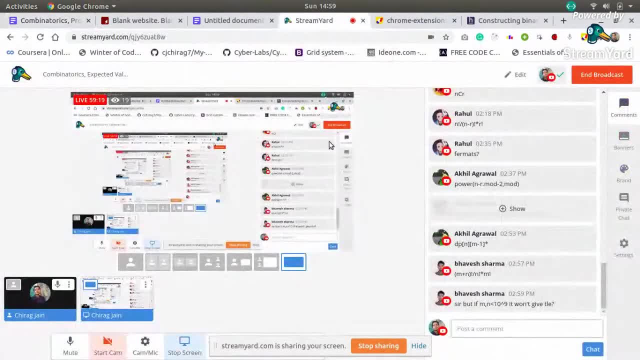 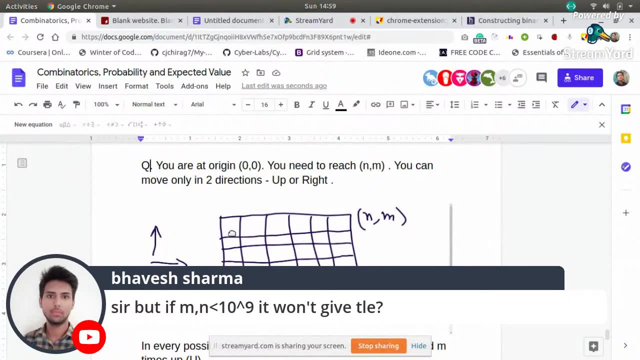 If it is not clear, then please mention what. what problem you are facing? Okay, Okay. So one question is that if M and N are greater than 10 to the power nine should, would it give TLE? So it will not give TLE. if you compute, the means what you 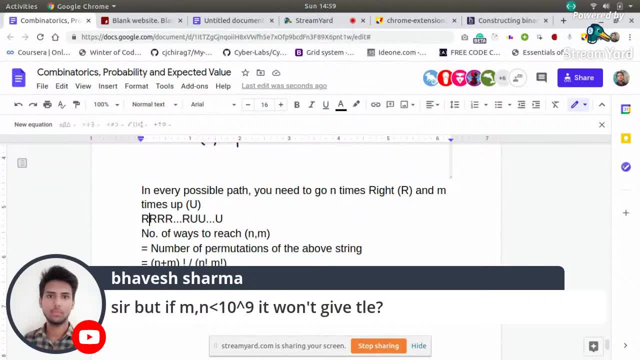 need to do? you need to find just this number and some NCR, some NCR value, And you know how to compute the modulo of some NCR value. So the time complexity of this. I forgot to tell you the time complexity of this Lucas method. 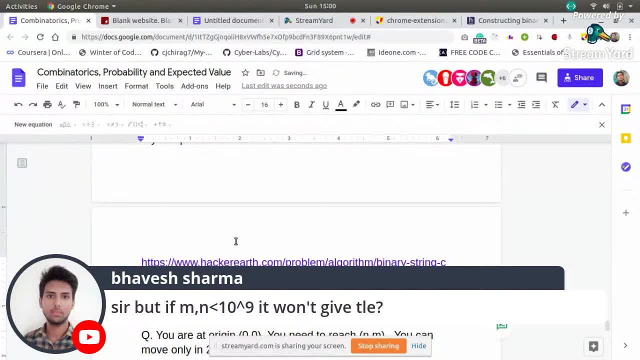 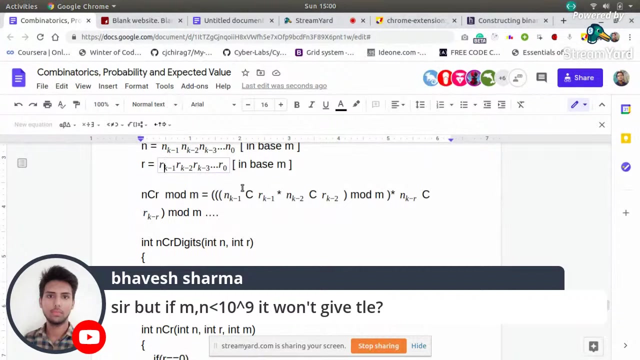 Time complexity. Time complexity of this Lucas method is O of log m. Why? Because if you are writing any number in base m, so always there will be. you can say: for every digit you need to go there, So there will be how many digits in that number. 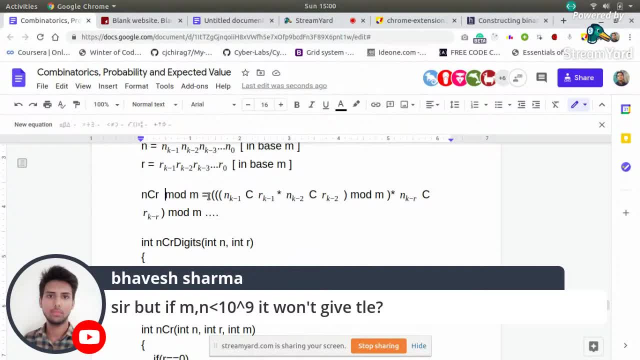 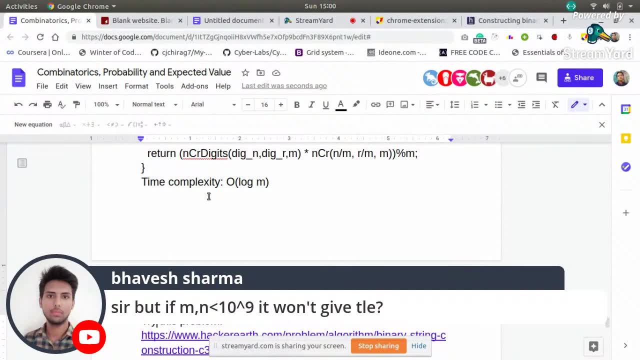 It depends on the number actually, So that the log m, log n, base m, something like this. The time complexity of Lucas theorem should be something like this: OK, let me think The space complexity would be obviously very less because you do not need to have any extra space for anything. 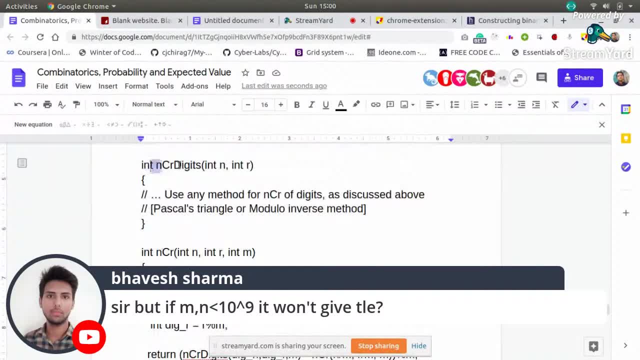 except you need to just compute for all the digits. You just need to compute the factorials. For that you need some space. But if you see the time complexity, we are just going through all the digits of the number and of the given numbers of which you need to compute ncr. 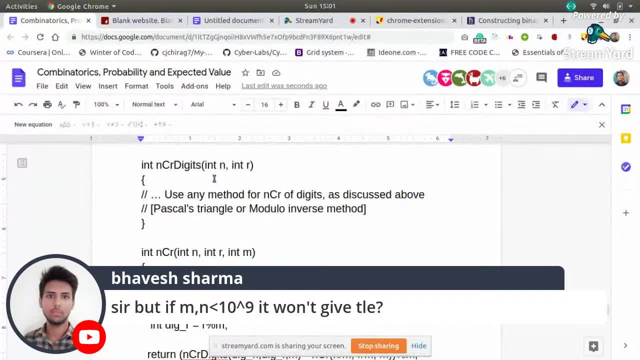 So the time complexity would be of the number of digits in base, m of the number, So how many digits it can have at maximum is It would be. yes, It would be. It would be log of the n and r, n and r. 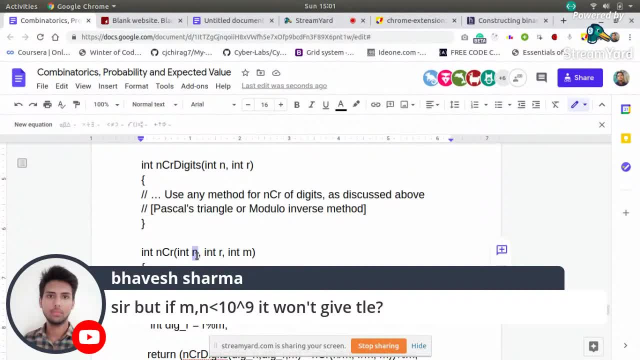 Since r will be always smaller than n. so we can take log of n base m, That will be the number of digits And for each digit, just we need to compute it So you can write it as time complexity would be log of n. 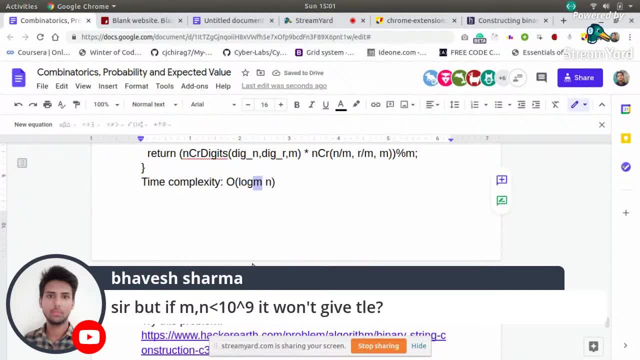 base m. m is the base of log multiplied by the time complexity of log. OK, So the time complexity of computing this ncr of digits. So this ncr, if you compute in o of 1 or o of log m. let us say: 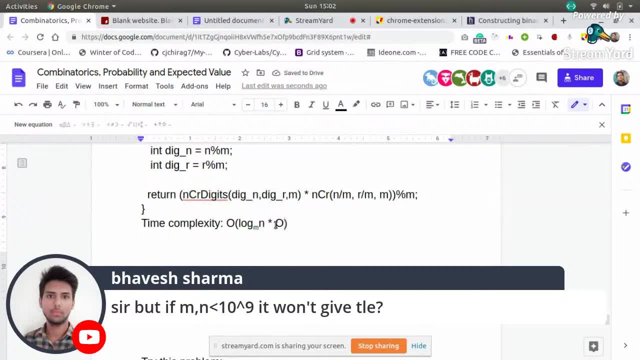 So it will be multiplied by it. So let us say we compute it in log m, So it will be multiplied by log m. It depends on this ncr digit function. If you are using Pascal's triangle, so it will be o of 1, so accordingly, 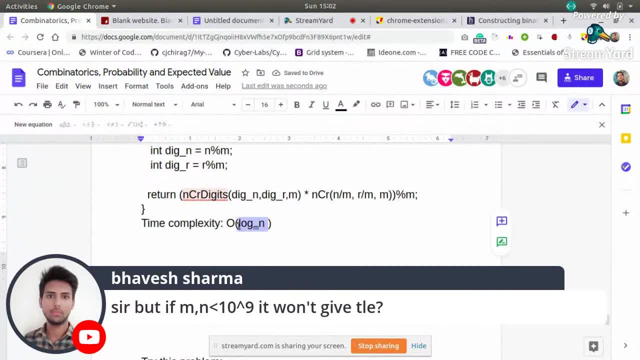 So m means into something. This thing would be always there Because if you are writing any number n in the base m, there will be always log. So log n digits, log n base m digits. So the time complexity would be this: 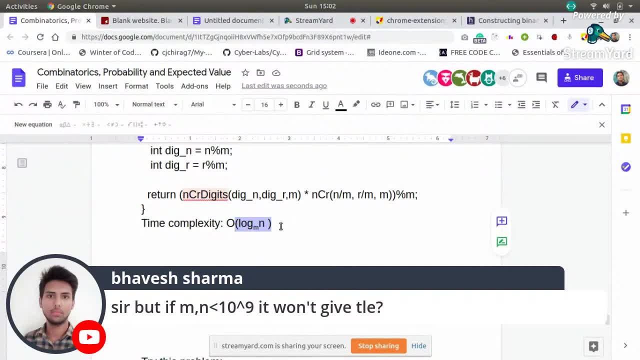 So you would not get t ad when n is 10 to the power 18 also. Then, also assuming that this because this log will be always small, so you will not get t ad. OK, so this is the time. complexity of applying this Lucas theorem. 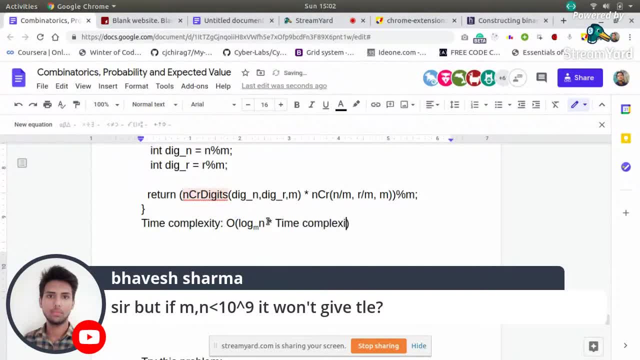 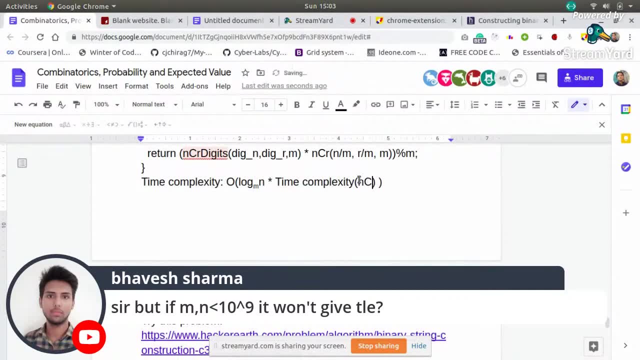 I am writing: multiply k. I am multiplying it by the time complexity of whatever function you are writing for this thing: ncr digits. It depends on this time complexity, also the time complexity of ncr digits. I hope it is clear now. 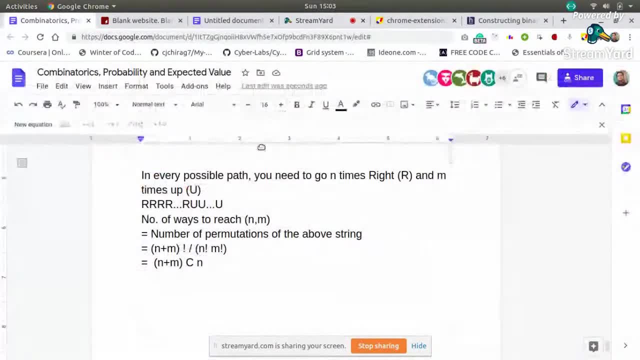 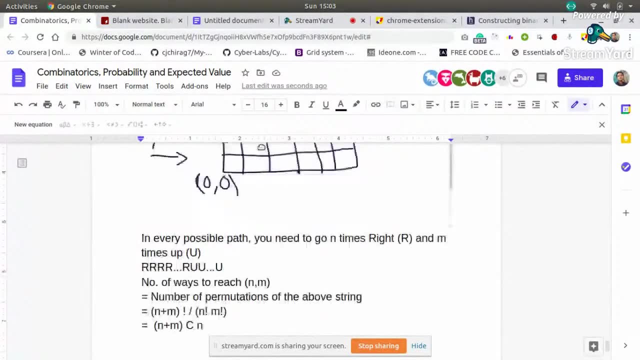 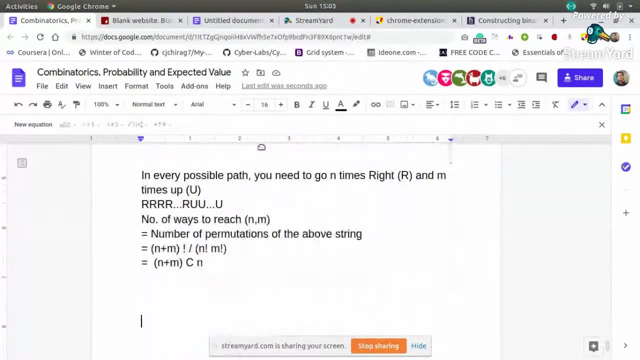 Any other difficulty we are facing. OK, so now I modify this question Like: now you need to Like. let us say you have the same problem, but now you think in three-dimensional space. So just try to answer like what. 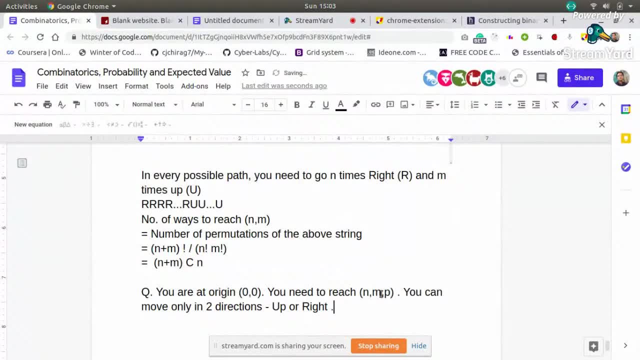 would be the answer when you need to reach some n m p, And you can move in three directions now: either up or right, or up right, or, let us say, forward Means just in the positive direction of x-axis, y-axis. 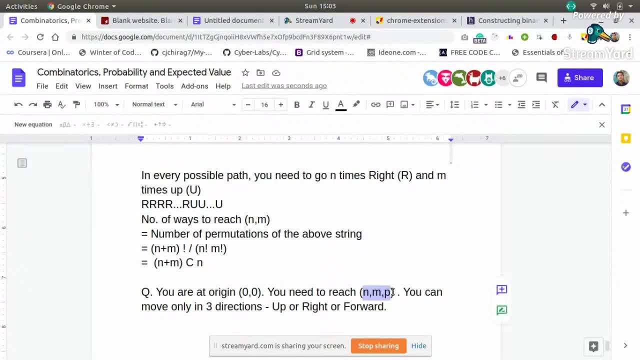 z-axis. So you need to reach this point Just in three-dimensional. it is now. So what would be the number of ways You are at origin means this. So this is the 3D version of the above problem. 3D version. 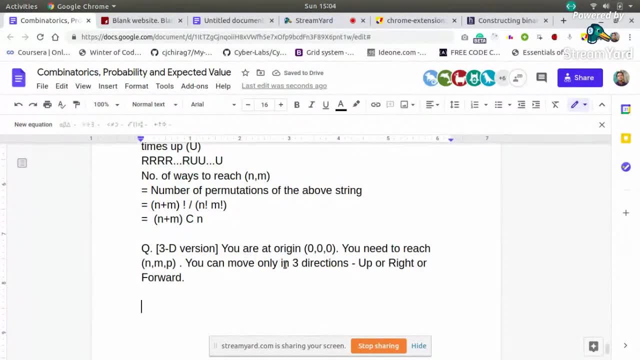 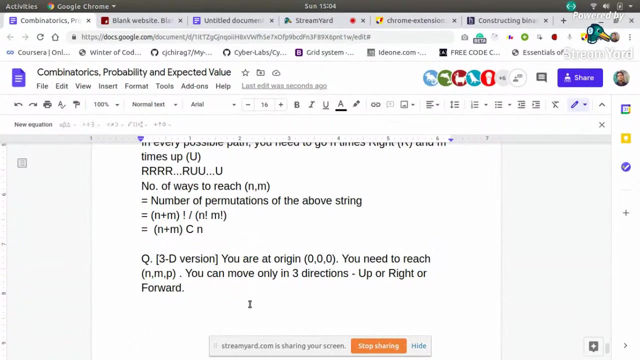 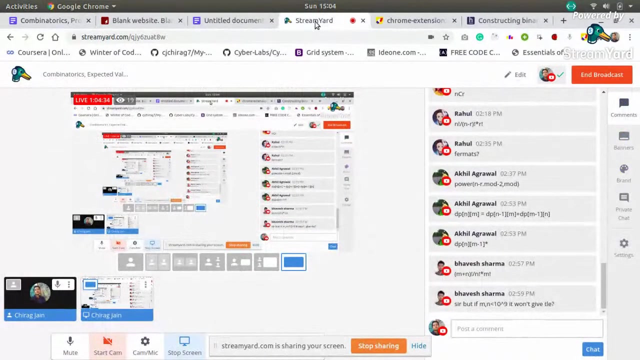 Can you answer similarly? So OK, I will give you 30 seconds or one minute. Try to think and write the answer. BHAVAT SUBRAMANIANDI, SPEAKER 1, BHAVAT SUBRAMANIANDI. 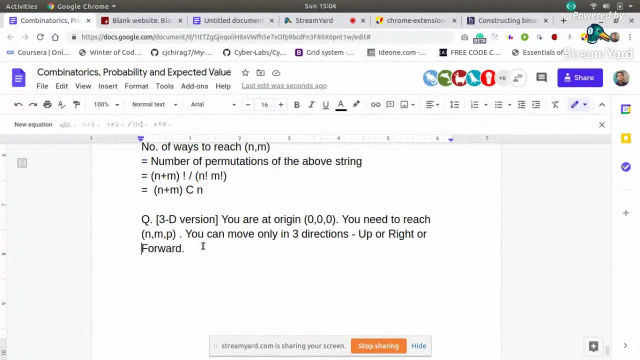 SPEAKER 1, It is just similar, Like you need to reach this point, point and you can move in these three directions. So just what the string will look like. Like, if you want to read this, what your path would look like. 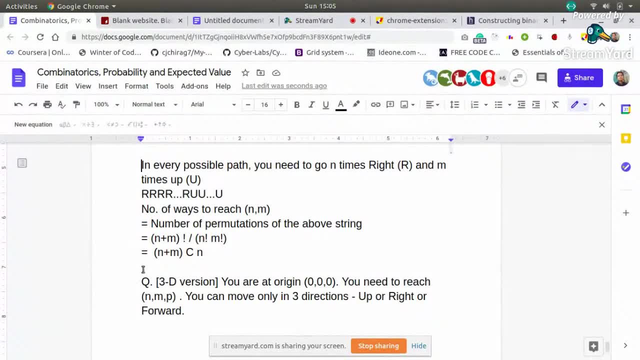 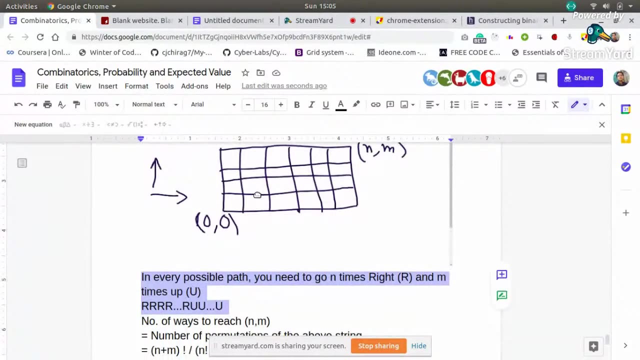 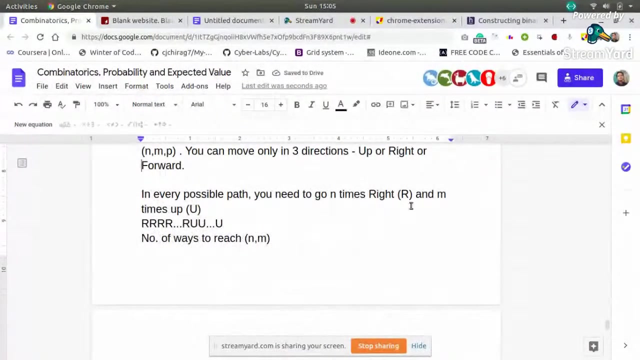 So in every path you need to go to n times right, m times up and, let us say, p times forward. So these are the three directions, So the string here also the similar thing will be there. So in every of the path you need to go n times right. 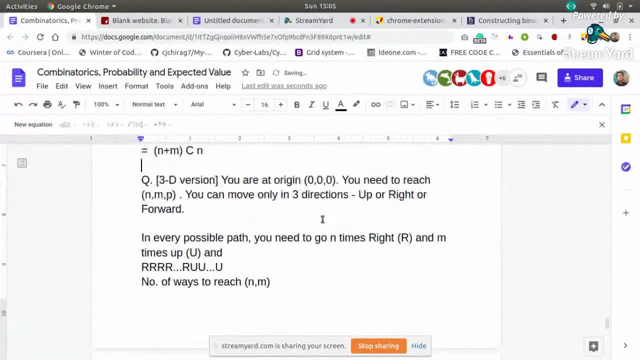 and m times up and let us say how many times p times forward. So you then after that p p, p, p p times something like that: Sorry, p f forward, p times f. 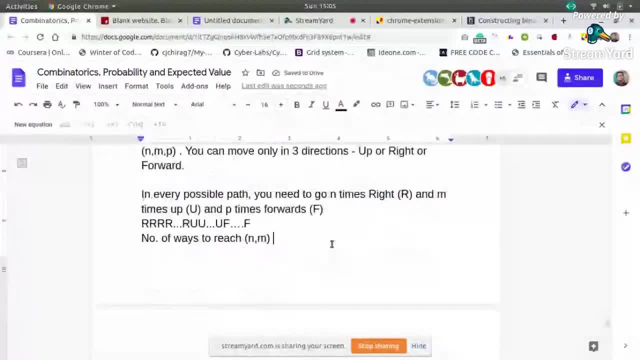 So the string would be something like this: So just you need to find the pattern, You need to find the permutations of this string. So the answer would be: permutations means total number of characters in this string is n plus m plus p, and that n plus n plus p, factorial divided. 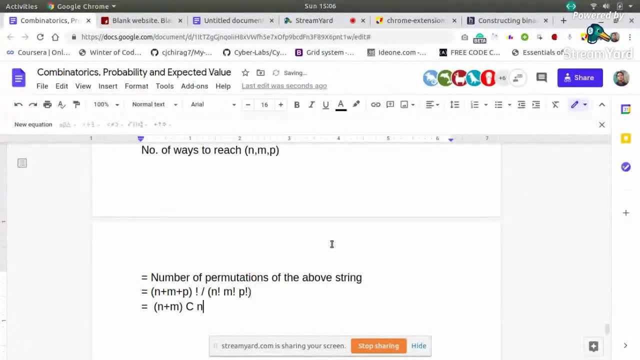 by n factorial, m factorial and p factorial. This will be your answer. This will be your answer, And OK. so if you write, If you know multinomial coefficients, so you can also write in the form of that. So it will be like n plus m plus p comma, n a m- p. Like multinomial coefficient. 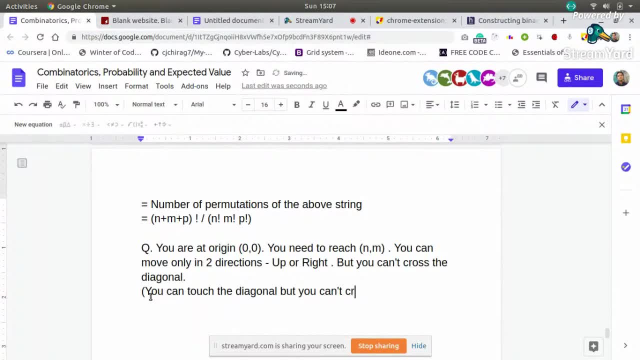 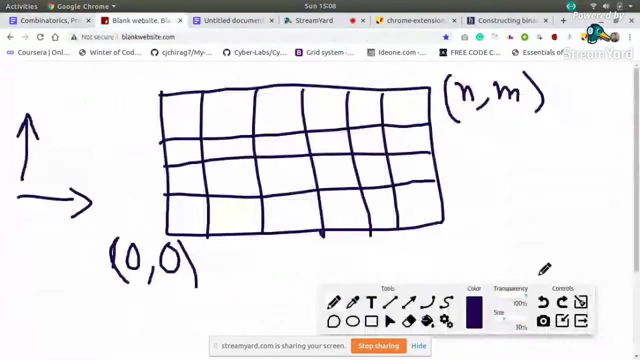 can't cross, it means you cannot go to the other side of the diagonal. so this is the condition. so you need to find the number of ways to reach n comma n such that you cannot cross the diagonal. so any idea about this? try to write in chat. 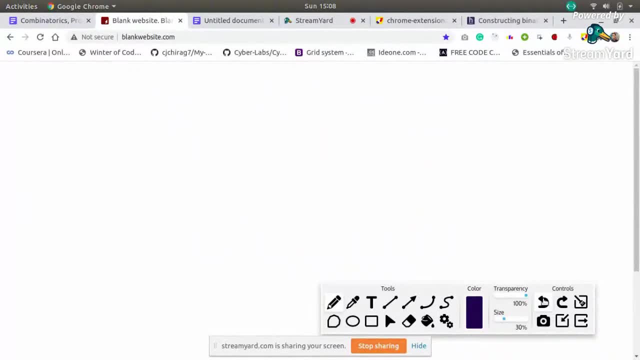 if you have any idea, okay, one hand. I can give just the total of the number of ways of paths you know to reach n, comma, m. now you subtract the invalid paths. what are the invalid paths possible? so try to find out how to count the invalid paths. Invalid paths are those. 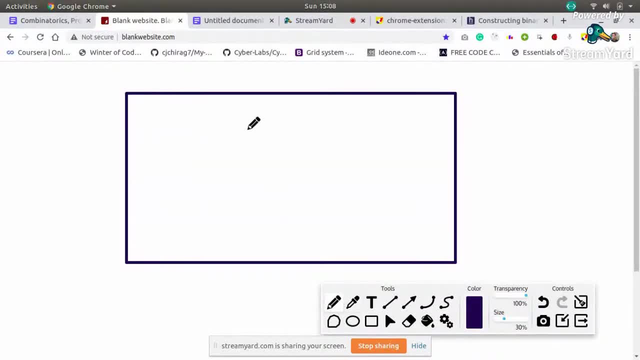 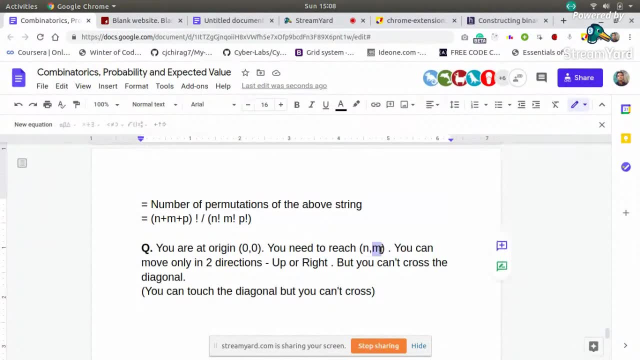 which are just, you can say, crossing your border. and now let us simplify the problem. this problem is now not for n comma m, but it is for n comma n means it is just, you can say, a square grid now from 0, 0 to n, to n: n. 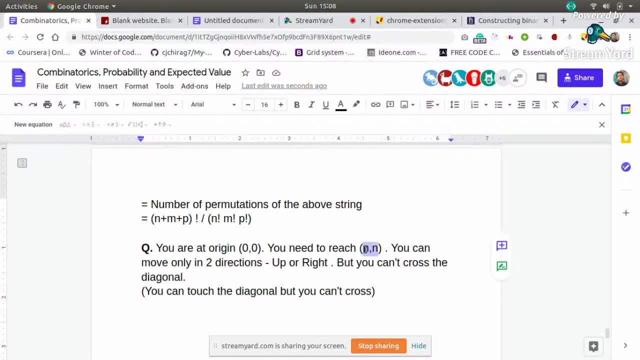 I simplified this now. just you have to remember that this is only a diagonal, but it is also a當然- n comma n point, as you can see, into this n comma n point and you can move in 2 directions only, either up or right, but you can't cross the diagonal. 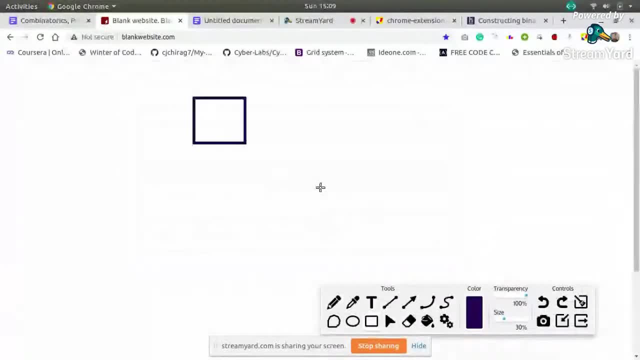 But you touch the diagonal but you can't cross it. So now it is a square grid and it is a pattern and you cannot say n comma, n point, as we have done for now. so I am going to reduce this limit so like: uh, the diagonal would be something like this: 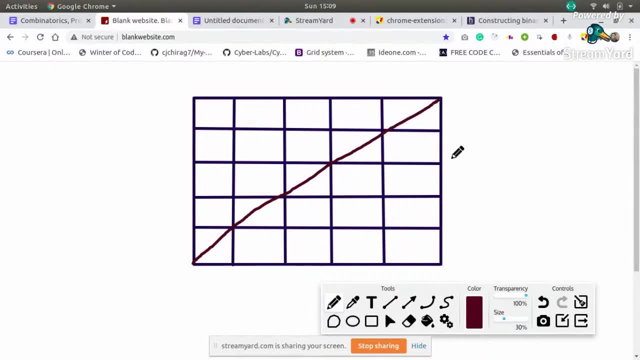 so like one possible path is like, if you go this up to this, up to this, i told you you can touch the diagonal. so i am just touching it, but i am not going across means i am not going to the that, this part here. so some path like this: this is one possible path. 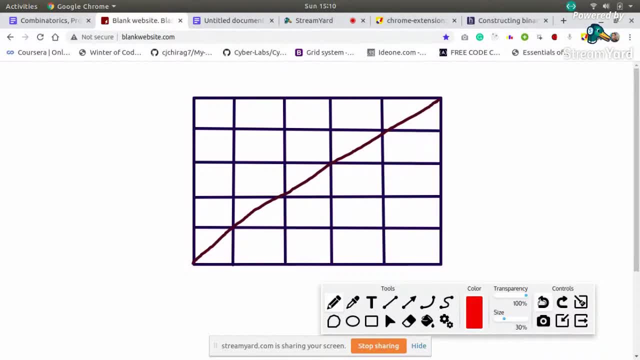 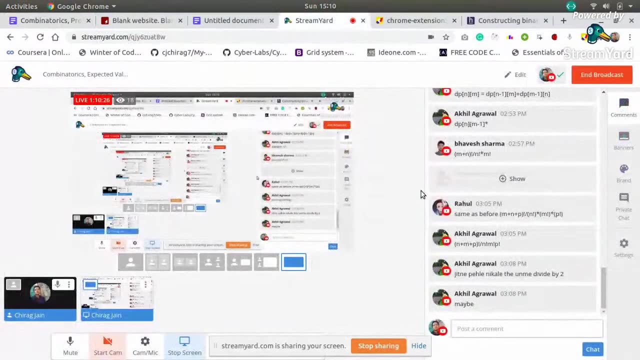 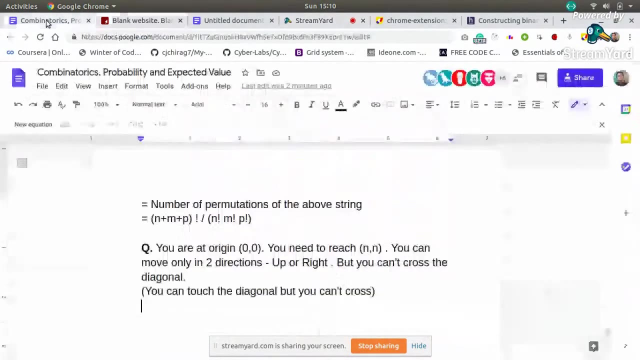 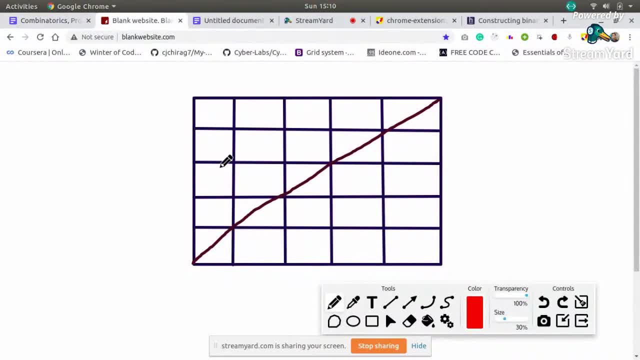 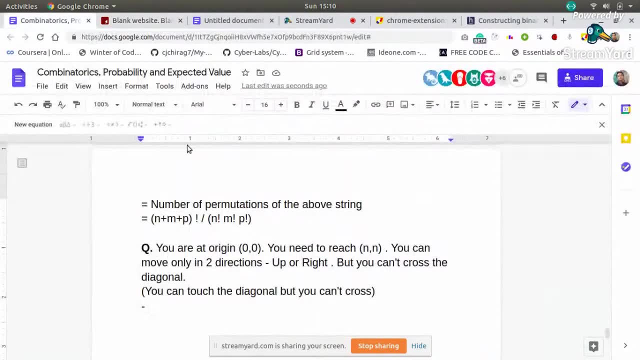 he uh, is he he when you observe all the paths. so it will be like this: he uh. your path will contain: uh means your path. you know that your path contains n r's, uh and n ups, so it it is just a, it is just a permutation of. 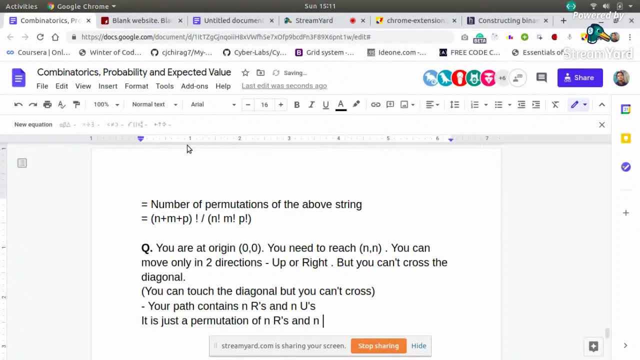 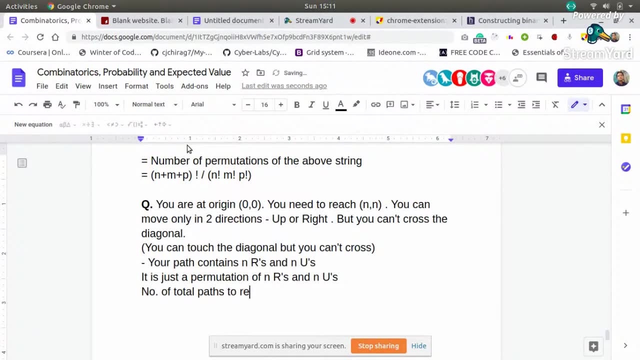 n? r's and n? u's. so, uh, the number of total paths needs to reach, to reach n comma, and you know it. okay, what is the total path? it is just 2, n, n plus n is, and plus n equals to 2n, so 2n factorial. 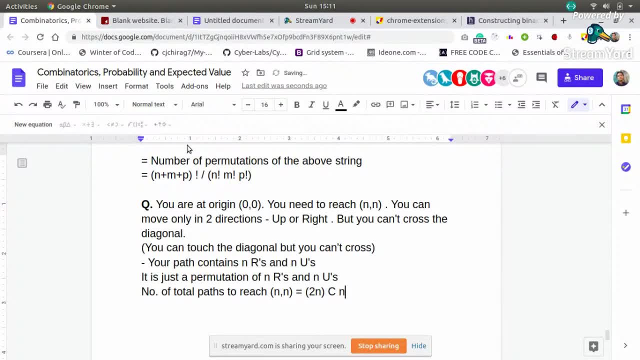 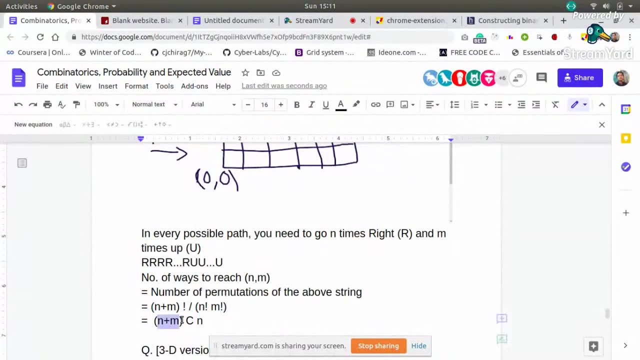 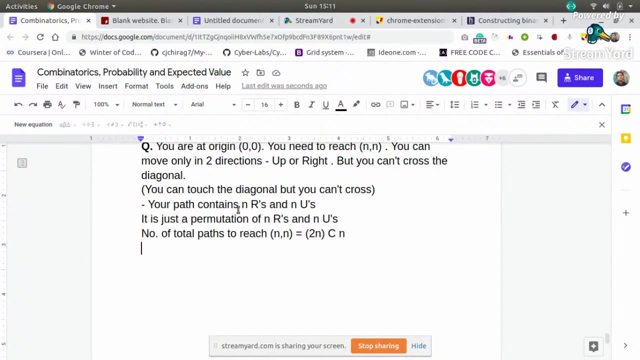 2, n factorial divided by, or even say two and gn. how this has come, we have already derived. it means we already uh, just solve it for when we needed to reach n comma m. so you put m equal to n, so you will get n- cn. there is one condition: you cannot cross the diagonal, so you find the invalid paths. 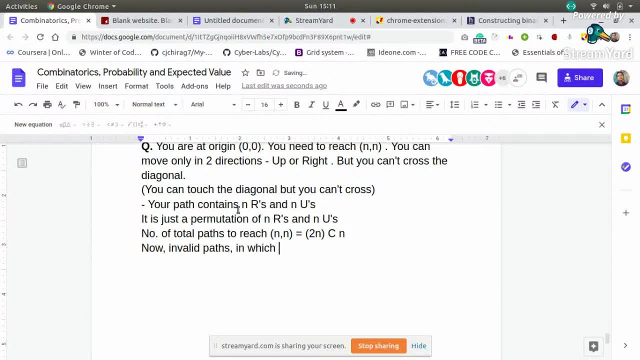 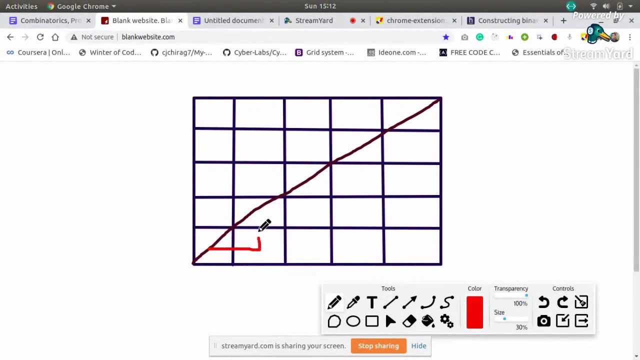 now, uh, invalid paths in which we cross the diagonal. we need to find them. so let us observe any pattern which we find in the invalid paths. so just try to observe any pattern. now let us say i'm drawing an invalid path, so i go right, then i go up up, then again. 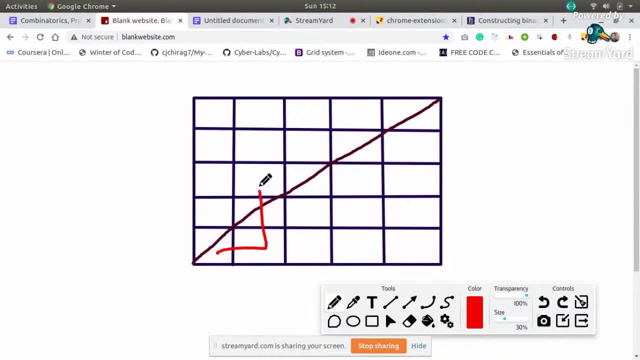 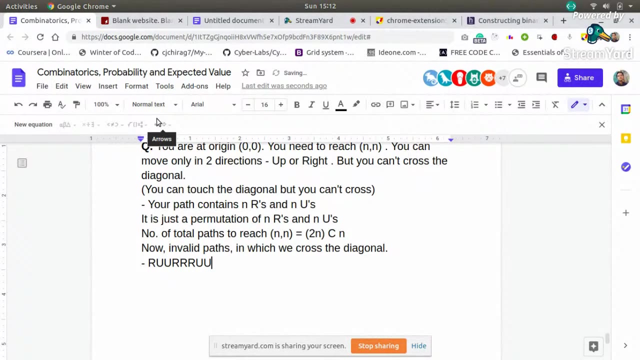 let us say i i go right up up, right, right, right up up, something like this. so i'm writing this pattern: what is it right up up? so it is right up up, r, r, r up up. is it the same four times up and four times r. 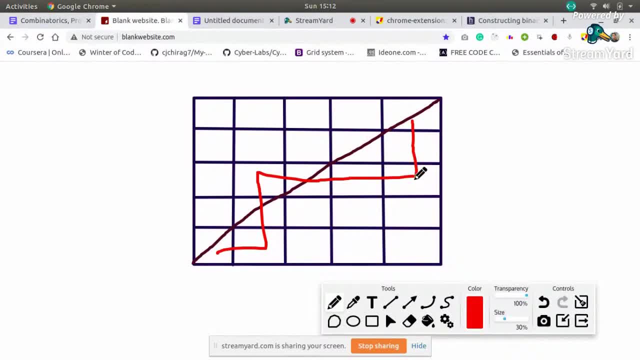 i think this is the same: right up, up, right, right, right up. so this is one path. now, just, uh, let me draw one another path in some other color. let us say: let me draw this path, let us take it right, right up, up, up, right and up. 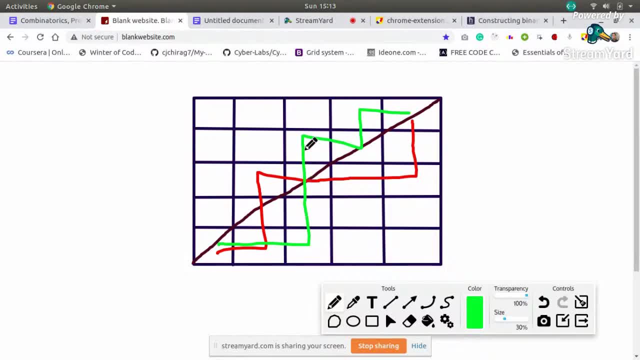 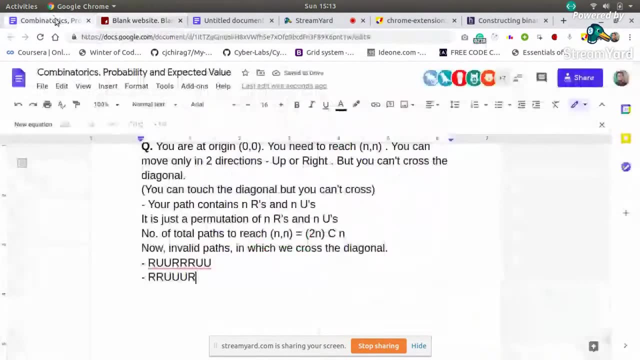 right, something like this: so r r u u u, so it is r r u u r r u u. you are, and you are, it is like this. so, uh, similarly, you can draw many more paths. so main thing i want to tell you is now: observe one pattern key. uh, if you just 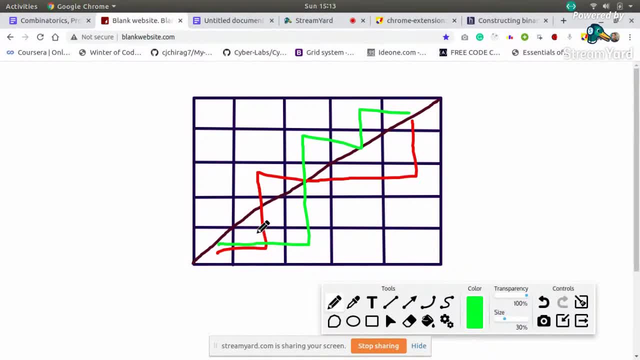 find the first, first, first alphabet which crosses the diagonal. so if you do not want to, if you do not want to cross the diagonal, it means that r should be greater than u at that moment. okay, you, you, you can know it like: if i have more r's, then i am always below the diagonal, but at the moment, 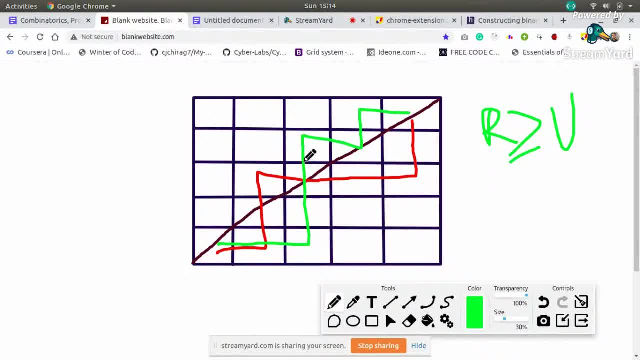 i have more up than the r when, like at this point, i have more up. so you find there are two r only and there are four up. one, two, three. there are three ups. so i have more ups than rights. so whenever i at that point, whenever i have more u than r, that time i am above the diagonal. i am at 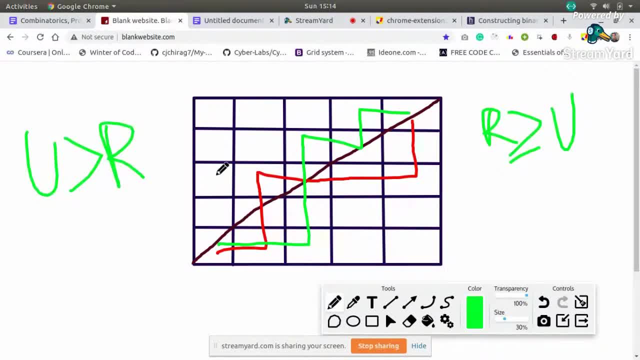 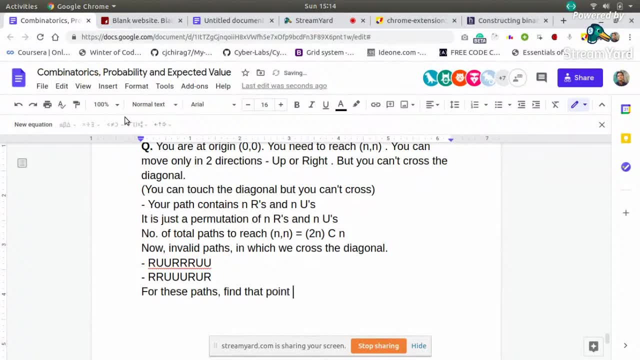 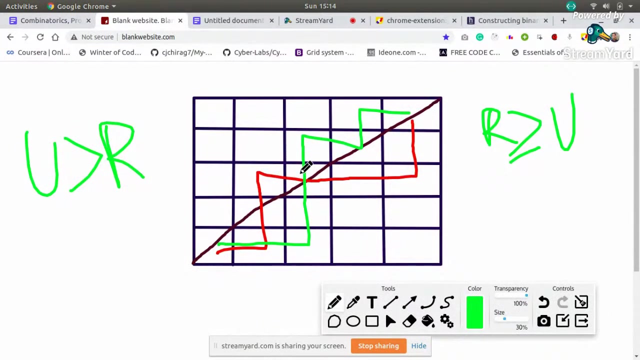 i am above the diagonal. okay, so uh, just find that point. so for these parts, find that point at which, uh, we are above the diagonal and reverse this path means and uh, reflect this path. or we can say so now, now i am just reflecting the whole path. so reflecting means like, uh, just a convert r to u and 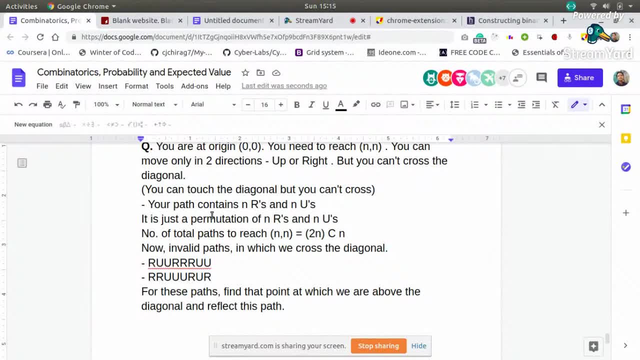 u to r. so like it can be after reflection what this path will become now. like you see, in this particular point r u, u. so i reach above the diagonal and then i am at the point where i am the diagonal when i find a second u, because at this time r and u are equal. so when i was having 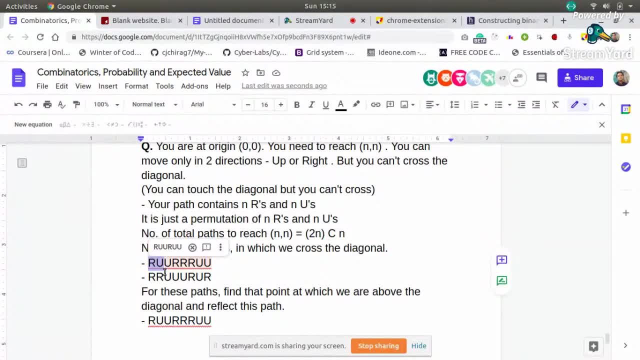 these two alphabets, so r and u are equal. so i am just below the below, or just touching the diagonal. but once i find one more u, so the number of u become more than the number of r, so i just reached above the diagonal. so since i reached above the diagonal, 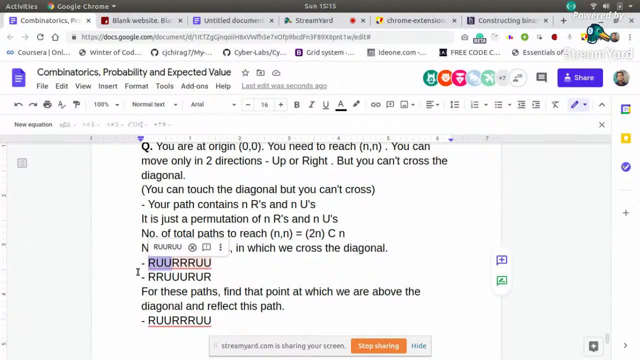 since i reached above the diagonal, i need to just just uh. just, i'm observing one pattern, so i just reflect all the remaining means. i just uh wherever. wherever there is r, i, i write it as u, so it will be u, u, r, r, something like this. so i am just 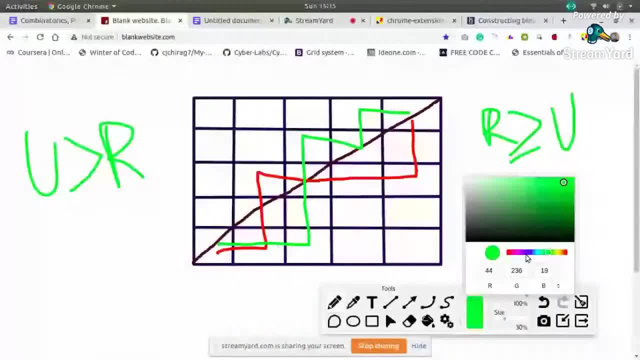 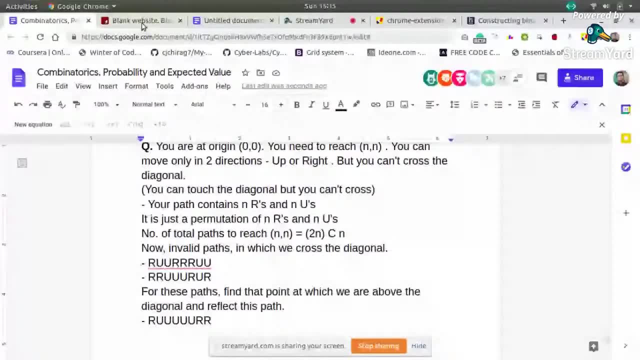 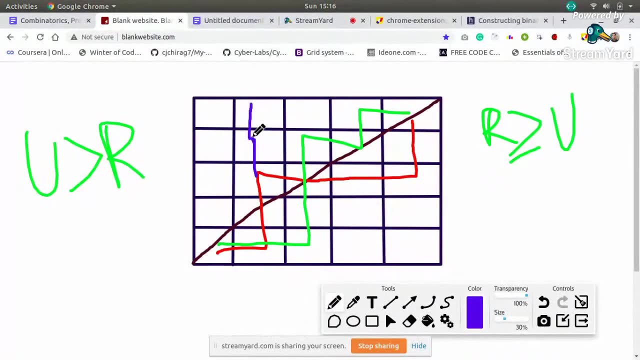 reflecting this path. so let me use any other color. so i am reflecting this red path. so it will that up to three points it will remain the same. so one, two, three: here it is remaining the same, but this r will convert to up. this r will convert to up. okay and uh. 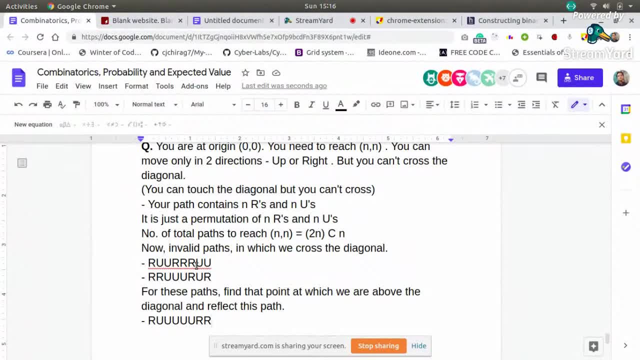 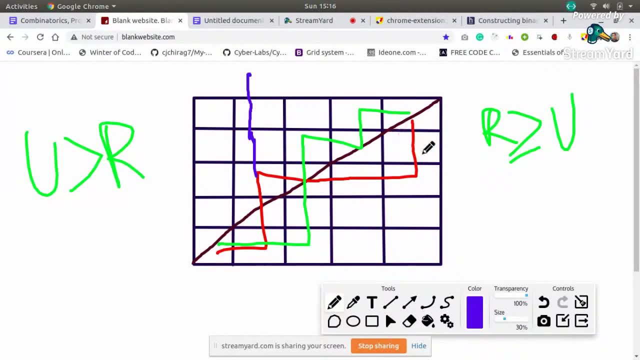 since we have one more r, since there are three r's now, so it will be again up, and after that we have two right, so it will be one right, one more right, so we reach this cell. okay, we wanted to reach n- cross and n- comma n, but we reached somewhere. 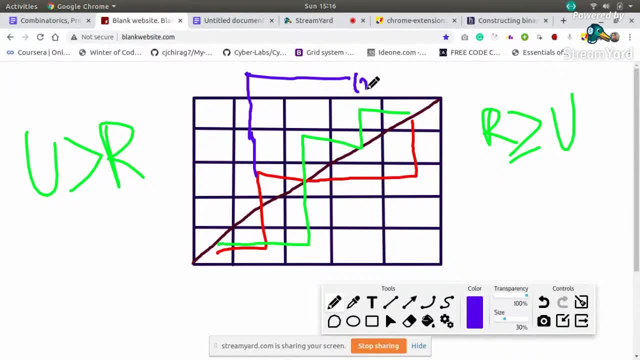 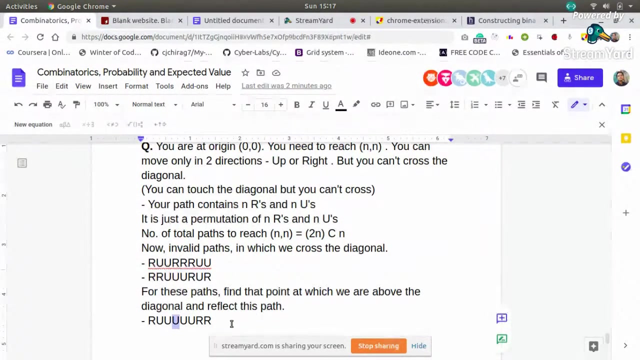 here. so the coordinates of this place are: uh, if you write it: n plus one, uh, sorry. n minus one comma, n. okay, and minus one comma, n plus one, uh, is it correct? n minus one comma, n plus one, uh, sorry, uh. i mean, i think, uh, i need to just, uh, just reverse it from this point, like: 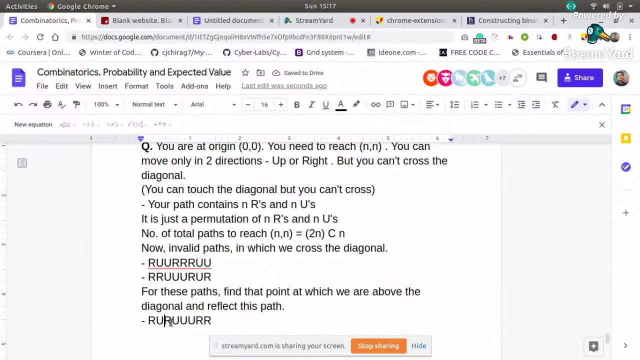 uh, if it reverses it from this point, like if we reverse it from this u, so this u should become r. so now i think it should be fine. so like this: so if you reverse it from this part, so it will become crosses the diagonal. you reverse it so it becomes something like this: it is up, so i make it right. 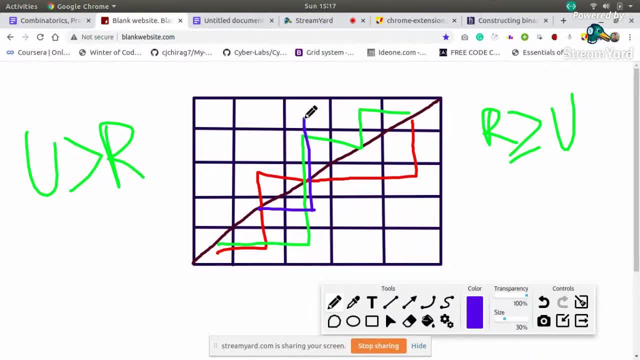 it is going right, so i go up, right up, i go it up, then in this way. so it should be, uh, like what the path is: r? u r u r triple u r r, so r? u r triple u r r, so i will reach at the same point. no, no, just give me one minute. so it should be like if i reflect it at: 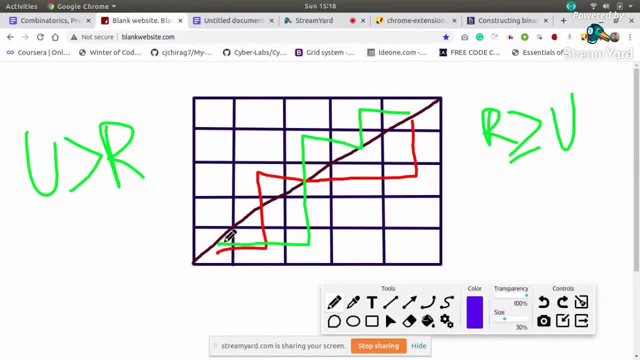 this point only, so if i reflect it here- only means something like this: so, uh, you will find that means uh, whenever you do this, you will means if you do the same thing for this part. so at what point? at what point? i'm crossing this diagonal at this point, so just from this point, i 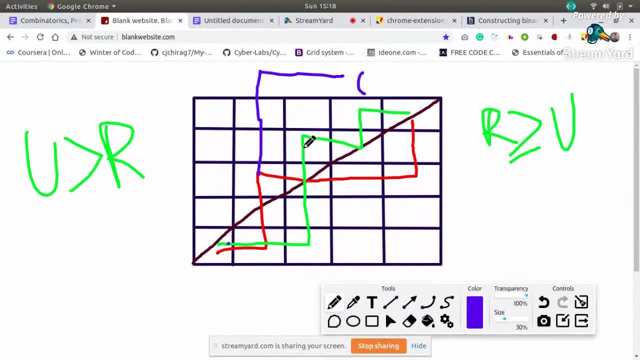 will. uh, you can say, i will just reverse all the paths. so instead of going this about the, about this place, so i will make it move. uh, i will make it move about means up to. instead of right, i will make it move above, or similarly, here also, we are going here. we are going to the right, so we are. 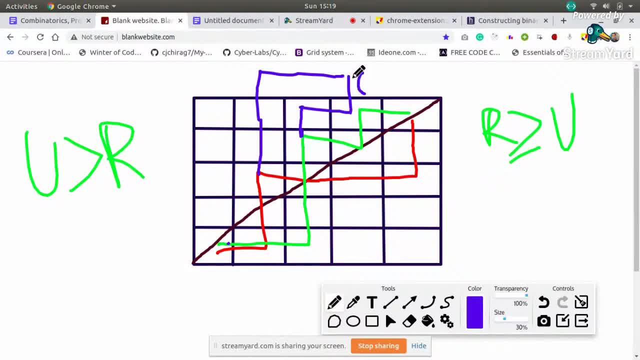 going first above, so it will be right then, about something like this: so at every point you will reach this point only means i mean to say that you greater than r reflect. reflect means r up and down, so always you will reach this point. ok, so this point will always be. 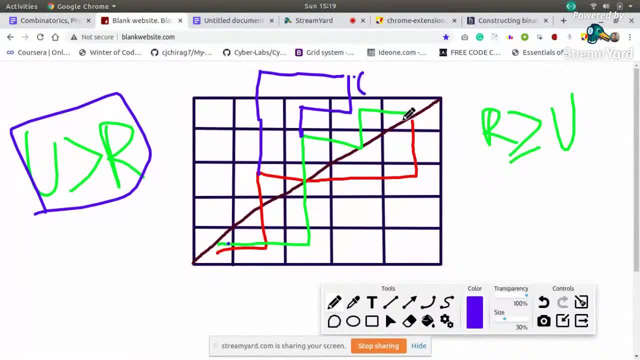 if you find it this: uh, our aim was to reach here, but we reached just uh point just, which is just above and left of this, so you will always reach this particular point. so this should be the coordinate of this should be, i think, n minus 1 comma. n minus 1. 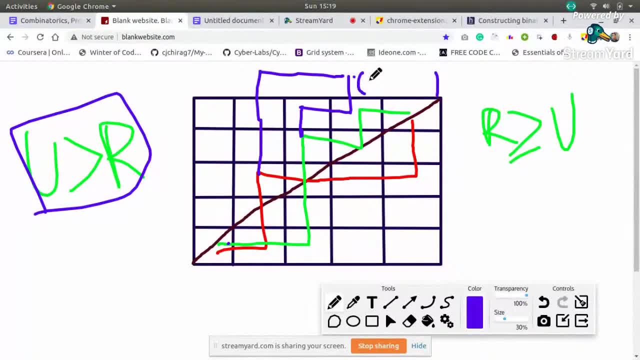 is it correct? anyone wants to say anything at that point? so you will always reach this point, so this should be the coordinate of this. so this should be the coordinate of this. and one more thing like: so uh, we will reach some point here, so it will be. let us say: n minus 1 comma, n minus 1. 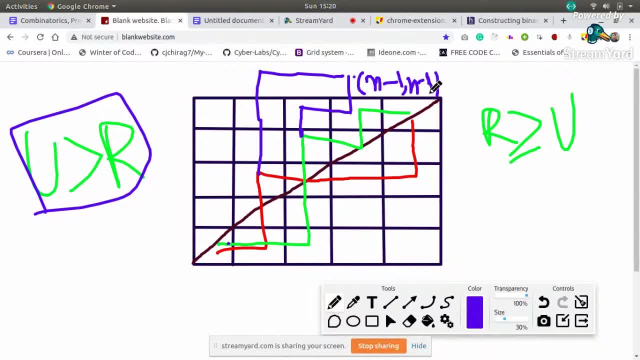 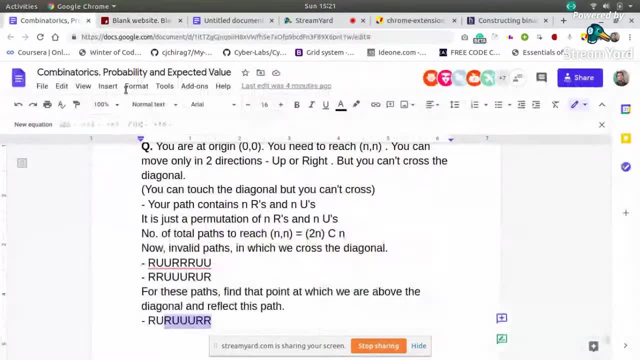 so, basically, you need to find the number of ways to reach this particular point. so i think i have done some mistake, maybe. but uh, uh, you can, uh, uh, try this thing. okay, i will uh just confirm this one. but uh means the when you will count all the you may. you may say all the. 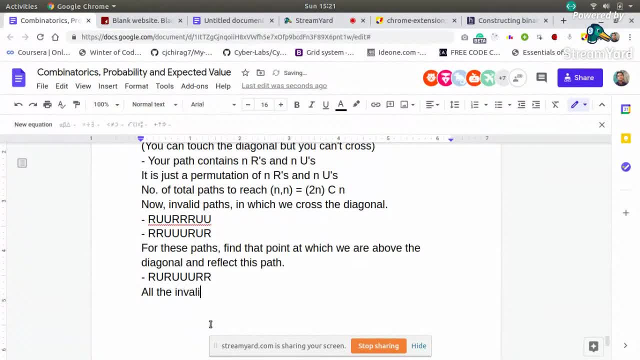 invalid parts. so all the invalid parts would be like it would be: you will get 2n, c, n plus one. you will get this way. only try to think of this key when you reflect it. whenever you get the first you, so you will reach at one point. uh, i'm not getting like. 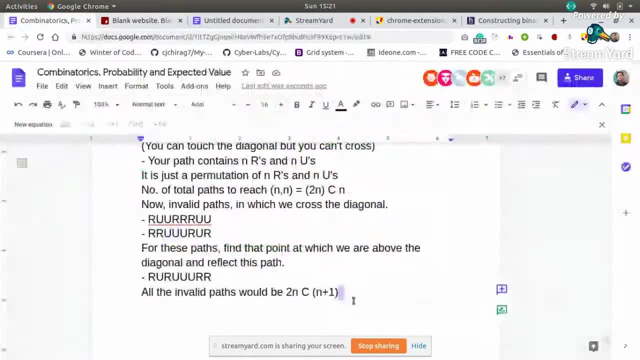 so i will try to, maybe at the last i will try to correct it so you will always get this number is 2n, c, n plus 1.. so what means these are all the? these are all the invalid parts. so the total uh means you can say total parts which. 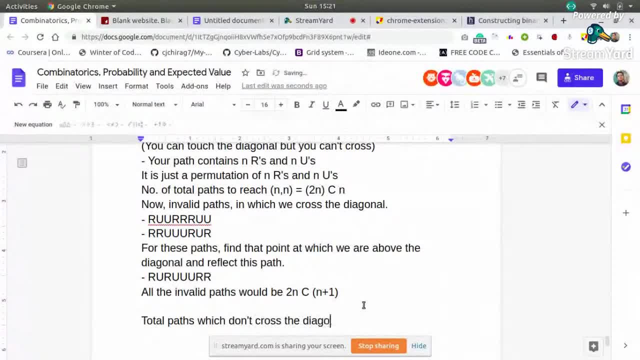 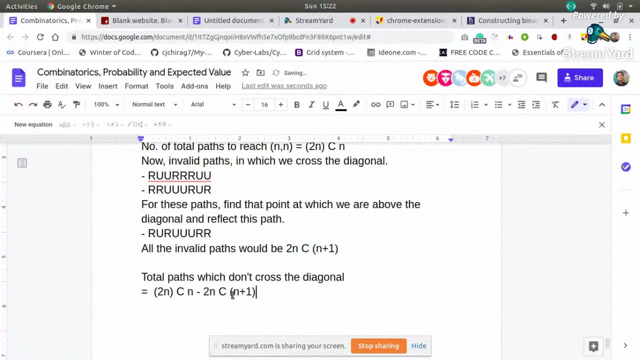 do not cross the diagonal, would be this the total pass, you know, to reach n and comma n minus the invalid part. so it will be 2n cn minus this thing, 2ncn minus 2n cn plus one. so from here you get some meets. this is, uh, some special number which is also called catalan number. 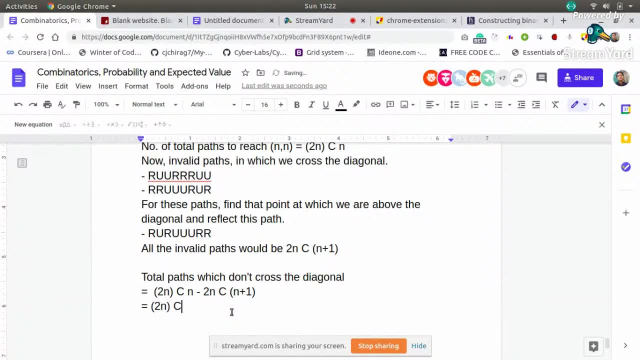 is. you can also solve it, so it becomes key two and c ones, n, n, and they will find the Nationals number cn divided by n plus 1, 2n cn divided by n plus 1.. So this is your Catala number. This is also called Catala number. 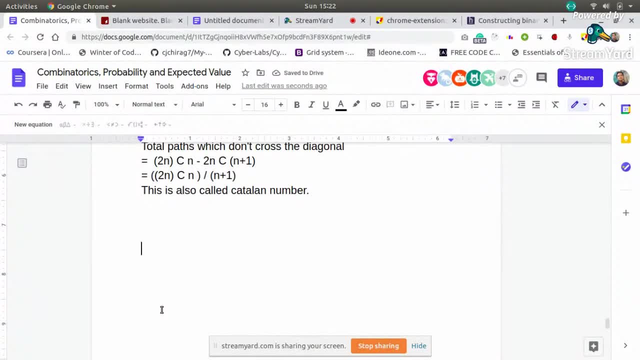 So the specialty of Catala number is that means Catala number. We can have many, many of the things Like. Catala number represents many things Like, for example, you say, the number of balanced parenthesis of a string of length 2n. 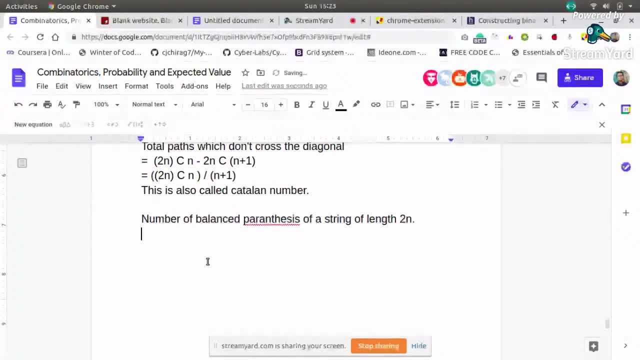 It means you have a balanced parenthesis. It means it may be like this: The opening braces should be equal to the closing braces at every point. Or it means you can say: at every prefix, you can have more left parenthesis, but you cannot have more left parenthesis. 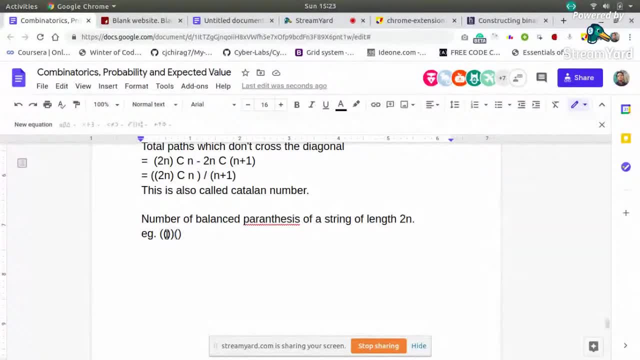 You cannot have right parenthesis. You should consider any prefix. So at any prefix you may have, if you consider a prefix of length 2, so you have more left parenthesis than the right one. There are two left but no right parenthesis. 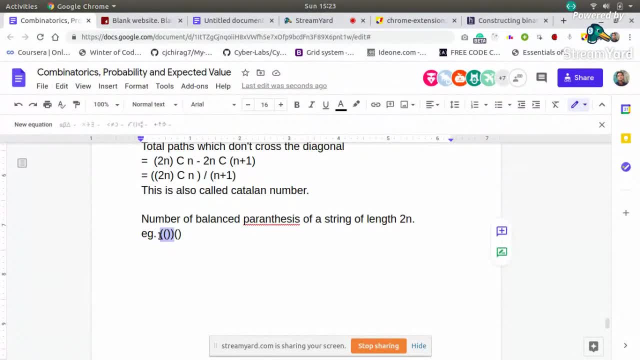 But if you consider a prefix of length 4, they are equal 0, 0.. That means 2 minus 2 is 0, so they are balanced. But you consider a prefix of length 5, you get more left parenthesis than right. 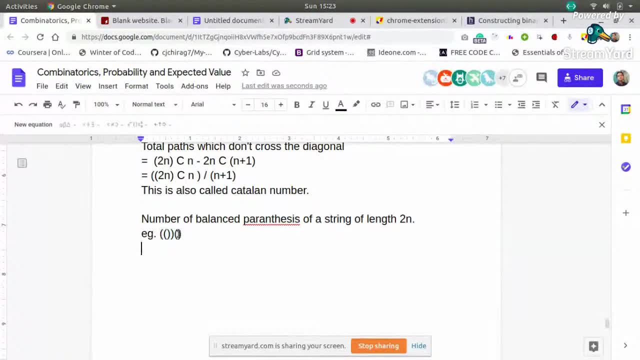 So at every point, either the left parenthesis is equal or it is greater than the right Number of right parenthesis And finally, the total. at the end, when you reach the total, number of left parenthesis should be equal to the number of right parenthesis. 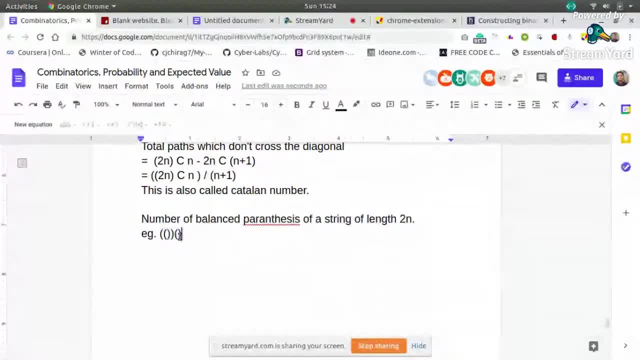 Means. it should be balanced. So such a string, the number of such strings, is also given by this number. It's same as this thing, It is also equal to this thing. So example: you can consider this one also. And if you consider this one also, there are many ways. 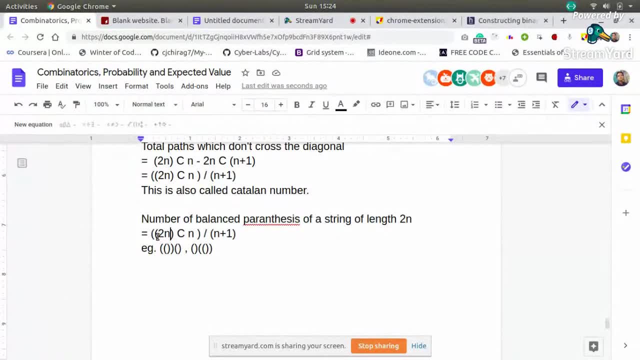 So, if you can, if you take n equal to 3, you will get. you can solve and get only that there will be 6 possible or something like that. only will be there possible balance. parenthesis for this. similarly, there are many ways which you can, many other problems in which 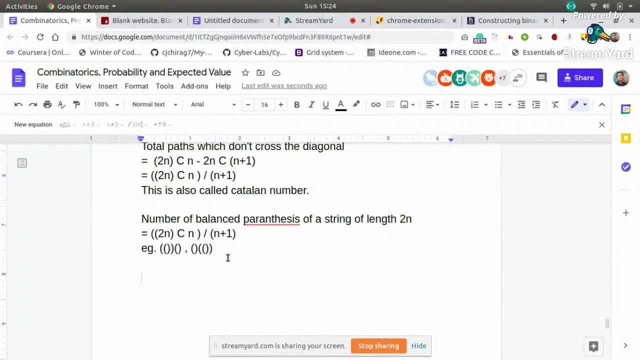 you get this. catala number is ki catala number. someone told something for every diagonal point. if we add up the ways to reach the point just above the diagonal point, then sum the total number of ways crossing the diagonal. ok, I will discuss it at the end. 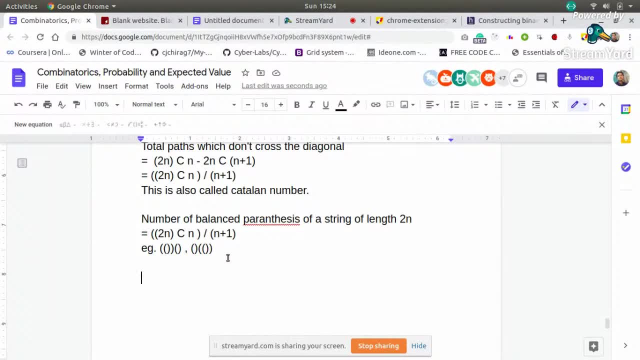 I will try to. I will try to see what mistake I made, where I will tell what the approach should be. you can consider other examples, like the number of possible binary trees of n nodes, how many binary trees of n nodes are possible. so if you try to find, 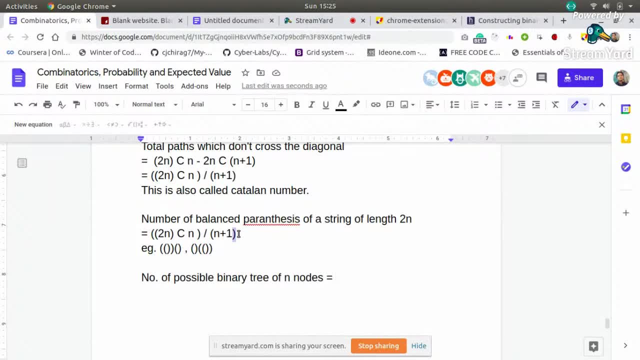 it. so it will also be equal to the catala number 2ncn by n plus 1. you can take example if you. I am not telling the proof, because proof is just based on some things like principle of mathematical induction and these things. just try to remember. 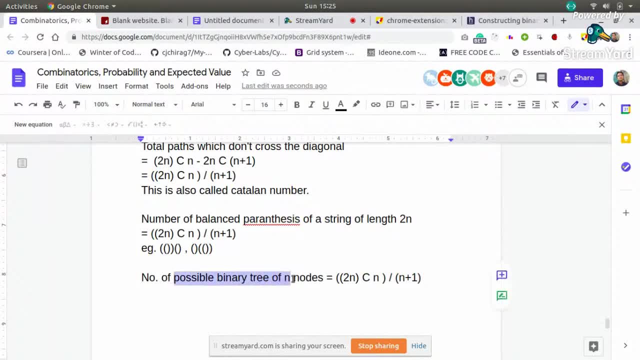 these. whenever you somewhere it is asked how many binary trees of n nodes are possible, it is without labeling number of possible structures of binary trees. if you consider the structure. I am not labeling the nodes, only I am considering the structure. so there can be such structure. I have some images for this. 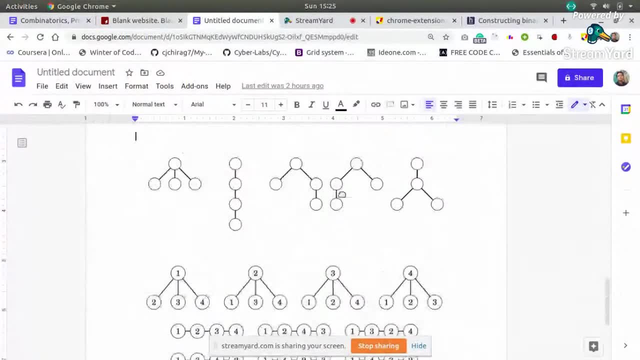 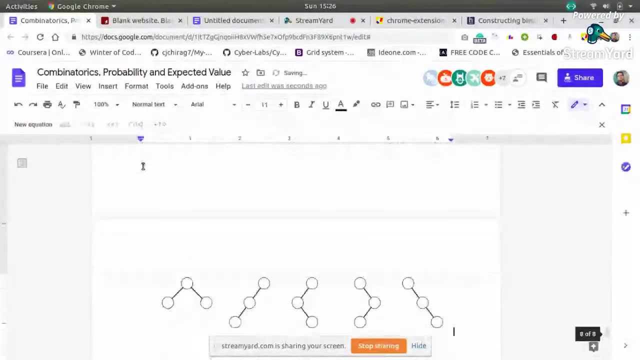 so like. if you consider the number of binary trees of length, let us say 3 of three nodes, so you will get these only possible structure for binary tree. binary means that each node can have only either 0 children or means 2 children like this, or one. children means not more than that. 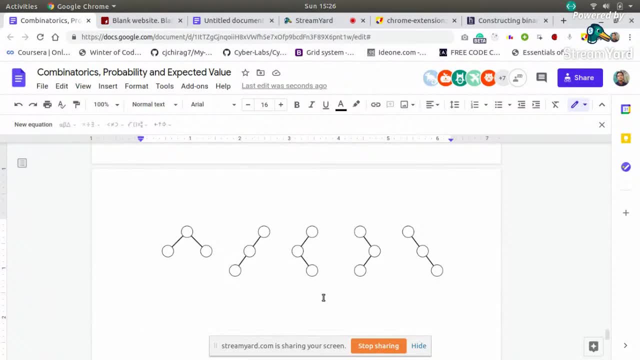 like this one is having only one child. this one is also having one child like this. so this one is having only one child. this one is also having one child like this. so So you get. only these possible structures are there And similarly, this was an example for n equal to 3.. 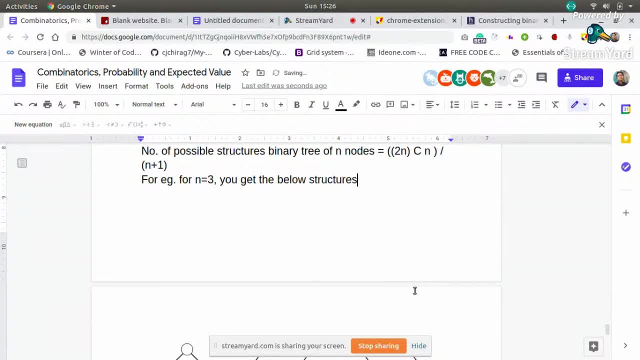 You get the below structures: If you try to draw more structure for n equal to 3, you cannot draw. All the structures that are possible will fall into one of these categories. Similarly, if someone asks you what are the possible rooted trees for n nodes, 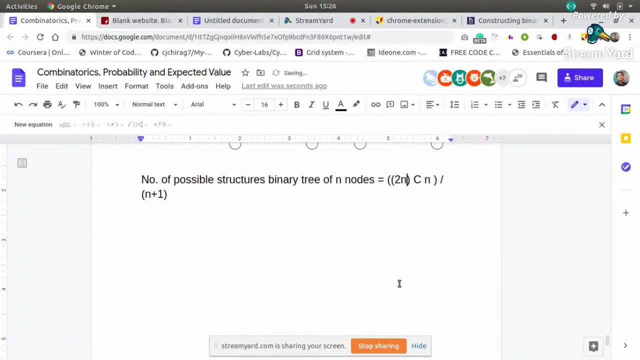 number of rooted trees for n nodes. so the possible structures of rooted trees. So it will be n minus 1th Catalan number, n minus 1 Catalan number. So nth Catalan number is this. You know, the nth Catalan number is this. 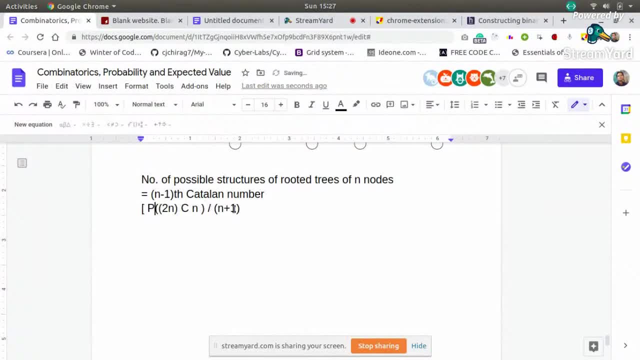 So just put n minus 1 in this equation. So I will say: put n minus 1 means or replace Wherever there is n. replace n by n minus 1 in this equation, So you will get the number of possible structures. 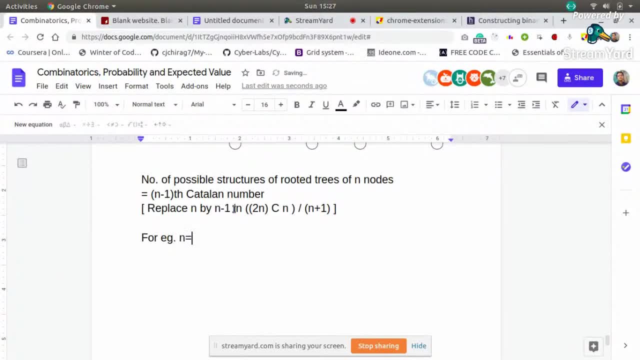 of rooted trees. So for this also, let us say we have n equal to 3.. So these will be the possible structures which you will get for any rooted tree. Rooted means it is not necessary that it is a binary tree. There will be only one root. 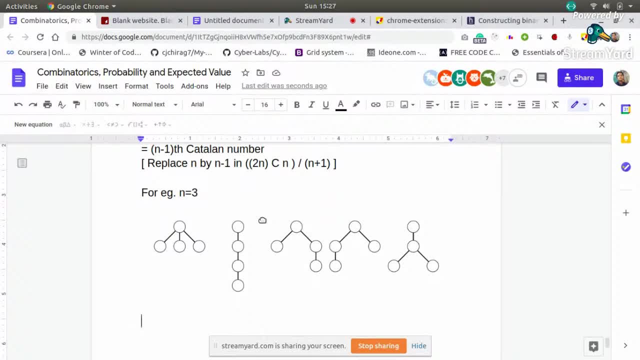 That root should be. you can say at the top or somewhere, But that root will be fixed. But there can be any number of children for one node Like this has three children. so in this way, So you will get for any n, you will get n minus 1 Catalan number. 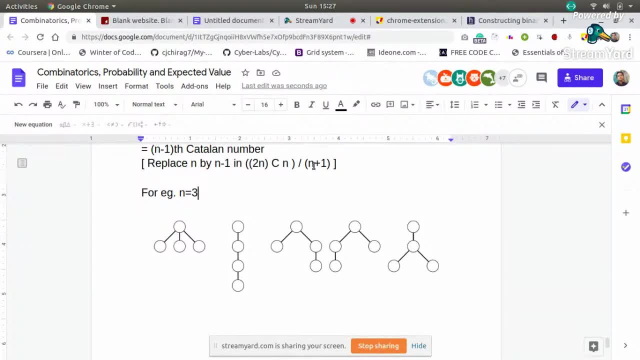 This many structures are possible for any rooted tree, And OK, so this is one thing. Apart from this, one thing is like: if you have labeled nodes, so If you have the total number of labeled trees of n nodes is n to the power, n minus 2.. 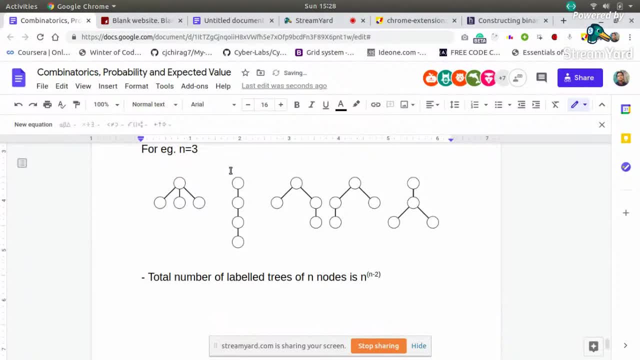 When there are n nodes. so the total number of labeled nodes is n to the power, n minus 2.. Like you have, for n equal to 4.. This was for n equal to 4.. For n equal to 4, these many possible structures are there. 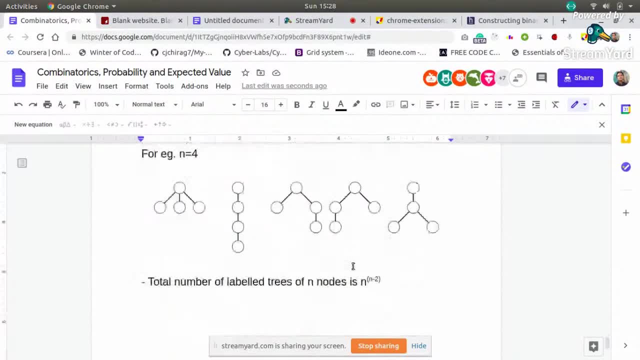 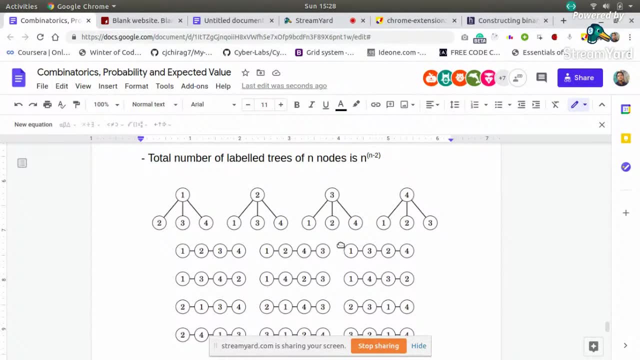 The above one was for n equal to 3.. And the example of labeled trees means that if we give all nodes a label of 1,, 2,, 3,, 4, like this, then how many total labeling, or how many total structure labeling? 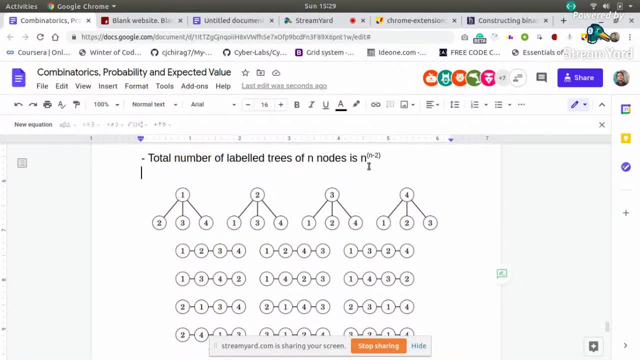 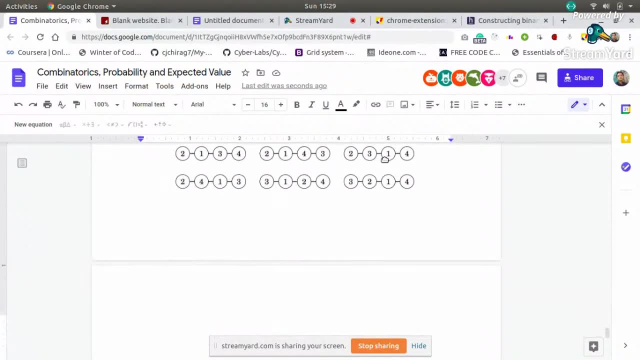 whatever you say or how many total trees are possible, So that will be n to the power, n minus 2.. Just try to remember these. Nothing else can happen. It won't be of much use, but just you should know it. 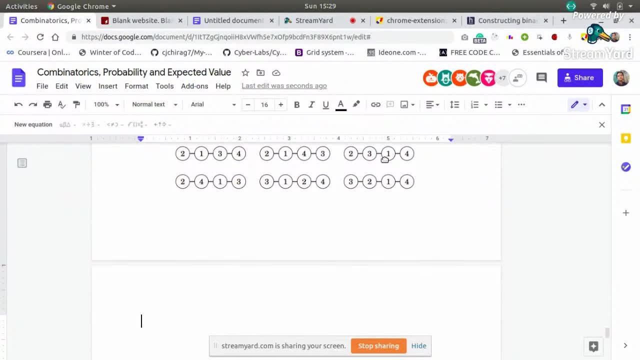 OK, now let us solve some problem. So let's look at a problem. So let us open this problem 178d. I will send the link and check So it should be 178d. OK, Let's see. Let's see. 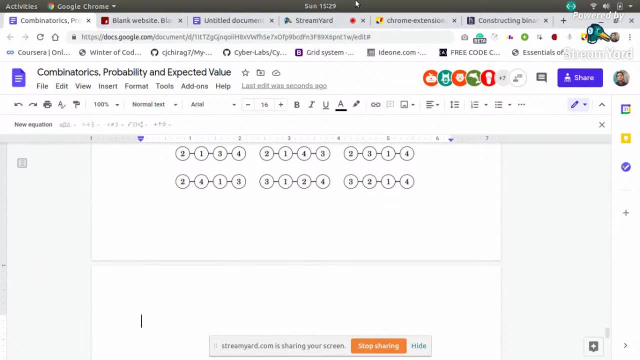 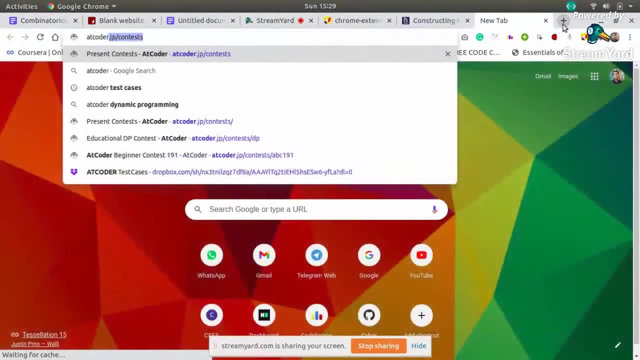 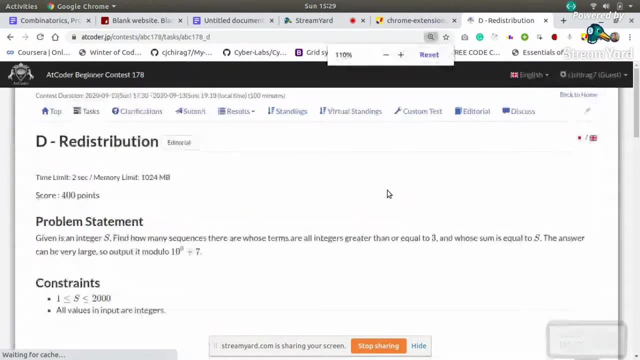 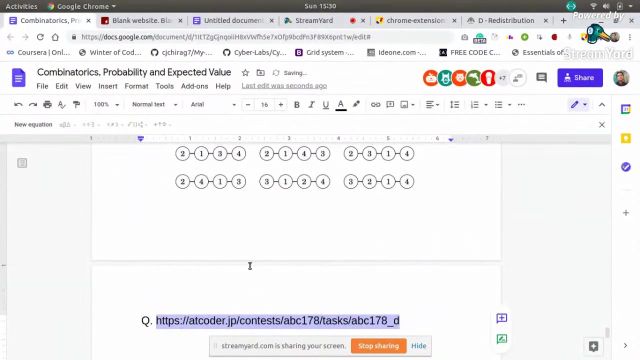 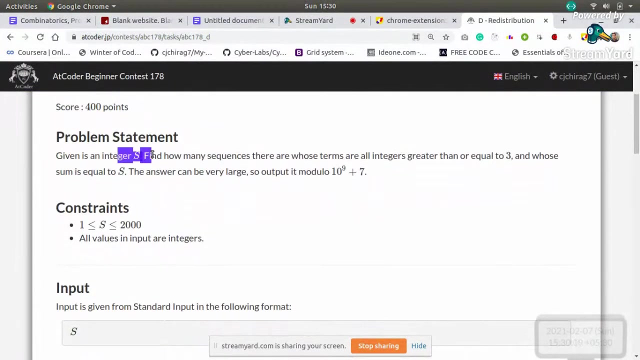 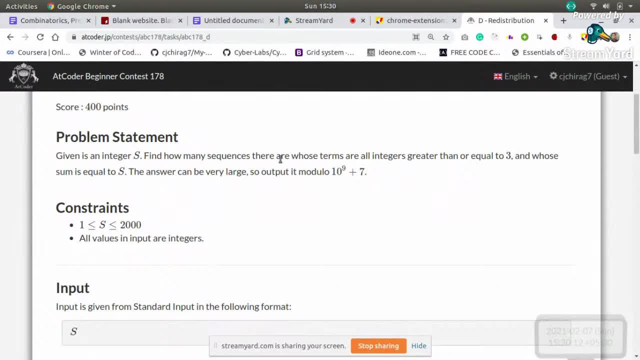 And you need to find how many sequences are there in that sequence, such that whose terms are all integers greater than or equal to 3, and whose sum is equal to s. So the sum of all integers should be s, And all the integers should be greater than or equal to 3.. 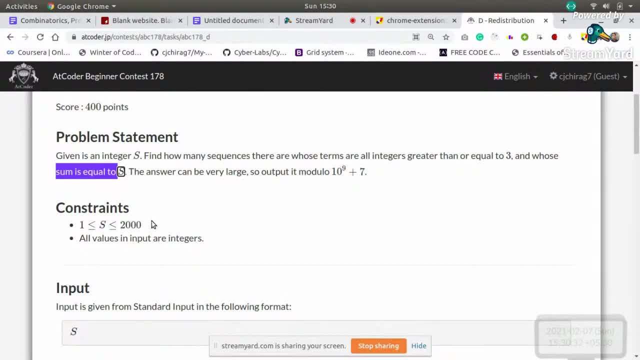 It is like this. So how many sequences are possible? And s is less than or equal to 2 to the power 3, 2,000.. And since the answer is very large, you need to output the modulo 10 to the power 9 plus 7.. 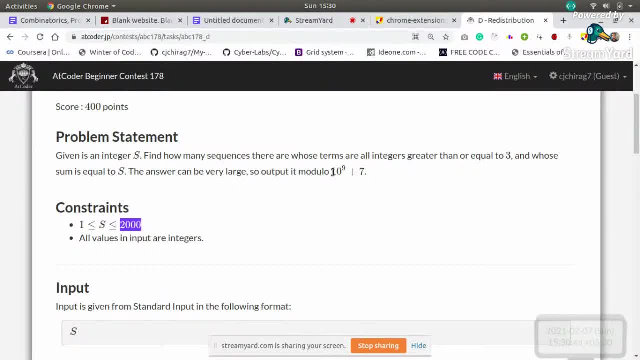 OK, OK, Good, OK, OK, Good, So try to think of any approach. OK, OK, OK, So do any. So just I will repeat the question once again. So you are given an integer s and you need 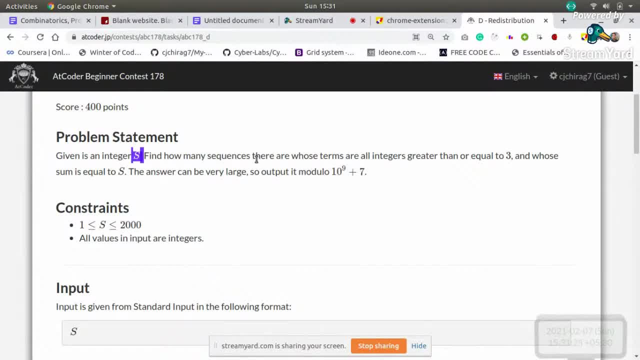 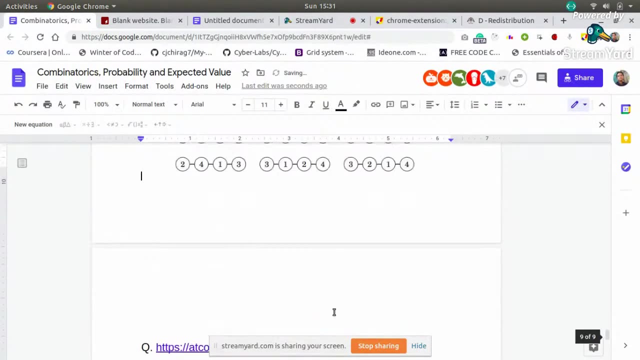 to find how many sequences are there such that in that sequence all the terms should be greater than equal to 3 and whose sum should be equal to s. Okay, so before this let us discuss one more problem, So one just general problem, like if you are given, if you need. 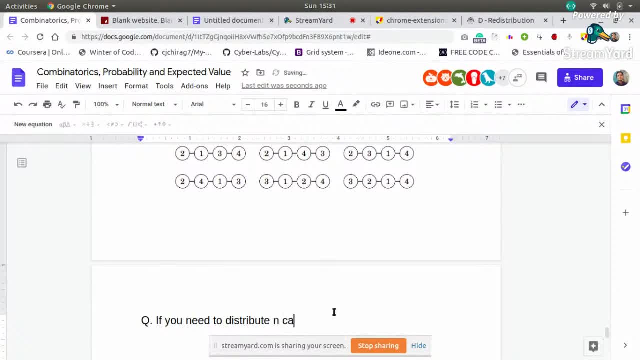 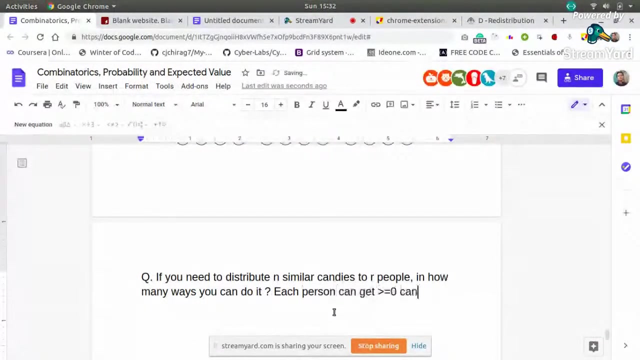 to distribute n candies. you can say n similar candies to. you can say r people in how many ways you can do it, Try to answer. or such that each person can get greater than equal to candy. greater than equal to 0 candies means you can also frame this problem as something like this in the 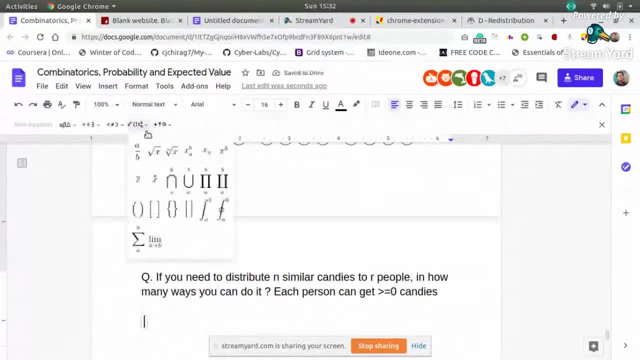 form of equation. you can write it as something like summation k equal to zero to, you can say, means k equal to 0. Now you can write that. So what you can write is that in the form of equation. you can write it as something. 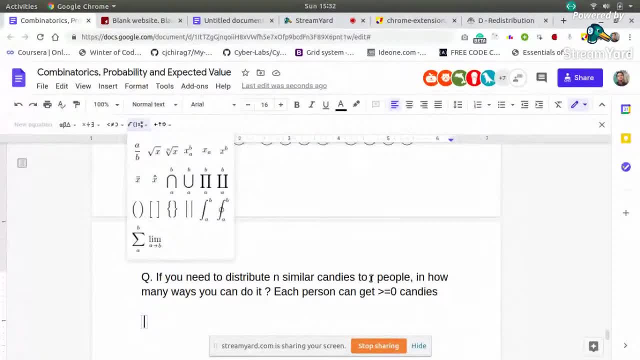 from we need to distribute to our people. so there will be, you can say, our variables a1, a2, a3, up to ar, and summation of all of them should be equal to n, so that each variable can take greater than equal to zero values. it can be written as something like: let me take from i equals to. 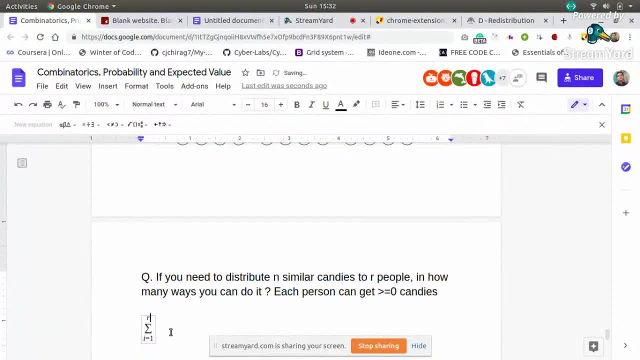 1 to r. we have something like a variable ai, the summation of which should be equal to n. and okay, let's say you are given n is less than equal to 10 to 10 to the power of 6 and k is less than equal to 10 to the power 6, k or r. so it is 10 to the power 6. 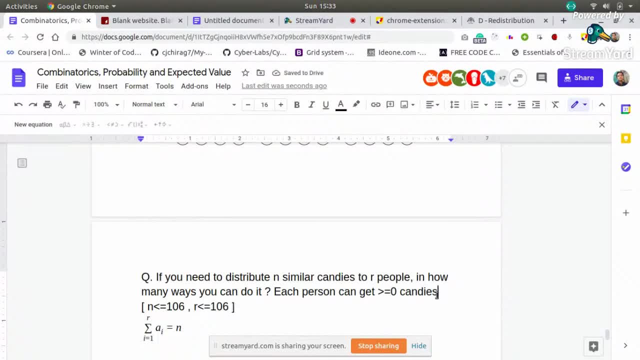 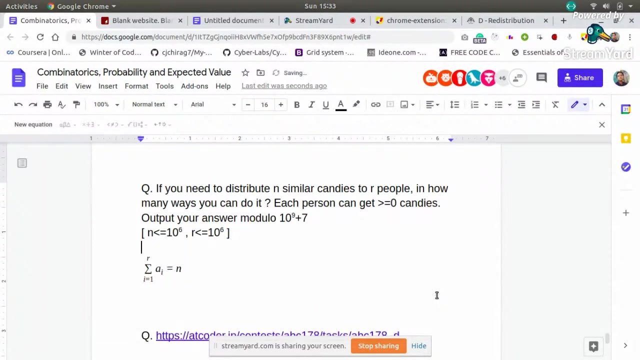 and output your answer modulo 10 to the power 9 plus 7. first try to solve this question. output your answer modulo 10 to the power 9 plus 7, so you can write this as in: in the form of equation. in the form of equation, we can write it as like this: 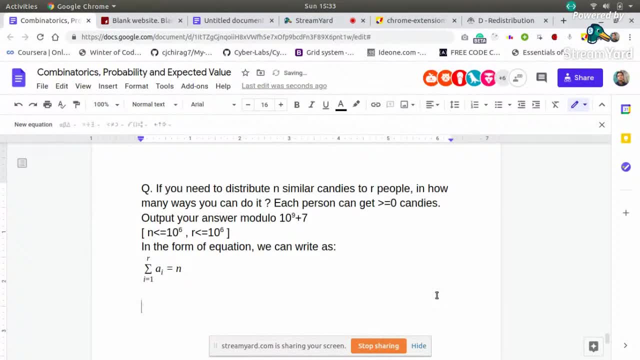 so in this thing, like if you have equation like this where you have, you can suppose it. like you have a1 plus a2 plus a3 up to ar, there are r variables and each variable can take where each ai can be greater than equal to zero. so each ai can be greater than equal to zero. 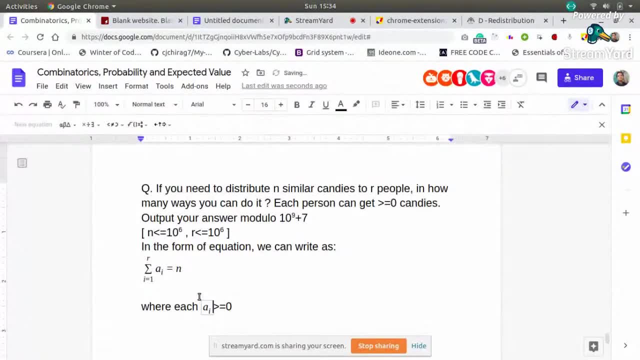 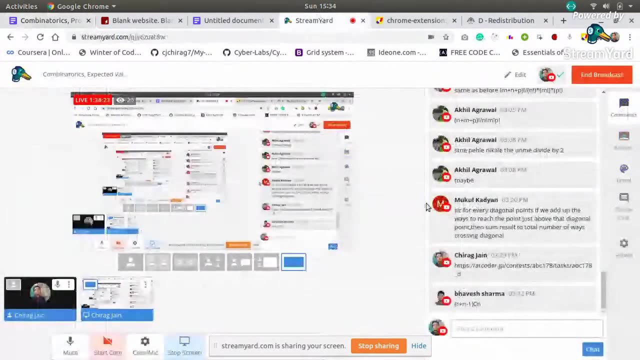 should be means you can say, should be greater than equal to zero. so one person can be there who has not got any candy and one person can be there who has got all the candy. it is also possible. so you need to find all the possible solutions. so any answer: n plus r minus r plus n minus one c n. 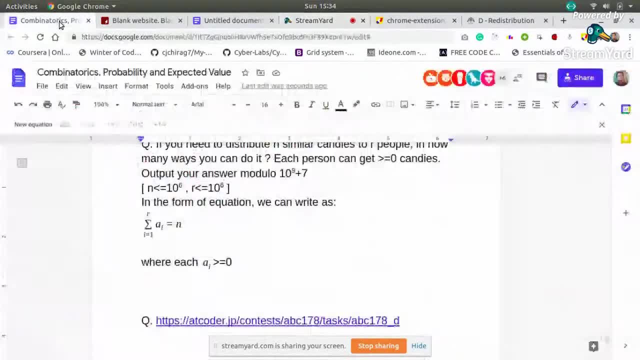 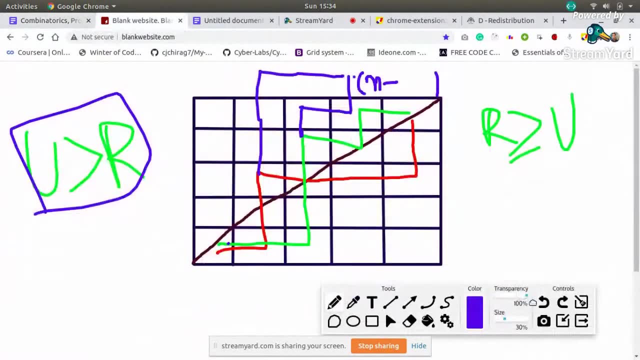 so it seems correct. so let us see how it is derived. so let us see how how it comes. so this, whenever you get such kind of problems, so uh, actually cannot erase this form, let me see. okay, so first i will draw it later i will first try to explain it. so we have, let us say, 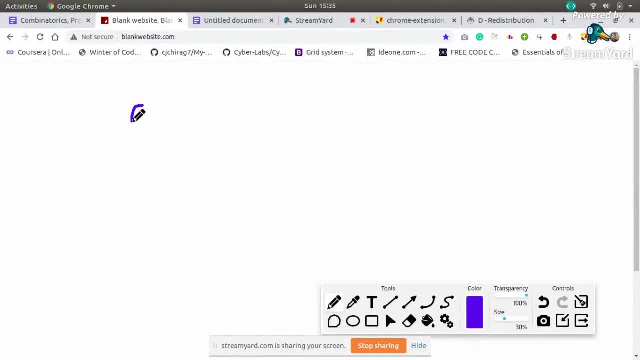 suppose we have, uh, some n candies, so i can draw candies as something like this zeros kind of thing. okay, so instead of that we can simply take something like sticks. so okay, we have some candies. so let us say something like this: so we have some candies here, now we need to distribute it to our people. so 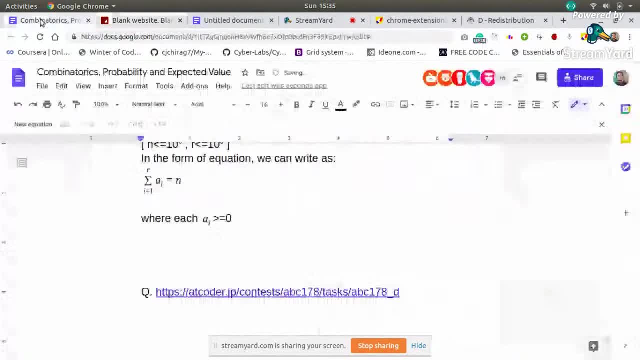 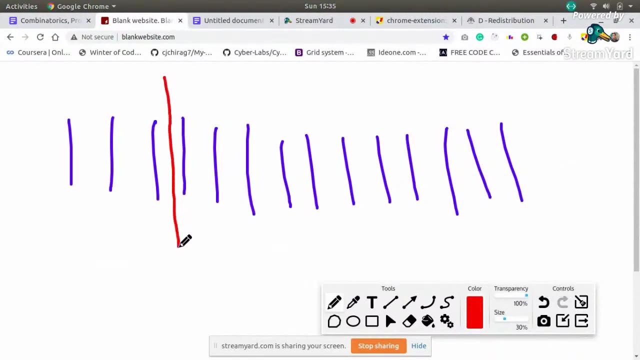 what i can do is consider r minus one sticks. so consider r minus one sticks or dividers, whatever you say. so you, i am drawing now dividers with a different color. so, like i will say, this is one divider, anywhere i can place the second divider and anywhere i can place it may. 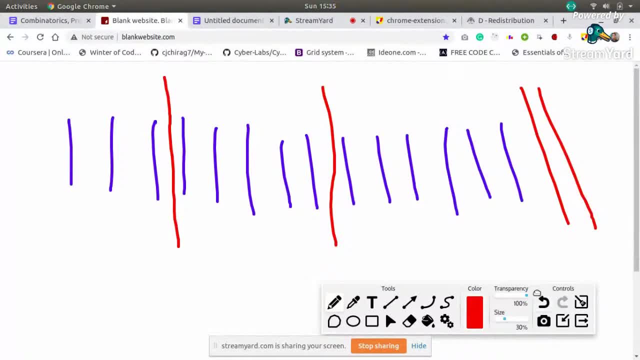 be like that. two dividers are like this also, it is possible. so just for now, suppose ki there are some. let us say: i how many sticks, i how many candies i have. three, four, five, six, seven, eight, nine, ten, eleven, twelve, thirteen, fourteen. so fourteen candies are there, the blue color ones? 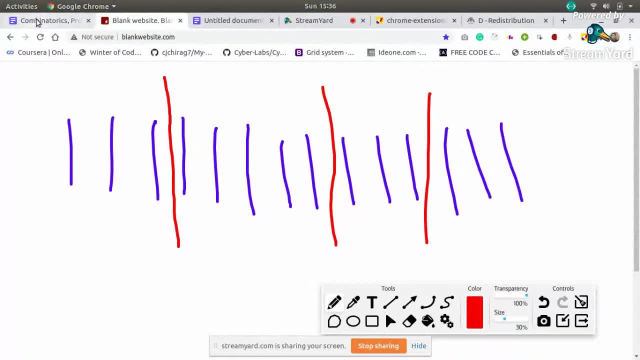 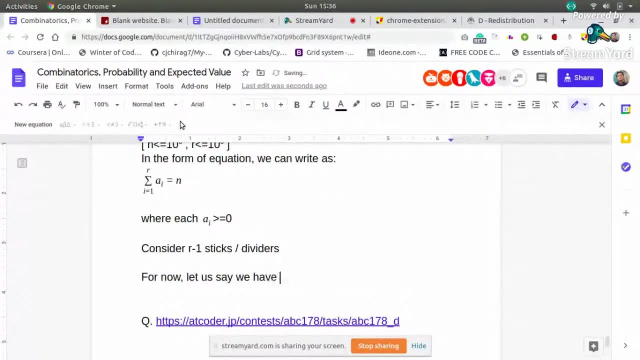 are candies, so i need to distribute among four people. four people, let us say, for now. let us say: we have how many candies? fourteen candies and we, we are distributing to four people. so what i can do is ki jitne people ek kam stick banalo. there are r people. 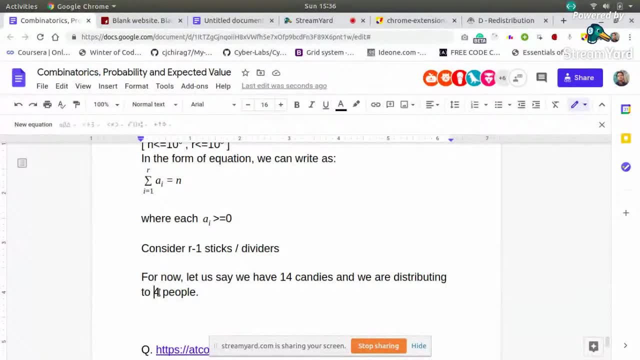 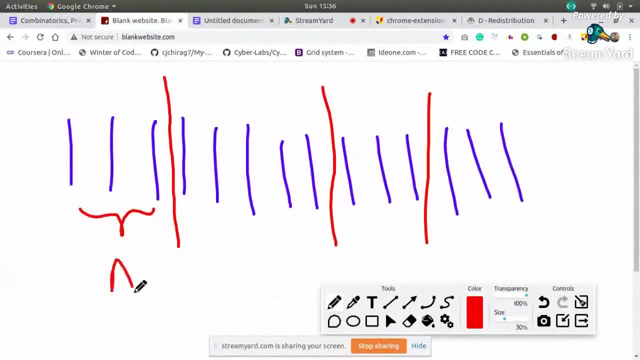 so draw r minus one stick. there are four people, so draw r minus three. four minus one. three, three sticks, so three sticks or dividers. i have drawn. so what it means ki. the person a will take this, these many candies. the person b will take these many candies, c will take these many and whatever. 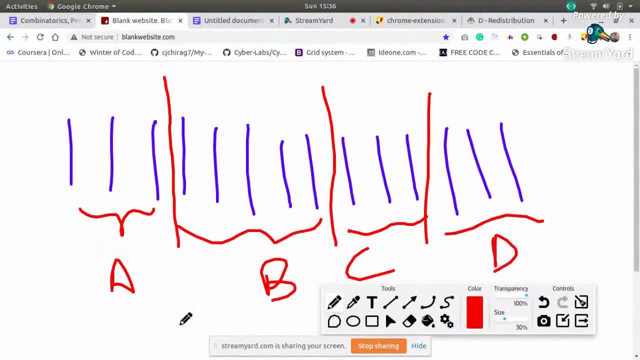 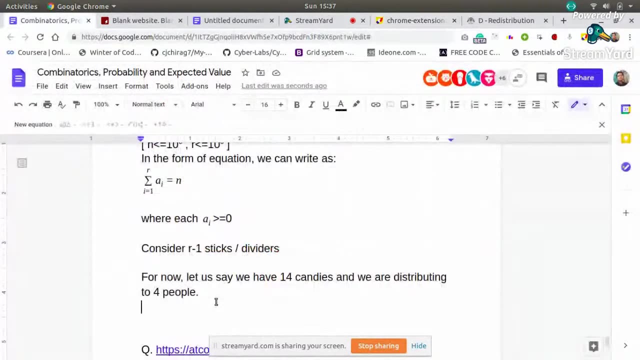 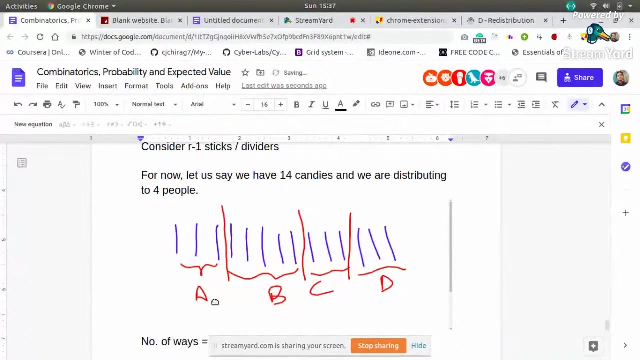 remaining the d will take. so i have drawn, since i wanted to divide among four people, a, b, c, d, so i have taken only three sticks or three dividers, so like this. so just i need to find all the permutations of these sticks and these candies, so it it can be something like this: so the total, so number of ways, is permutation. 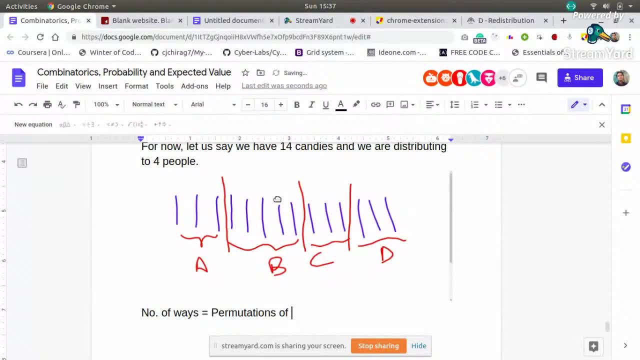 permutations of. you can say permutations of four people, so i will just write these four people: a, b, c, d. so i have taken only three sticks or three dividers, so like this. so just i need uh here if we have 14 candies and how many sticks? we have three sticks because i wanted to divide among four. 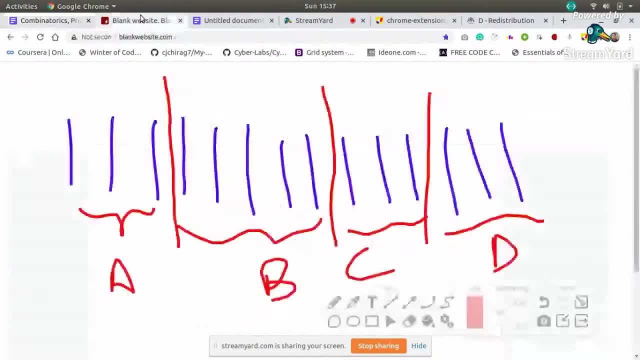 people. so i have, uh, three sticks only. so, please, i want to just permutate. it means arrange it. so what are the number of ways to arrange these? since these all candies are similar, these all sticks are similar, so the total number of objects are n plus r minus one, since n are the 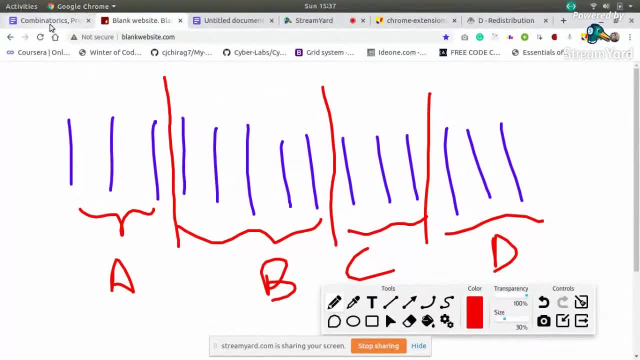 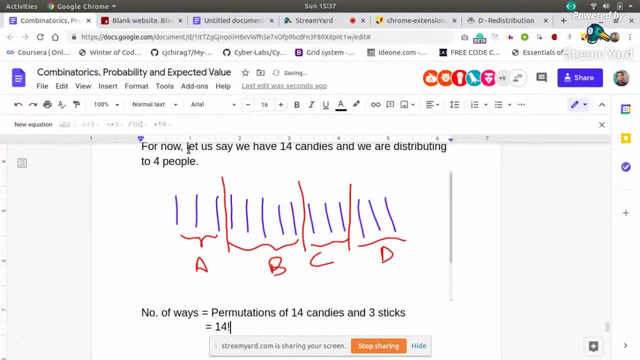 number of candies and r is r minus one is the number of sticks. so if you write in the form of uh this thing like 14 and 3, so it will be 14 factorial divide, 14 plus 3 factorial divided by 14 factorial into 3 factorial right, something like this: 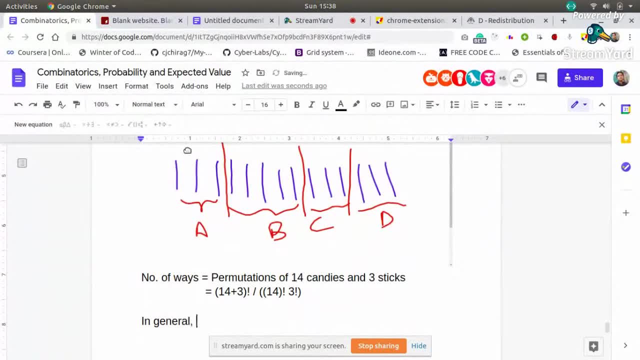 so in a generalized way. if you write in general, uh number of ways would be n plus r minus one by r minus one, because for r people we need r minus one sticks, and total objects will become n plus r minus one. so i want to just uh do its factorial divided by, since these n objects, these n candies are. 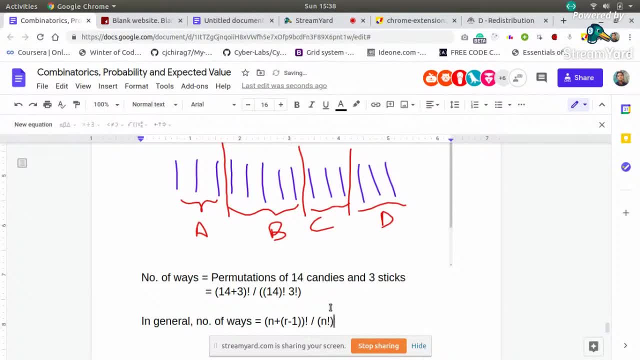 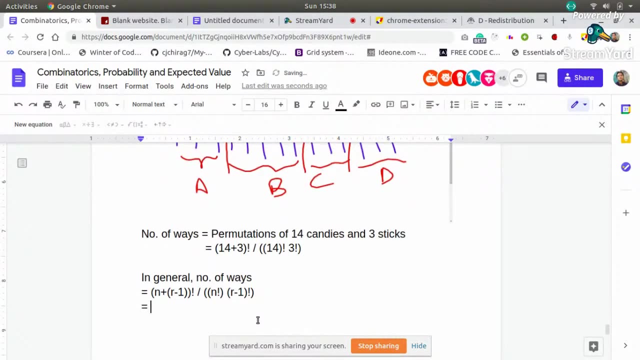 similar. so i divide by n factorial, so n factorial divided, or r minus one factorial. we divide over here like this: so we have the this as the total number of ways. fine, so you can also write the same thing as n, like he wrote. uh, you can, since by definition of combination we know that. 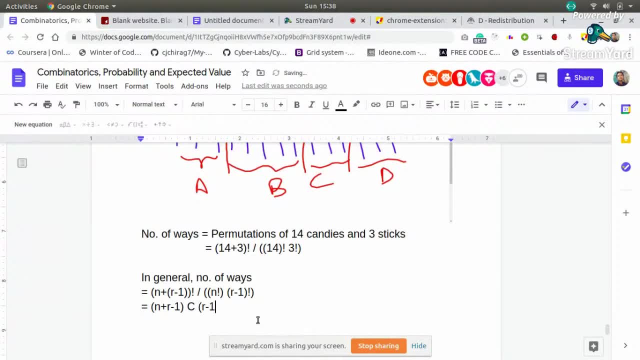 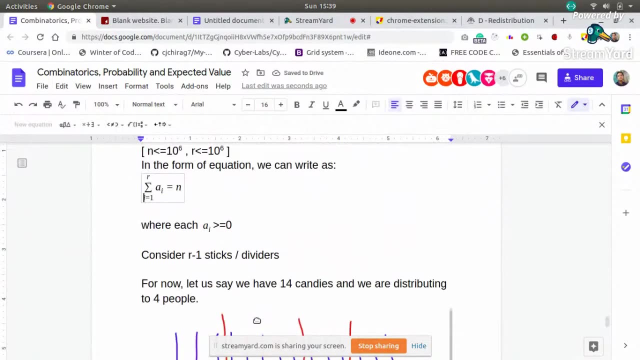 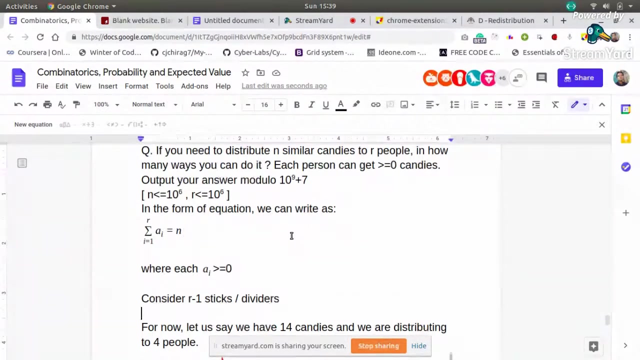 c is equal to n plus r minus one. c, r minus one. fine, so this is one thing. so this is when, when you have equation for r variables, each variable can take a value greater than equal to zero whole number. so this thing will work. so this, this general. 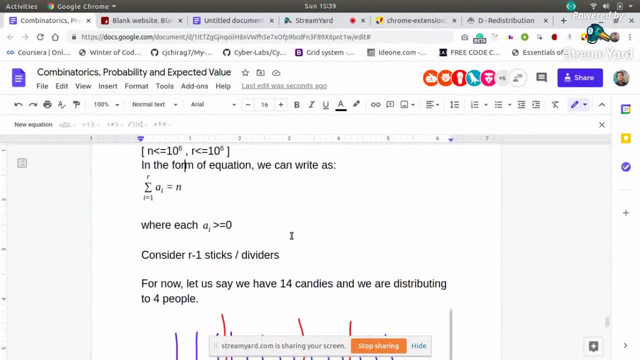 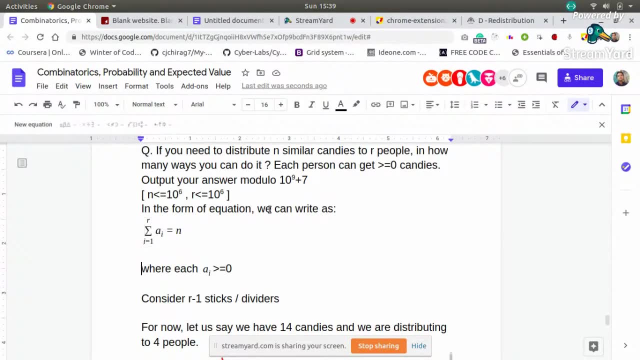 formula whenever you want to divide some values or whenever you want to, because this summation ai is equal to n means you are dividing n things or n candies among r people, so this equation is same as this. so this is, this is a general formula. you should remember it. so, if you don't know it, if you 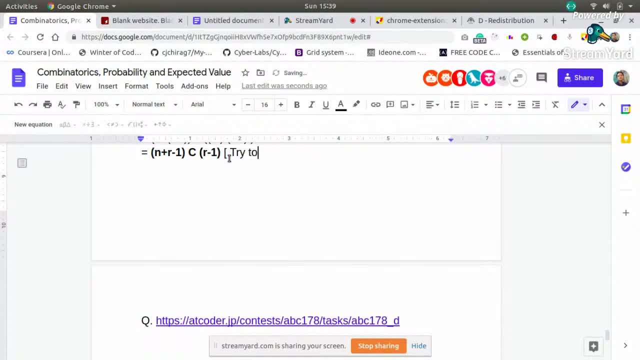 know it is good, otherwise try to remember it. it is used many times, like in. the problem which we are discussing now is in this. this means you can also solve it using dp, but if the constraints are very large, you are bound to use this formula, otherwise you will not be able to solve. so. 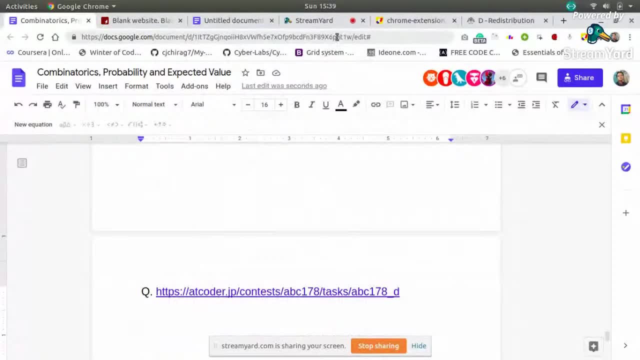 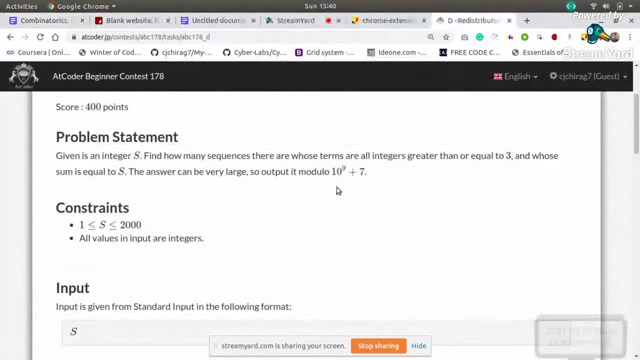 just uh, I think I would need to take, uh, 10, 15 minutes more. 15 to 20 minutes more you can means you can join that link after that. okay so, okay. so this uh this problem. I will discuss the approach. okay, I have already opened it, but if someone has any idea how to solve it, 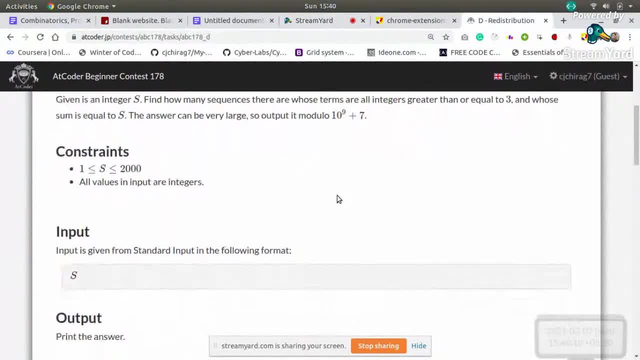 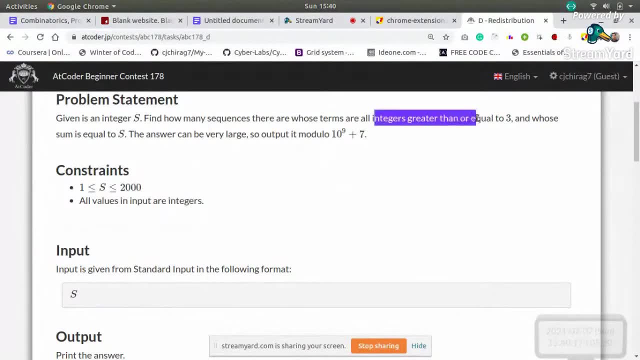 okay, he wrote so in this thing also. we are just wanting that our sum of all the numbers should be equal to s. but since all the numbers should be equal to s, all the numbers are greater than equal to 3. So you can say that if you try to reduce that thing. 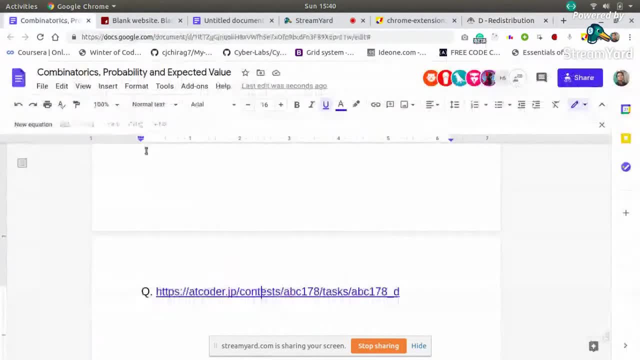 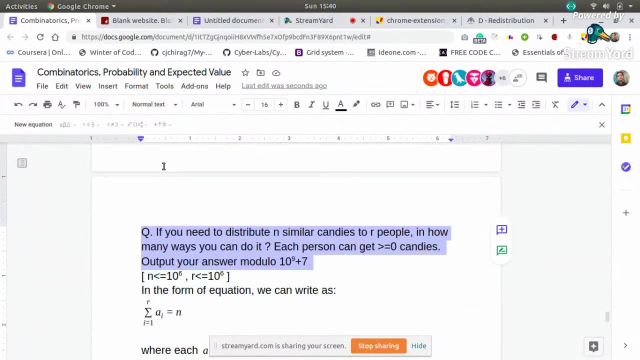 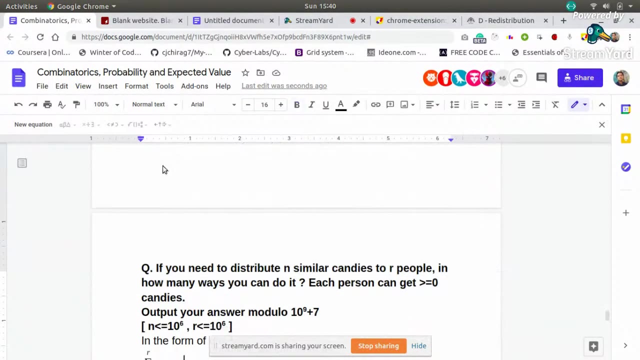 to the above formula if we change this thing in the question that. suppose you have something like this if you need to distribute n similar candies to r people. but now one constraint is there: each person can get greater than equal to, let us say, some c candies. 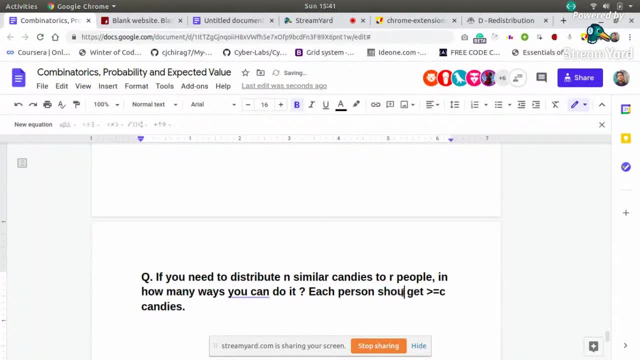 It may be anything, Each person should get. So what will be your answer Now? I have just changed one more constraint. Like earlier, any person can get 0 candies also, But now each person should get at least c candies. You can say at least c candies. 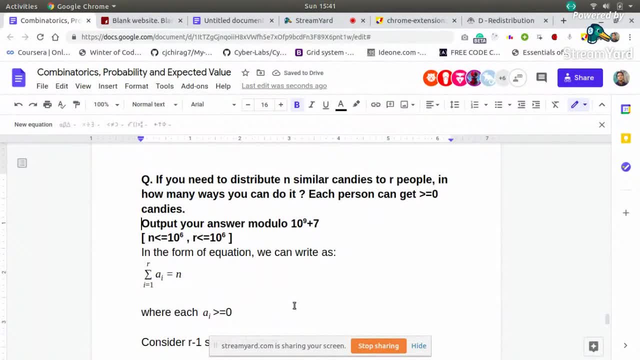 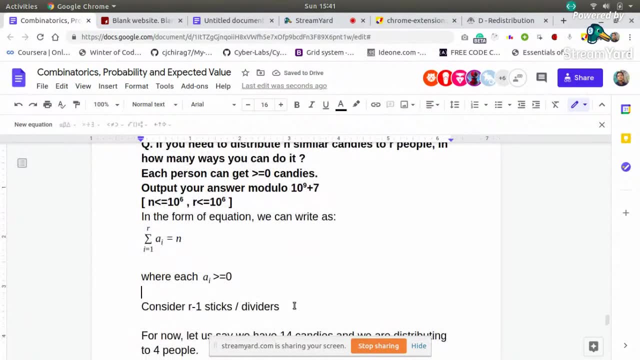 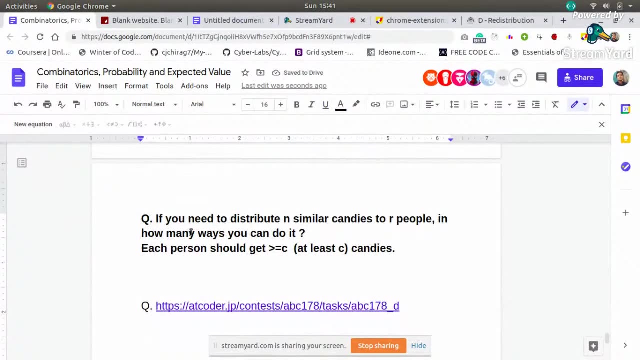 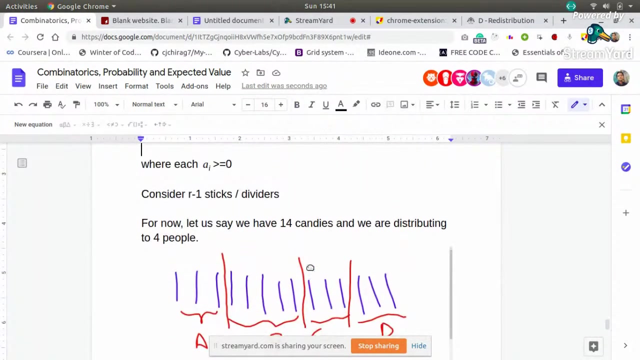 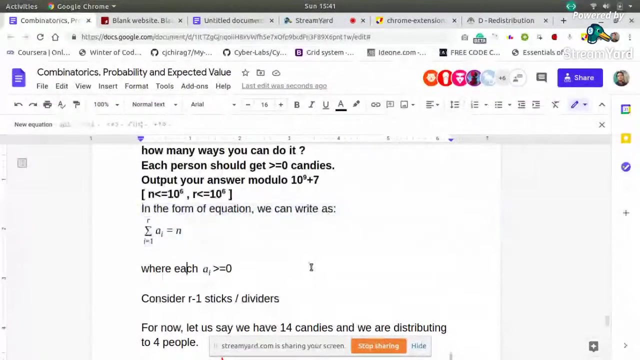 So what would be your answer? If there are n candies, you need to distribute among r people such that all the r people, each of them, get at least c candies. So if you write the above in the above equation form, so you can say that each a i is greater than equal to c, 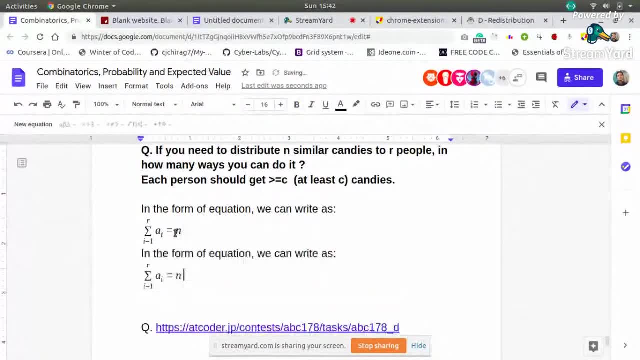 So if you write this thing, so this thing where each a i is greater than equal to c, so I replace a i. You can take some variable b i Take a. Take b i equals to Take b i equal to a i plus c. 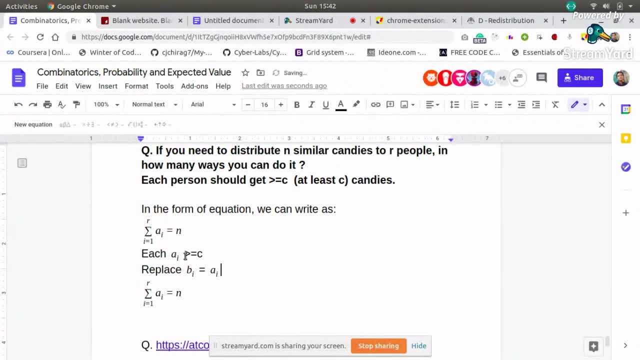 Or you can say a i minus c, So you can write that below. You have to write that. Yes, So if you replace B means this thing in the above equation. so what you get is you get a similar equation with this thing: n minus you say R into C. How I will get. 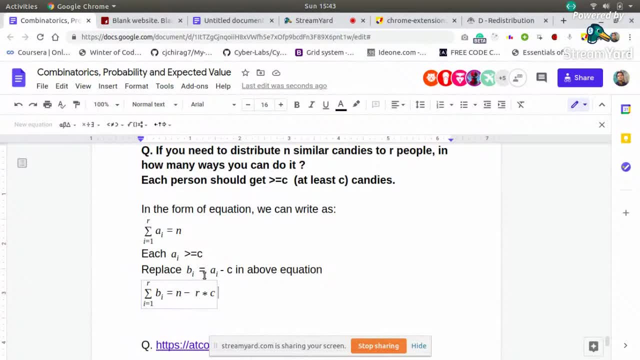 This will be something like A1 plus C. Okay, so let me see once again. So it will be. since Ai is greater than equal to C, I can write it as Ai equals to C plus Bi. Okay, So. or you can say write it like this also: 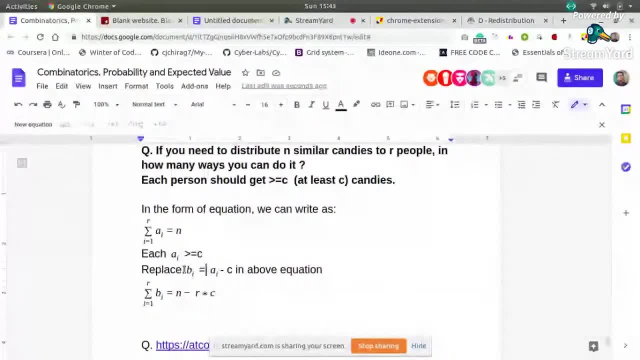 Okay, means you introduce one more variable which is Bi equal to Ai minus C, Ai minus C for every like A1, for A1 you have B1 equal to A1 minus C, So that this new variable will always be greater than equal to zero. 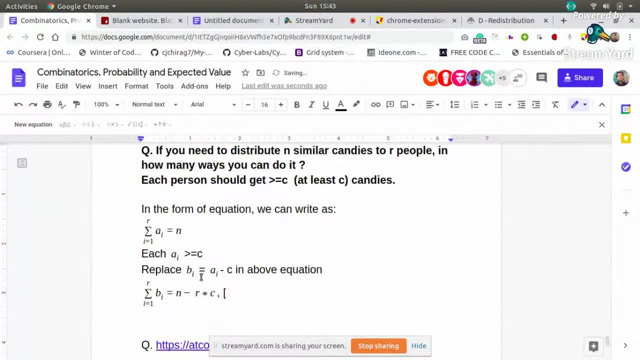 So now you have Now all. Bi should be greater than equal to zero. Bi should be greater than equal to zero for all. Okay, this thing should be there so that this summation will become equal to. if you do it, so it becomes n plus R into C, Is it right? 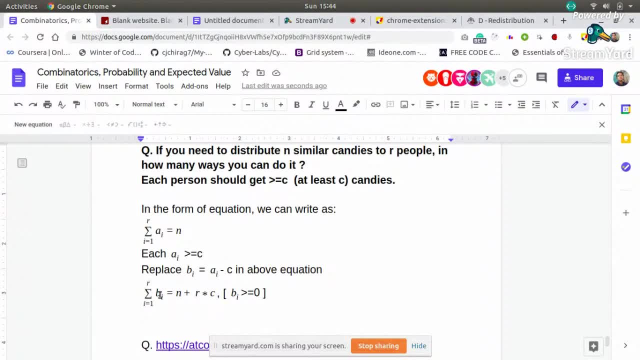 Is this thing fine, Like everyone agrees, this thing will be correct If you replace this in the above equation, because for every variable you will have R variables, A1,, A2, A3, for every variable you will have minus C term, so there will be. 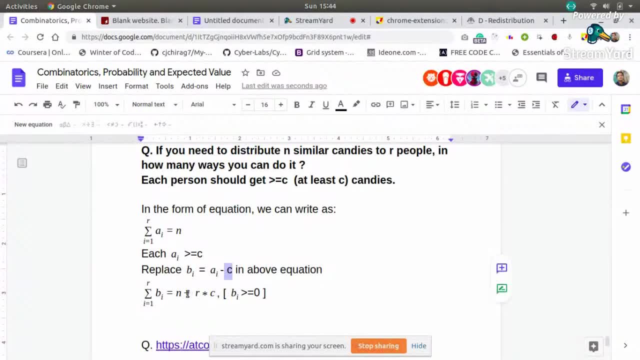 total minus R into C. So if you take it to the RHS you will get plus R into C. So this thing you will get. So the number of ways would be then this thing. just we have derived it whenever this variable is greater than equal to zero, these are whole numbers greater than equal. 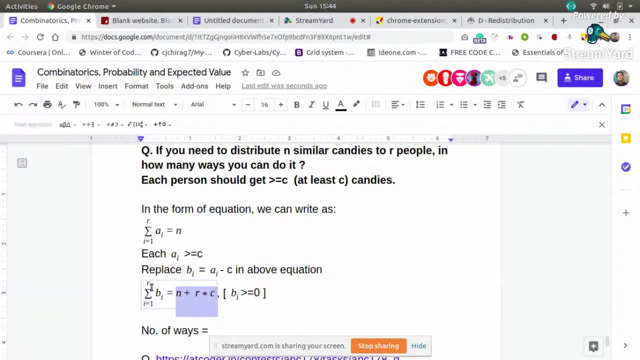 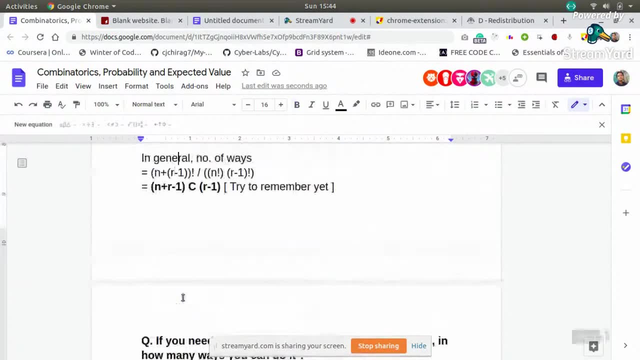 to zero And we need to distribute some number of candies among these R people. so you know that nCr minus one, nCr minus one, Something like this. So you just replace this thing in the above formula, So you will get. what you will get is okay. what you will get is, instead of n, you write: 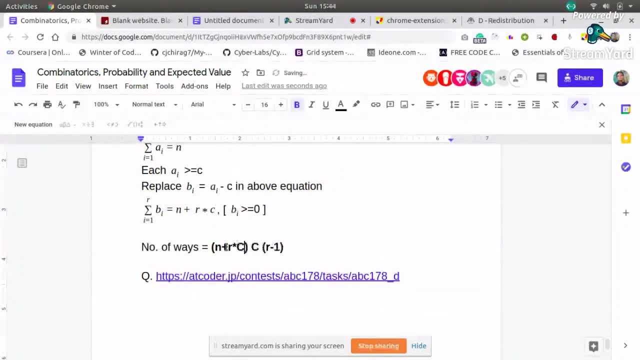 n plus R into C, this thing n into R, R into C, plus R minus one, C R minus one, because we need to distribute among R people only. But the sum has changed. We need to distribute now these many candies. 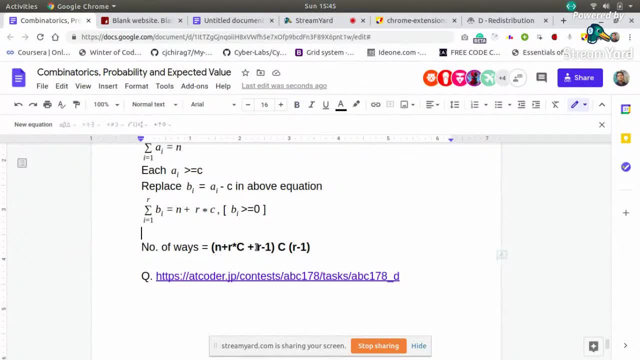 So it is something like this: n plus R into C plus R minus one. Take it. So the formula will be something like this: So is it fine? Now, if you know these two things, I feel it is correct in this, or it should be something. 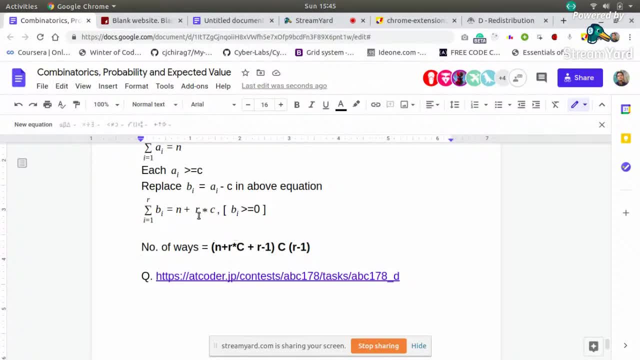 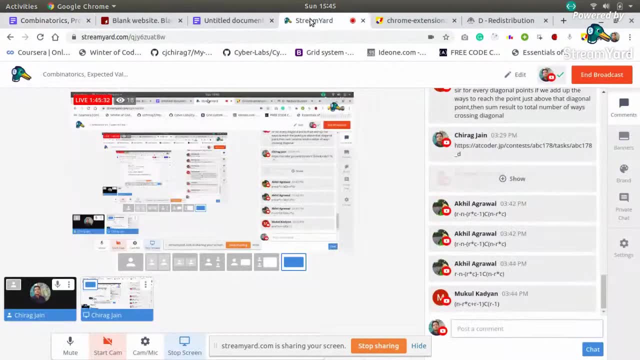 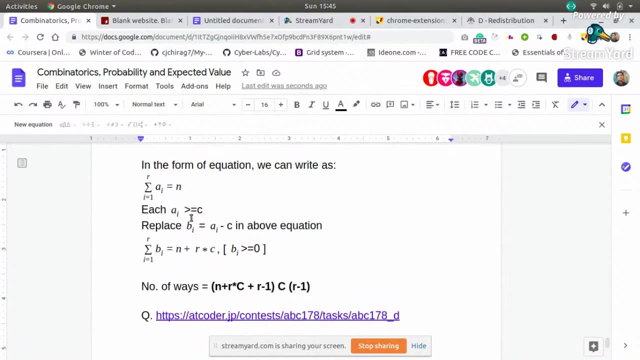 else, I think it should be subtracted, Okay, Okay. Okay, Okay, Is it correct? I feel it. I have done some mistake. like Ai should be greater than or equal to C, Each Ai should get at least C values- C candies. 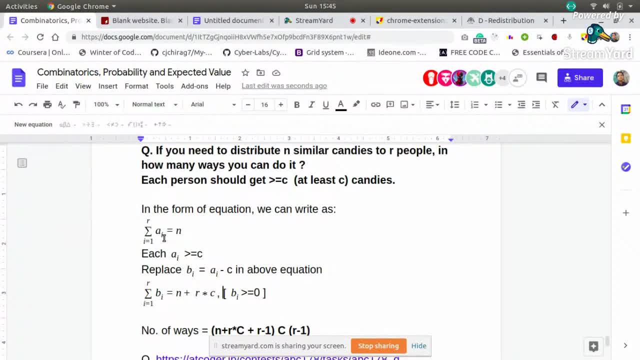 So if we do Bi, equal to Ai minus Ci, Ai minus C. okay, okay, so this thing will be. it should be minus because you will, you will do something like this: Okay, Okay. So if you will do the same thing, then it should be. it should be equal to, I think, Ai. 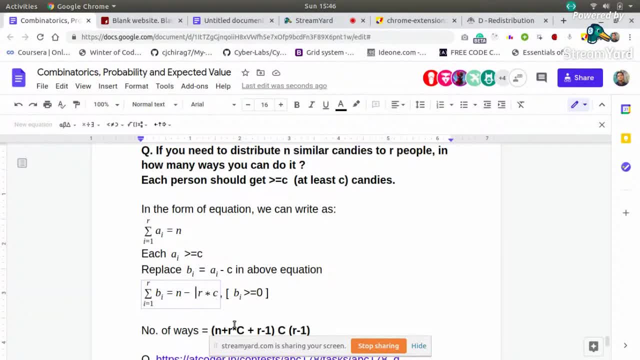 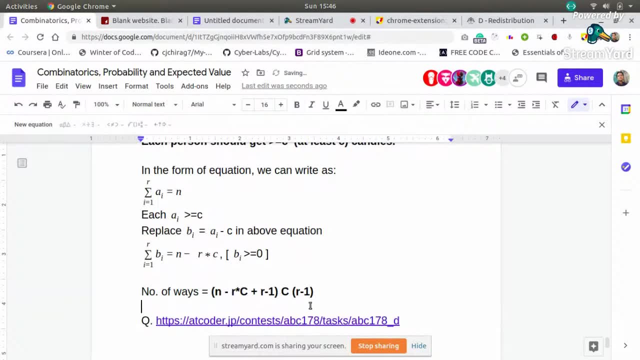 will be equal to Bi plus C. So when it will go to that side it will become minus. so sorry for this. So it should be minus sign here. Yes, Now it should be fine. N minus R into C plus R minus one. 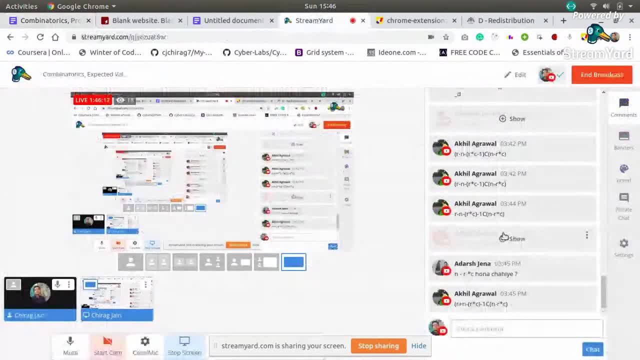 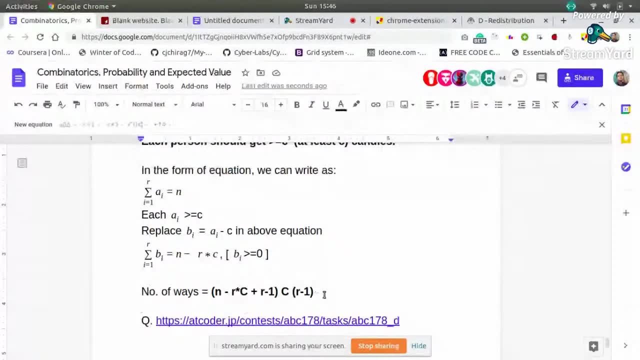 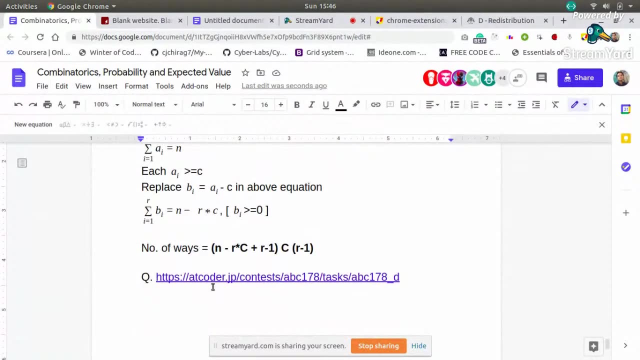 Is it correct? Take it Now, it should be fine. Now is it correct? This thing should be your answer Now for this question. what we need to do? Just, we need to just make the sum equal to the given sum s and we, we have. we have, we do not know the. 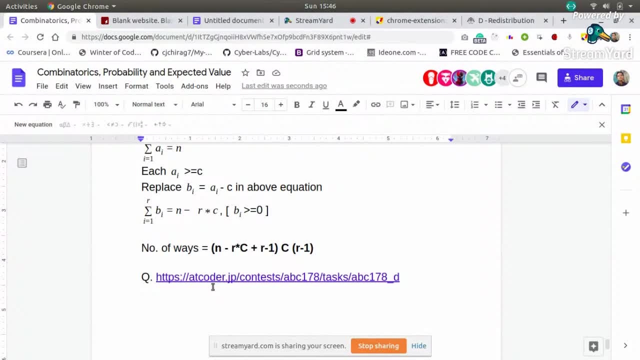 length of the sequence so we can just run a loop. so it can be something like for each value of the length you can run a loop for, let us say, for length equal to, because you do not know the length of the sequence. so it is in the question. it is not mentioned of anything about, about the 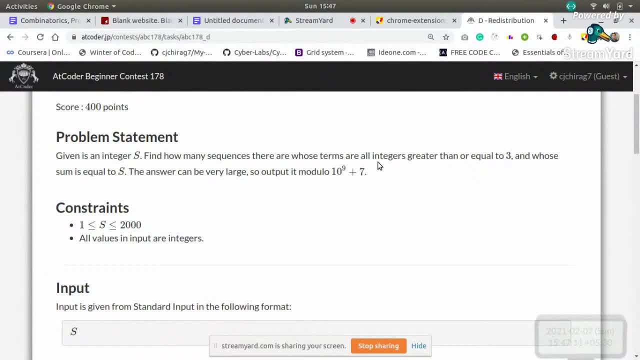 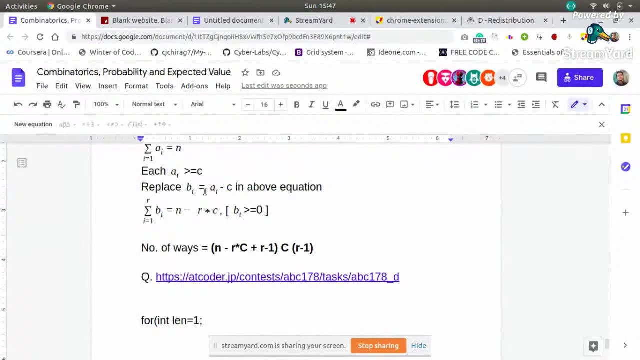 length, but it has written key: how many sequences are there, such that all interiors are greater than equal to three and whose sum is equal to s. so for each length we can find how many means, how many sequences are there and we can sum it up. so this will be something like: for each length you will 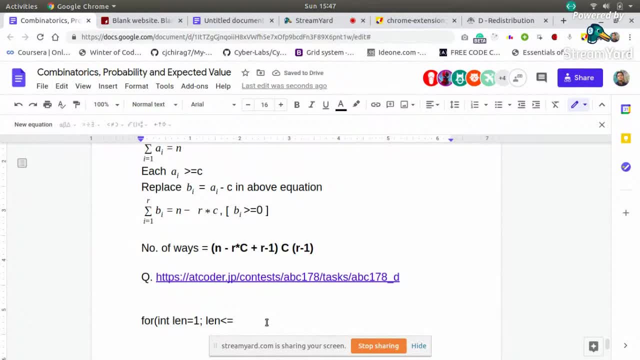 go then? and what way? what can be the maximum length, since your each variable can be at least three, so in the worst case all will be three, something like that. so you will get length maximum length as s by three, so s by three will be the maximum length. 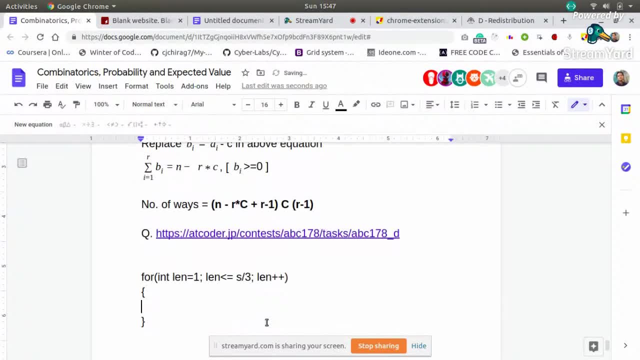 and length plus plus, and for each length you do: uh, what your sum would be. some would be means uh, some would be s only. but this sum, this thing would be, means which. or you can say directly, you can also write this formula, also you can directly use. so 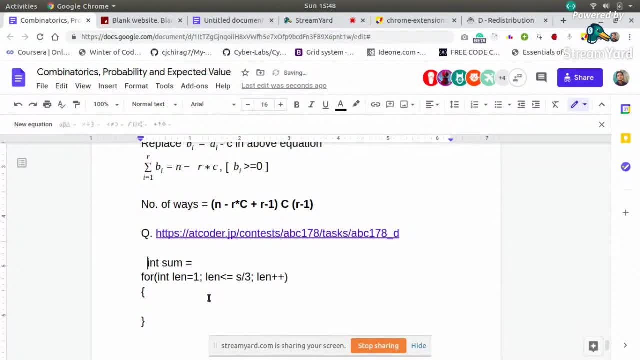 let us say we have total number of. let us say we declare a variable answer here into answer equal to zero. and just for every length you sum up the answer: answer plus equals to answer, plus equals to ncr of this thing. so what is n here? n is the total number of total sum. so the sum is s here. 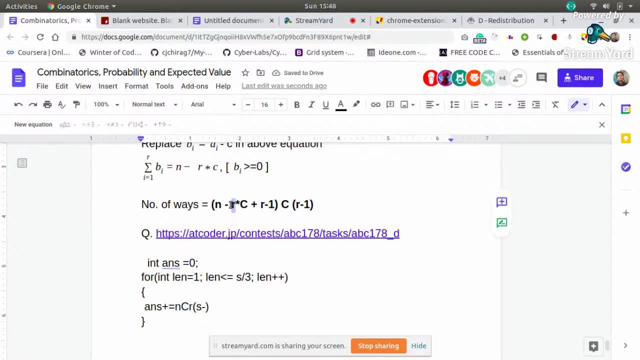 s minus the length is since this r. this r is the length. how many variables are there, or how many people are there whom whom we want to distribute among? so this will be uh the length, or uh a length is constant c. this c will be. since we have taken uh, at least each person should get at least c candy. 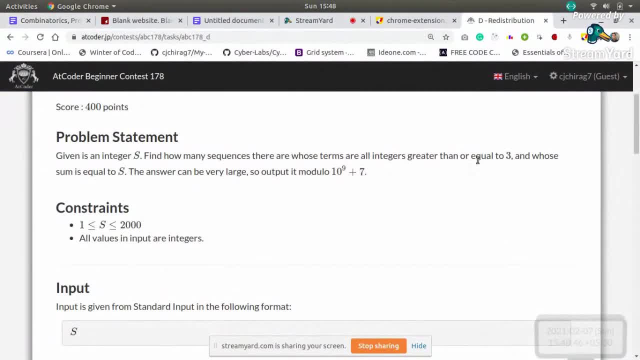 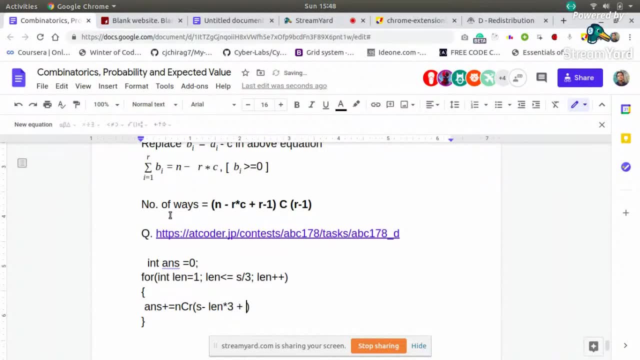 so here each person should get at least value of 3. so here c equal to 3. so replace 3 by 3 here length into 3, uh plus you get r minus 1. r minus 1 people means uh. since here length is l, uh, this len so. 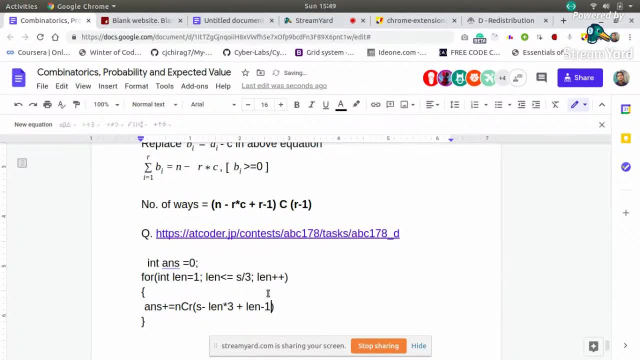 this will be the number of people. so this is r r minus 1, something like this, or your: uh, this r minus 1, it will be l? n minus 1, because you want to distribute among this length number of people. so it should give you the answer for every length. you will sum this up: 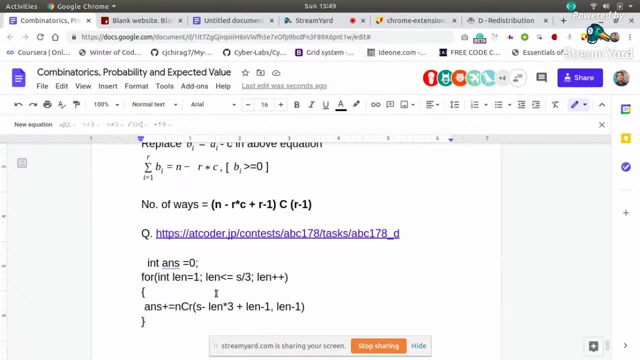 okay, so this thing you will get it directly. or one case can be when, uh, if this sum you are getting is less than zero, so in ncr function, when this n is less than zero, you return zero. that thing can be done like uh in ncr. 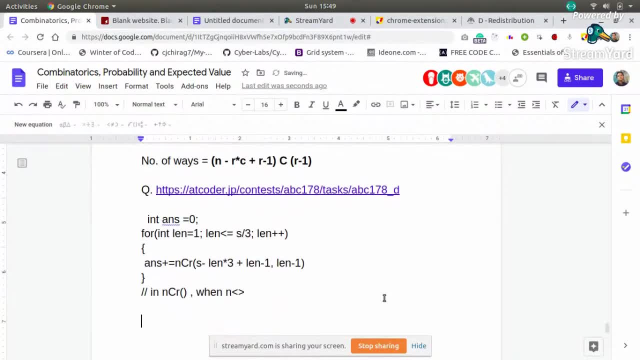 when n greater in and whenever you write this ncr function of n cross r. so when n is greater, n is less than zero, return zero because it is. since n is negative and should not be negative, it is outside the domain. so you return zero. okay, so this will give you the answer. so this was just 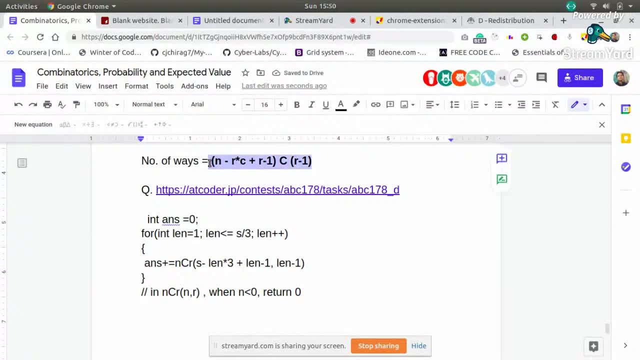 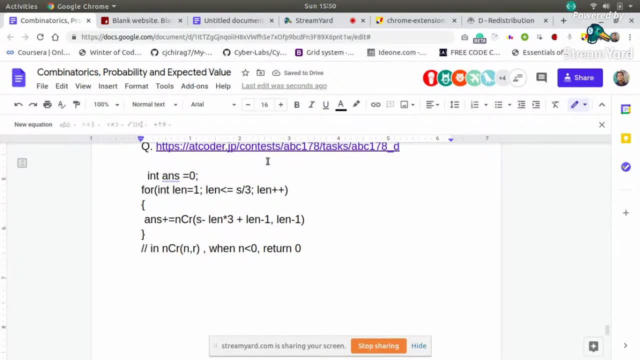 based on this type of so many times you get this problem. this formula is used many times in we will give some more problems. i will just paste the links here after the session, so just try to practice it them. and this time i want to discuss one more thing. uh, like you all might be knowing, distinct. 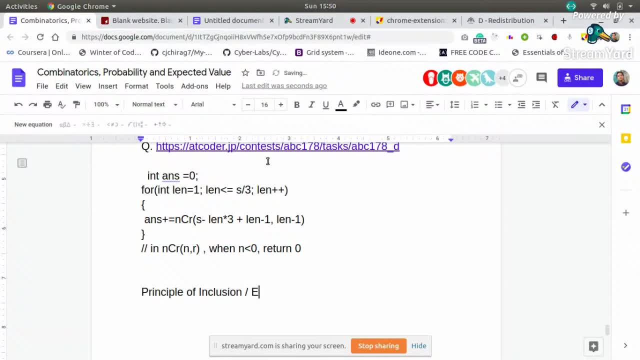 principle of inclusion, exclusion. but for this uh, this i want to discuss it one time- like uh, how you use it, like suppose you have some, when you use it like suppose you have two things like a and b, and you have, you have the number of ways to perform a task a and perform a task b, but you have to find the uh either you need. 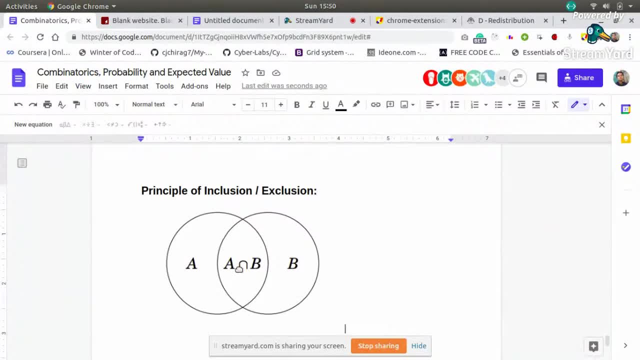 to find the number of ways to perform either task A or task B. but they have something in common: They are not independent. So that time you use this formula, A union B is A plus B minus A intersection B. Why this thing is there? Because when you are taking A plus B, the number of ways, 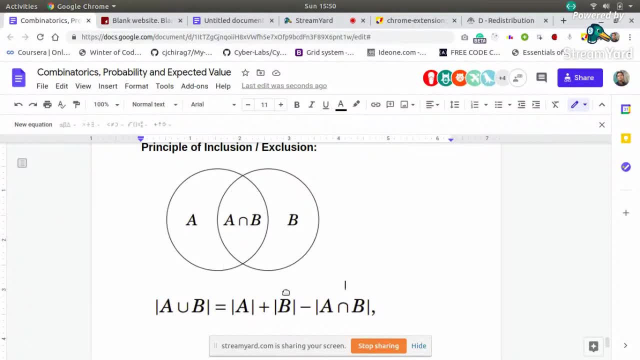 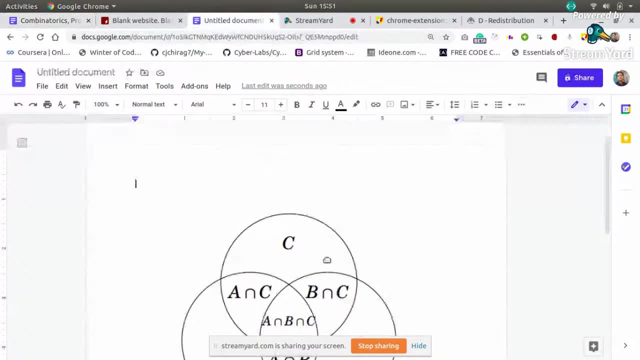 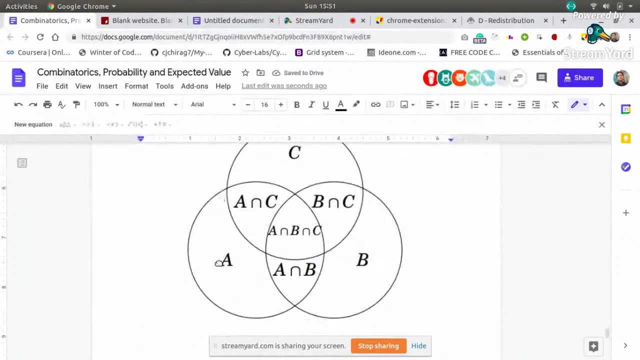 to do A plus number of ways to do B. you have double counted this A intersection B, So you subtract it once, So you get this thing. So, similarly, when you have three tasks or three ways, or you can say three kind of sets. So if you need to find all the summation of all, 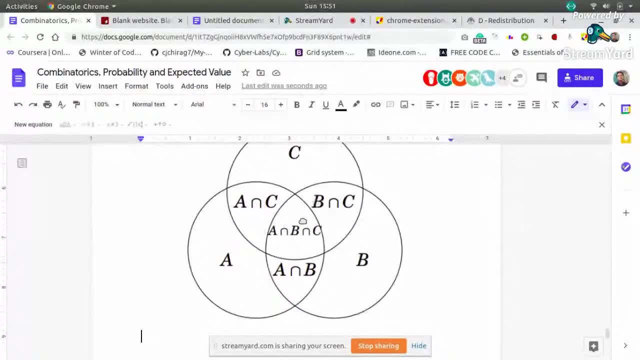 doing any one of them. so A union B, union C, either of them. any number of ways to do any one of them would be just: you can say number of elements in the set A plus number of elements in B plus number of elements in C minus this thing: A intersection B minus B. intersection C minus. 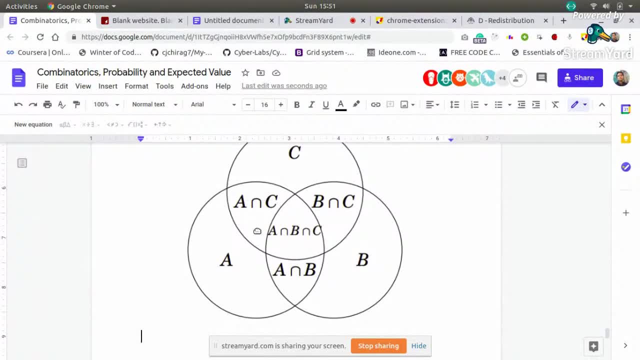 A, intersection B, Since minus we are doing because we have added these things two times. But whenever you do minus these things, minus these three things, so you will see that you have double subtracted. this intersection means one extra time, So you need to add it up. So 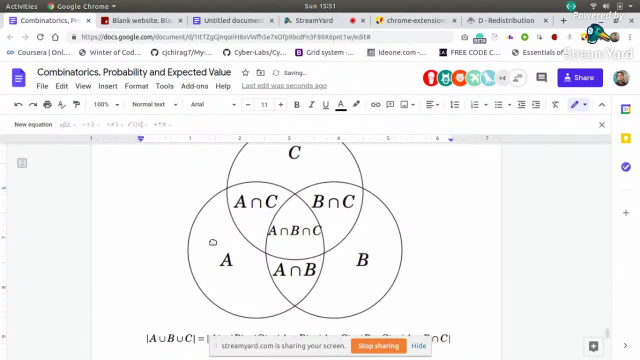 the formula becomes something like this: So I think you all might be knowing this, So just I am writing it directly. So you all know that. why this is called inclusion-exclusion principle? Because inclusion-exclusion- inclusion means you are including this element. 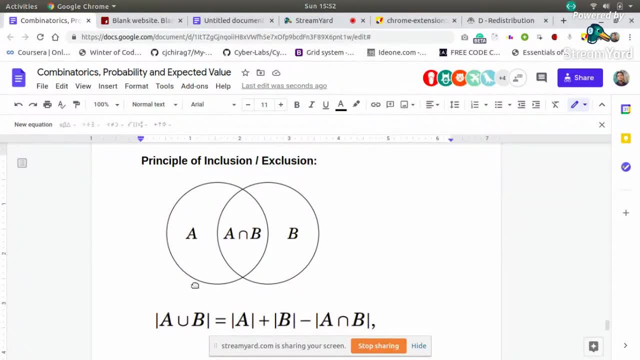 And exclusion means you are not taking it. So since whenever you are just finding A union B, so we are including A and B, But since we have double counted this intersection part, so we are excluding it. Similarly, inclusion-exclusion means that we include something. 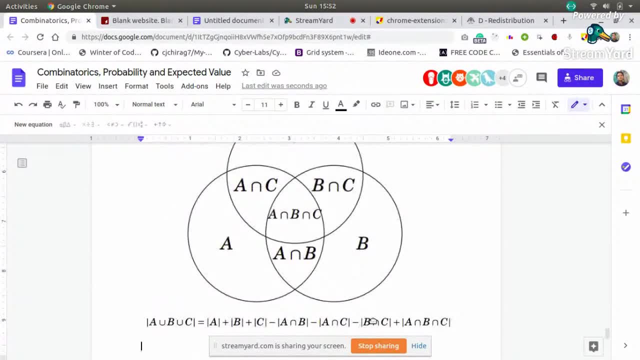 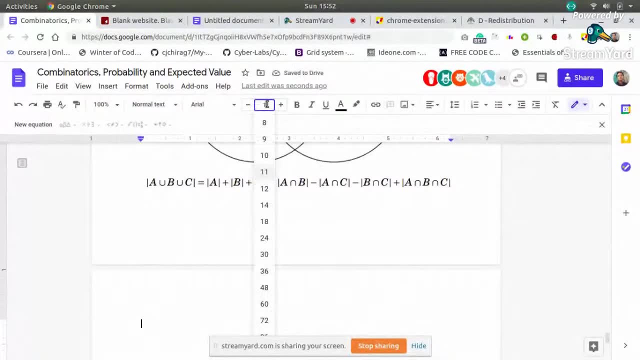 but there is a double count in it. That thing is excluded. So when is this used? It is used generally, when it is used when we need to find means. when you say when it is, you say when it is easy to find intersection of some offsets or anything, intersection rather than union. So suppose that in very easy it is. 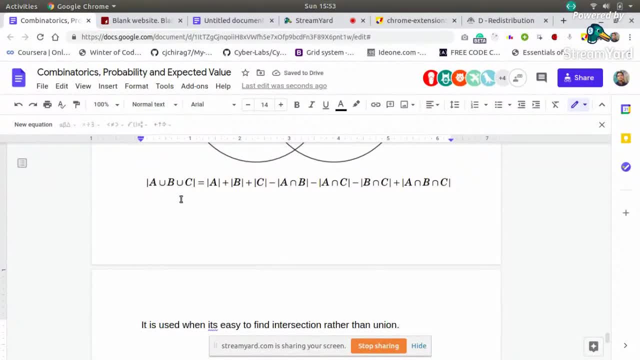 very easy to find this intersection So you can directly find the union using these intersections. So in such kind of problems you will use this thing, So try to remember it. or taken So. similarly, you have something called derangements. So derangement means there are, let us say, if you have, let us say you have n people. 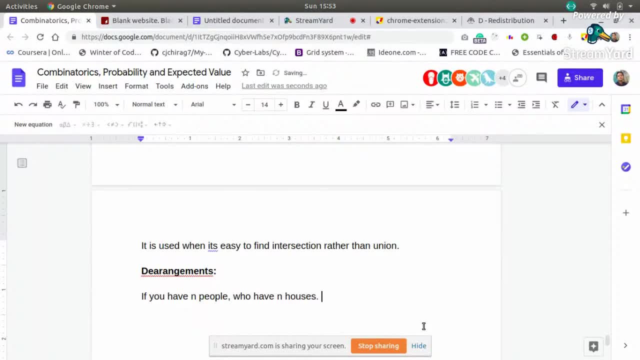 who have n houses. you can take n houses and find the number of ways so that no people, no person reaches his own house. So since all the people are having some house, like one person is having some fixed house, second person has is having some fixed house some. so you need to find the number of ways. 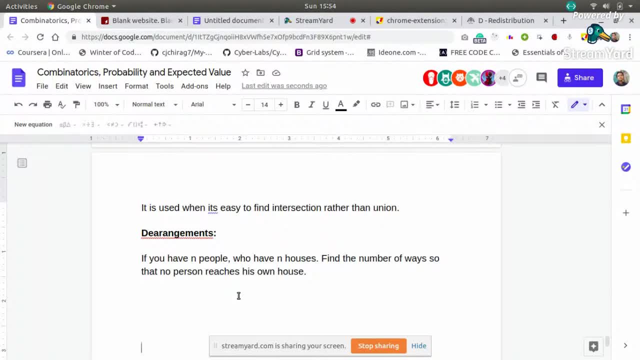 such that the person cannot reach his own house. So number of ways for this. so the number of ways would be using you, You can find it using inclusion, exclusion principle should be a number of number of ways to find this thing is just suppose there is no such restriction. You just need to distribute these. 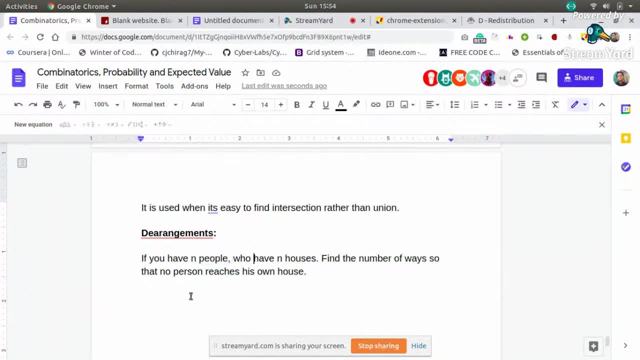 n people, or arrange these n people for n houses, So you can arrange them in total ways n factorial, but you subtract whatever are the ways, invalid ways in which suppose we say, let us say, at least one person reaches his own house. So how many ways are there such that 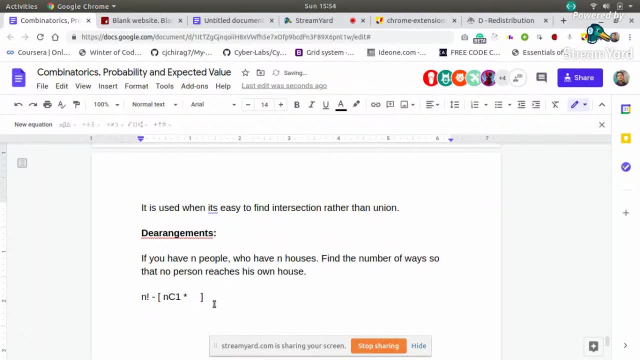 One person reaches his own house, So it will be n? c one in two, since one person has already reached his house. So how many are remaining? n minus one. So those n minus one people can be arranged in n minus one factorial ways and minus one factorial ways, And similarly it may be. 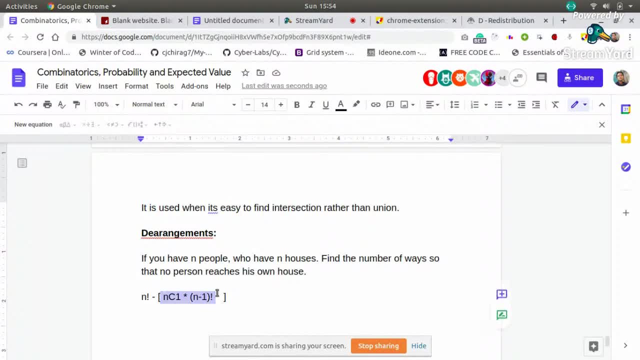 possible key means. in these ways we have double counted those ways where two people have reached their own house. Take care, So we will. just you can say We will subtract it. So what are the ways when two people, at least two people, have reached their 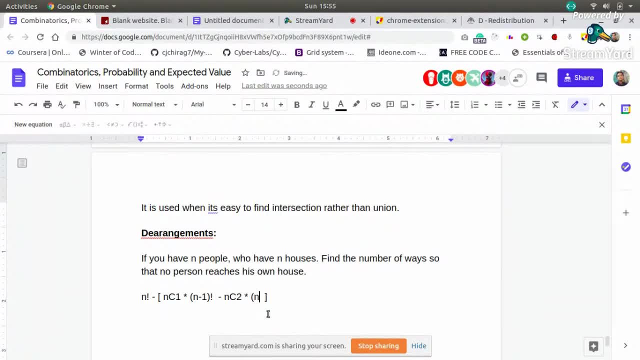 own house, It will be n c two into. remaining people are n minus two, So they can be arranged in n minus two factorial ways. Similarly, in this, in these we have, in these things, we have double counted those where three people have reached their own house, So at least three people have. 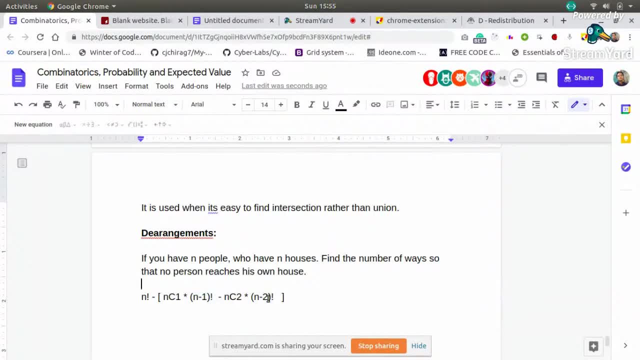 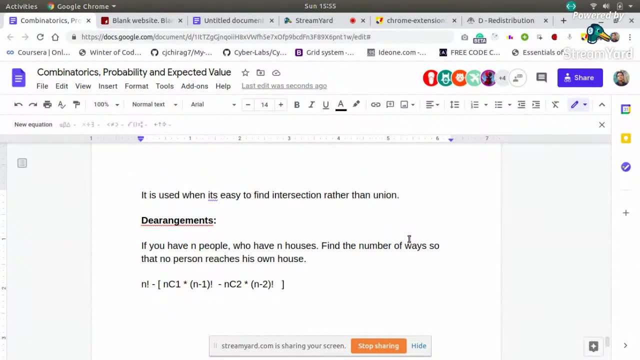 reached their own house. We have double counted those. So we need to add it up like just: we are following this principle of exclusion and inclusion: plus, then minus, then plus and minus, and this is so on. So we add those people n, c, three into n minus three. factorial means at least three people have. 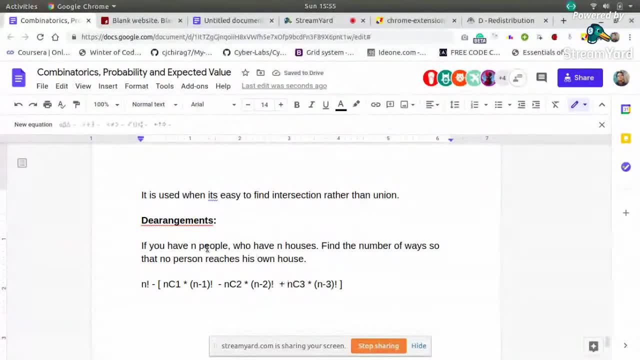 got there exactly. they have reached their own house. So it says: people is having only one house of their own, So we are arranging those people together. So in this way you go on up to, you will get it up to when this up to n c n. So it will be n c n will become one into n minus n factorial zero. 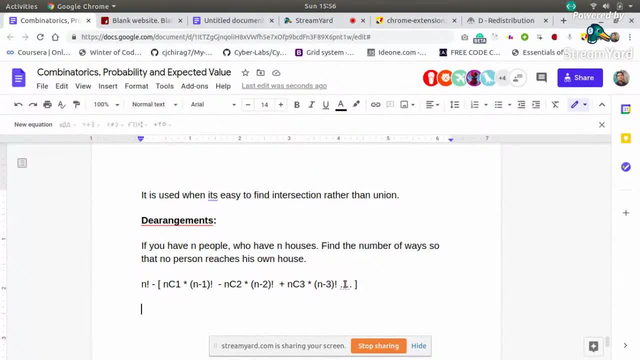 up to that term you will go on, so this thing is also called day arrangements. you can also write in: uh. if you simplify this, you will get something like: nc1 is n, so n multiplied by n minus 1 factorial, so it is n factorial, n factorial. or you can write in: n factorial by 1 factorial. 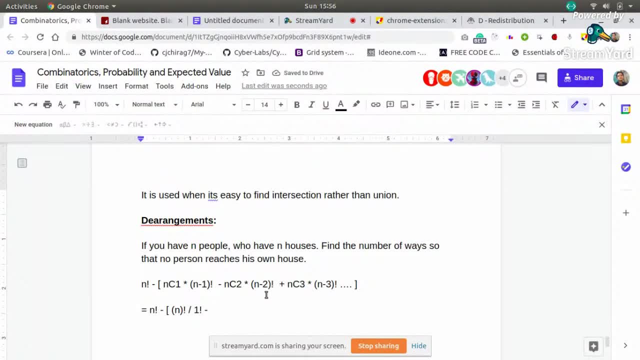 minus. if you do nc2, it will be n into n minus 1 divided by 2, and n into n minus 1 divided by 2, so it will be n? uh into n minus 2 factorial, and so it will be n factorial divided by 2 factorial. 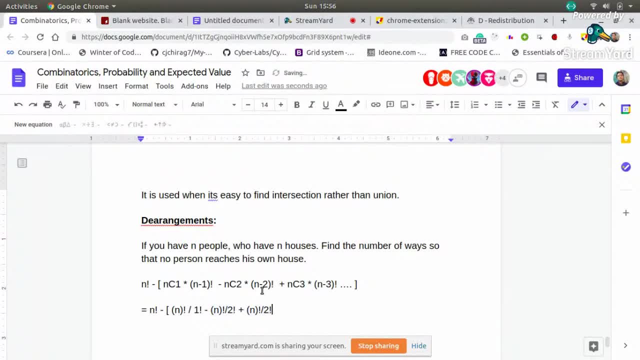 and so on. so it will be uh. for the third term it will be plus n factorial divided by 3 factorial. for the fourth term, it would be n factorial divided by 4 factorial, and so on. so this is the formula for d arrangement. it can be similar thing like, it can have similar question like and you: 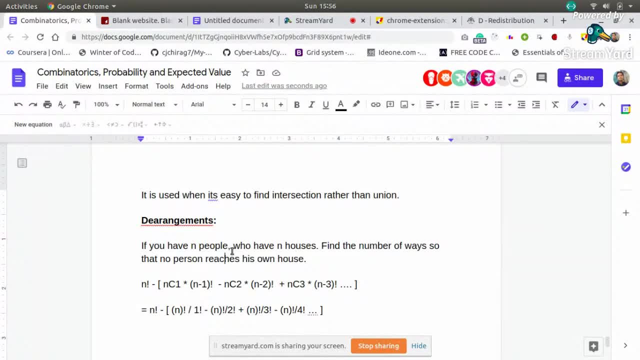 want to send n letters to n mailboxes such that one letter is uh having a written. it has written the address of one mailbox only. so the number of ways you need to find such that no letter reaches its uh destination, uh mailbox something like that, so means uh such kind of. 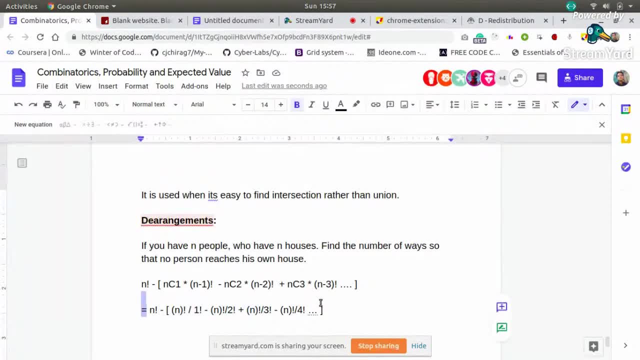 problems are uh under the category d arrangement, so you can solve it using this formula and if you know this, how it is derived, using the principle inclusion- exclusion, you can solve it directly. so now, just i will discuss one or two, uh small problems of probability, then i will hand over to 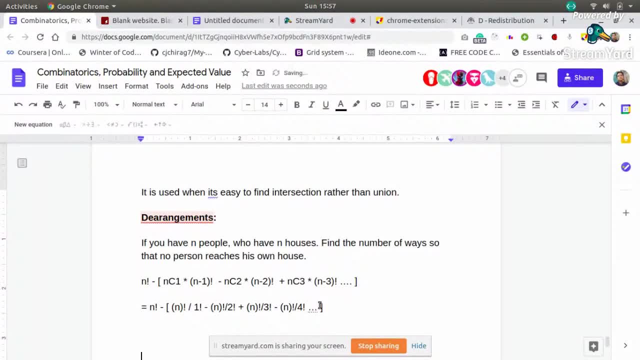 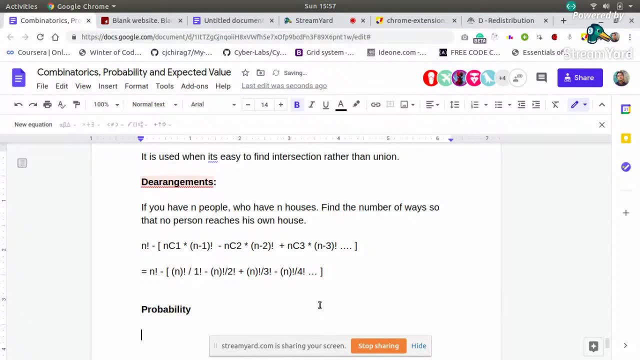 uh, let me, let us consider this problem. i have a probability. uh, there is nothing to discuss as such, but you should note that for probability, that, uh, the formula is probability of an event, of an event, e is the favorable outcomes divided by total outcomes. favorable outcomes for event e. 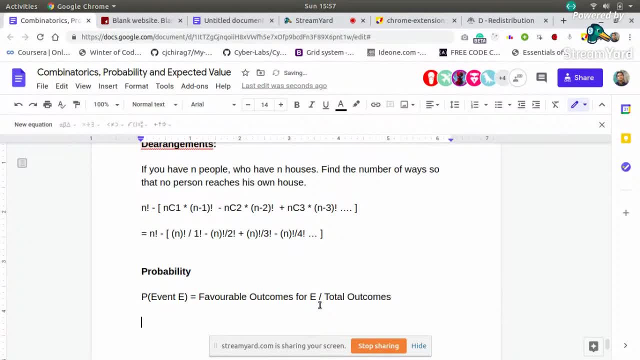 divided by total outcomes. you all know this, so let us try to solve one problem. so you are. you all know that uh, in a deck of cards they are are 52 cards means there are 52 cards in total, 13 of each category, 13 of spade, 13 of uh like. 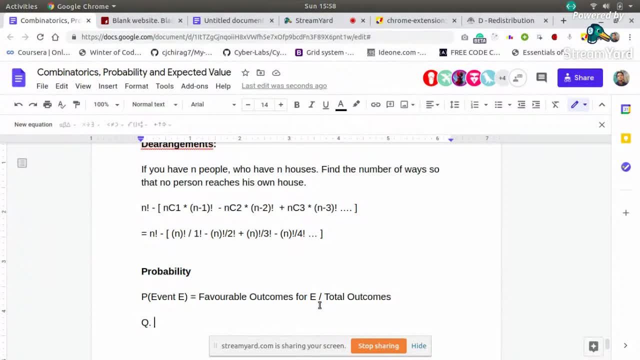 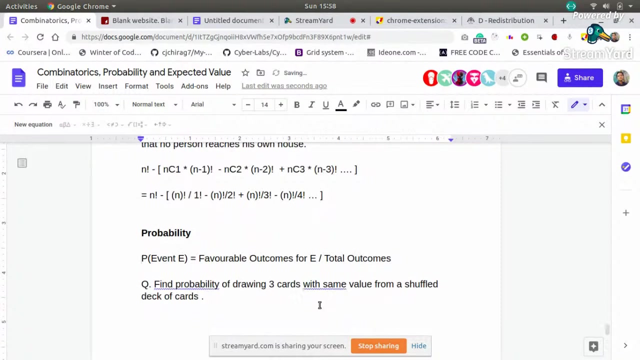 what we call diamond or whatever. so you have a deck of cards, so you need to find- uh, find probability of drawing three cards with the same value, with same value, from a shuffled deck of cards. so, anyone, what should be your answer? you need to draw three cards with the same value from a shuffled deck of cards. so what? 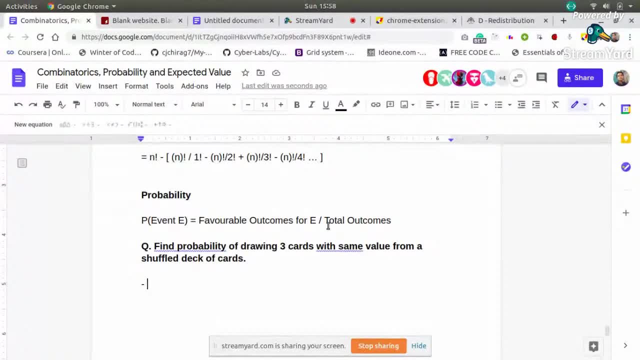 what will be the total number of outcome? total will be 52 c3, since you need to draw three cards with the same value from a shuffled deck of cards. after 52 cards, you are selecting any three cards, so total outcome will be: uh, total ways or total outcome? total ways or total outcome would be 52 c3. fine, 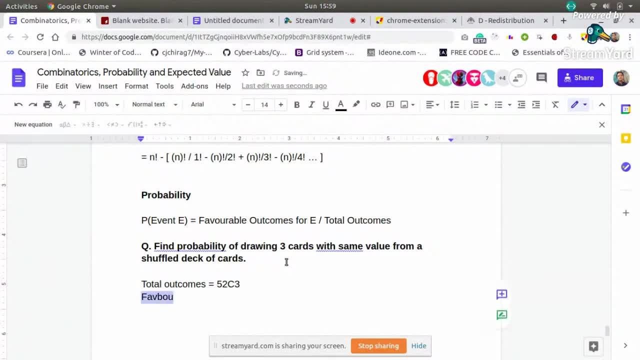 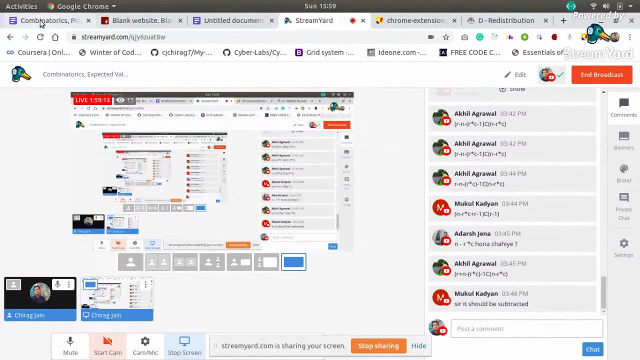 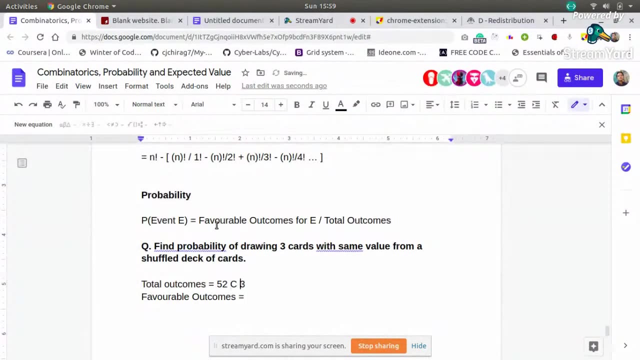 and your favorable outcome would be- uh, try to answer if you know it: 52 c3 is the total outcome and how many are favorable. so for favorable outcome, just you select, uh, any one deck like like any, any one type of card, like either a spade or diamond or something like that, and out of 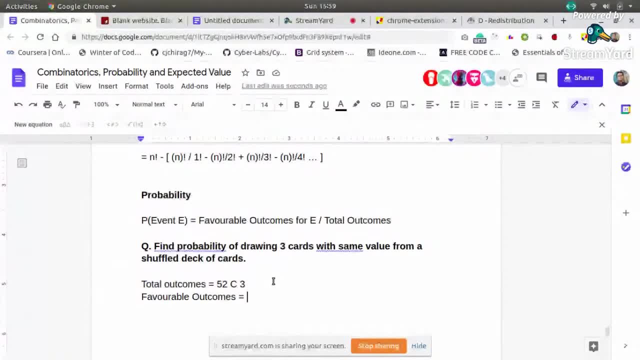 like you can say, you need to select cards with the same value from a shuffled deck of cards. so it will be something like you select a value out of 13 values, because there are a total 13 values. so you select first any of the cards that you select and then you will get a total of 13 values. 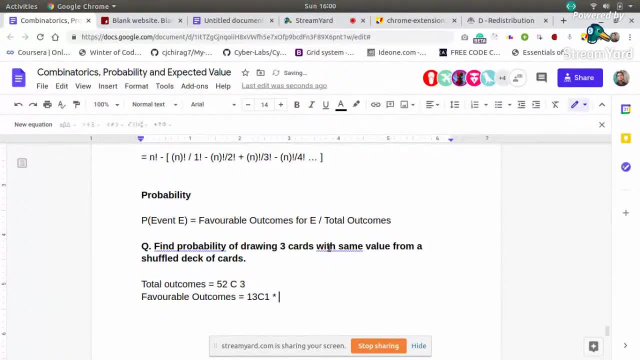 then you will get a total of 13 values: 13 c1 multiplied by now, 13 c1, uh. 13 c1 means 13 ways to select any one value, or, and after that we selected one value. let us say like i've selected a value of four. so there are four categories. 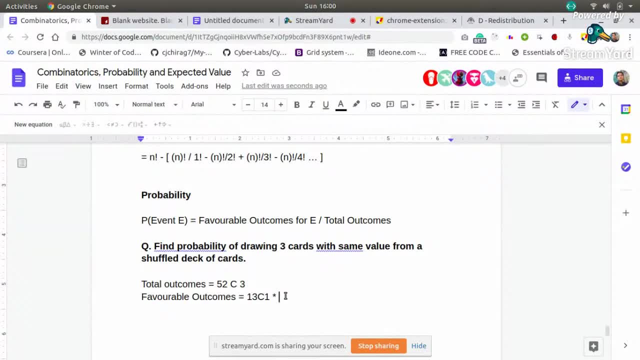 of in four categories in cards. okay, so in those four categories, select any three categories. so that will be the number of ways. so it will be. it will be something like 4, c3, because there are total four categories, like spade, black heart or whatever, heart, diamond, whatever- i don't know the names in english. so those were. 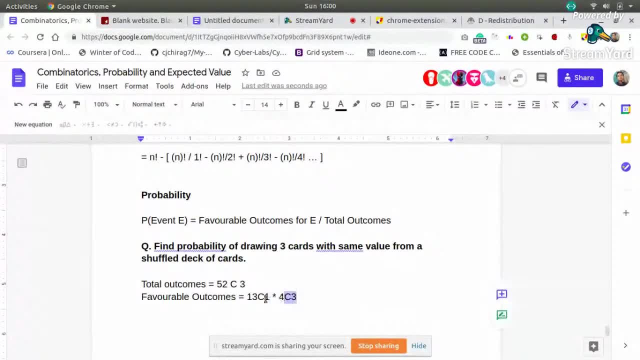 four categories. out of that, you select any three categories. so four series, three ways for that, and you select any one value, because all should have the same value. so it will be this, it will be this. so the probability would be this thing divided by this thing. so, uh, for probability, for. 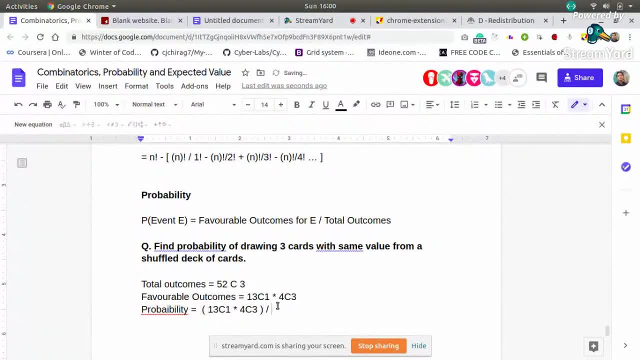 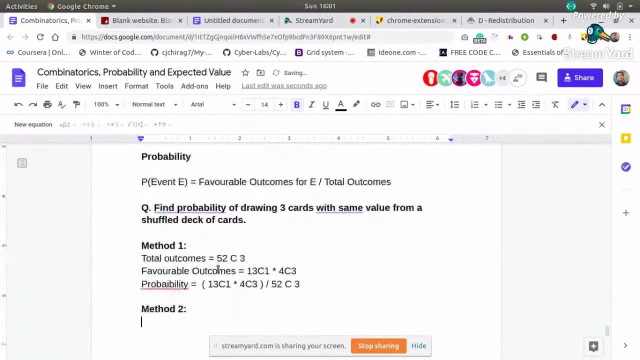 finding probability. there are two ways actually. uh, one is this: using this formula, but sometimes it is easy to just go by the events. so, uh, this is method. one. or one more method is just: uh, you can say: just simulate the, simulate the events, like, uh, if you just simulate the events. 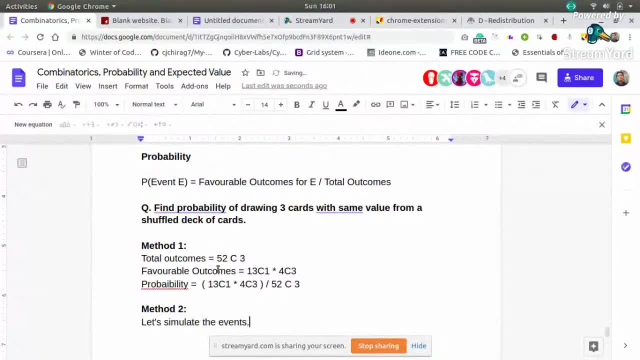 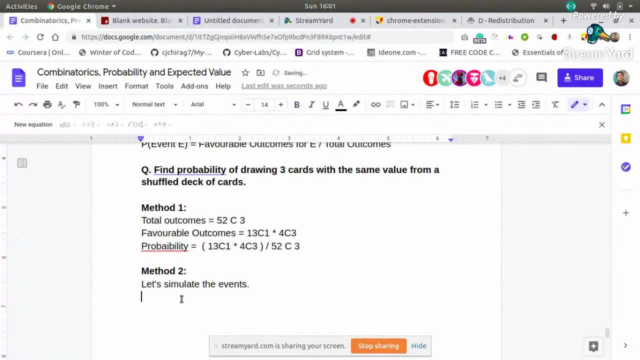 so first you will select any card. so since there is no restriction on the first card, first card can be anything, so there is only uh means one. you can say uh, it is not having any role in the event, so you can just go by the events. so this is method one. or one more method. 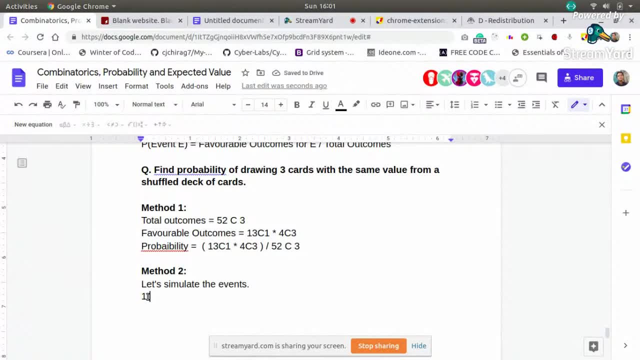 in the probability, so you selected any one card, let us say so, for that will be having a probability of one, so you need to select any one card, so it will be having a probability of one. so you will always select one card. and after that you have selected, let us say, one card, so you need for the 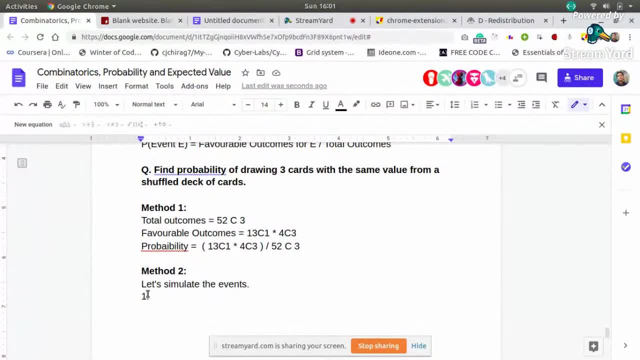 second card. you need a card with the same value. so, like you selected the first card, as with value five, so the second card should also have the same value five. so how many cards are remaining with the same value, so that from those many cards you select- uh, you select uh- any one of them. and so it would be something like: since you have selected one card, 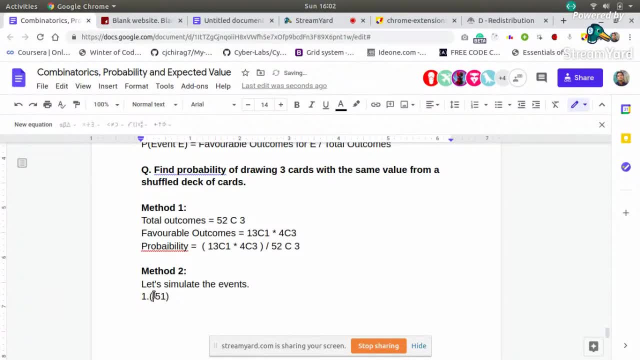 it will be. the remaining card will be 51 and out of those 51, you can select only uh, since you have selected, let's say, a card with a value of five. so they, how many cards are remaining with the value of five. there are three cards more remaining with the same value, so it will be 3 by 51. right and for. 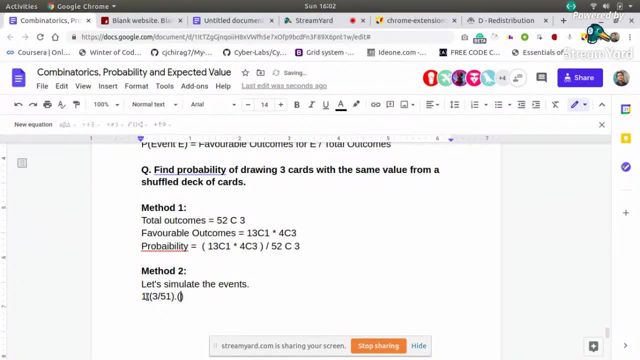 the third card. also, you need to select the card with same value, so that card will be 15 right. so? and since you have selected two cards with the same value, so only two cards more will be remaining with the same value. so it will be 2 by 50.. why 50? because now, since you have selected two cards, so 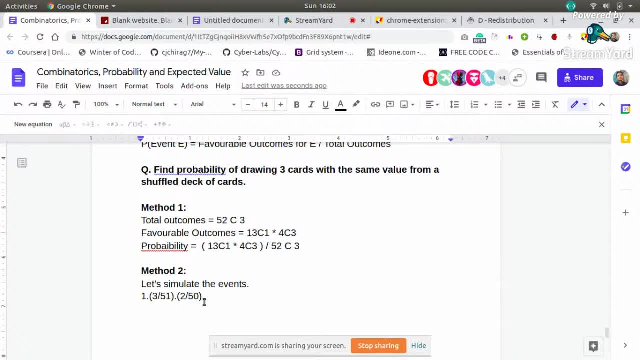 the remaining cards in the deck is 50 only. so this is also it. both of these should give the same answer. you can try calculating. you should get the same answer. okay, so this was one question and one last question of probability like: uh, and why we are multiplying, because it is just following the 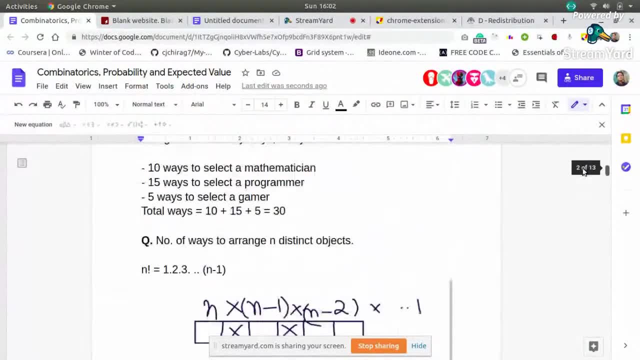 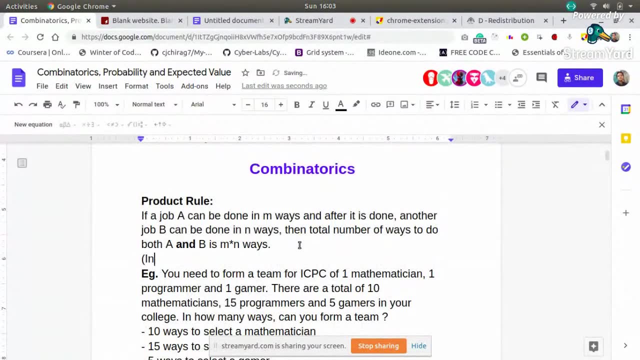 simple product rule which we discussed in product rule. what is it? keep one by one. whenever you are performing the event one by one, and they are independent events, you multiply them. uh, i forgot to write it: independent events, independent event or independent jobs. whatever you say, similar rule applies for probability when. 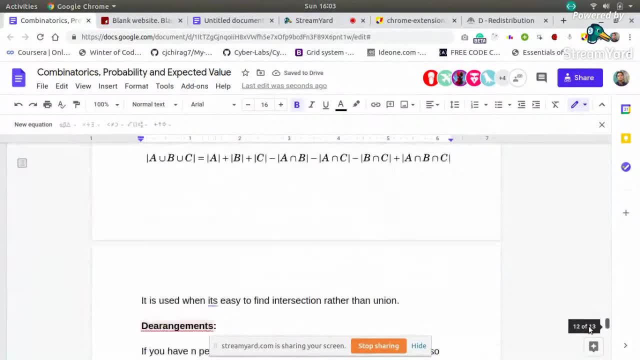 they were. whenever they are independent events, you multiply them to get the total probability. so here, since these are independent events, first selecting the first card, then second card, so i'm doing it one by one, but uh, like it is something like which is uh, you can say: uh, i'm doing it well, these events one by one, so i can. 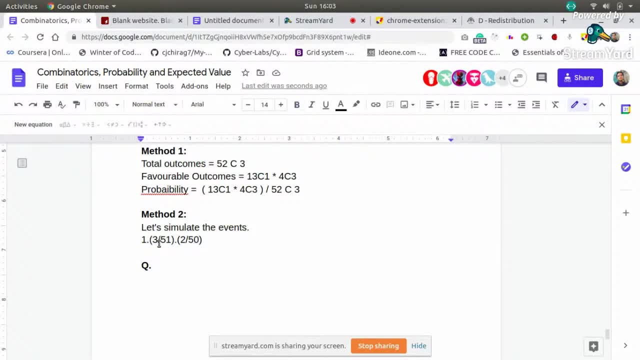 you multiply it in such cases. so try to solve them means try to solve this one. you will get the final expression: is this okay or one more thing? is just uh one more question or probability? then i will hand over to varun. so you have uh 50 white balls and 50 black balls. 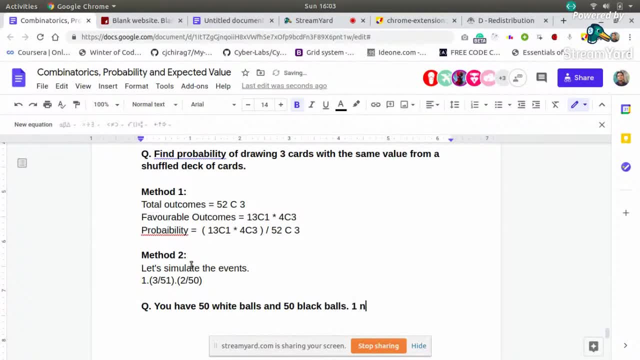 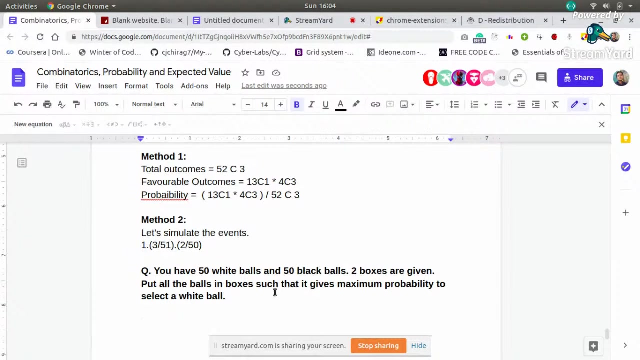 and two boxes are given to you. put them in uh ticket to put all the balls in boxes such that, uh, it gives maximum probability to select a white ball, means the thing is that you are selecting any ball out of any box and, uh, the probability, whichever you get to select, the probability of selecting a white ball should be maximized. 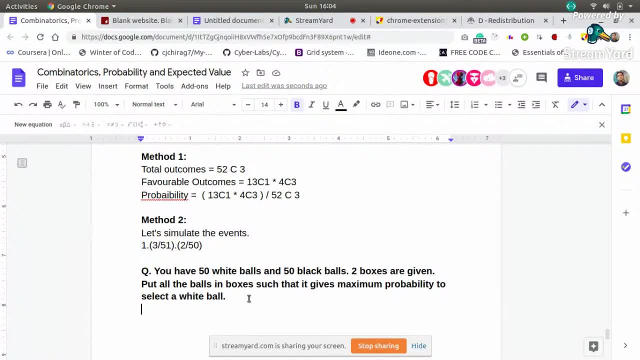 so you need to put the boxes in. uh to you need to put the balls in boxes. this probability is maximized. so how would you do it? like uh means two boxes are initially empty, you can place any number of balls in any boxes, such that, uh, whenever you are selecting a ball, you can select a ball from any of the box. 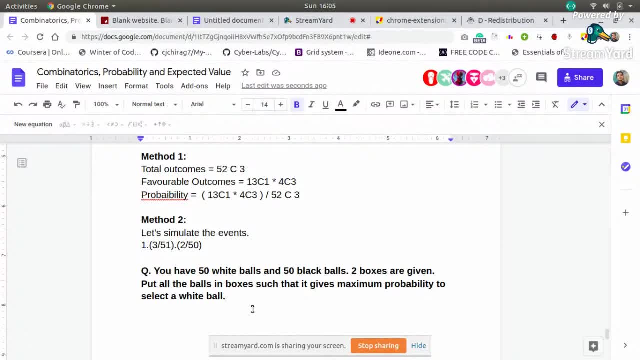 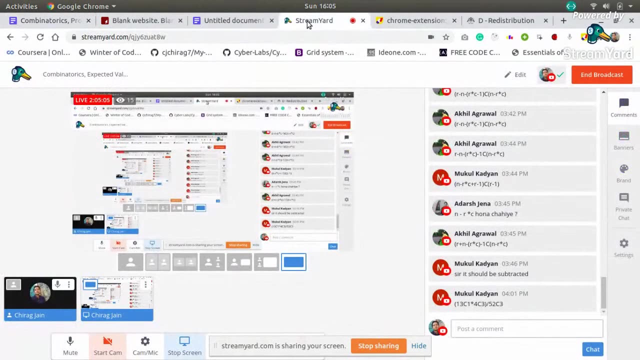 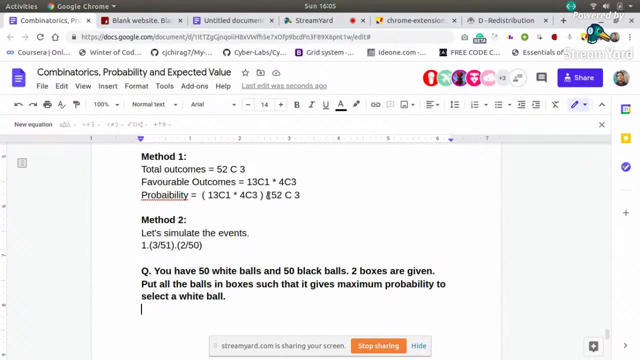 so it is like there is no restriction on that. but, uh, you need to maximize that probability. so what would, what would be your arrangement? so how many balls will you put in each box? try to answer this. this means, uh, these, these ballers, these balls are initially. uh, you have these balls initially. 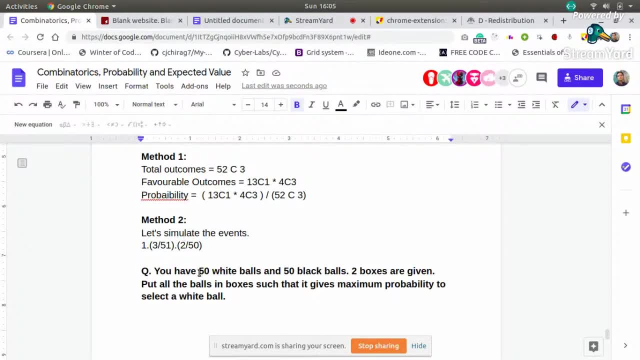 and these two boxes are empty initially. so you need to put all the boxes in some of the box, like, uh, in some of the boxes you need to put all the walls, such that it gives you the maximum probability to select any match guess out of all the boxes. 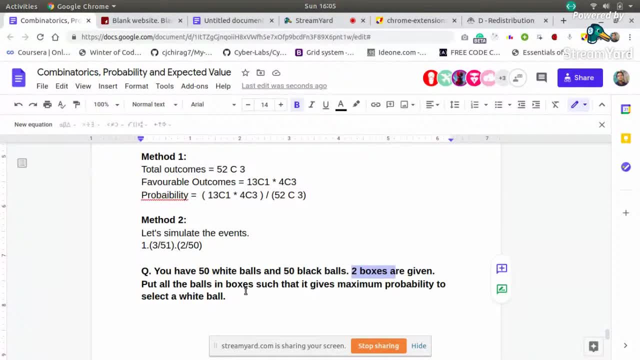 that i just psyche in most cases is 0, because the more boxes are empty, the more you put the ball in it you will get in combo. so everything else kind of like that point is going to be the select a white ball. so the probability of selecting a white ball should be maximized. 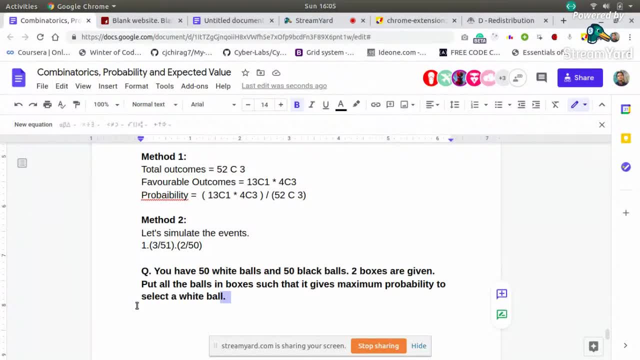 so what kind of how, how many balls in which box you will put if you put all white in one box? so okay, one way is this. so uh, someone is told, so let us try all the possibilities, whatever are the possibilities we have. so one way, uh, like if we put all white in all right wall in one box, 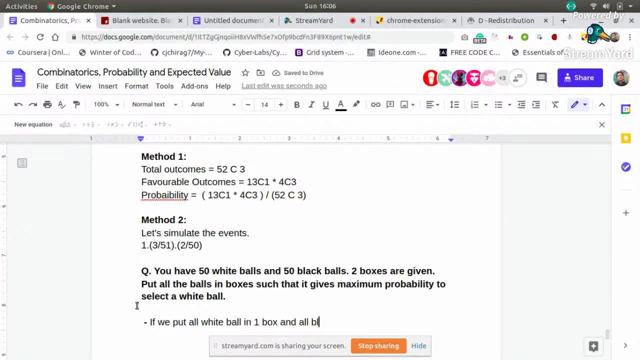 and all. so if you put all by all white balls in one box, then definitely you need to put all the black boxes in the second box, because you need to put all the balls, all the balls in some, in some of the box. so, and all the black uh, all the black balls in second box. so total number of uh then 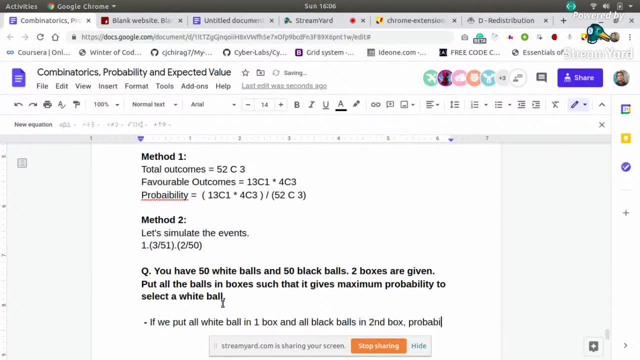 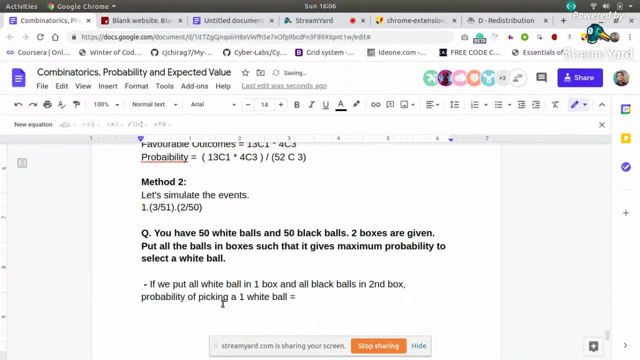 the probability. so, in this case, probability of picking a white ball is what will be the probability, since, one by two for selecting the box, one by two, multiplied by one by two, multiplied by if you, if there are, uh, all the white balls in one box, it will be one plus in the 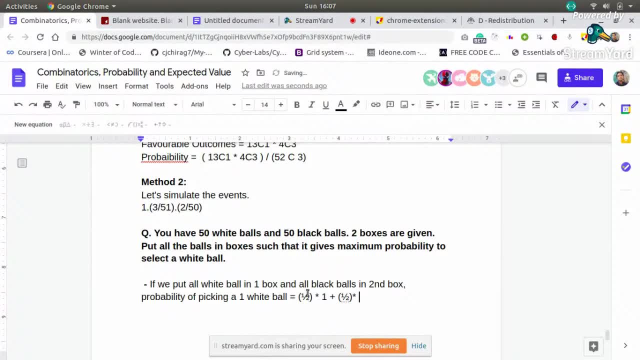 second box. uh, probability of selecting the box. second box, because there are two boxes, any box can be selected. so half probability for this box, half probability for this box, so half into one, for in the ball, in the box which we have all the white balls, and second for the second box, so in the 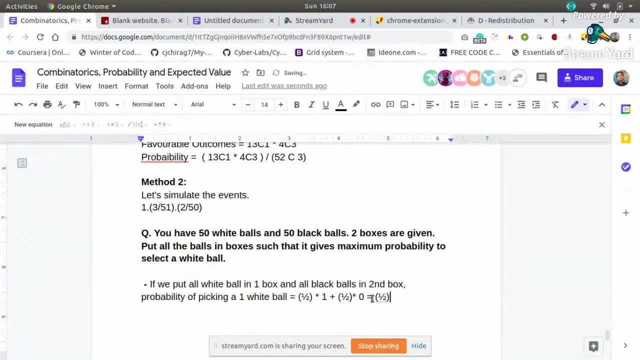 third will be zero. so you will get the probability as half only. so the question is now: can you increase the probability more than half? uh, 0.5 probability. so try some more cases. so all all right in one box gives me the probability of one by two. now my question. 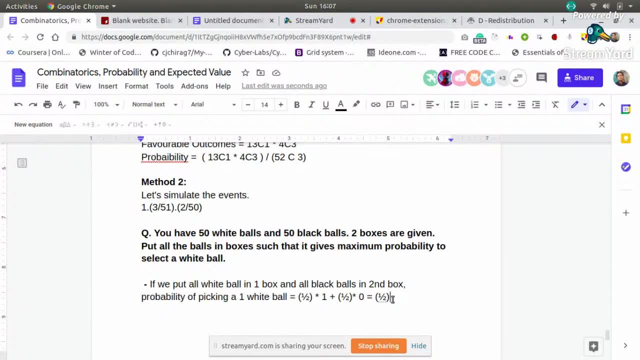 is: can i maximize this probability even more? so, just uh, this, let's try this thing. if we put uh, only one white ball means you are close to the answer you thought. so if we put only one white ball in one box, in box two, all remaining, box all remaining, you can say 49 white balls and 50 black balls. 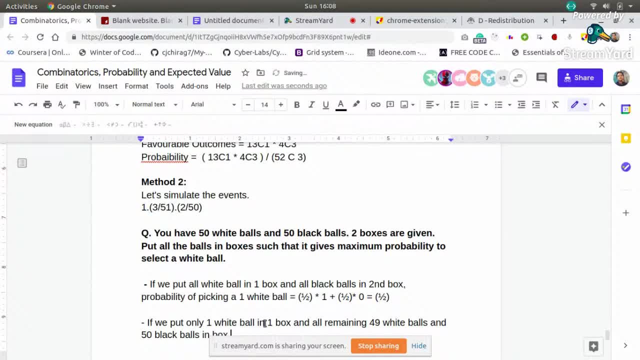 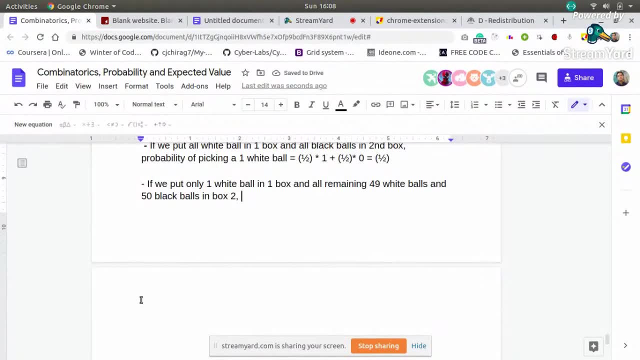 in box, two in ticket. so that time probability of uh getting one white ball would be what the probability of picking one white ball becomes half into one, because in one box, uh in the first box, only one white ball is there. so definitely if we go to the first box we will get a white ball. so 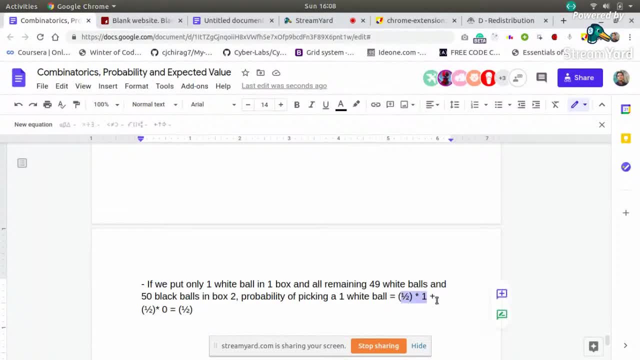 half and two it will be plus considering that. so if we take 0.5 probability, then we have 1 white ball. what will we believe? yeah, in your final box, 1 white ball, Half into 1, plus half for the second box, Half into 49 by 50.. 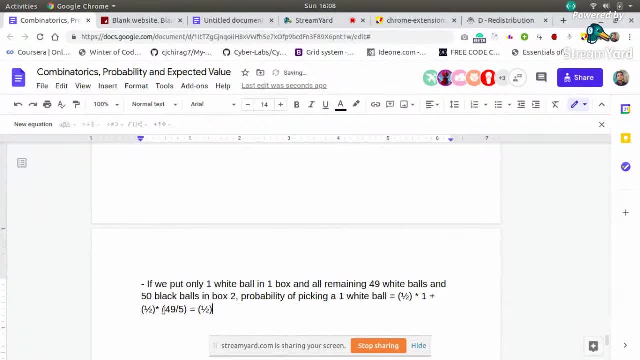 Now I have maximized the probability for the second box. So this thing: 49 by not 50.. It will be total balls of 99.. 49 by 99.. Yes, Because in the second box there are 50 plus 49.. 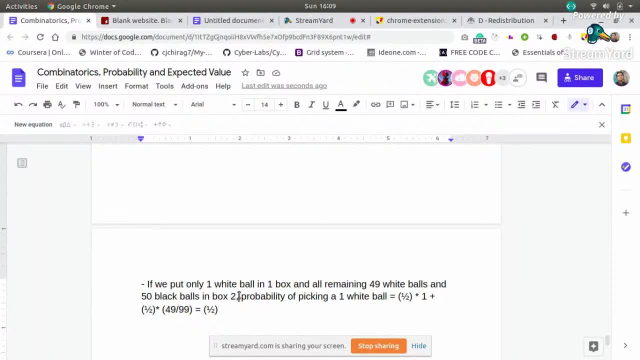 Total 99 balls. So this will be your answer. So this is the maximum probability. So this is not half, but more than half Half. plus this thing, You can say 49 by 198.. Plus half, Take it. 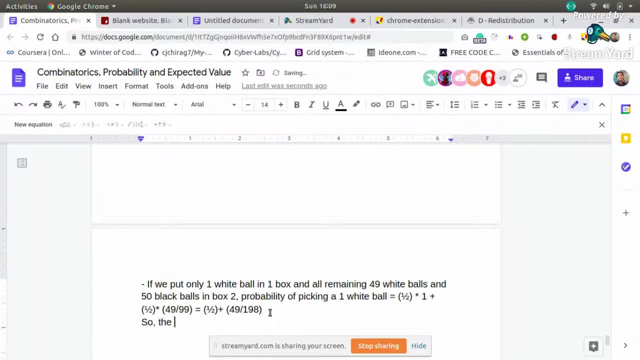 This thing you get. So this is the maximum probability. This is the maximum probability, Fine. So if you have any questions, you can ask in the chat. So now, Bharat, you can join that link. So I will allow you to screen share. 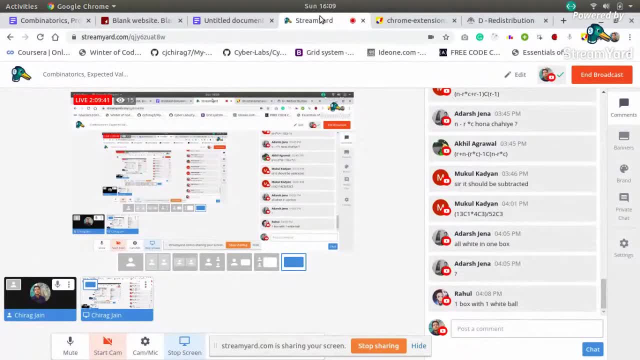 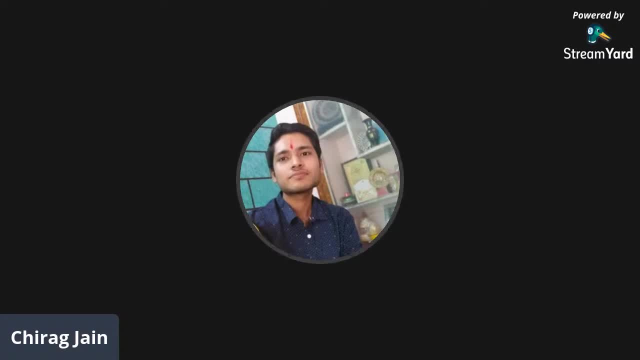 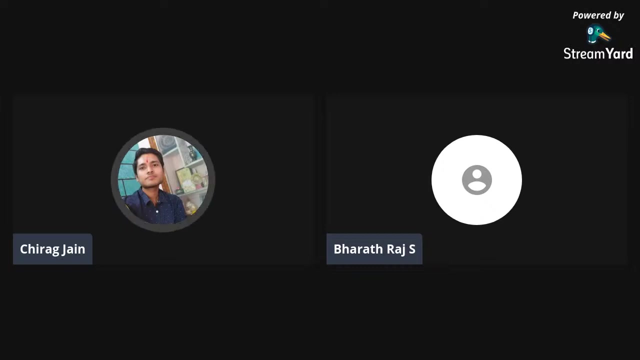 One box and one whiteboard. Bharat, please join this link so that Just wait a minute here We will join in two minutes. Till then, take care, Any doubt, you can ask Bharat. you can share your screen. 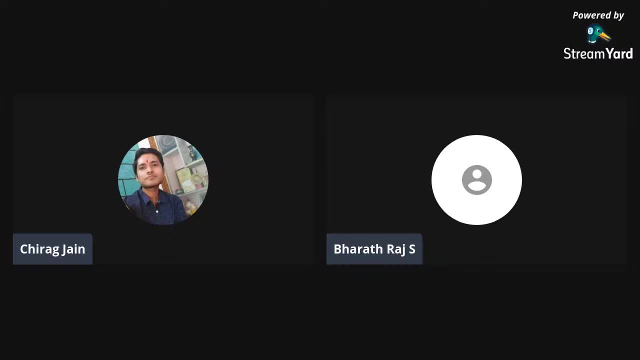 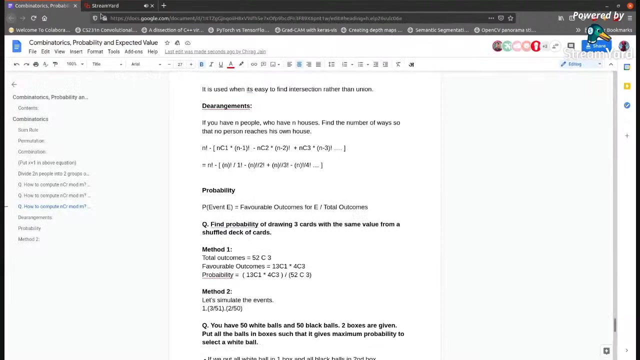 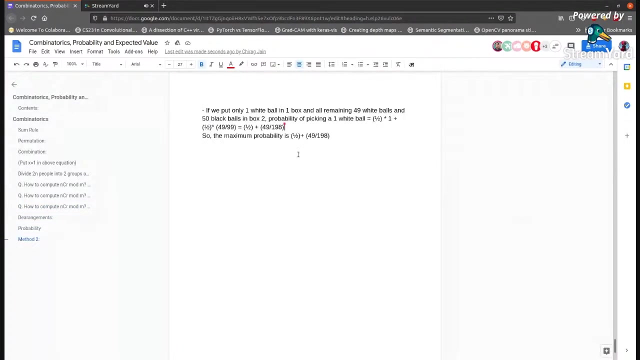 Okay, It is visible, right? Yes, it is visible. It is visible, So probability is done. So next we will go to Expected values. Expected values, So expected value basically means E of expected value. Expected value basically means: 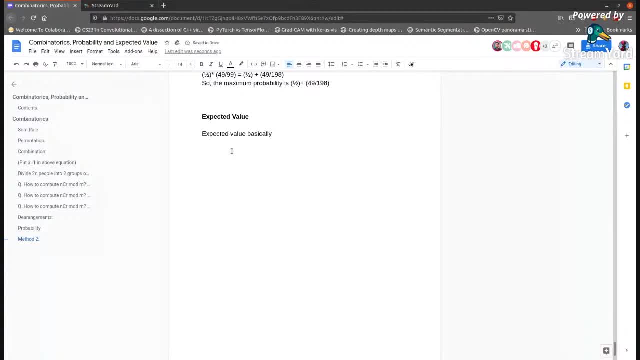 The You are performing some experiment And which is the value that you are most likely to get. This is the basic idea behind the expected value: The value that is most likely to occur in an experiment. Experiment means here random experiment. So if we take it as mathematically, 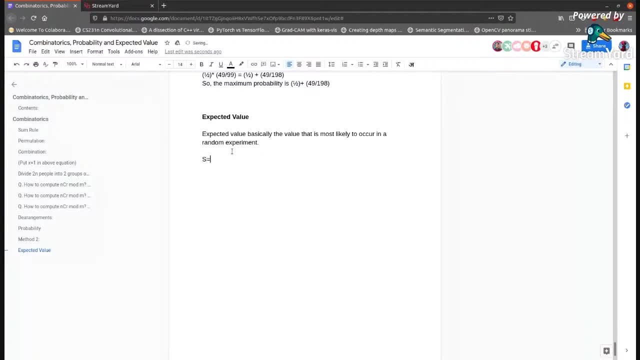 Let's say you have a sample. You will have a sample space That is having S 1,, S 2, and so on till S n events And expected value of this sample space Will be equal to and sometimes the events. 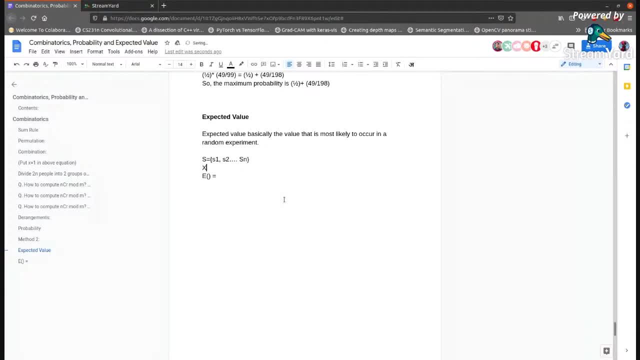 These events will not be numbers, So for that you have to associate a value, So that value you'll call us random variable. This random variable is x, So So X of S1 will be some integer X1 instead of 1. let us take some other value. I So expected. 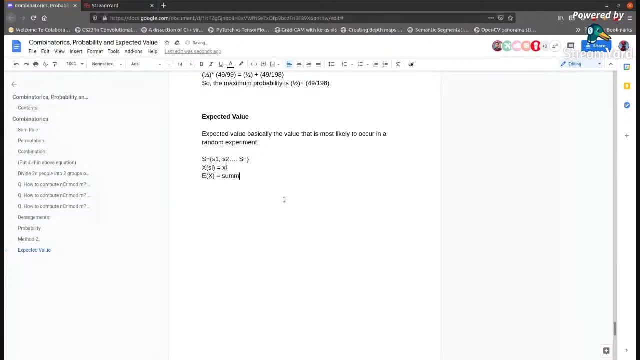 value of this random variable will now be equal to summation of probability of event S i times X i. This X i is basically the value associated with this event for every i. So this is the basic mathematic definition, and I think most of you know this already, And 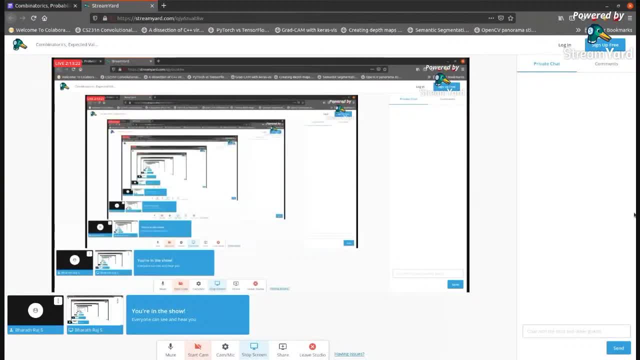 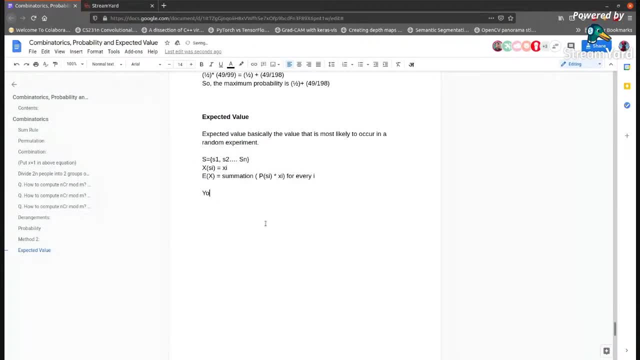 so we will start with the basic problem. So you are rolling a six sided dice: What will be the expected value? So you can try this problem based on this equation. So here your values will be 1,, 2,, 3,, 4,, 5 and 6, and what will be the expected value? 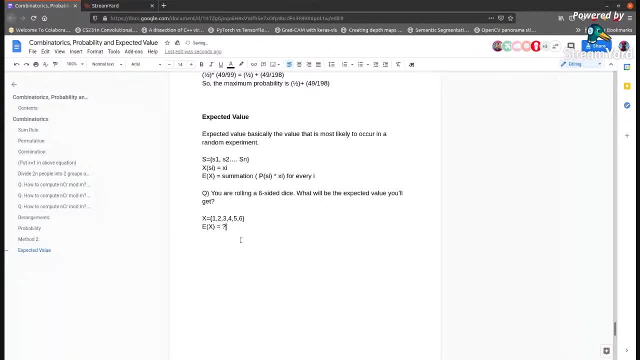 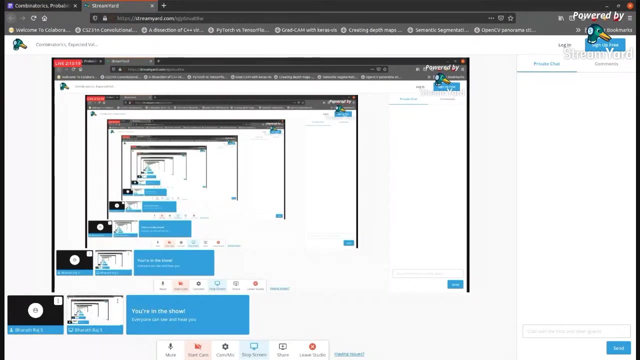 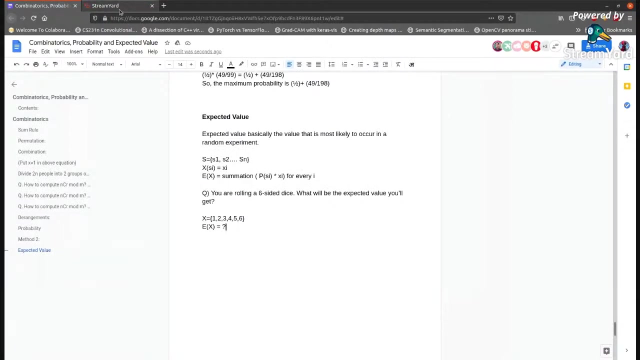 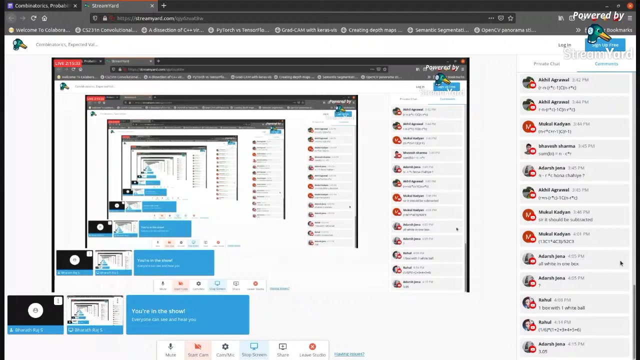 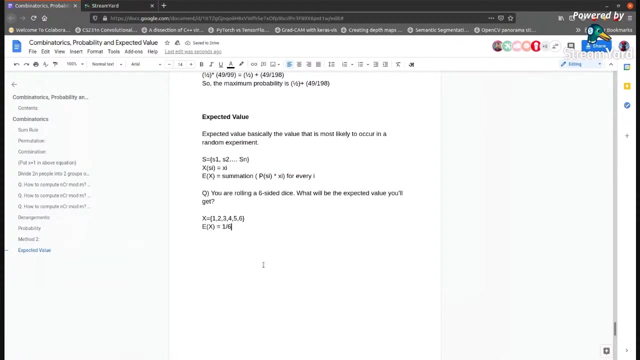 of this You can type in chat: 3.05,. okay, yeah, exactly. so for everything, the probability is going to be 1 by 6, probability of getting 1 by 6 is going to be 1 by 6, probability of getting. 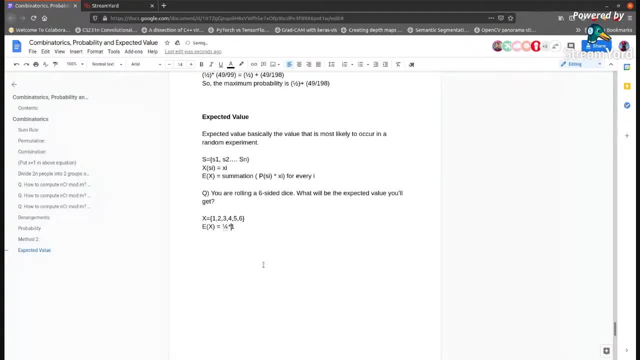 any number is going to be 1 by 6, so answer will be 1 by 6 into 1, plus 1 by 6 into 2 and so on. so we will take this 1 by 6 common outside and let's write this: 1 plus 2 plus. 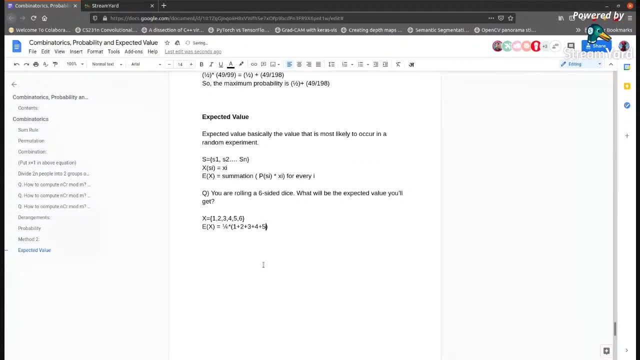 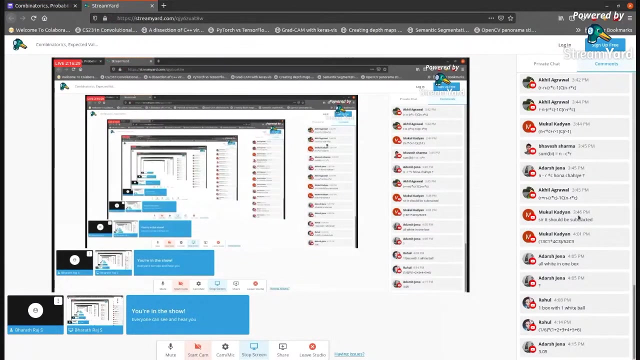 3 plus 4 plus 5 plus 6, this will be your expected value and this will be 6 into 7 by 2 by 6.. Okay, I hope this is clear to everyone, so let's go to the next problem. so, basically, 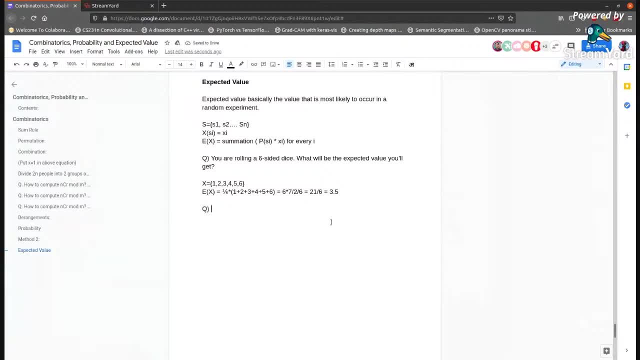 first we are solving some basic problems by hand, then we will go to CP point of view. Let's take the same problem and change it a little bit. So let's take the same problem and change it a little bit. So basically, first we are solving some basic problems by hand, then we will go to CP point. 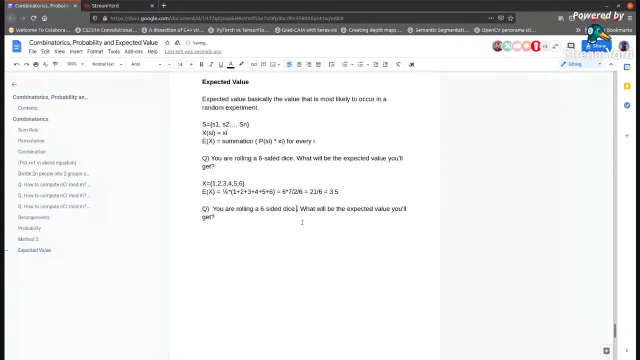 of view. So let's take the same problem and change it a little bit. So basically, first we are solving some basic problems by hand, then we will go to CP point of view. So basically, first we are solving some basic problems by hand, then we will go to CP point. 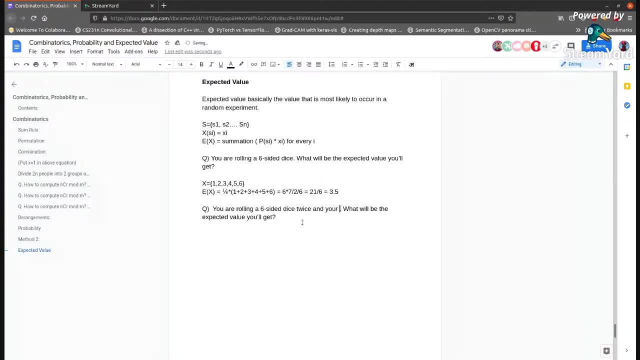 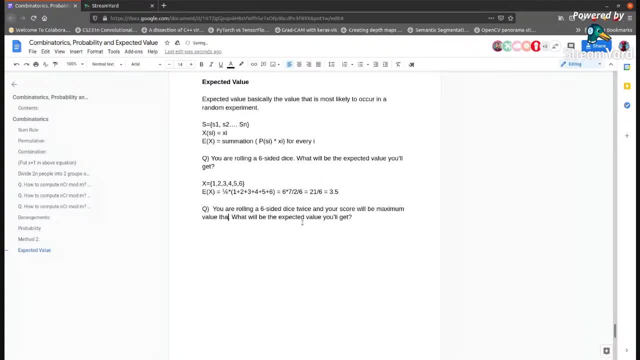 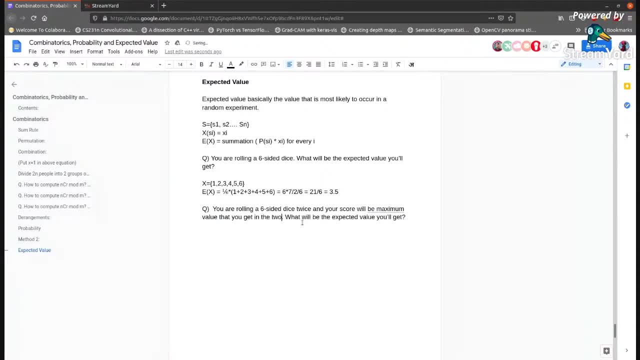 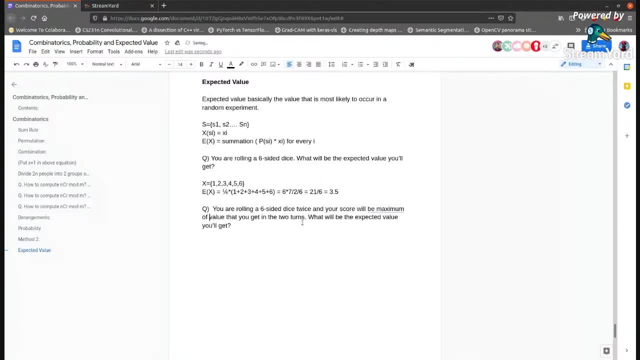 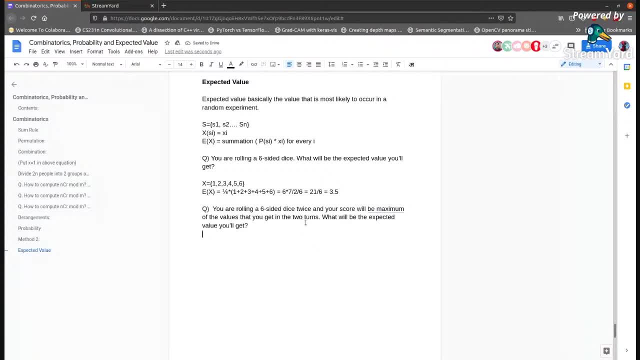 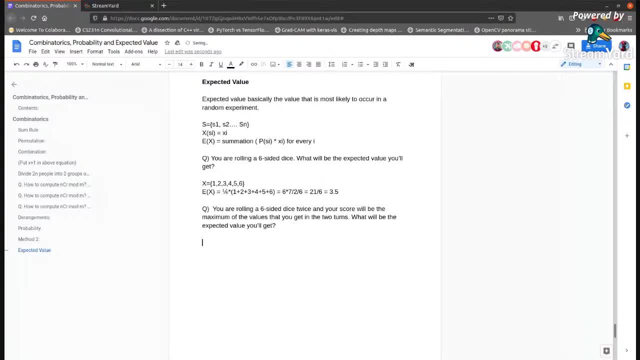 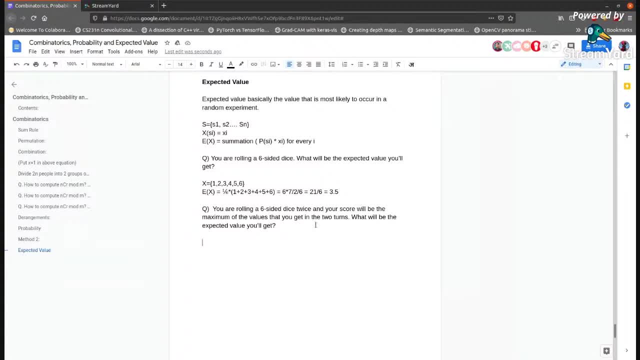 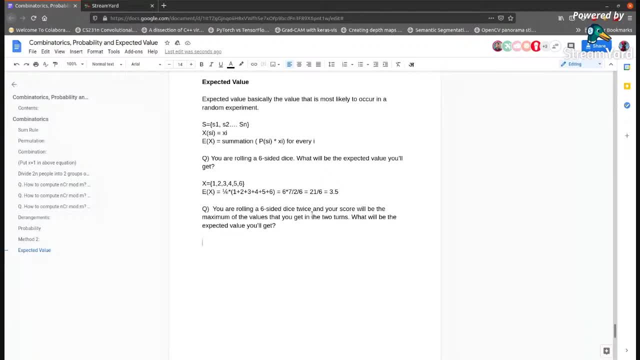 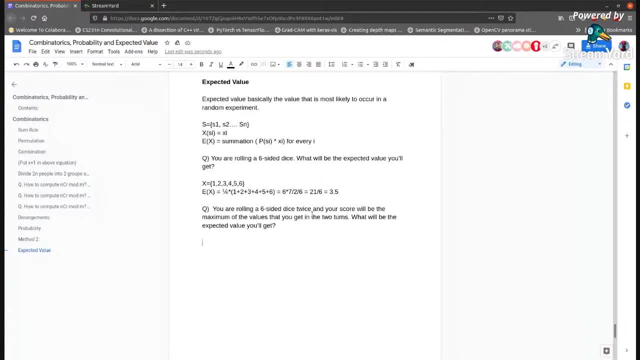 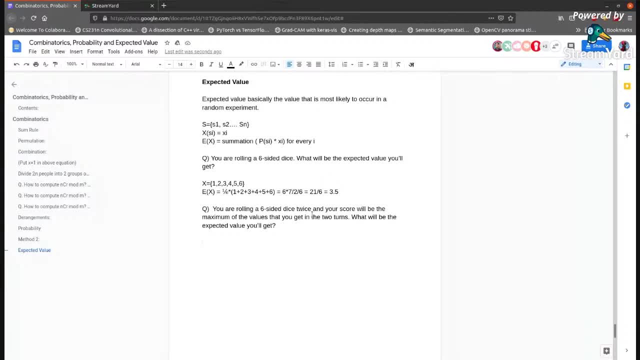 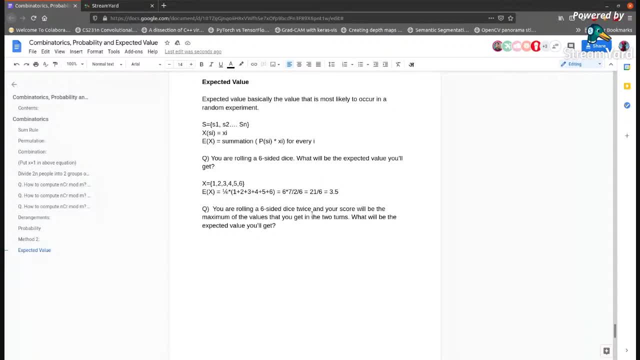 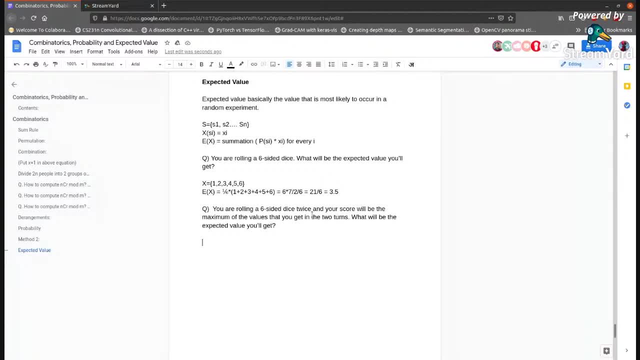 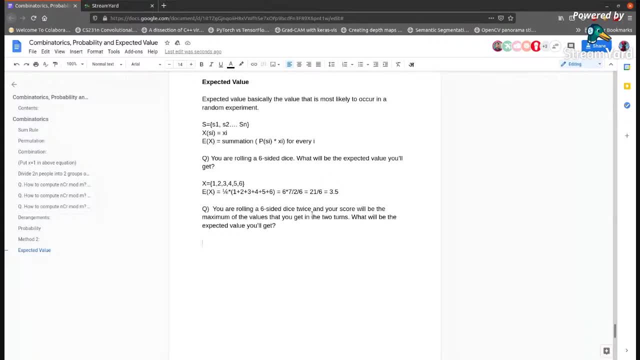 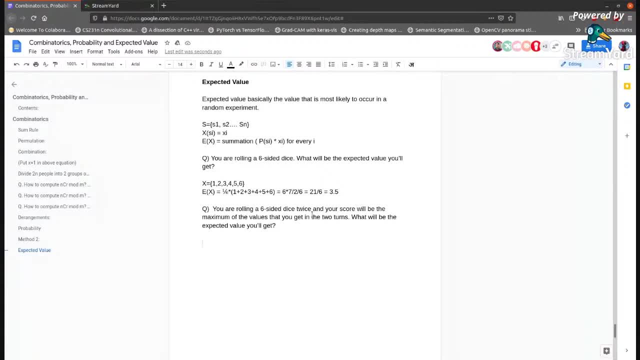 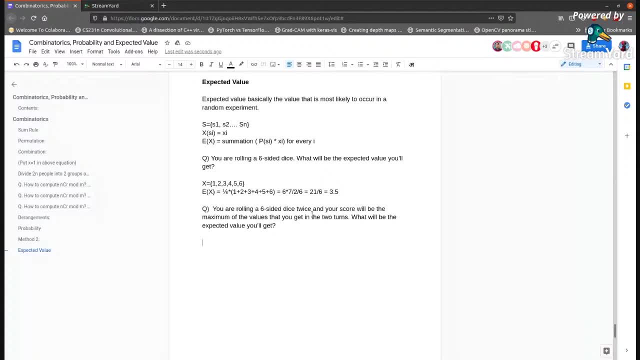 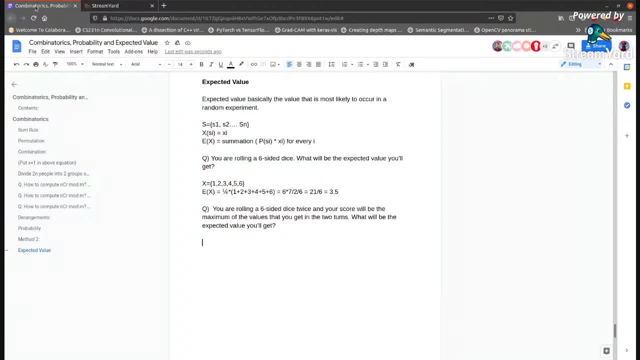 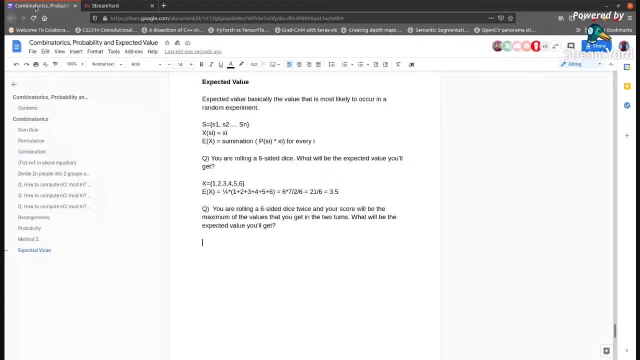 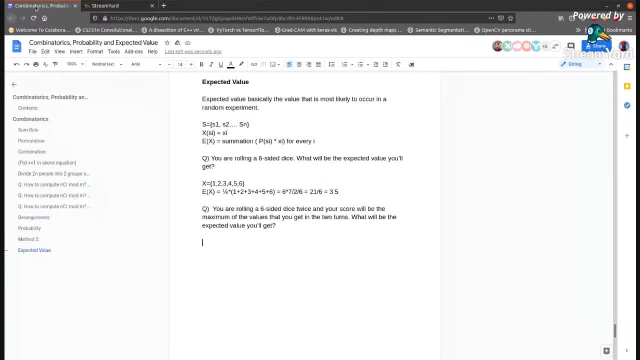 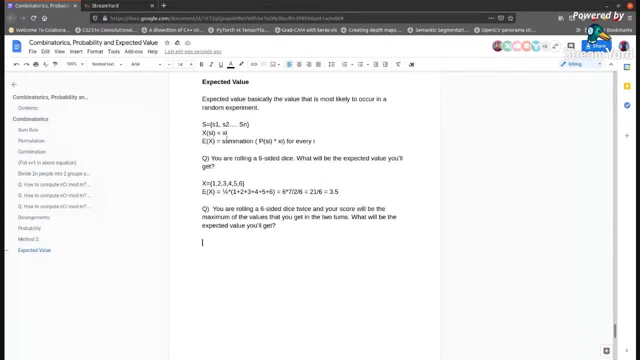 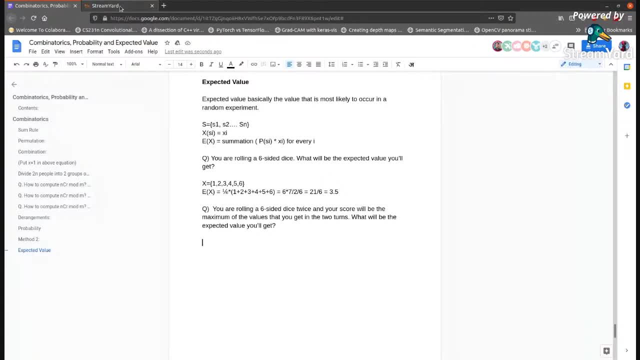 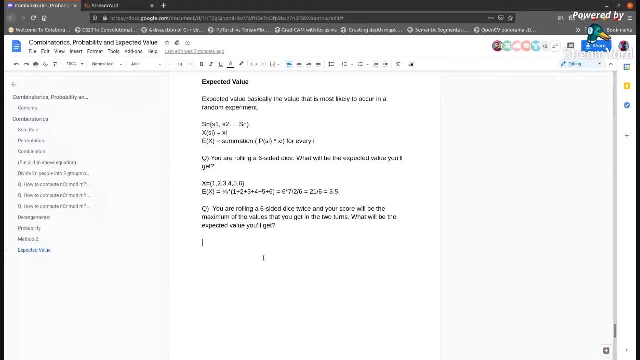 of view. So basically, first we are solving some basic problems by hand, then we will go to CP point of view. So first we will find this P of i, equal to the probability that i is the maximum of two numbers. What will be P of i? Since time is less, I will just proceed with this Probability. 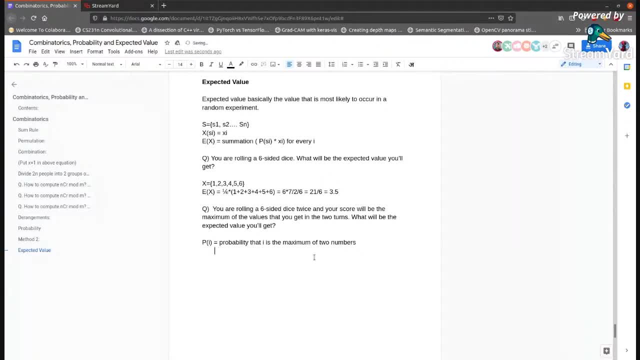 that i is the maximum of two numbers. Now, every turn we can represent like this a pair of numbers: i comma j, And obviously i is the maximum of two numbers. So this is the one of the values. So first, every turn we can represent as i comma j, And for i to be 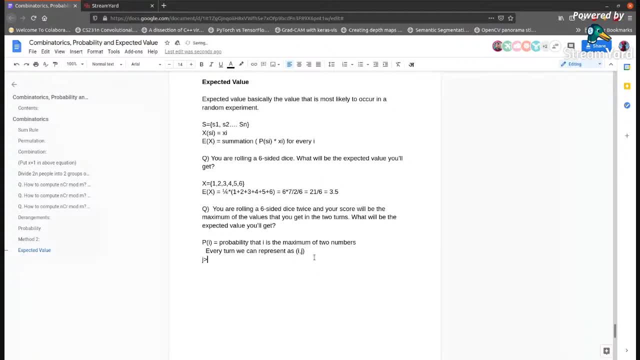 the maximum of two numbers, j should be greater than or equal to- sorry, j should be less than or equal to i. For i to be the maximum of two numbers, j should be greater than or equal to the greater element. j should be less than or equal to i. Let's consider this. 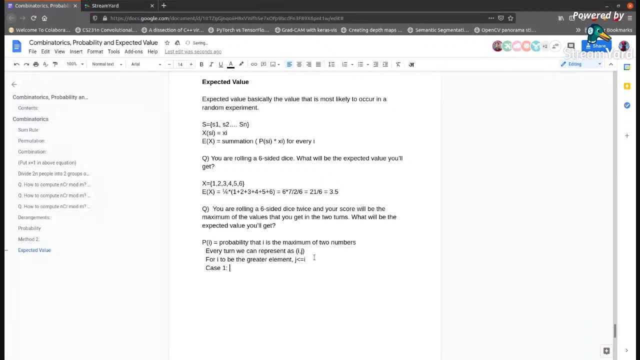 case 1., That is j equal to i case. This case there is exactly one value, one way. And case 2., That will be j is less than i. This will be two times i minus 1.. Because i comma j and. 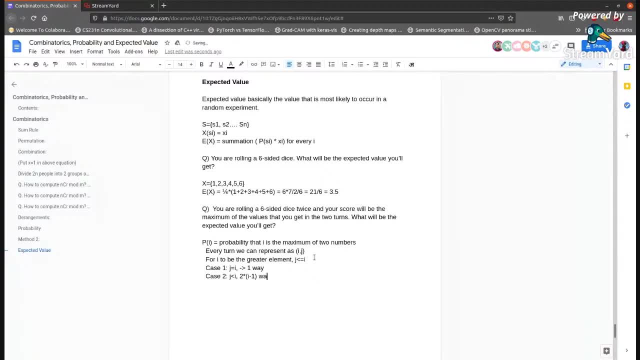 j comma i. both are different, So totally P of i will be equal to number of favorable outcomes. That will be 2 into i minus 1 plus 1.. This you can write it as directly: 2 into i minus 1.. 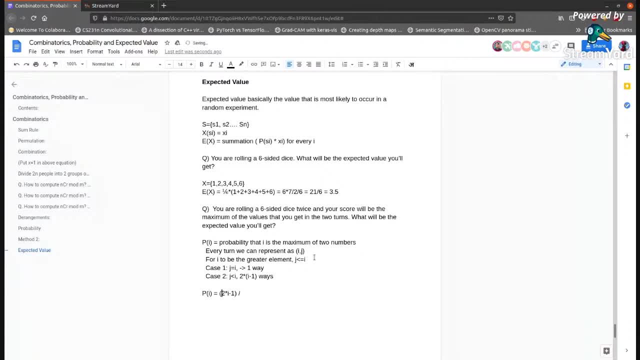 Divided by total number of outcomes is 36.. So our expected value That will be equal to summation of 2 into i minus 1 by 36 into i. If you take 36 into i, you can write it as 36 outside. It will be 1 by 36 into summation of 2 into 2 into i square minus i. If you 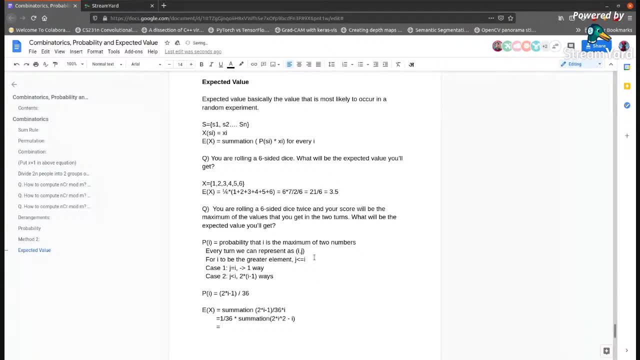 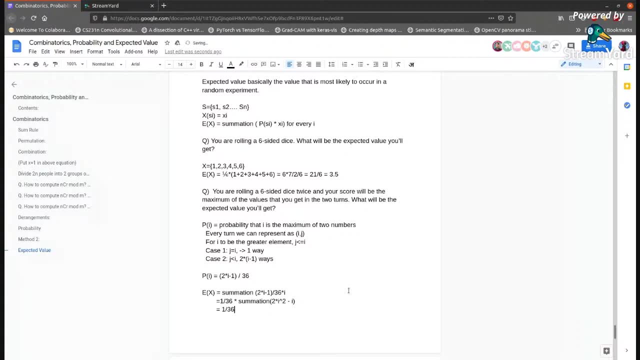 simplify this. it will be the answer: 1 by 36 into 2 into some other value. So you can write the sum of first 6 squares That will be 6 into 7 into 13 by 6. It should be 7 into. 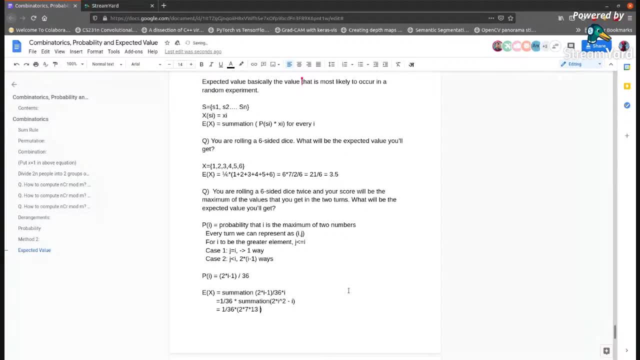 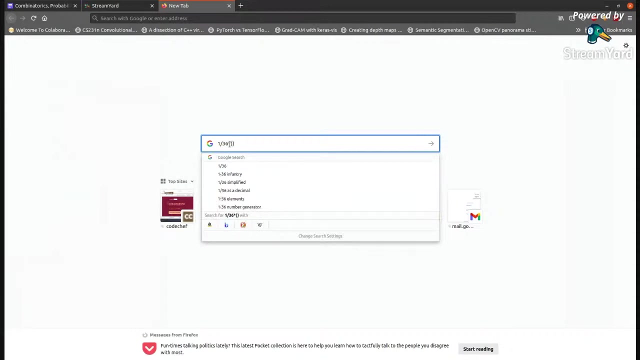 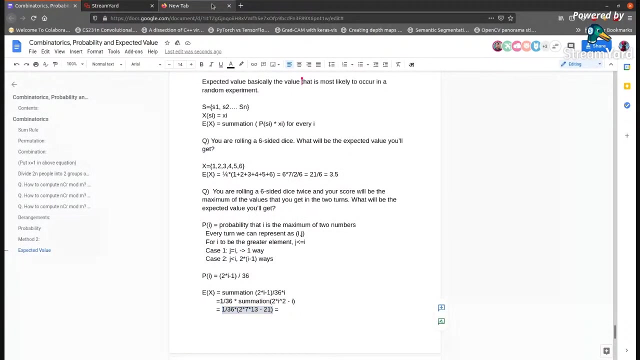 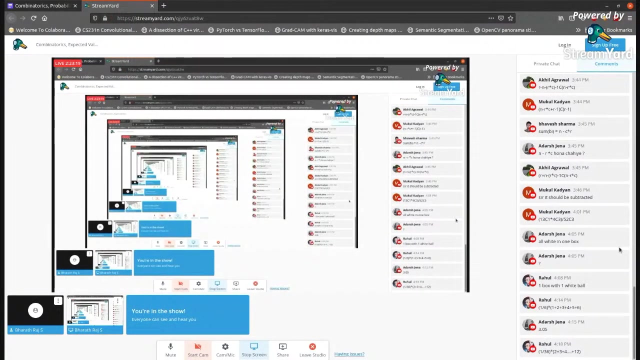 13.. 30 minus sum of first 10 natural numbers, First 6 natural numbers, That will be 21.. And just simplify this, Then you will get the answer. Or I will just do this 1 by 36 into, So this will be your answer. Is this part clear to everyone? Is this part? 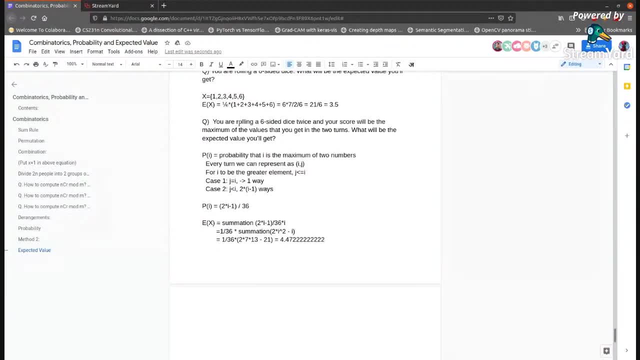 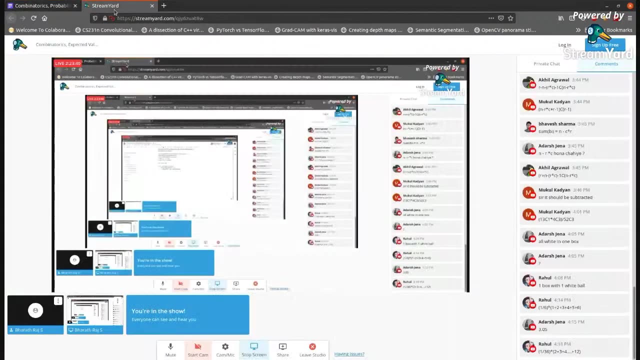 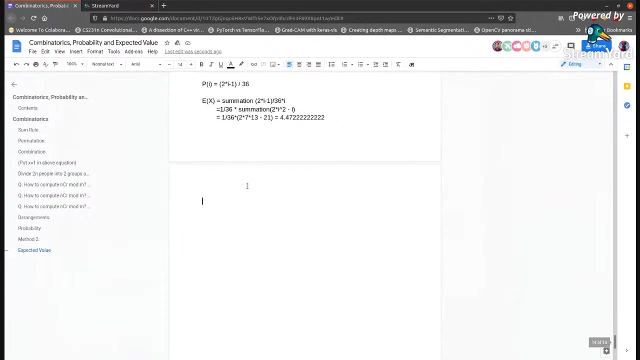 clear to everyone. Yes, The second question. If you have any doubt, just type in the chat, I will see. So I hope there is no doubt till now. So then we will move to the next problem. So the problem is: you are given a sequence of n distinct numbers And you have to choose. 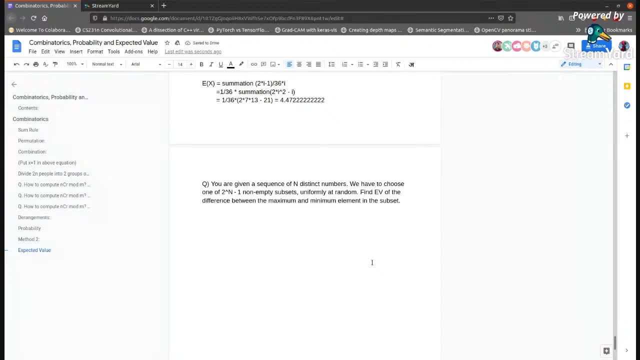 one of the 2 power n minus 1 non-empty subsets uniformly at random. Uniformly at random means the probability of choosing any of the non-empty subsets is same. It does not matter which subset you choose. Everything has same probability. Find the expected value of the difference. 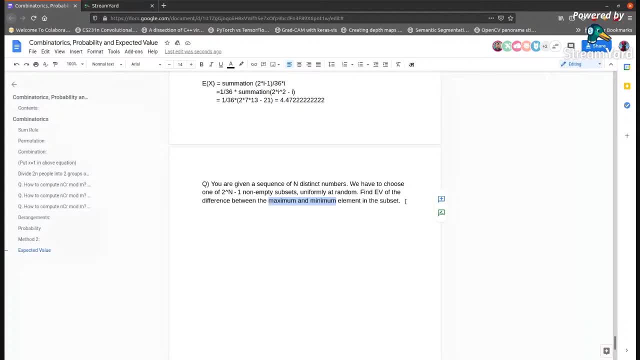 between maximum and minimum element in the subset. If you have any doubt, just type in the chat, Because I don't know whether you are understanding or not, Especially the second problem. So this is the first problem, So this is the second problem. 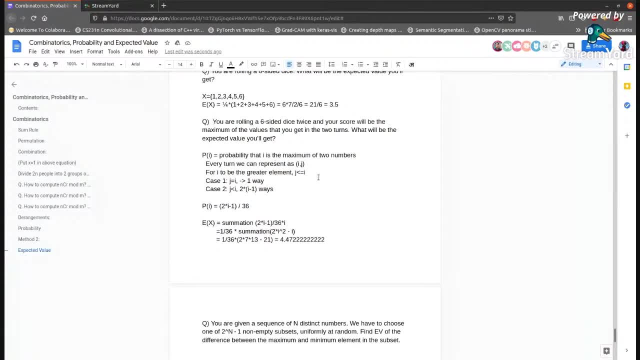 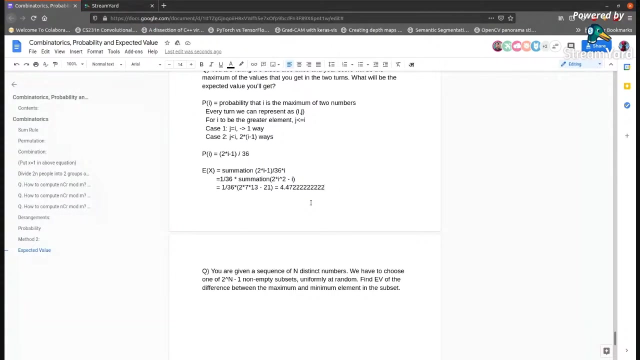 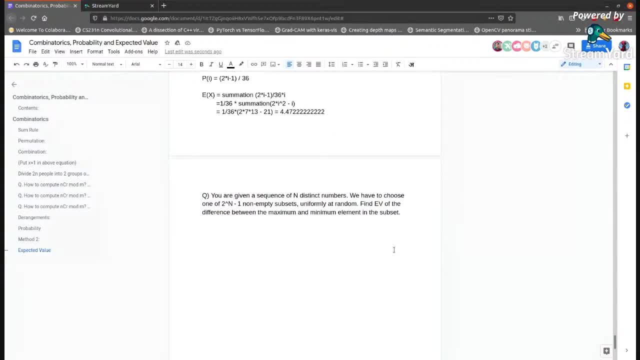 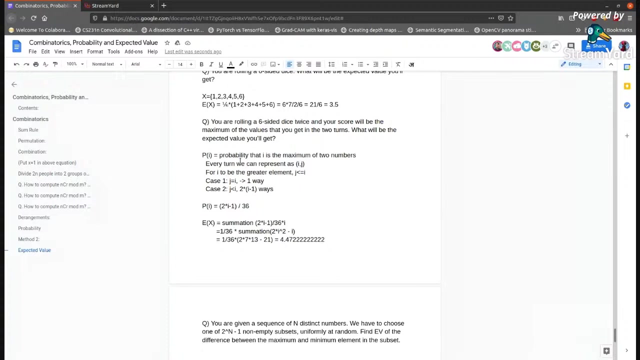 something in the chat, whether the question is clear or not. it didn't think for five minutes. i will give the solution. i will give the solution first and second question. Okay, so first what I'm doing. this: i'm calculating the probability that I use the maximum of. 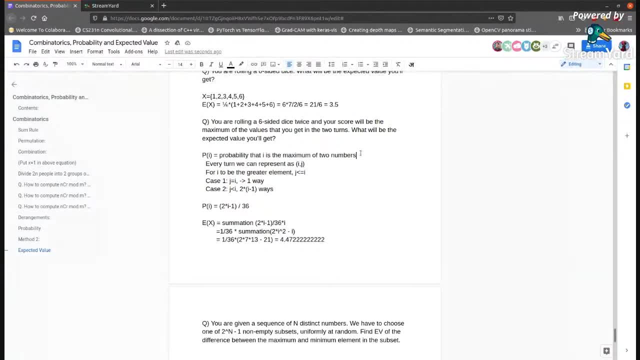 two numbers, And if you see the, every time we'll get two numbers. I come out there that I'm representing- representing as i comma, He's too numbers, and for it to be the greatest element. First I'm thinking: one: is j equal to i? there is exactly one way that is possible. and the next case is j is less than i. 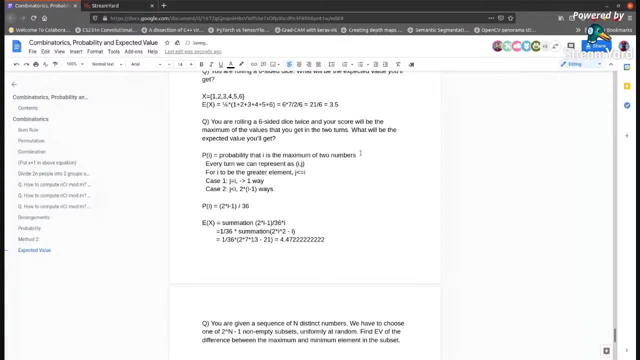 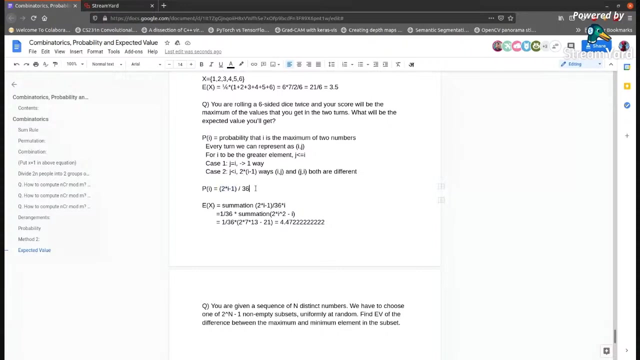 there will be two into i minus one ways, because, uh, i comma j and j comma i both are different. so for that, for that case, i'm multiplying by two and probability is, uh, the favorable outcomes, that will be two into i minus one. divided by total number of outcomes, that is 36, and next is expected value. expected value is probability of. 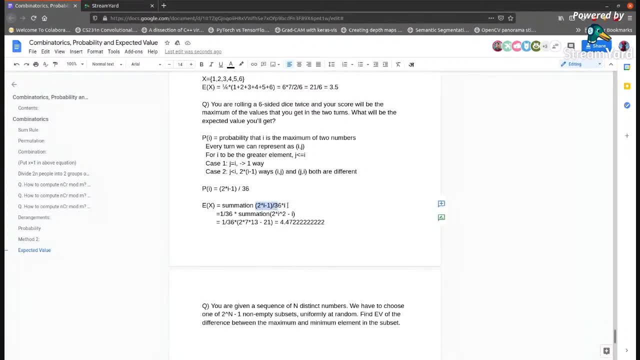 the event times the value associated with it. so probability we have just calculated as two into i minus one by 36 times i, and this i i'm just multiplying inside, so that will become two into i square minus. then after that it's just some summation. 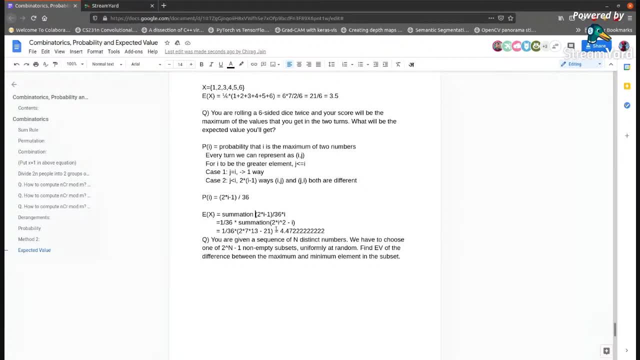 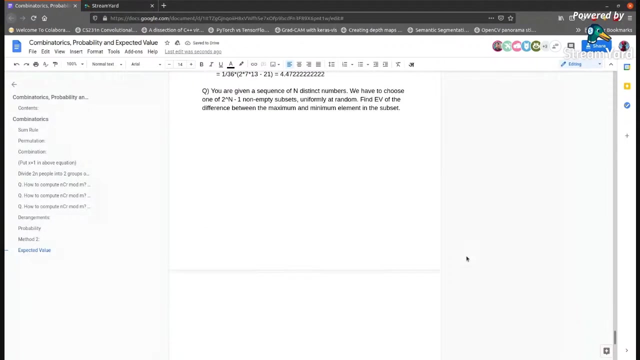 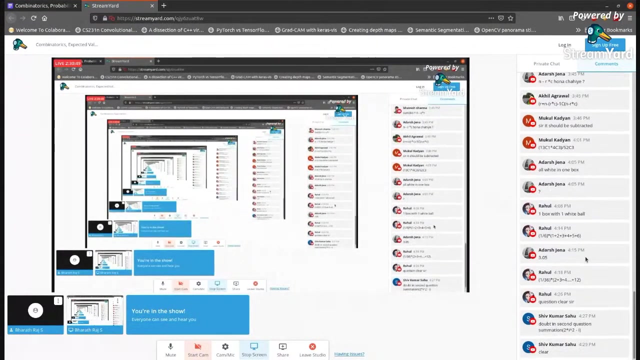 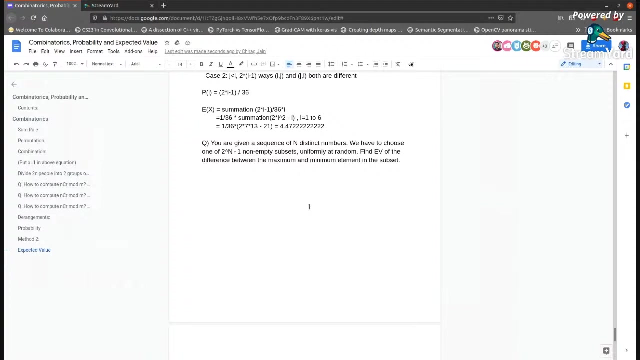 is it clear now? so i equal to one to six. just mentioning i thought it was obvious. no, so so you were j and kos j z Mos v, Amen, Amen. So in this particular problem, if we approach the problem similar to the previous two problems, 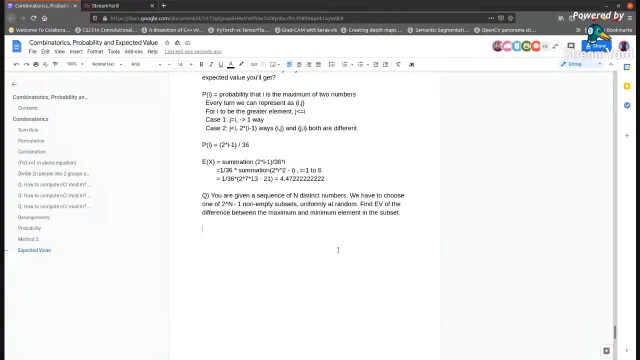 that is probability, that max minus min value is something, and times max minus min value, that is as per the definition, then it is very difficult to say the answer. So for this, what we'll do is we will find the contribution given by each element. 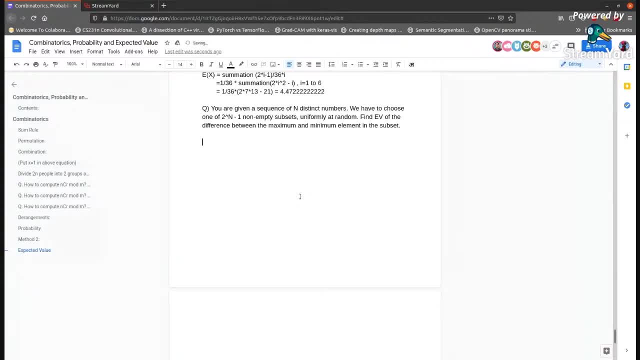 So, for example, let's So first before this, for simplicity, let's sort, Sort the given array And after sorting, the array becomes something like this: A0,- sorry- A1,, A2, so on Here. 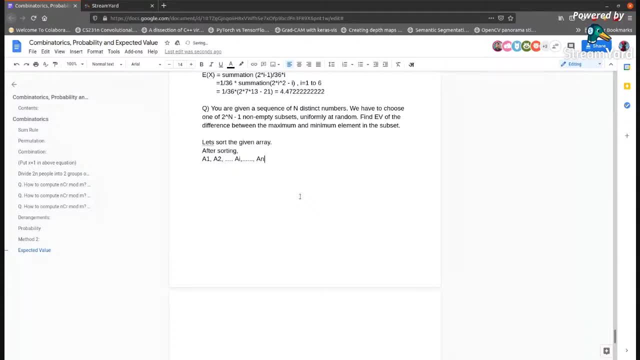 And so on till A1.. This will be your array after sorting, And let's take some element. Let's consider an element: Ai. So what will be the contribution of Ai? If you look up on the contribution of Ai, If in some subset 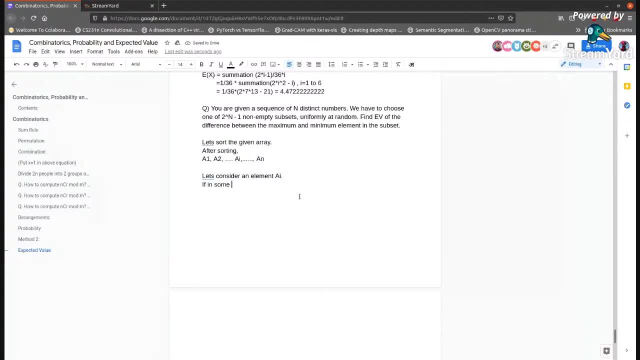 Some subset. Subset here refers to non-empty subsets. Okay, In some non-empty subset Ai is the maximum element, Then its contribution: A1. A2., A3. A4., A5. A6., A7., A8.. 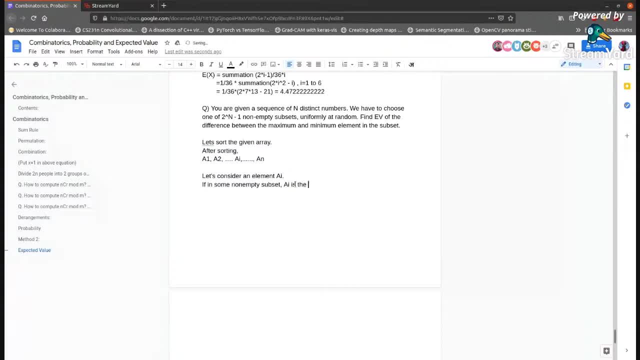 A9., A10., A11., A11., A12., A13., A14., A15., A16., A16., A17., A17., A18., A19., A20., A21., A22. 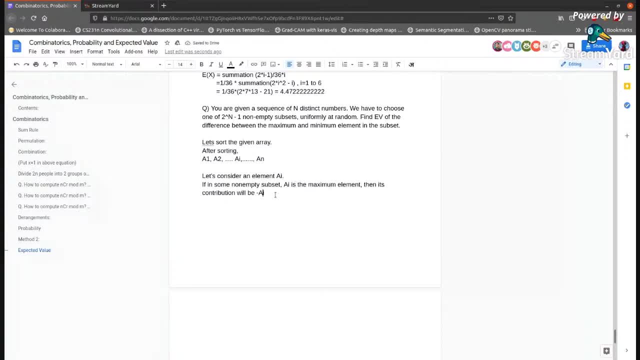 A23., A24.. A25., A26., A27., A28., A29., A30., A31., A32., A33., A34., A35., A36., A36., A37., A38. A39., A41., A42., A43., A44., A45., A46., A47., A48., A49., A50., A51., A52., A52., A53., A54., A55. 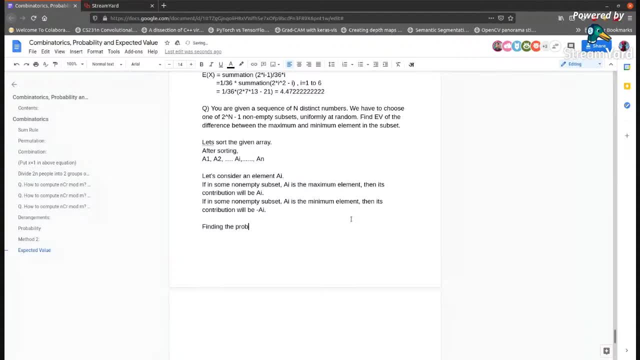 A56., A56., A57., A58., A59., A59., A60., A61., A62., A62., A63., A64., A65., A67., A68., A68., A69. 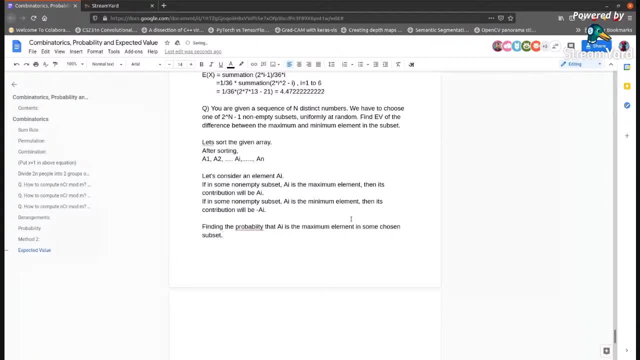 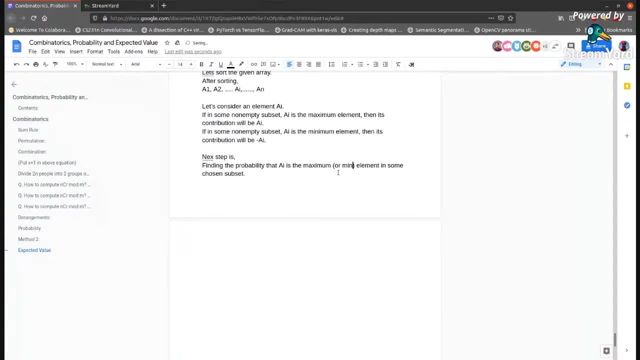 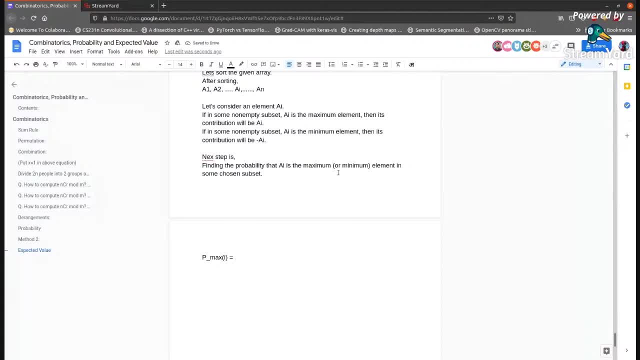 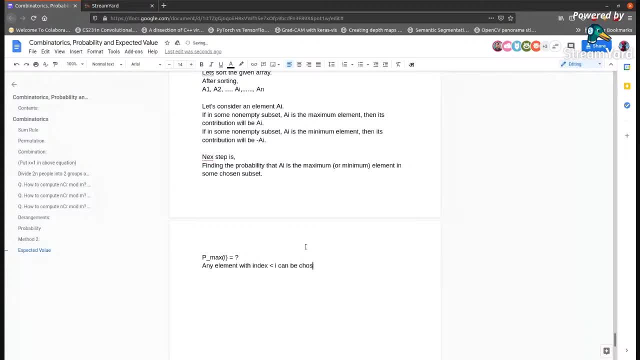 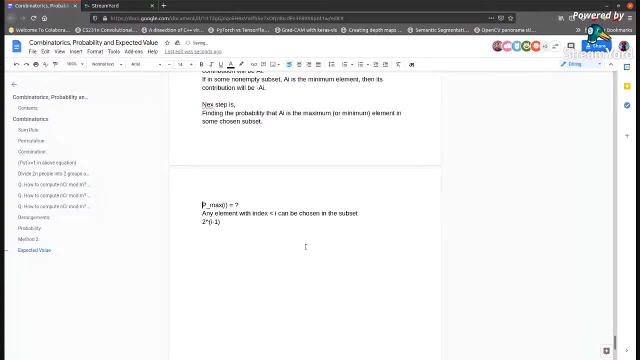 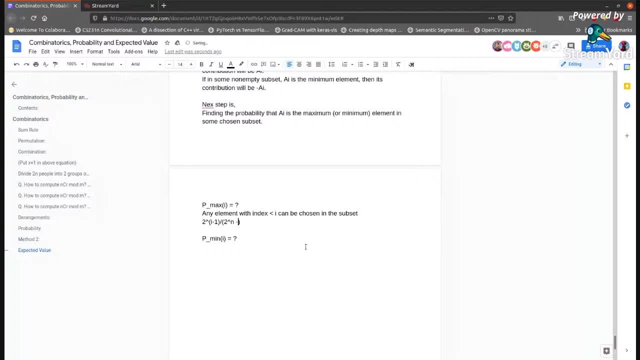 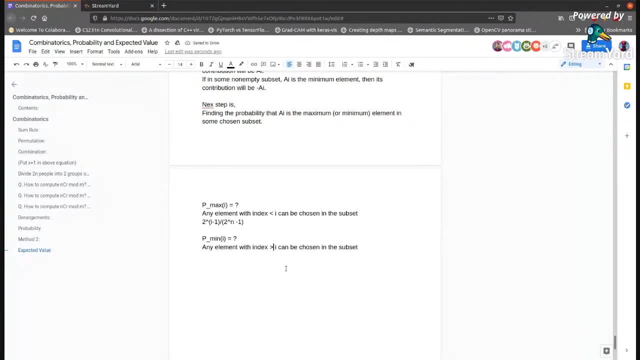 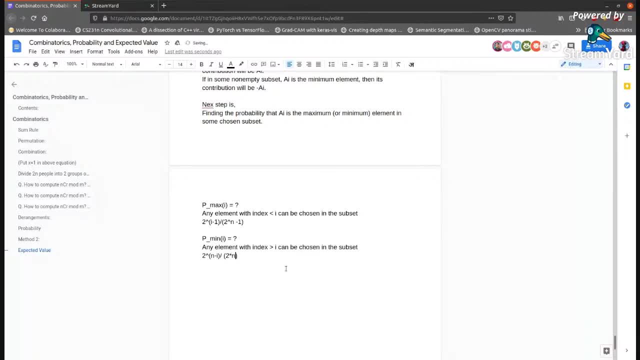 A74.. A74.. 2 power: n minus 1. and so for the answer what we'll do is for int. i equal to 1 plus n equal to n. i plus plus. to the answer we'll add this value into a of i and to the answer we'll: 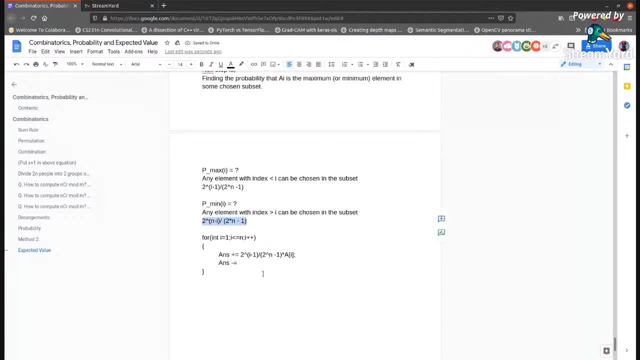 subtract this value. So just don't worry about the overflow and all. the idea is just to teach the concept, not thinking about overflows and all. So if you have any doubt in this, you can ask specifically at which point you have doubt. How do you write any element with index greater than i or less than i in the two cases? 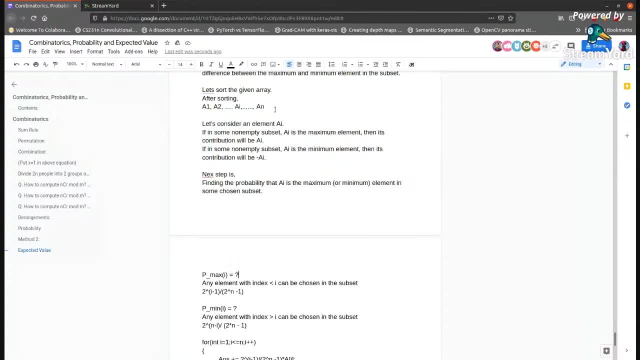 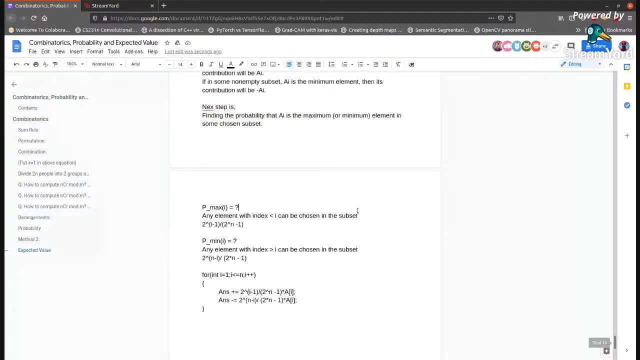 So first we are considering the contribution of the element right. So in some chosen subset, if a is the minimum element, Then we'll subtract a? i, and for that we have to know the number of subsets where a i is the maximum or minimum element. 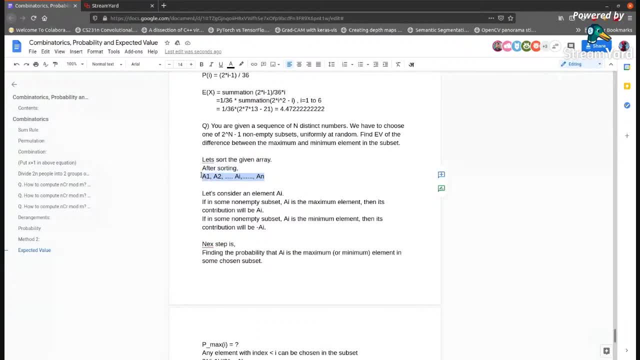 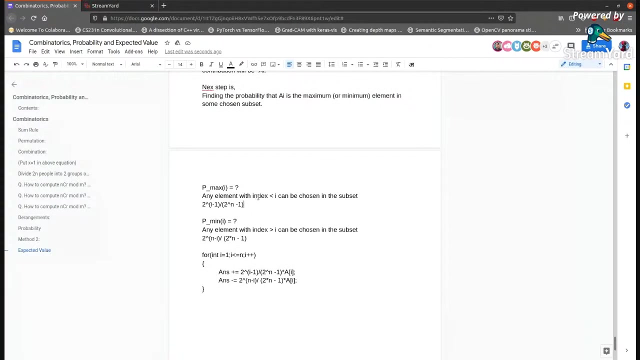 Since we sorted here already a1 to a n, any element with index less than i that will be smaller than a i and any element with index greater than i that will be bigger than a i, because every element is distinct according to the problem. We'll see these changes in the next lesson. 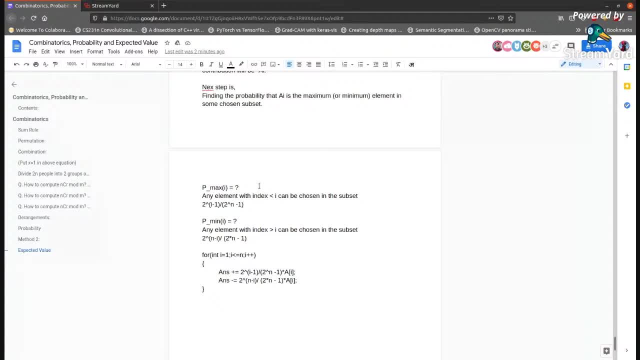 Is it clear or So any other doubt? you can also point at which point you are having doubt. Ok, Thanks See you once again. Hmmm, Bye, Because this trick is very commonly used. contribution to the answer. I'll wait for 2 more minutes. if you have any doubts, you can ask, otherwise I'll go for. 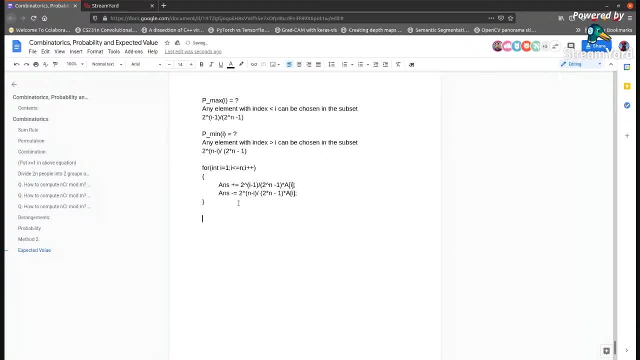 the next problem. Meanwhile I write the same thing. Next question: you are given bits of M colors, Colors And 43 points. Okay, For each color. for each color, there are infinite number of bits and you have to make a necklace. 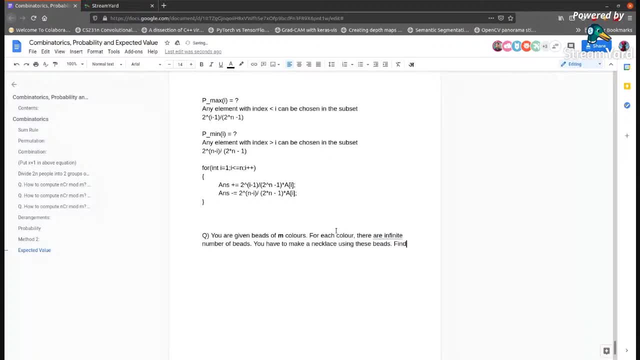 using these bits, Find the expected number of bits. Find the expected number of distinct colors in the necklace. So if the question is clear, just type something in the chat. if it's unclear, put it away. Okay, Number of bits. 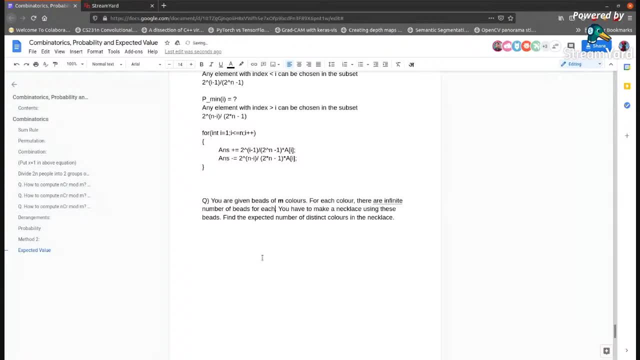 Okay, Number of bits For each color. You have to make the necklace of M bits, Sorry. So basically you are given M colors of bits, Right? Okay, colors of beads, and using those beads we have to make a necklace. and what will be? 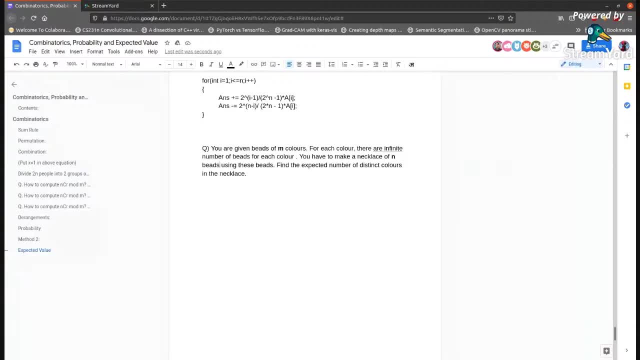 the expected number of distinct colors in this necklace. so for example, n equal to 3 and n equal to 3. suppose if your necklace has 1,, 2, 3, then it is having three distinct colors. like that you have to find the find for all possible. 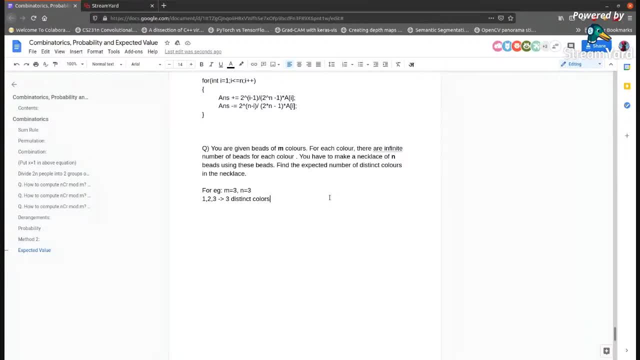 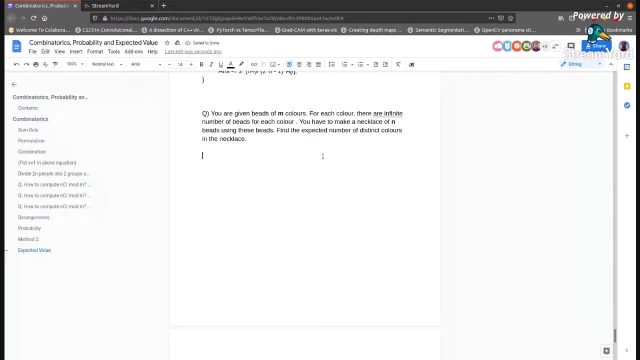 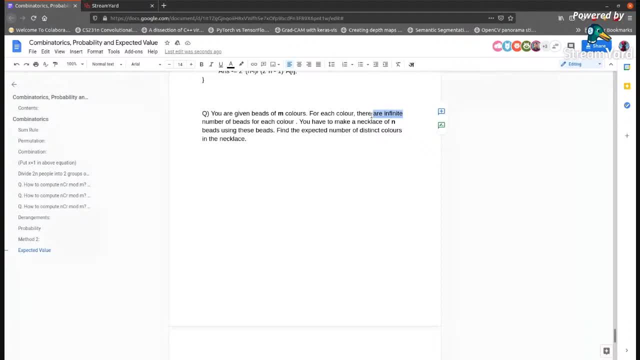 so then my just presented with some, but so, so, so, so, so so, of each color, each question is fine, only so. infinite number of beats basically means: suppose you take some bead. suppose, for example, at some point you take a bead of color 1 and the next time the probability of taking that color, one that will not change. that is the basic. 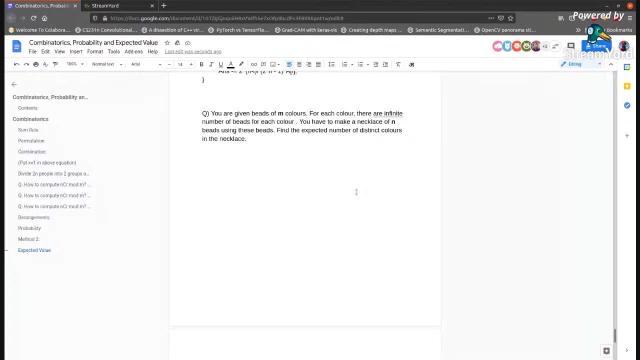 idea behind infinity, meaning every time you are choosing a color, i that will be independent. no, this will not be the same if we have no. if we had n, which means every time the probability will change right. so, for example, the first time you are taking, the probability will be one by n. 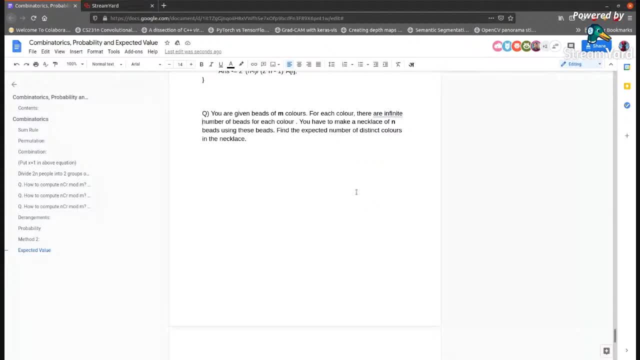 and after that, the second time it will be one by n minus one, like that. you add another one, a plus one minus one, or even a one to minus one of your Gentiles, and you add one coming out of a third. you take a plus four minus zero and that's the. 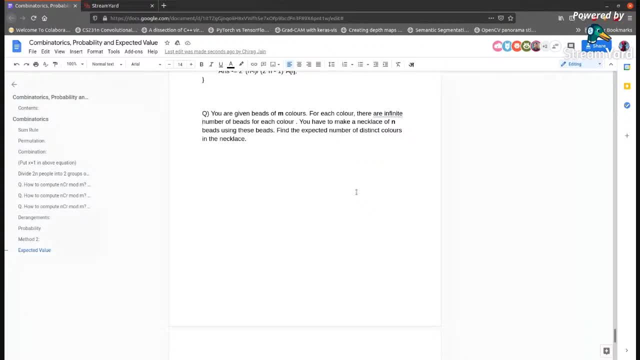 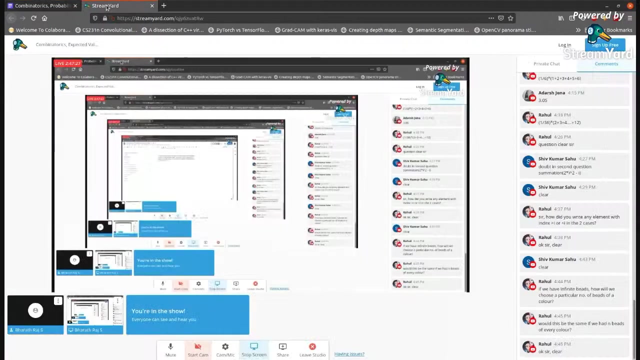 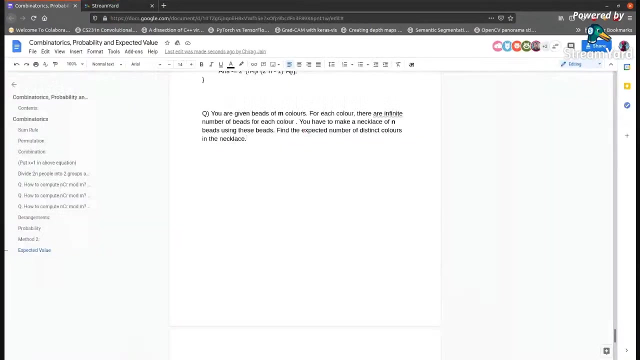 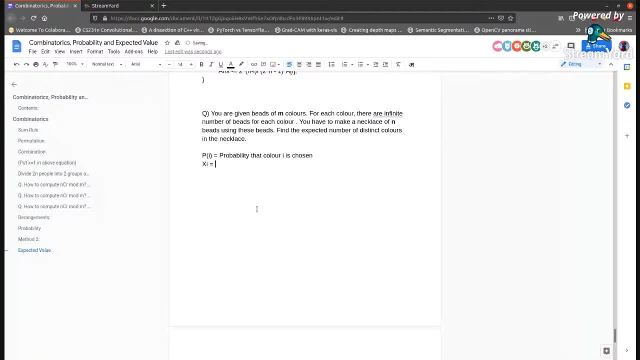 And what will be the value associated with this xi? This will be 0 if Color i is not chosen And 1 if color i is chosen. So now the problem actually reduces to this 0, multiplying anything with 0 is going to give us 0. 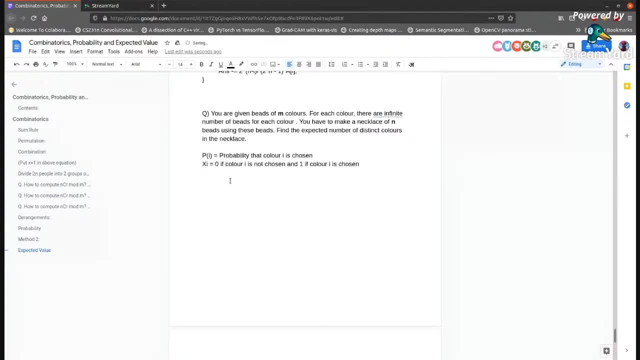 So problem is now reduced to: expected value of x is equal to Summation of P of i And by this definition, this infinite number of beads, we know that P of i equal to same for all i. Everything is equally likely to occur. 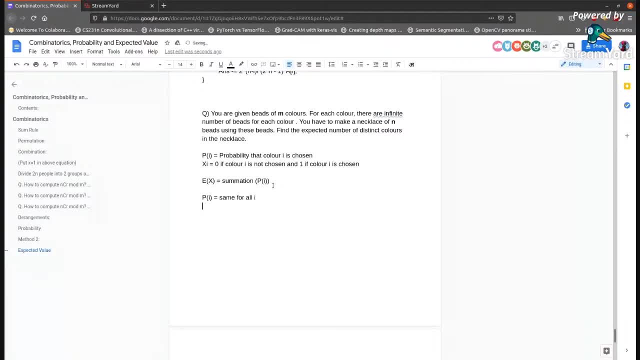 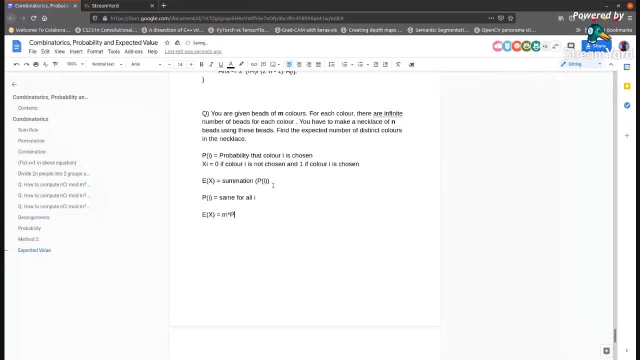 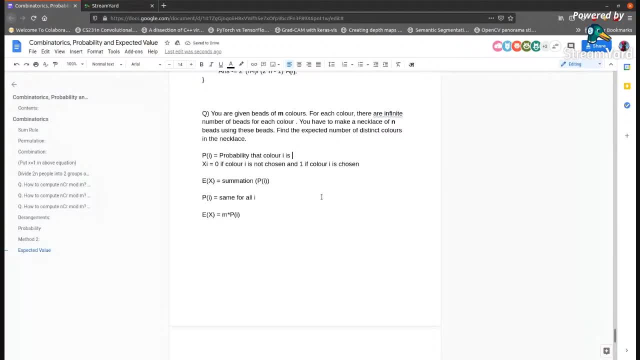 Oh sorry, This is not. i is chosen Probability that color i is present in the necklace And So probability that color i is present. color i is present means it occurs at least once. So this P of i you can easily write like this: 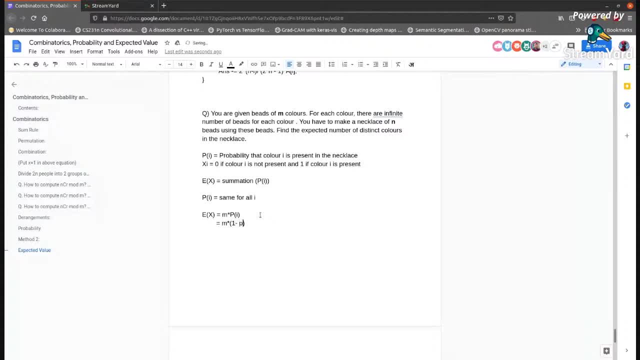 M into 1 minus P dash of i, That is probability that color i is not chosen even once. So what will that be? M into 1 minus P dash of i? That is probability that color i is not chosen even once. 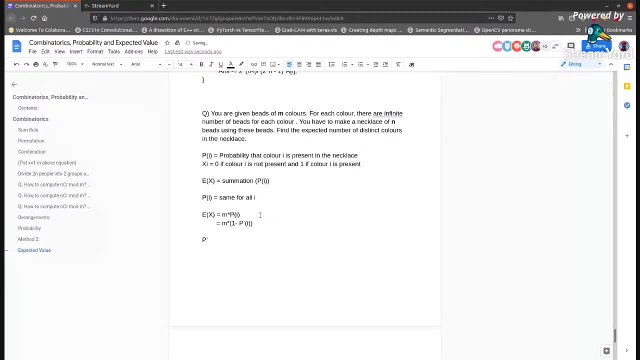 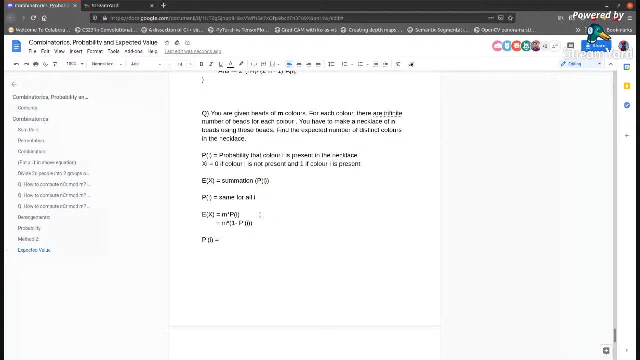 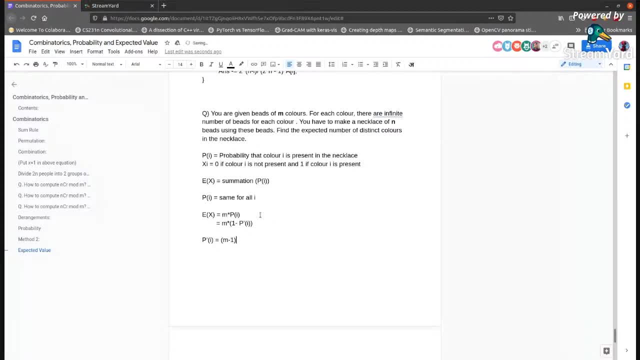 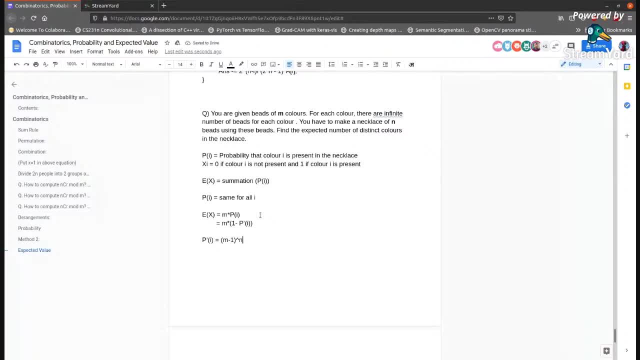 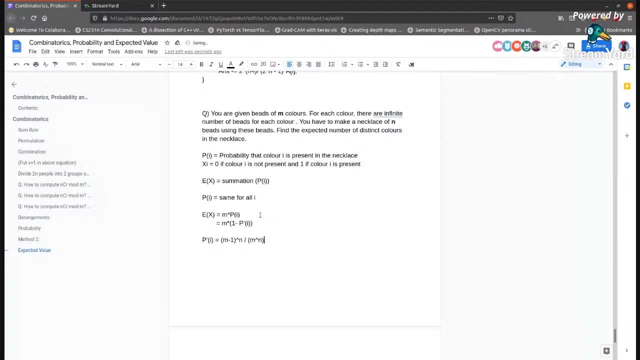 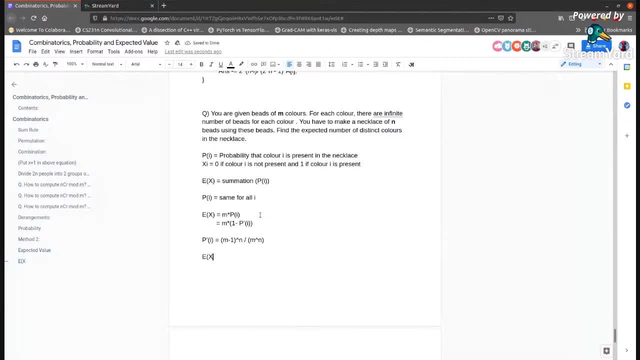 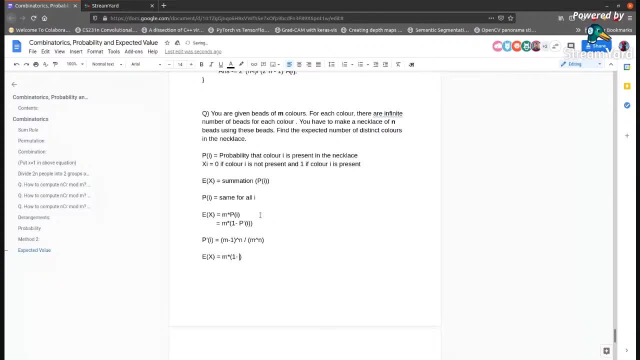 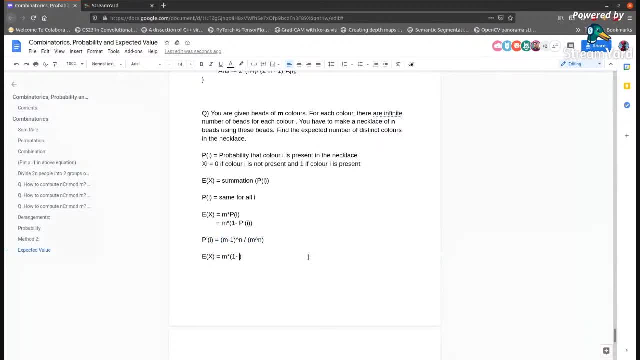 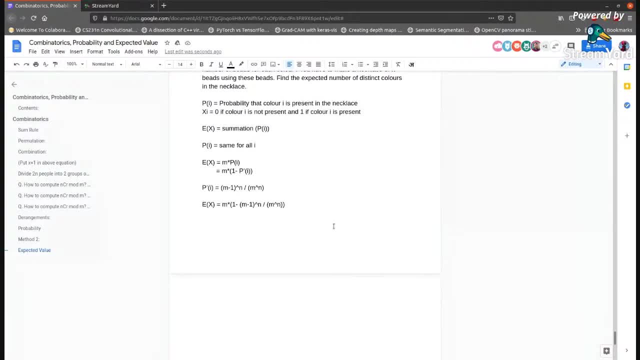 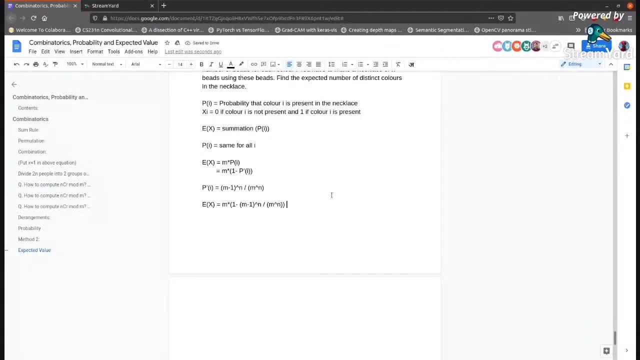 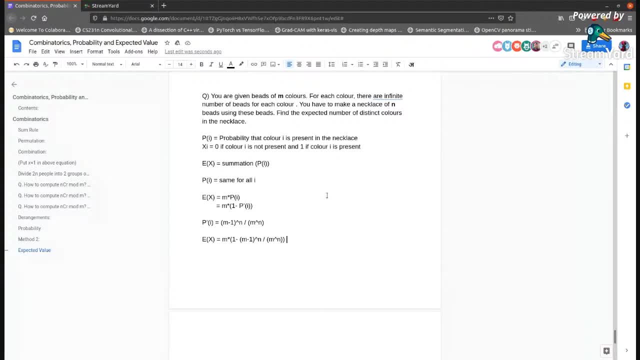 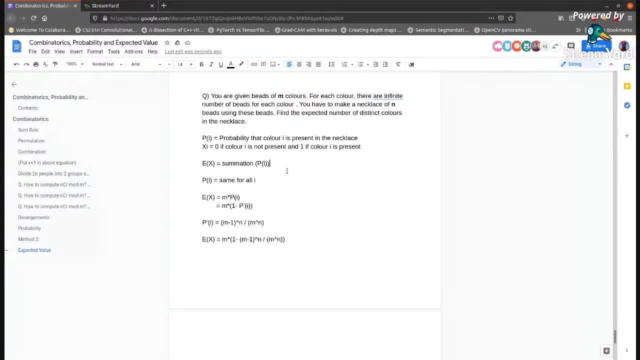 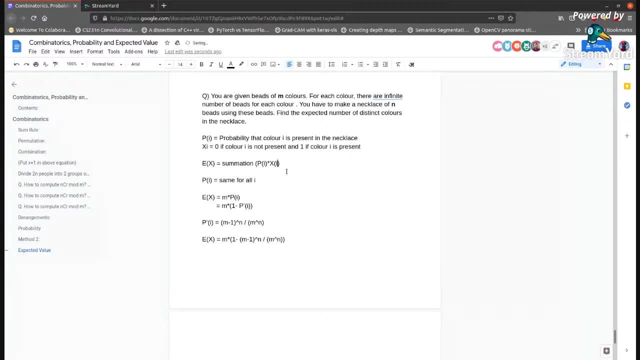 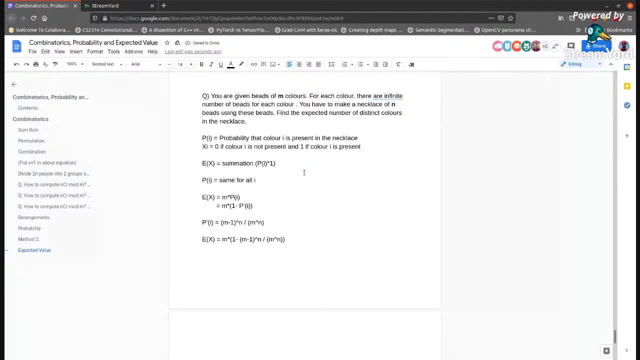 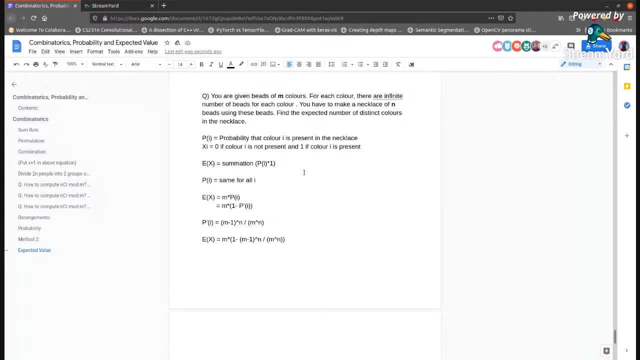 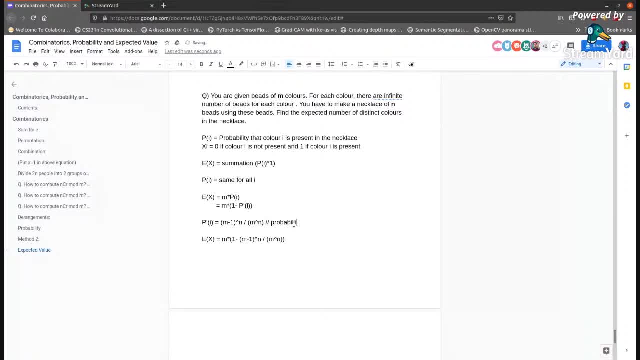 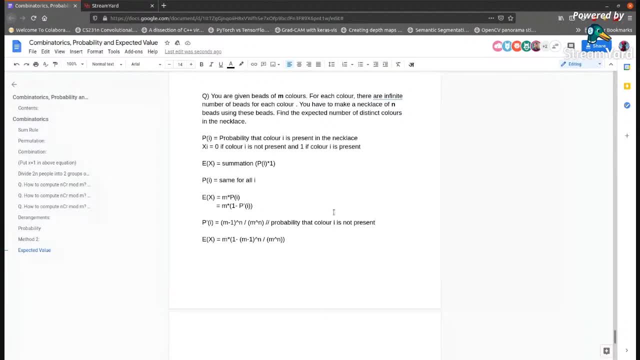 So what will that be? M into 1 minus P dash of i, That is probability, that color i is not chosen even once. So what will that be? M? is this clear for everyone, then? i don't think so. if there is any doubt, no, please ask in chat, because next problem will be difficult. 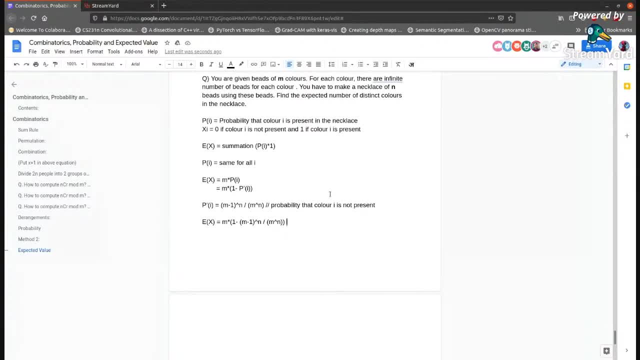 this is sort of basic thing, classical problem. you have any doubt, just type in chat. i'll explain one more time. so okay, so then i'll go to the next problem. next problem is you are given a random number generator that generates an integer from one to n. 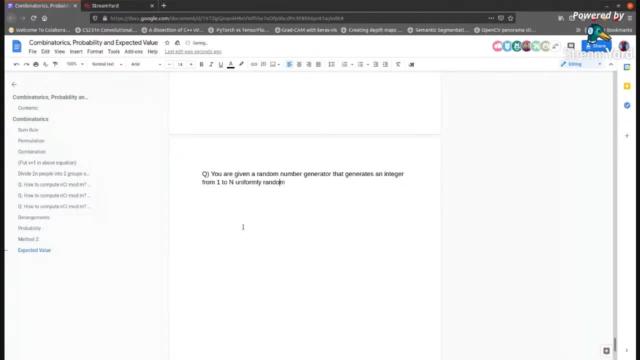 uniformly random, uniformly at random number. find the at each term. so basically at every time it will generate some random number. you have to find the expected. Let's put the number of turns needed to needed such that k distinct elements have to be generated and let k less than or equal to 10 power 5.. 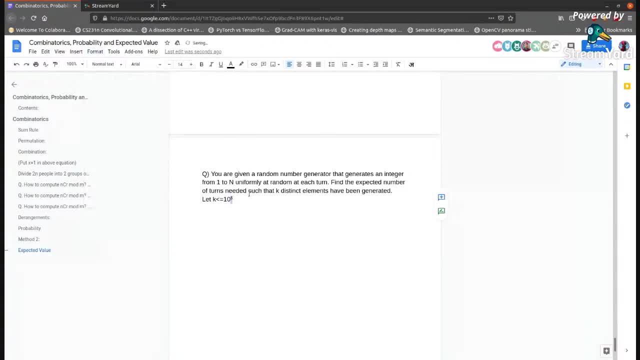 So let's put k less than or equal to 10 power 5.. Now just I will refine this easier to understand here. it will stop generating once k distinct elements have been generated. find the expected number of turns. Okay, This problem was asked in coordination coding round, actually. 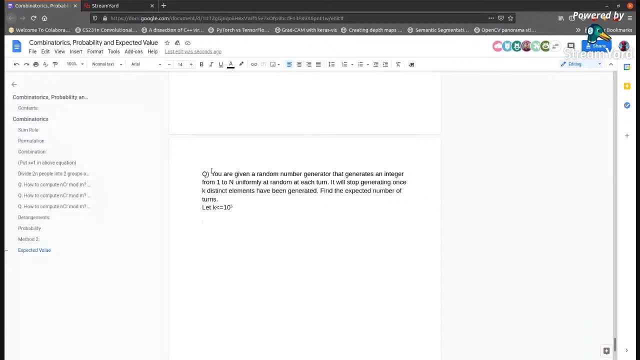 So, if you have any, if the question is clear or not, just type it in the chat, whether the question is clear or not. Thank everybody. Thank you, This is Joe. this is Nopeiladı. Thank you everyone. 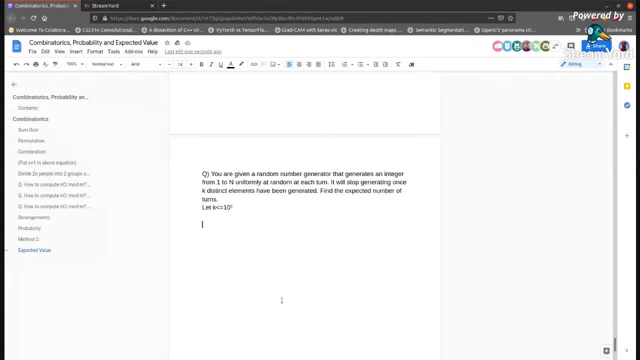 Thank you again. Thank you Very good, All right. Good morning. This is Brian from the Hastrell清掛网. Sorry for interrupting, asking for two more minutes today, and thank you everybody, That's fine. 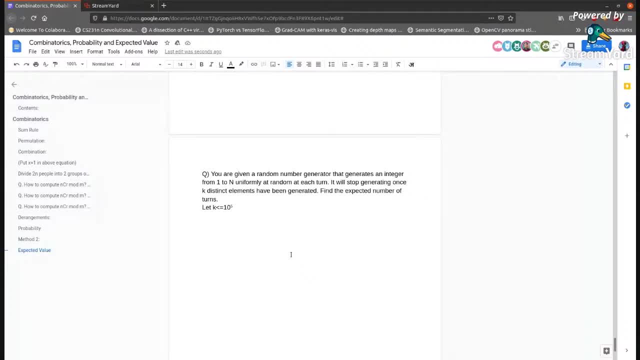 Bye, Bye-bye. Just type in the chat whether it is clear or not. If it is clear or not, then it is clear. Thank you, Thank you, Thank you. I will give you 10 minutes for this problem. I will give you the answer at 5.10.. 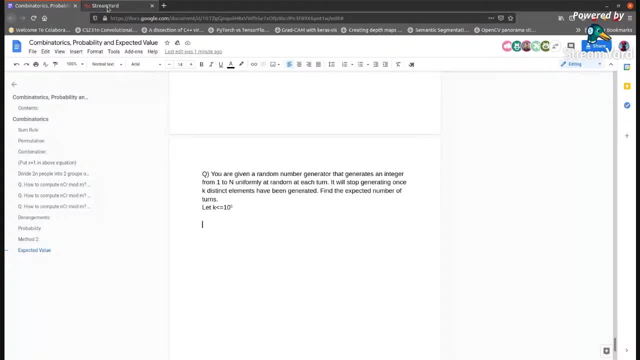 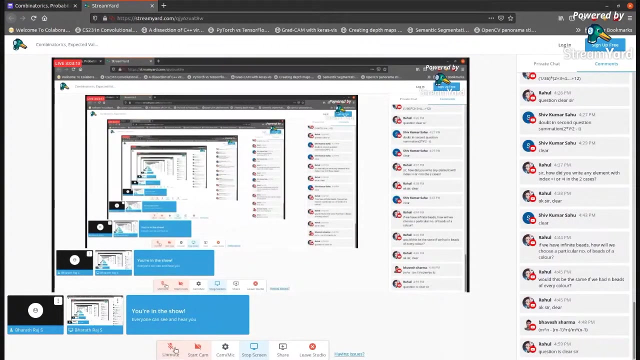 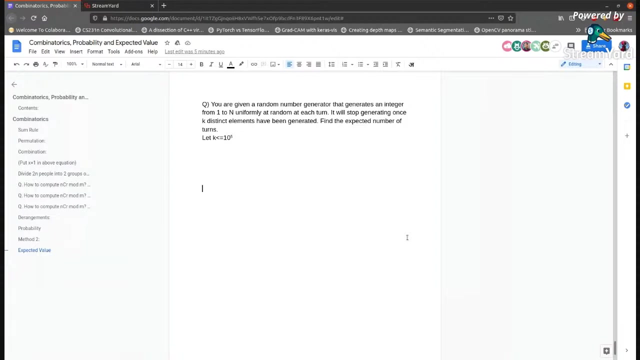 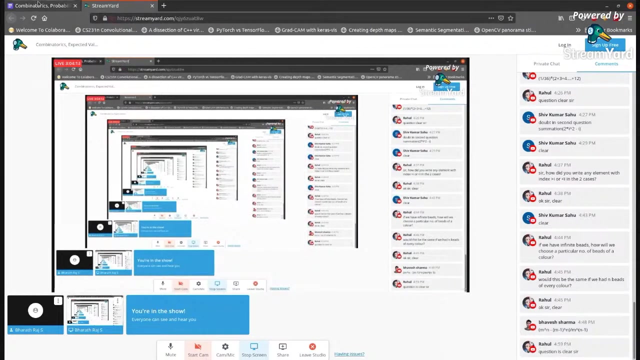 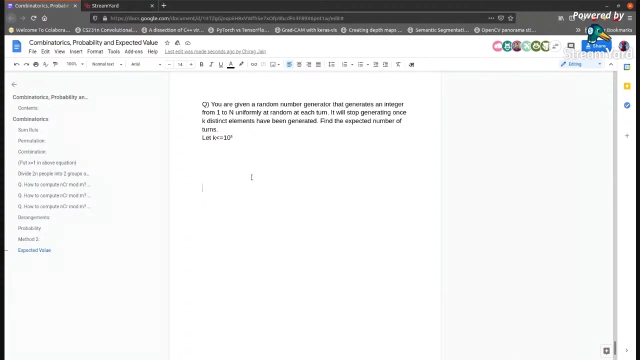 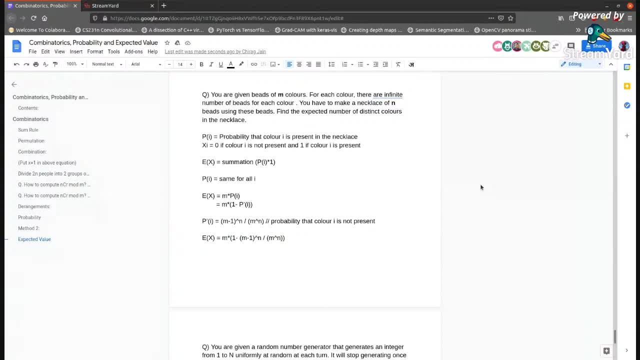 the formula that I discussed earlier: expected values, probability times that value, summation of that here. let's take a different approach here. basically, we use dynamic programming and state will be: BP of I equal to expected number of turns needed to reach a distinct elements, such that we have I distinct. 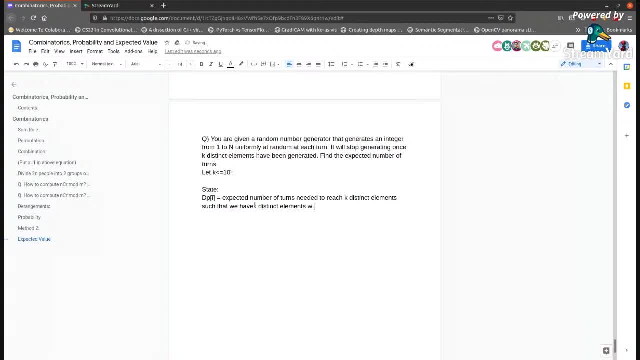 elements with us. you know I distinct elements right now. so what will be the base case? so if you have understood the state, then you can say this: what will be the value of PP, of K? you type in the chat you or is the DP state unclear to you? that also you can type in the chat. I will explain. 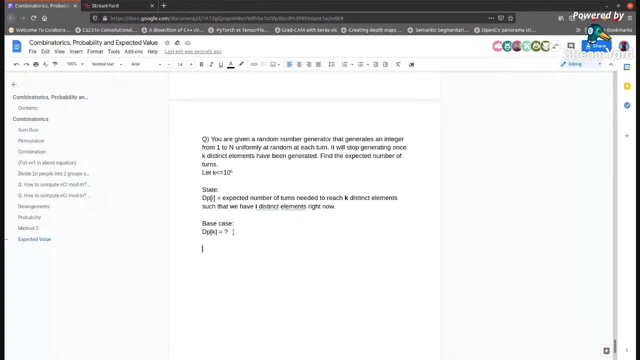 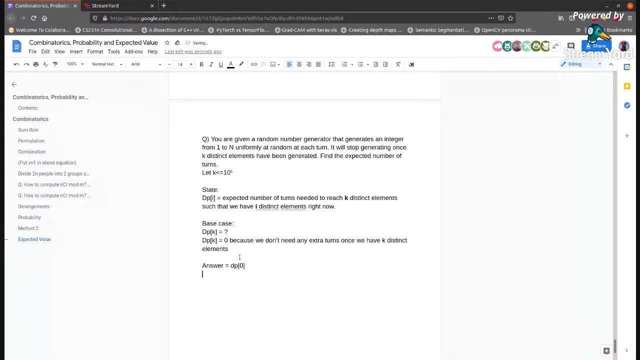 the number of moves. uh, needed to reach k distinct elements in expected number of moves. so let's see the transition. suppose current state is dp of i, then case one, the chosen element is from one of the i distinct elements already chosen. then in this case we will again move to this dp of i state and next is case two, the chosen element. 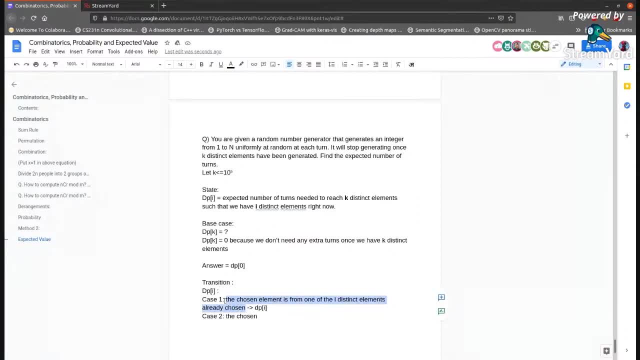 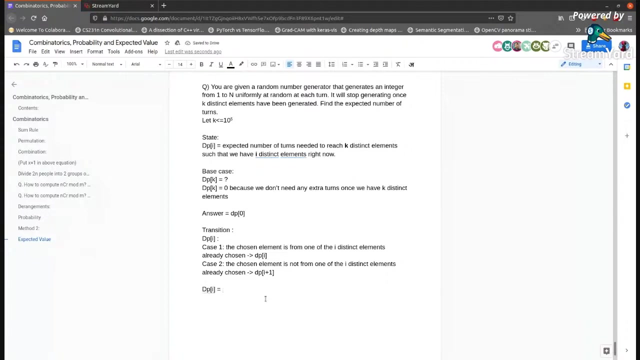 is not from the i distinct elements already chosen, then in this case we will move to dp of i plus one. so basically what i mean is dp of i will be equal to one plus, because we have to make one more, one extra more anyway into dp of. 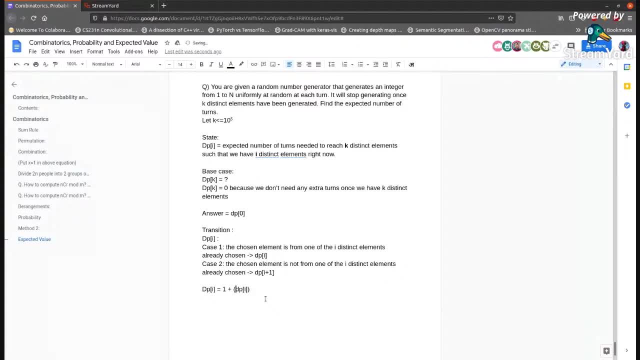 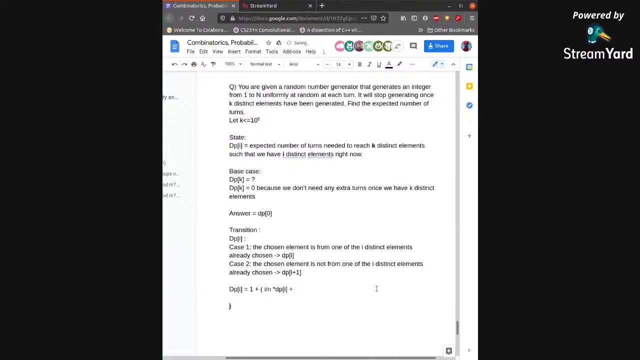 i into the probability of this happening is one by i. so we have to make one more, one extra more anyway into dp of i into the probability of this happening is one by i. Sorry, sorry, Hopefully this happens. i by n into plus n minus i, That is not these i. 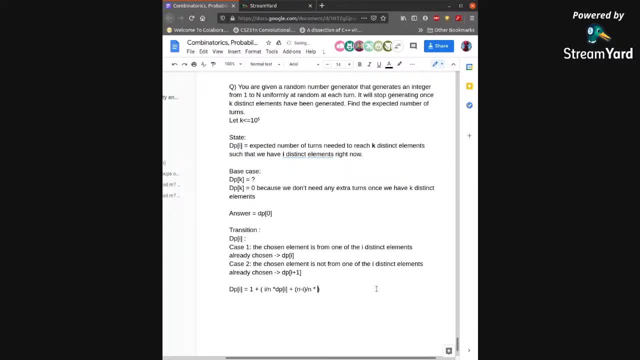 elements By n into dp of i plus 1. Because once you chose this element, run of the element from the i distinct elements, you will have one more distinct elements, So that will be i plus 1.. And if you solve this recurrence- okay, let's solve this recurrence and tell me. 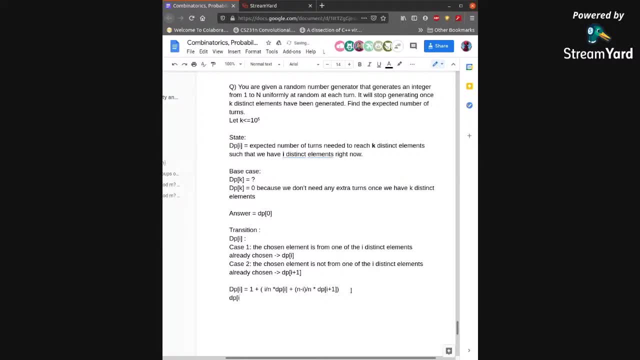 what will be the answer? dp of i by n into 1 minus i by n, equal to 1 minus i by n into dp of i plus 1.. And this again you can get loose n minus i by n Press 1.. 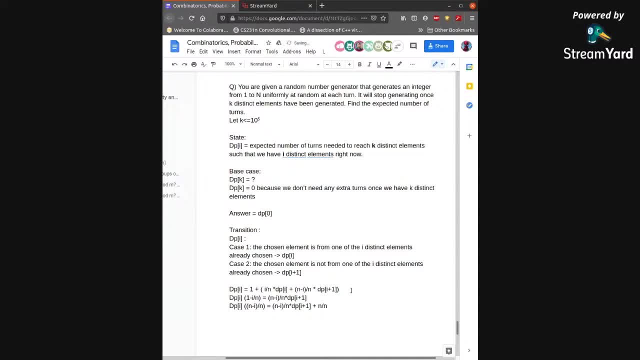 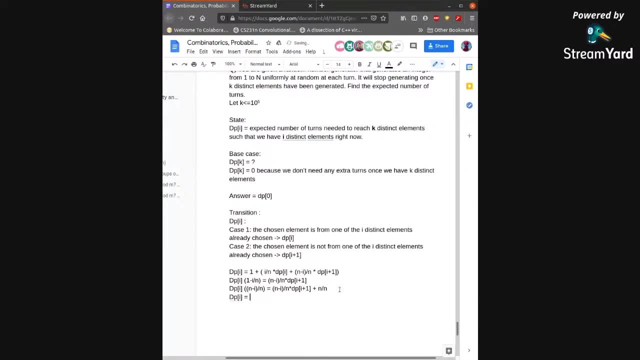 And it says n by n instead. Now, if you remove this n by uh minus i by n, Then dp of i will become equal to dp of i plus 1 plus n by n minus i, I think. so I'll just write it one more time and check. 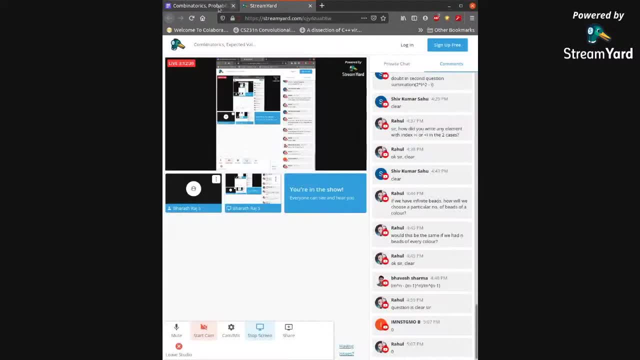 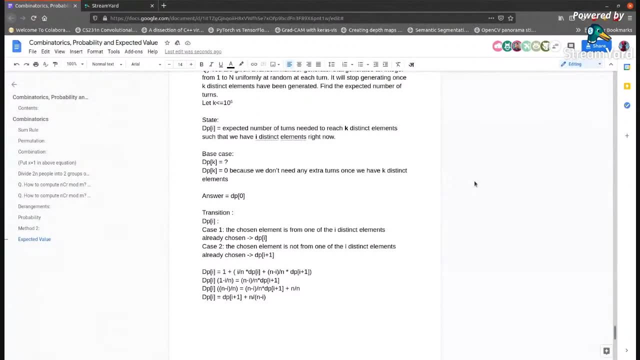 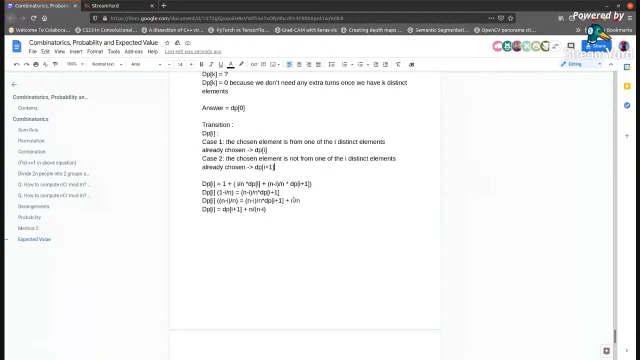 Yeah, it's correct. Yeah, i equal to dp of i plus 1 plus n by n minus i, And this you can calculate in order of k time complexity. So again, if you have any doubts anywhere in this expected value, you can type in chat. 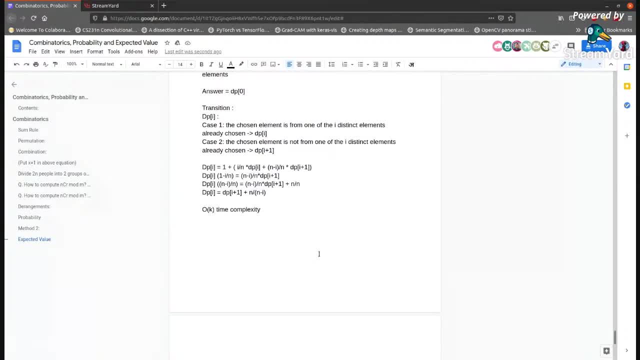 This is not an easy problem. definitely Because actually there is another way. Instead of using dp of i and the transition to i plus 1. We can transition to dp of i from i minus 1.. But that dynamic programming will be very difficult. 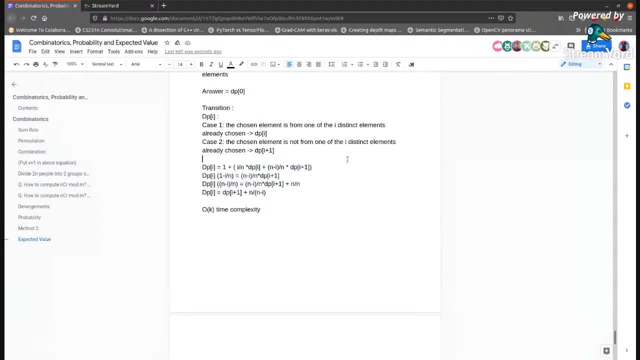 I mean, you can try it yourself. You will get something like an AGP And it will be very difficult to solve. But if you use this method you will get this nice recursion: dp of i equal to dp of i plus 1 plus n by n minus i. 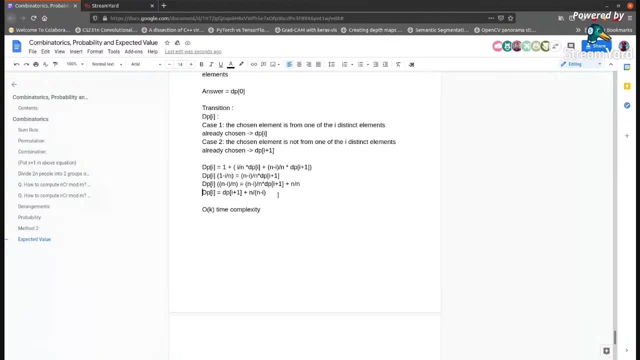 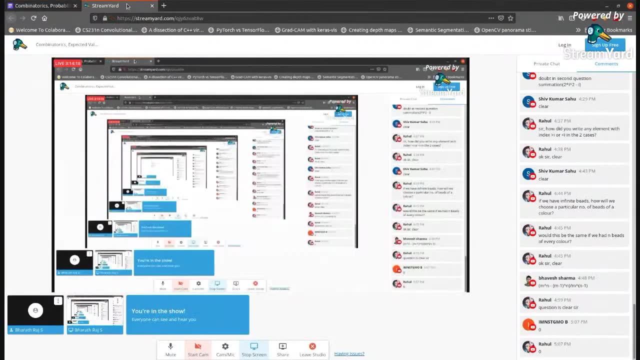 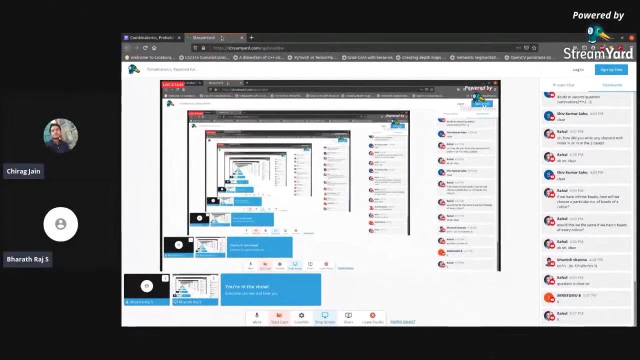 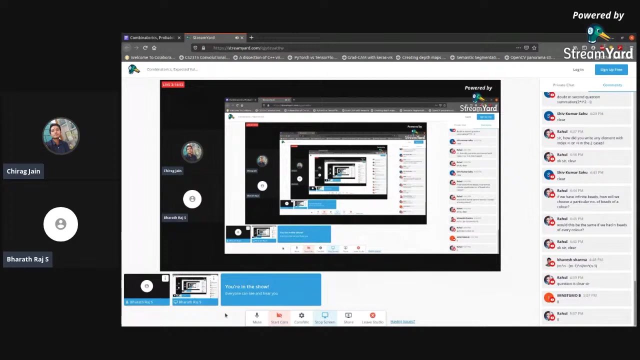 I hope it is clear. If you have any doubt, you can ask. I hope it is clear now Any questions? No, Okay, Thank you for your time. Okay, so if it is over, then just I want to just make one correction, which I told that 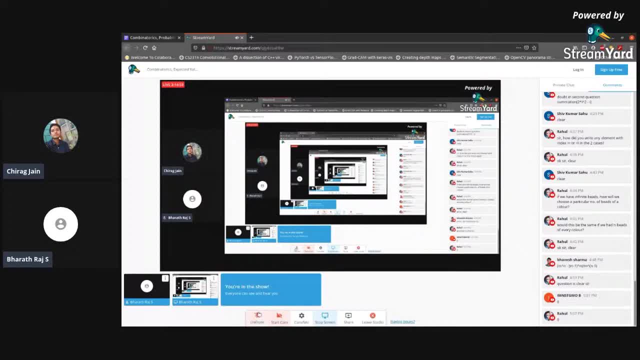 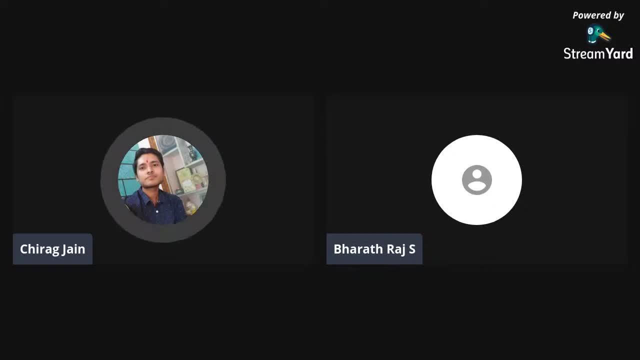 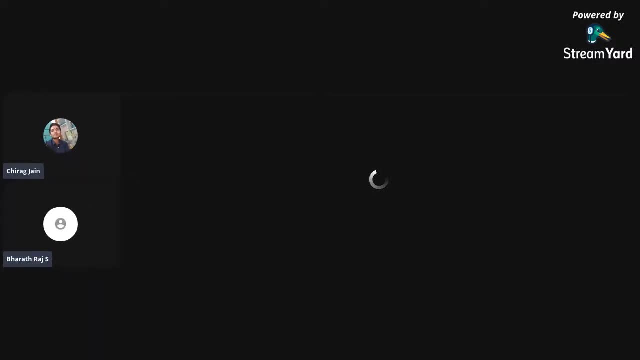 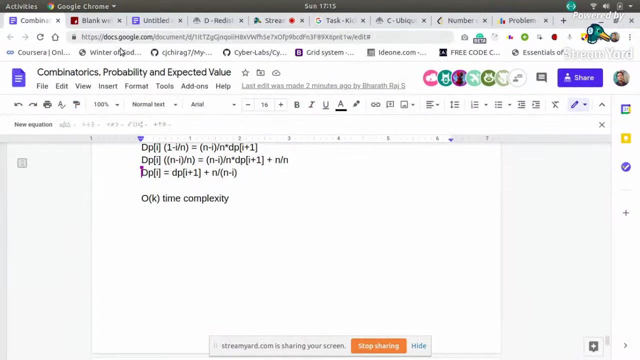 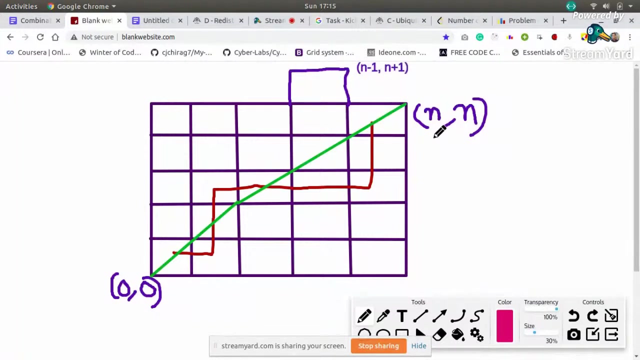 I told I will discuss at last. So so okay, just I'm sharing my screen, Okay. so uh, just what I told was, if we want to reach this place n n From zero comma zero, Let us consider any invalid path. So I'm just discussing that thing again. 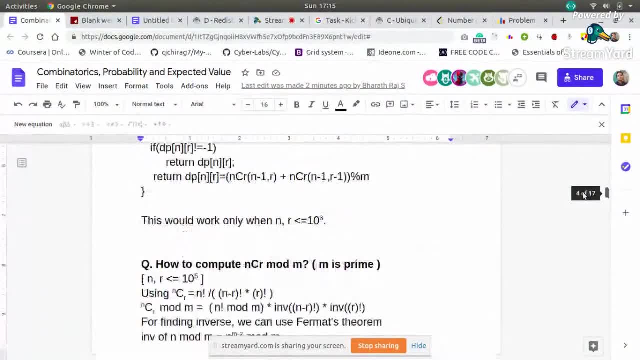 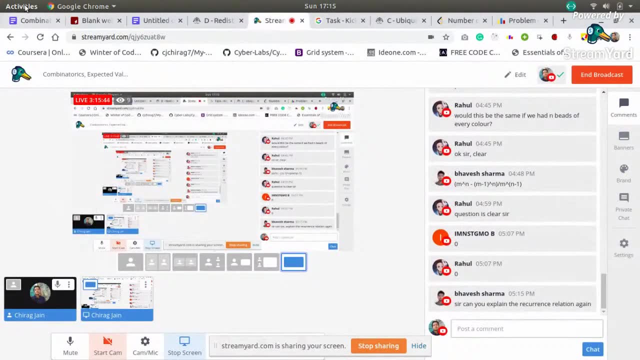 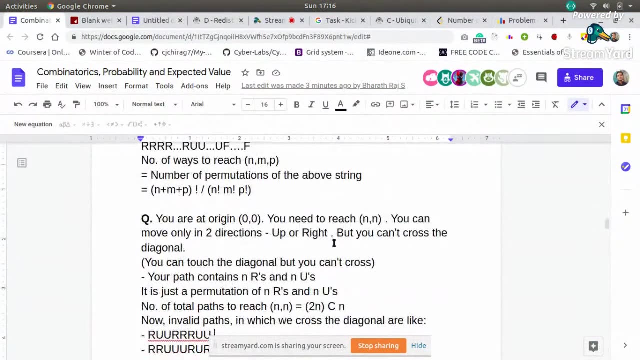 So we want to. our aim is to find out how many paths are possible if you want to reach n n from zero comma zero. Okay, I hope I'm audible. So this was our question, ki, we do not need to cross the diagonal matlab, we need to find. 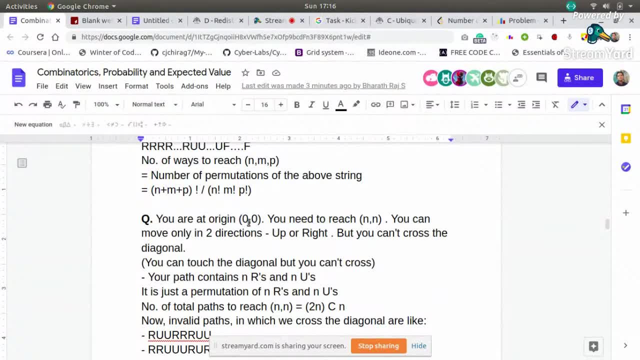 all such paths, such that we need to reach this place: n comma, n from zero, comma zero, and we can move only in two directions, either up or right. Okay, So, for example, if you can see here like this and let's say n comma, n from zero, comma. 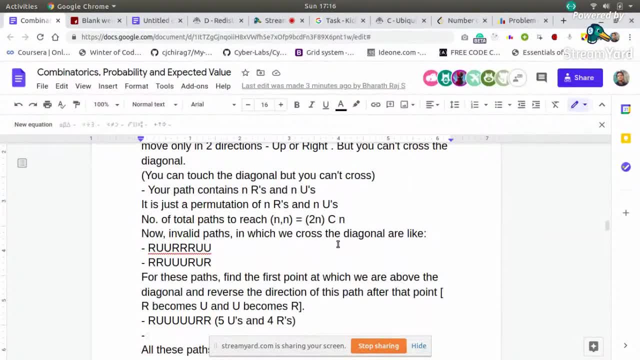 n is the path of q, c square, but you can't cross the diagonal. You can touch the diagonal but you cannot cross it. So just for first, we know the total number of paths will be always 2n, c n. total number of paths to reach this: n comma n. 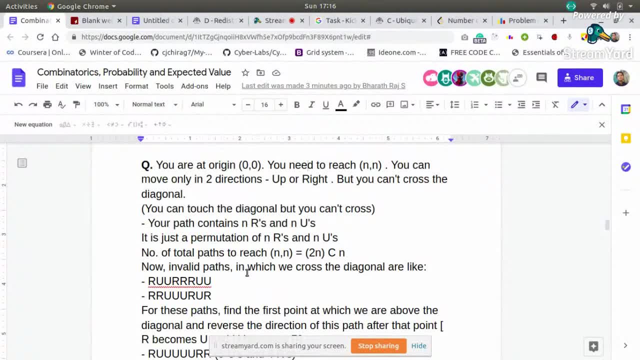 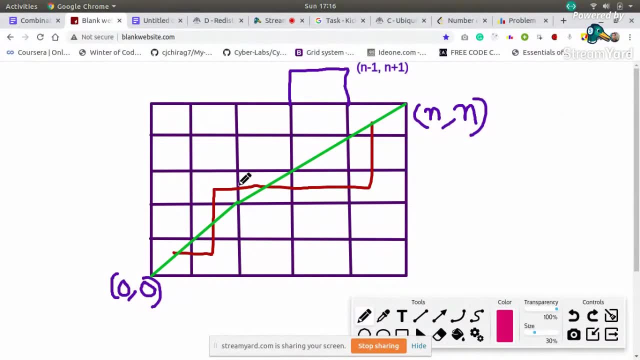 But we will just subtract the invalid paths from that. So what are the invalid paths? So, invalid path, one of the inverted path is this like this: r u u r, r, r r? u? u. So this I have drawn: r? u u r, r r u? u. 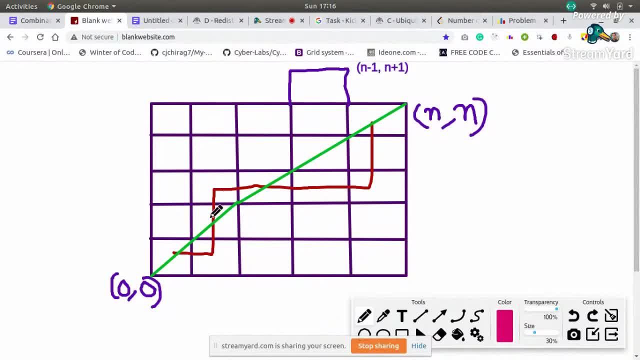 So this reaches n comma n. So this is an invalid path because it just crosses the diagonal. Okay, but it is also crossing it to one point above. so what is the indication that it is crossing, whenever you will find that at some prefix the number of u is more than the number of r? 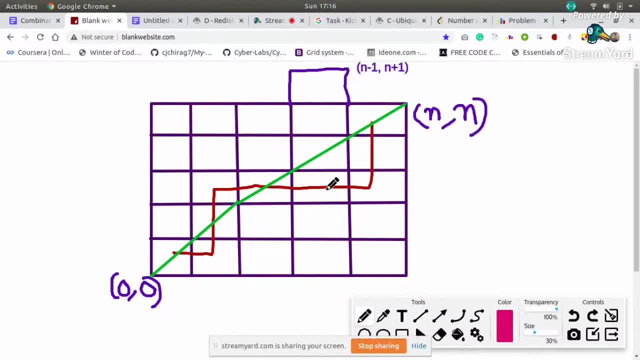 it means that it is crossing the diagonal. so okay, this is one invalid path. so just for every invalid path we can do one thing: that at that point, when it is just above the diagonal, it's fine up till now, but after this point, just reverse everything. reverse means this right will become up. 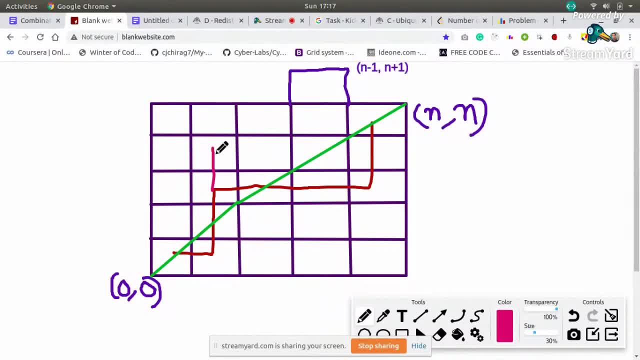 so it will be this from now: this again, one more right is there, so it will become up. so up will become right and right will become up. so, from this point, start reversing all the things. so this again, this right will become up, like this. now, this up will become right, like this: this again, this up. 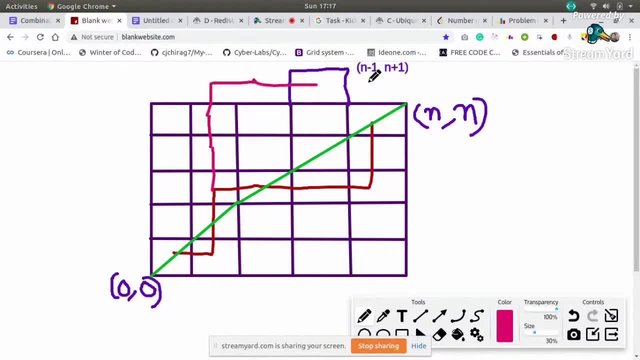 will become right. so you will reach this at this cell always, which is whose coordinates are. you can see, since the uh, you can say the row number is n minus 1 and column number is n plus 1. also, or x coordinate n minus 1 and y coordinate is n plus 1. 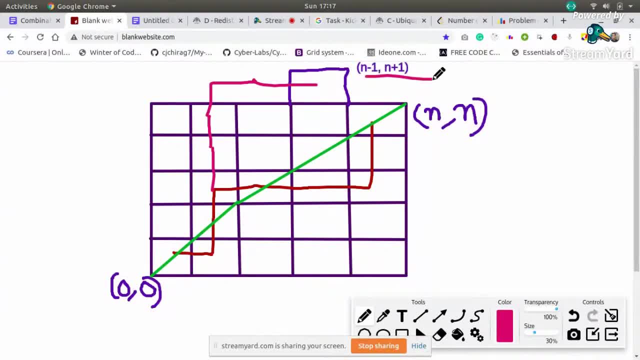 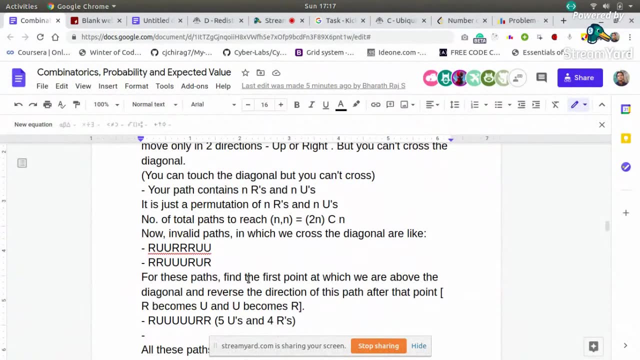 something like this. so we will always end up reaching at n minus 1 comma, n plus 1, take it so you can do it for any other path, like let me take any other example. so like, apart from this, if i, if i had, my original path is this, so i have written this thing here also, like find the first. 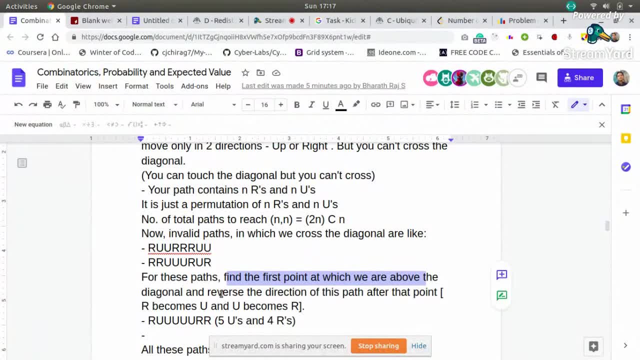 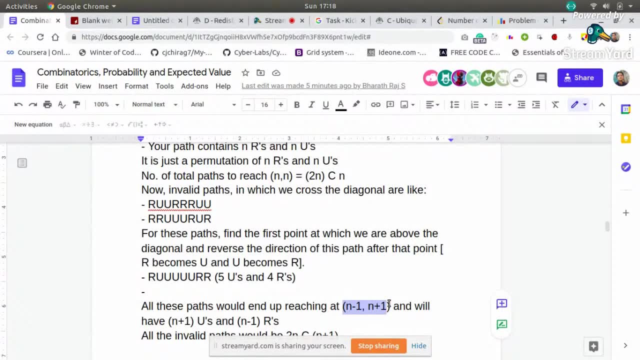 point, which is about the diagonal, and just from that reverse the direction, so you will become r and r will become u. so if you do this, so you will always end up at this position: n minus 1 comma, n plus 1 and n minus 1 comma. n plus 1 means that you need n minus 1 r's and n plus 1 u's. so number 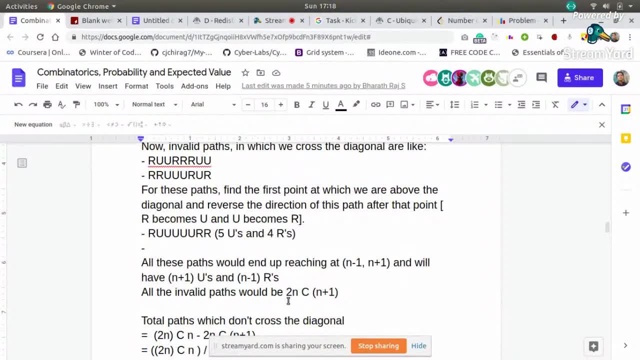 of u will be more and number of r will be less, something like this. so the total number of the total permutation of this path will be: since if you sum up the these, you will get n plus 1 plus n minus 1 will be 2n, 2n, c, n plus 1. you will find this because total permutation will be n plus 1. 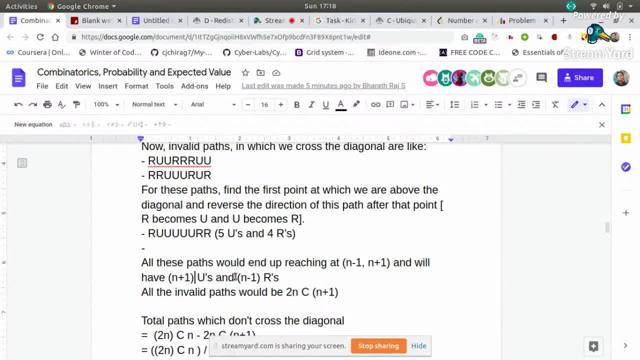 plus n minus 1 whole factorial divided by n plus 1 factorial divided by n minus 1 factorial, so it will be equivalent to this thing. you can try with this path also. let me try with this path. so r r, triple u r u r. so if i draw this path, this is my invalid. 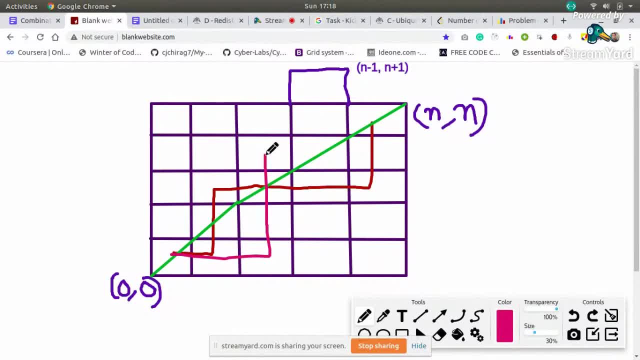 path r r triple u. so see r r triple u means the number of u is 3 and number of r is 2, so at this prefix the number of u is more, so it means it is definitely an invalid path. r r triple u, r u r. 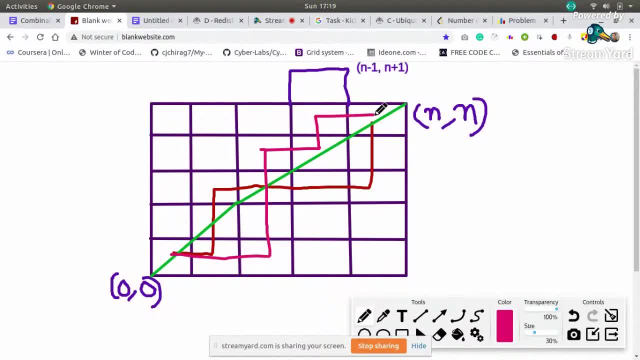 r, u r. this is my invalid path because it is crossing the diagonal. i don't want to count this path. so for every invalid path, i told you just what you do at that point when it is just first time reaching above the diagonal. at this point, just reverse all the things means r will become u and u will become r. or you can say this: 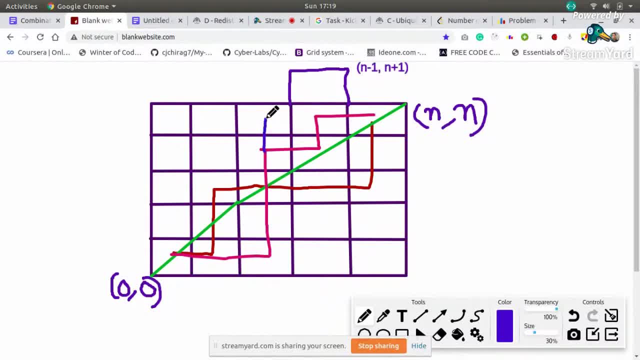 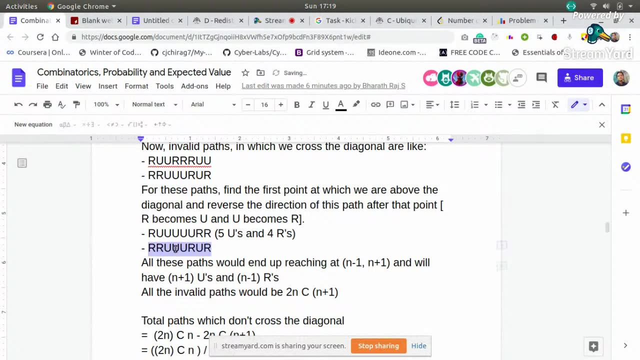 right will become up, and this after this right, this up will become right and again this right will become up. so i have written also this in the form of string. so in this form of string, if i write so, it would be something like up till this point. it will be same, because it is just crossing the. 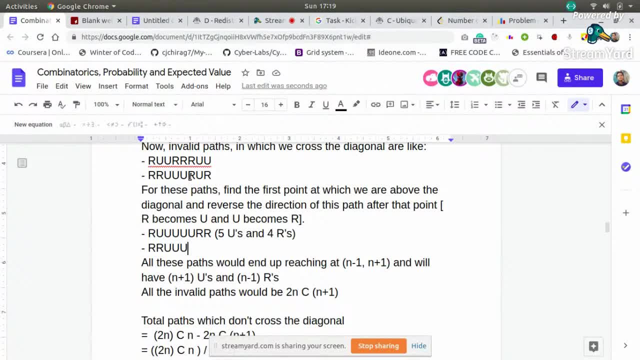 diagonal at this point. so up till this it will be same. from the next point i will just reverse it: r will become u, u will become r and r will become u. so this second path becomes this. just, i am doing this for every path, so you will find this also ends up reaching at this position, at this coordinate. 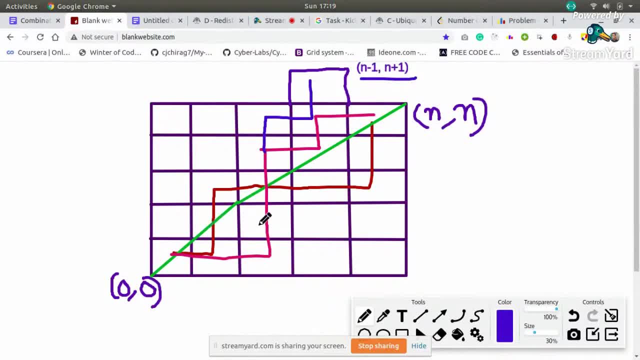 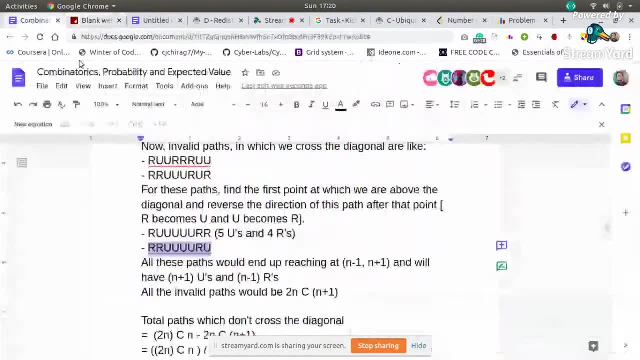 n minus 1 comma, n plus 1. so you will find that every invalid path can be written as the number of ways to reach this position: n minus 1 comma, n plus 1. so the number of ways for this is. i already told, told you that it is at 2 and cn plus 1. so that is. 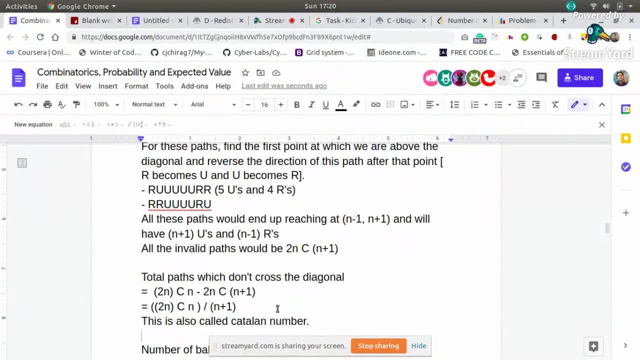 where the total number of path which do not cross the diagonal will be equivalent to this, and these are also called dyke paths taken. so this is the name dyke path, so this is the formula for that and this is equivalent to catalan number. this i told you and similar thing is valid for, if you think, in. 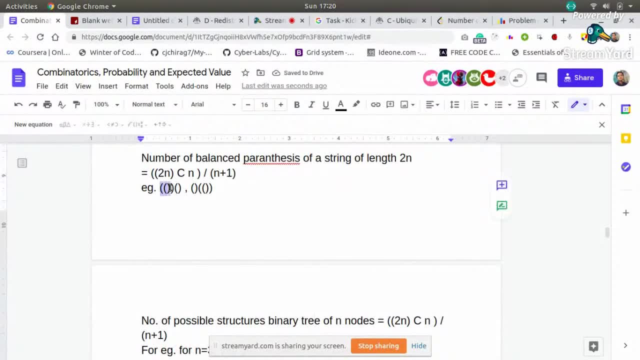 the term of bracket also now. so for bracket also, you think that for every invalid parenthesis and and for every invalid balanced parenthesis which are not balanced, you will find that one prefix for will contain one extra right bracket. So from that right bracket you try to reverse all the remaining brackets. 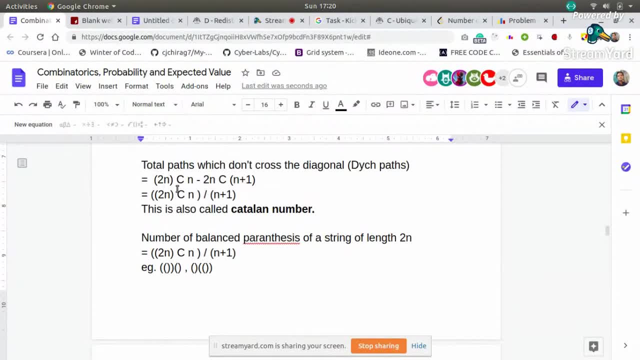 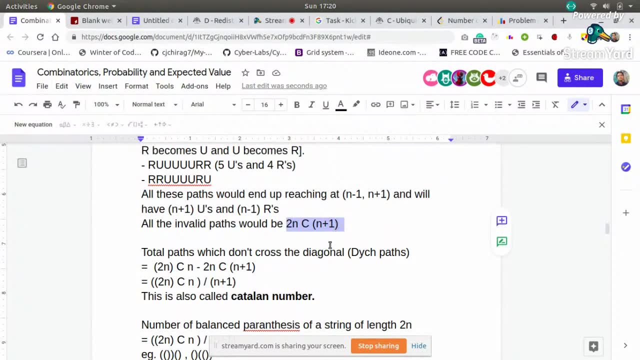 And you will find a similar pattern there, So you will find a similar number of permutations can be formed. You can derive a similar thing for brackets also, So for bracket also this thing be equivalent to 2nc in. So this is Catalan number. 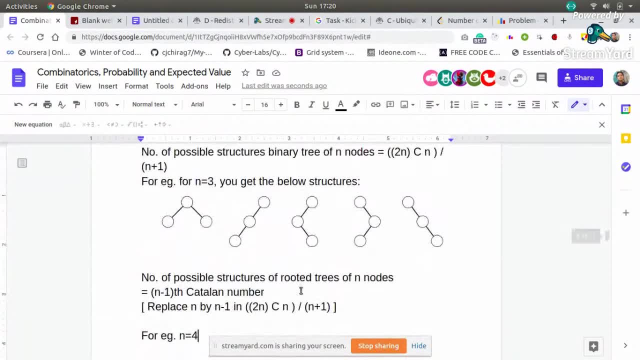 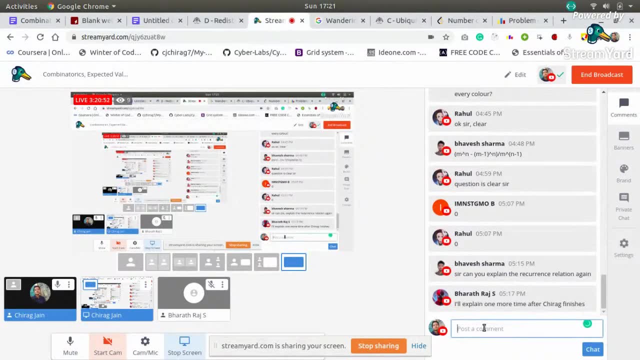 One thing was this: Some practice question I want to give you for combination. So this is one good question which was asked in Google Kickstart, So I will send the link in live chat also, You try it by yourself. OK, I will just give the practice questions. 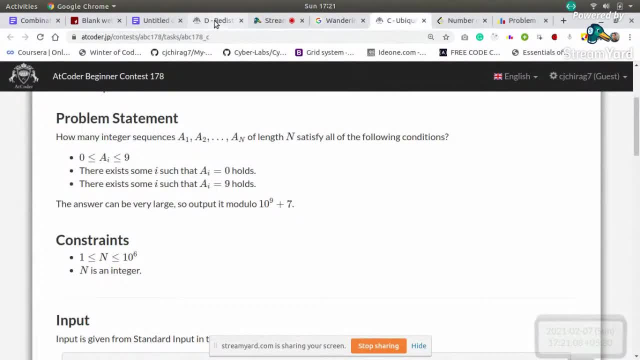 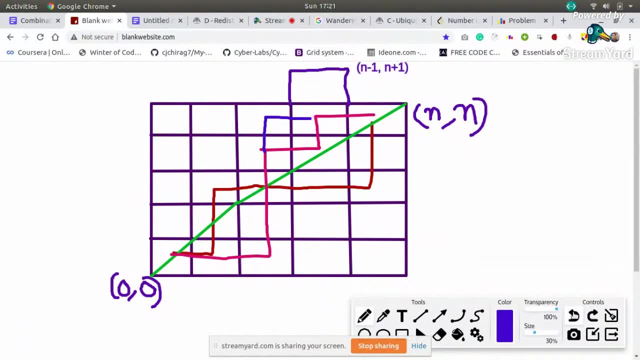 So these two, three are there, So one is this one. So in this problem, I will just explain you the statement in short. So the problem is something like that: a grid is given to you And you need to reach this n comma n from 0 comma 0.. 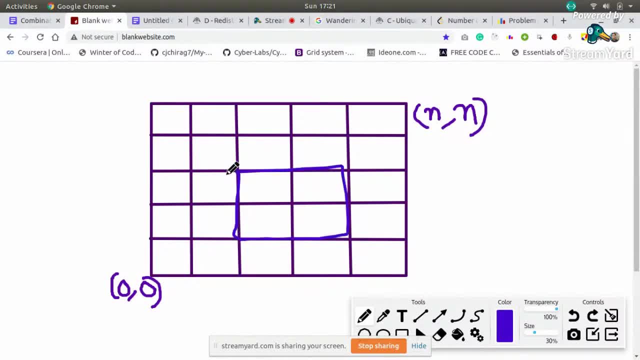 But there is some rectangular hole. you can say: So there is some hole like this. You cannot reach this place, Something like this, And you can see this. You can say that you need to find the probability that the person starts from here and reaches this point. 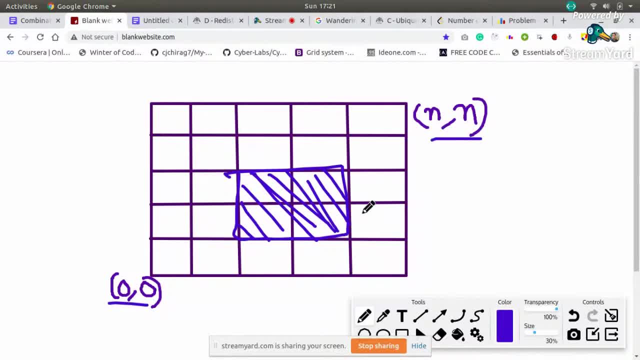 without falling into this hole. He doesn't move into this hole any time. So this was asked in Google Kickstart round C, I think. So I will share the link. So you try to solve it by yourself, But the problem is that if you try to solve it, 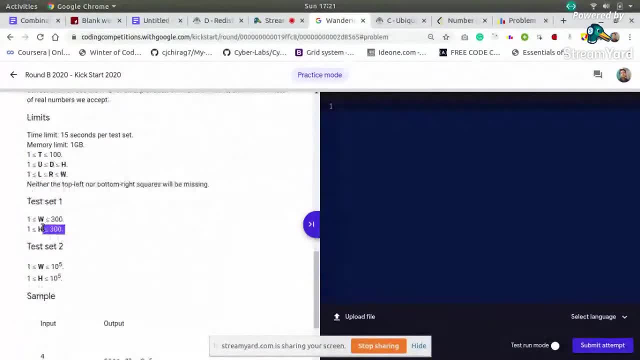 by using dynamic programming, then only test case one you will be able to solve, in which the constraints are very less, where this height and width of the rectangle is less than or equal to 300.. So this will be. you will be able to solve using dynamic programming. 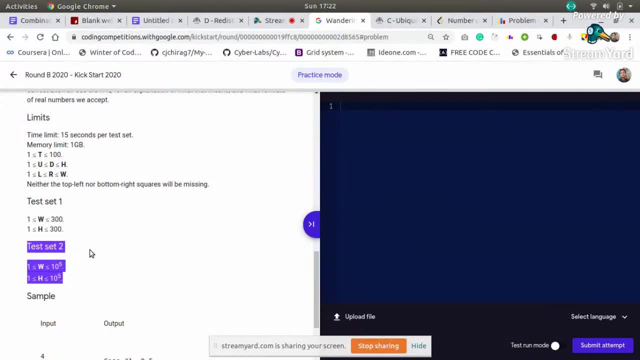 But this test case two: if you think you need to think of combinators, Then only you will be able to solve. So try to think of your own. But just one hint I will give you If you are facing difficulty for overflow, because NCR value would be very large. 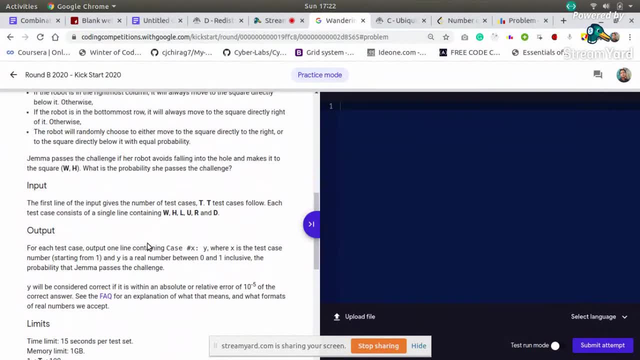 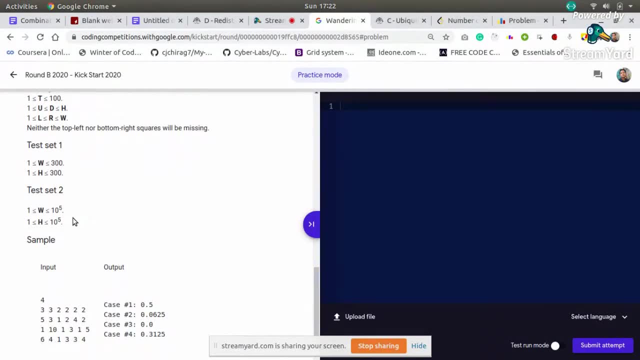 And here you do not need to find the mod of NCR, Here you need to find the probability. So basically, the values will be very large. So just try to find the logarithm of NCR or logarithm of the factorials. 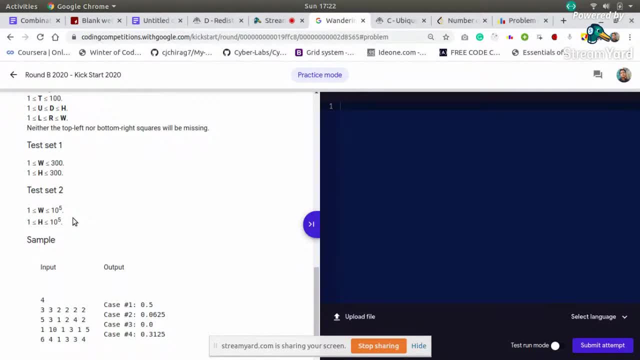 OK, So because the logarithm will be very small value, so it will not overflow And you will get accurate result, you can say So in terms of logarithm, if you try to solve it, you will be able to do so. 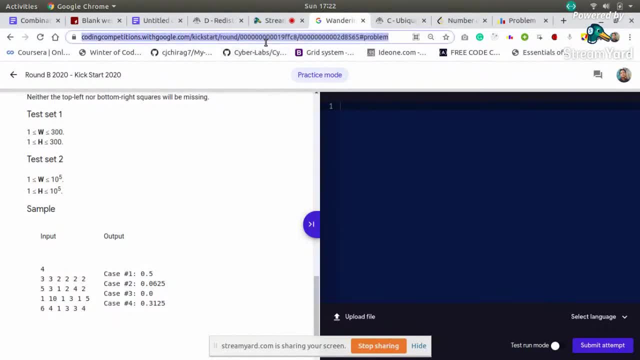 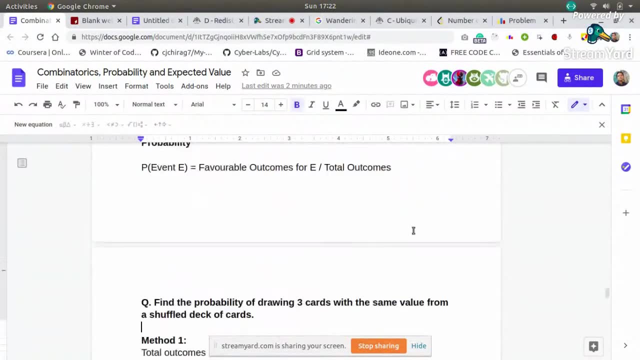 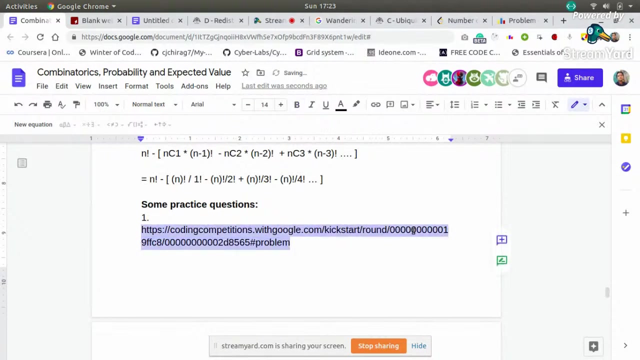 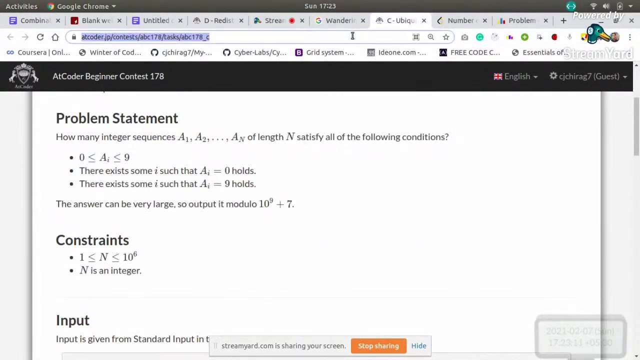 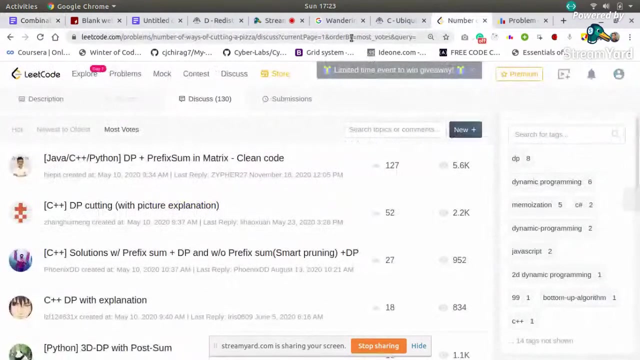 Try to practice it. So I will just share the link: some practice questions. So one is this one And one is this one. see this one, try to solve it by your own. And one more problem is sometimes in problems of dynamic programming. you will find that 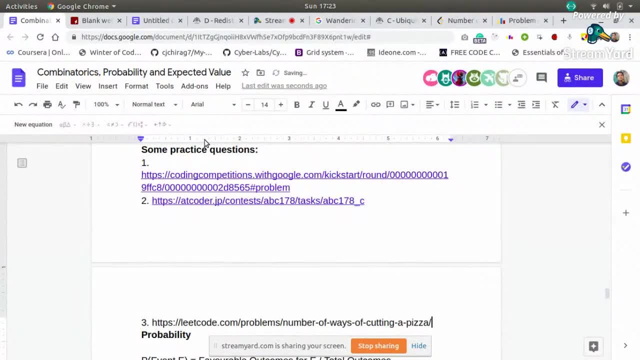 sometimes means, in problems of means which will be combinatorics, dynamic programming can be used. Dynamic programming can always be used in such type of problems. In most of the times you can solve by dynamic programming. So try to solve by any one of them, either combinatorics or dynamic programming. 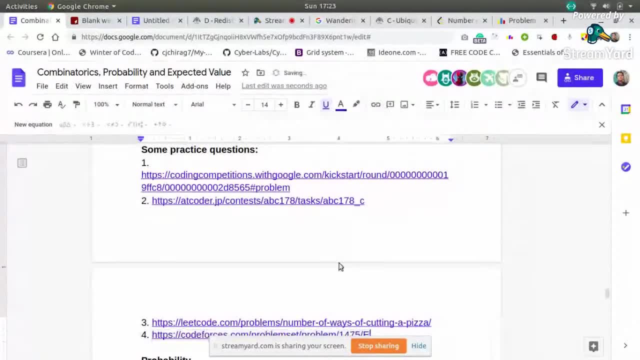 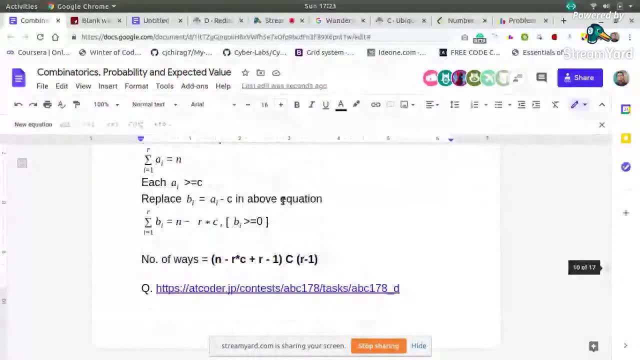 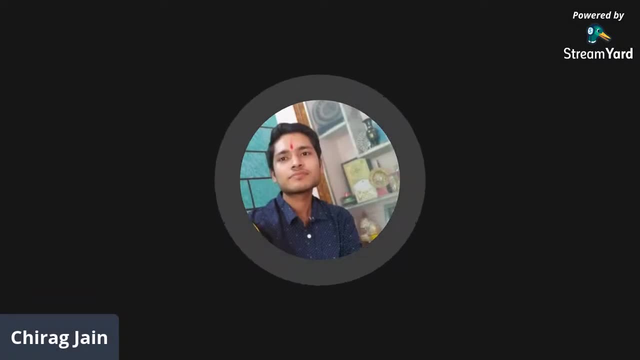 So these four problems I wanted to give Now I will just hand over to Bharat. And this dive path is clear or not, you can write it. if you understood it or not, Take it. So, Bharat, you can share your screen now. 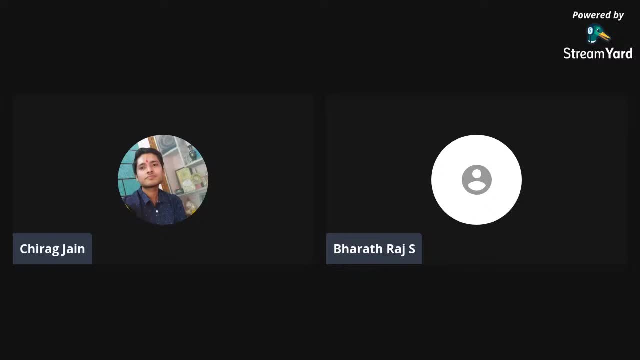 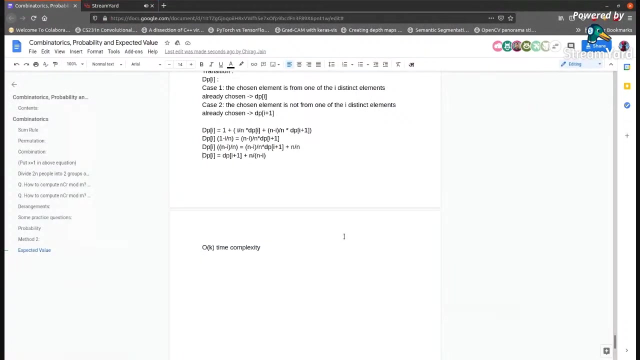 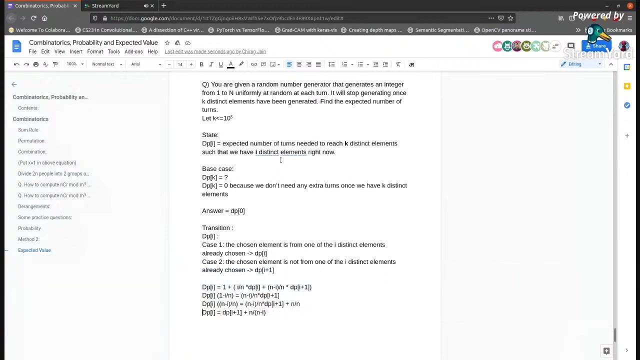 OK, OK, I think the screen is visible, so let's see So. first, the DP state state is: you are having i distinct elements. What is the expected number of turns you need extra how much? how many more turns you need to reach k distinct elements? that will be your DP state. 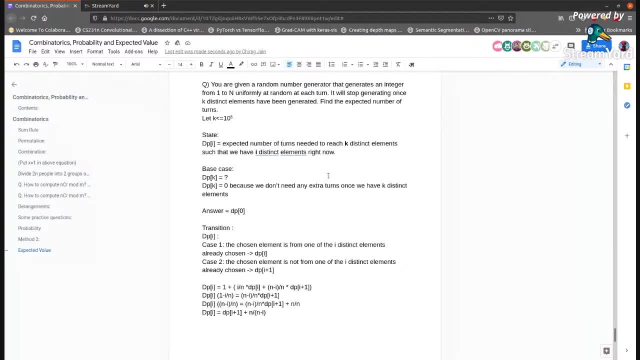 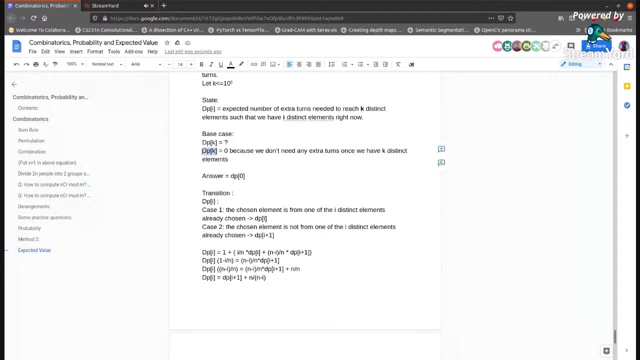 This expected number of turns, expected number of, let's say, extra turn needed to reach k distinct elements, such that we have i distinct elements right now. So obviously the base case is DP of k will be zero, because once you have k distinct elements, 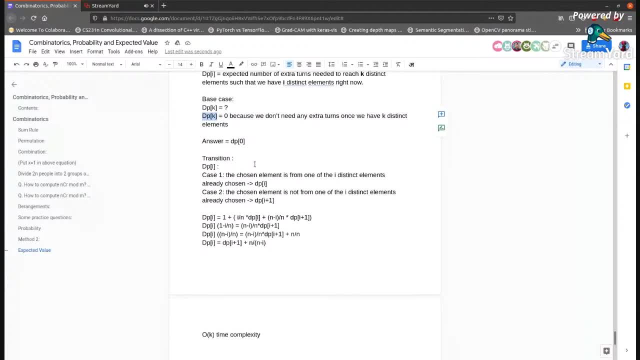 you don't need any extra step. That will be zero And for the transition, so if you are having, if you are choosing one of these i distinct elements. so this is just I'm taking some random i elements, So one, two till i some i elements. 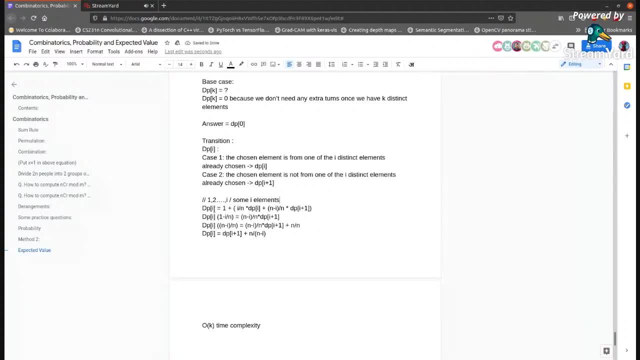 And these elements have been chosen. Now, if you take any one of these elements, one or two or any of these i elements, you will get k distinct elements. Now, if you take any one of these elements, one or two or any of these i elements, you will get k distinct elements. 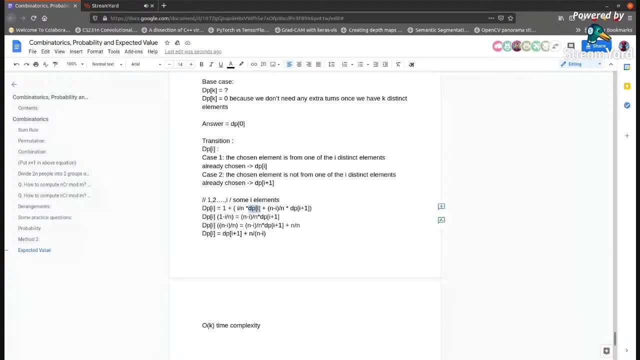 Then you will still need a DP of i This many number of extra steps. right, That is definitely. you have to perform one more extra step, That is, once you have i elements, i distinct elements, you have to choose one element And that element. after choosing that element, if it is one of these i elements, then you 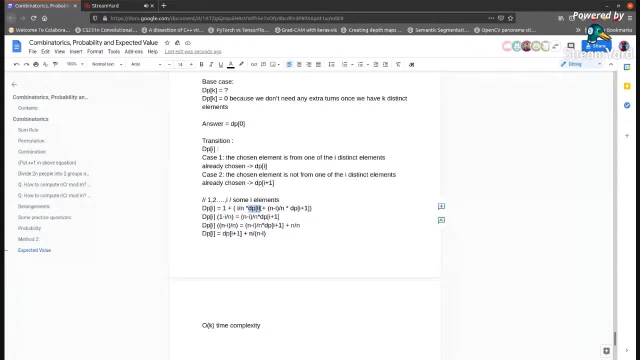 will still need these many extra steps- DP of i number of extra steps- And if you don't choose These i elements and you have chosen some other new element, then in that case you will have i plus one distinct elements And once you have i plus one distinct elements, this will be the probability of choosing that. 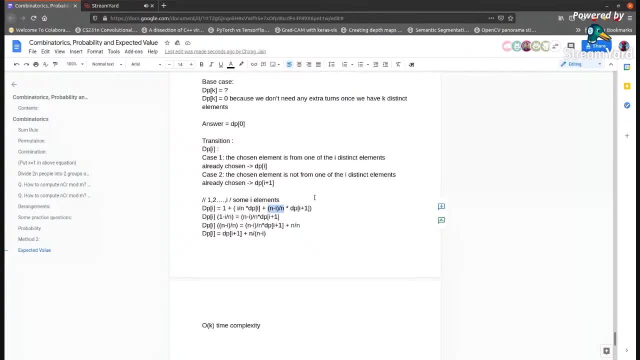 That is any number other than these i elements, And after that it is just simplify. This type of DP may be new to you because I think till now you have seen DP transition from one state to another, not from a state to the same state. 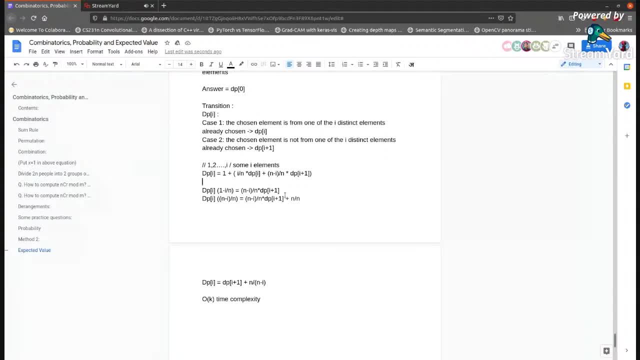 And this type of transition will not always have a solution. It will have a solution only when this n minus i, that is that this n minus i. only if it is non-zero it will have a solution. So just keep that in mind. 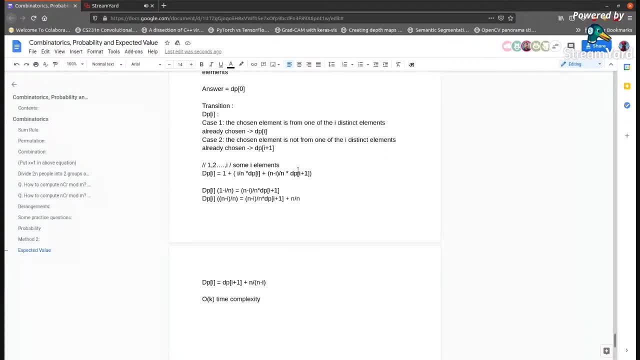 So is that clear? now? Treat expected value, just like that, in the literal sense. don't think about the mathematical values. Is it clear, Bhavesh, or anyone who has doubt? But if you have any doubt, just specify which part exactly. okay, then if anyone else is. 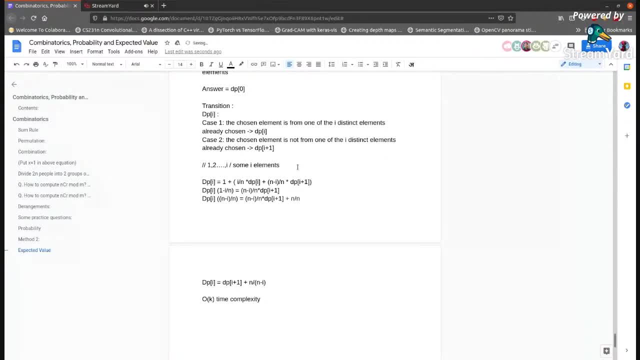 having a doubt, just specify that part and clear. Otherwise, Why do we need to add one? Because you are having i distinct elements and at each turn what will you do? You have to add one turn, right? Suppose say you are having, suppose, zero elements initially, then what will be the transition?